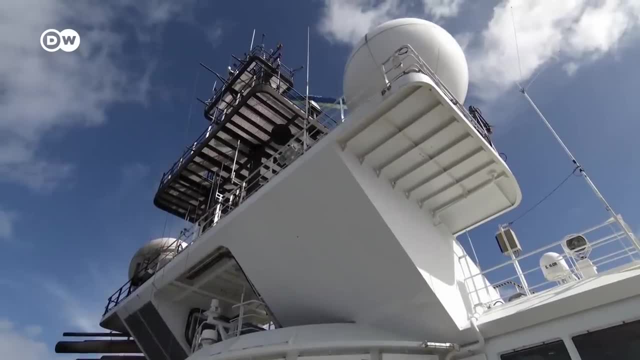 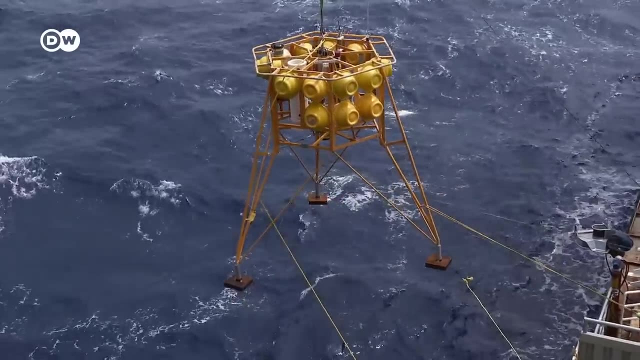 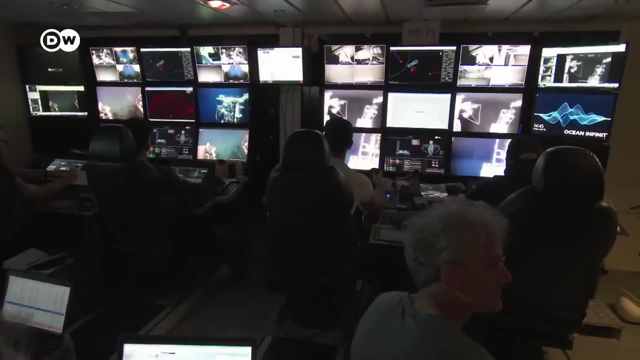 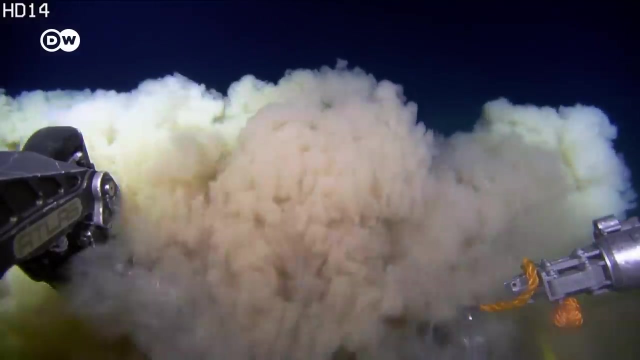 In the middle of the Pacific Ocean, an ambitious expedition has set out to explore the deep sea, Going where no human has ever gone before, Where enormous deposits of minerals lie dormant. Can humanity benefit from this untapped source of wealth? The technology to harvest it already exists. 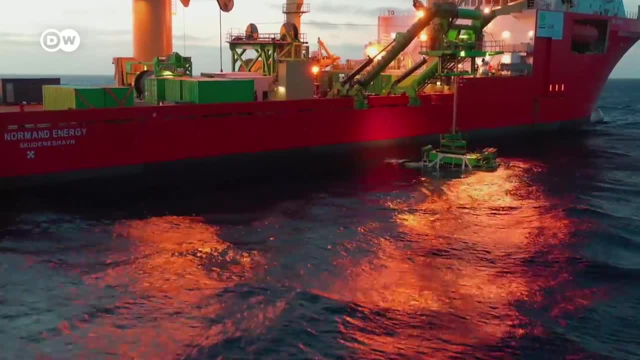 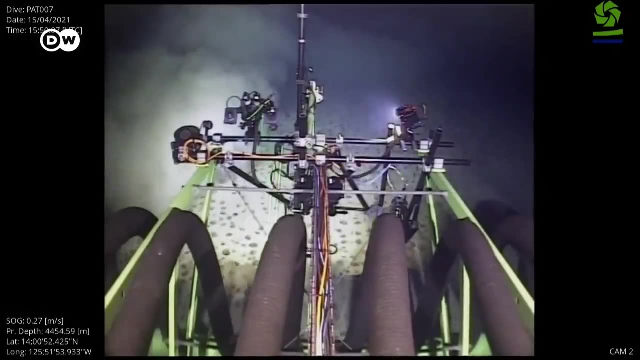 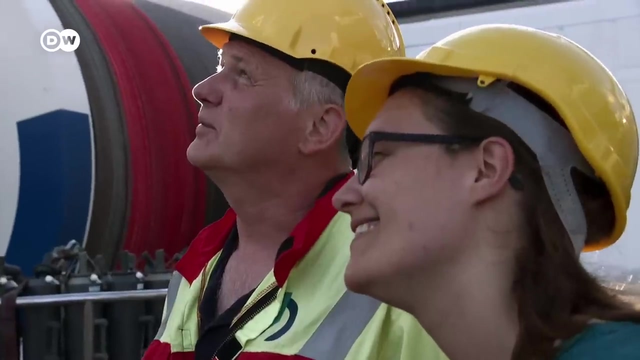 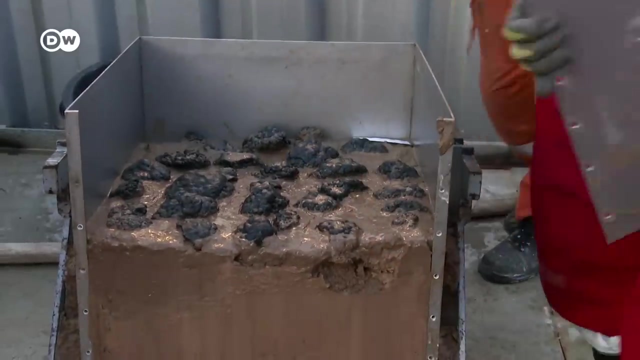 The first prototype of a deep sea collector for the treasured stones is called Petania. It's being tested at a depth of several thousand meters. Scientists are monitoring its deployment Because what is technically feasible may actually destroy a delicate underwater world. But is it worth the risk? 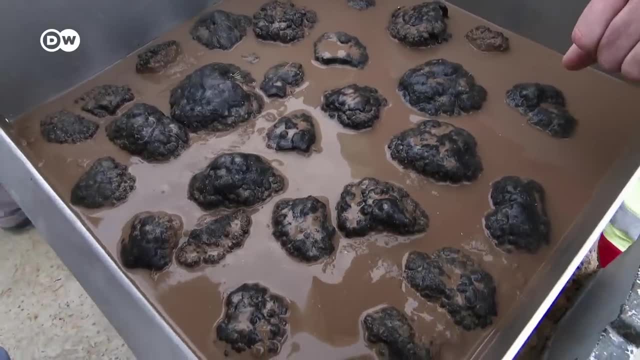 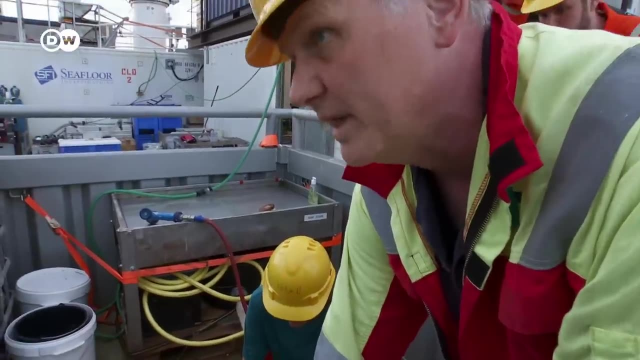 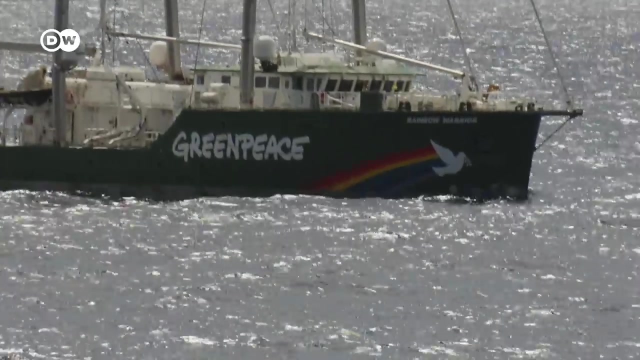 These are basically batteries in stone form. This is exactly what you need to build a battery. There's manganese, nickel, cobalt and copper to conduct the electricity. Environmental protection organizations such as Greenpeace want to prevent deep sea mining at all costs. 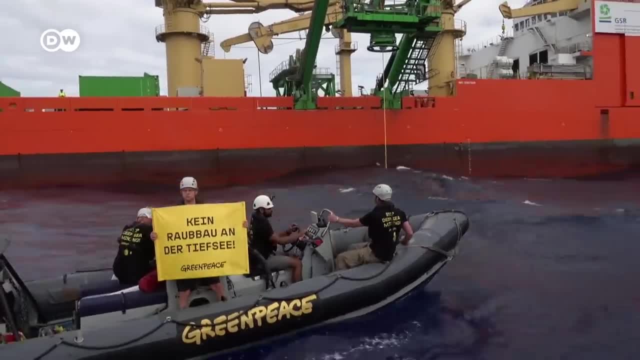 It's the last part of the planet that humans have yet to see. But what will happen if nation's ES huge米 don't achieve their potential? So the biggest question is that humans have yet to exploit for resources. Are the oceans in danger? 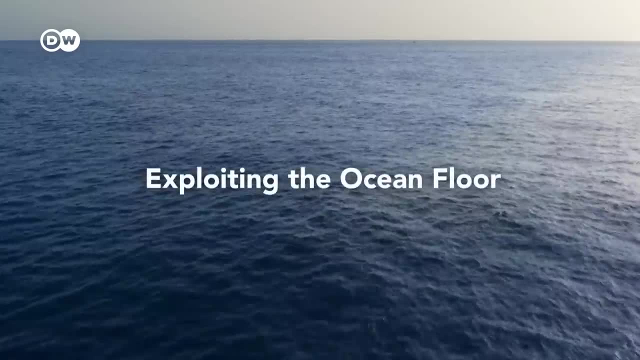 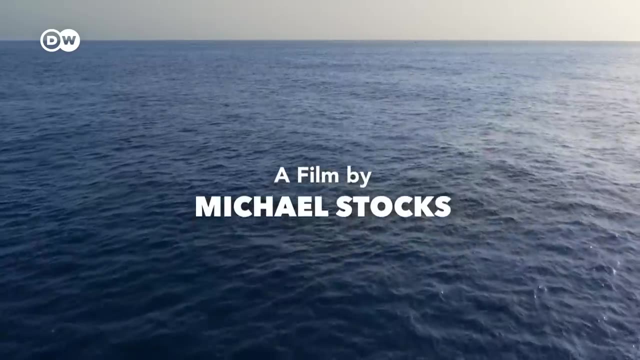 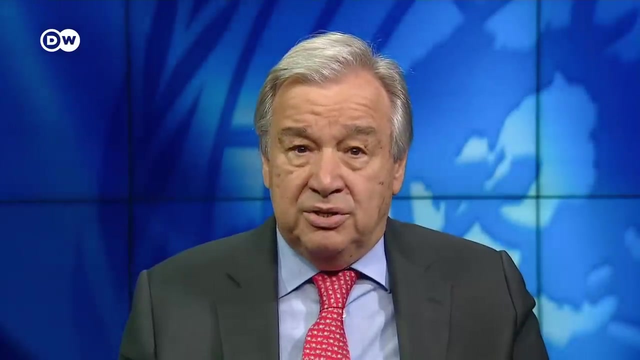 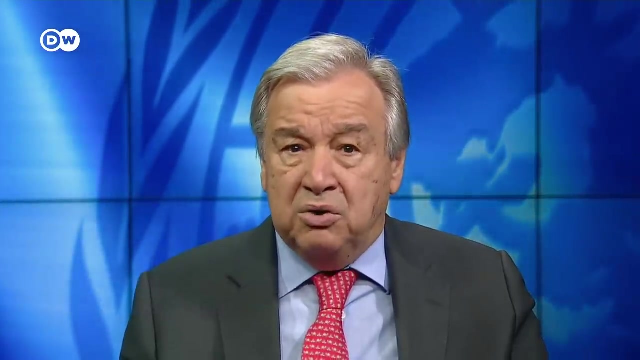 For more UN videos, visit wwwunorg. losangeorg 8app IY1- reuse gee. Making peace with nature is the defining task of this century. Preserving and restoring the ocean's ability to nurture humanity and regulate our climate will be the defining challenges of this decade. 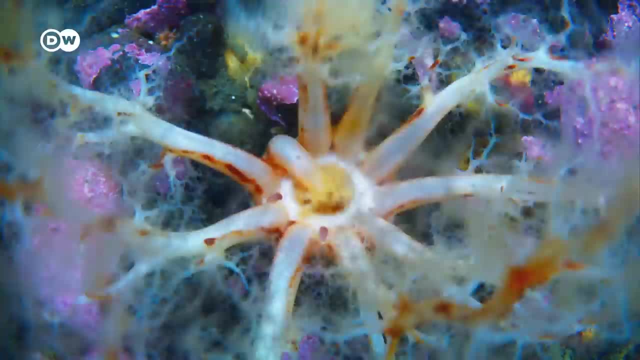 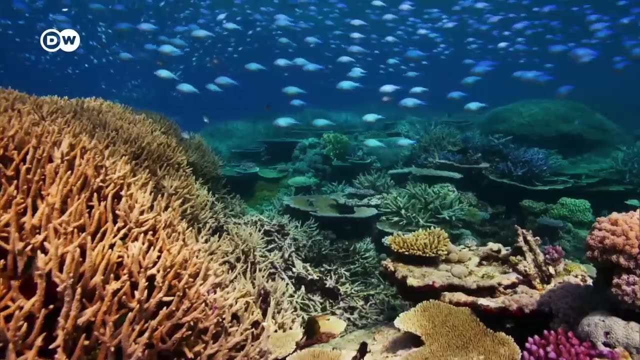 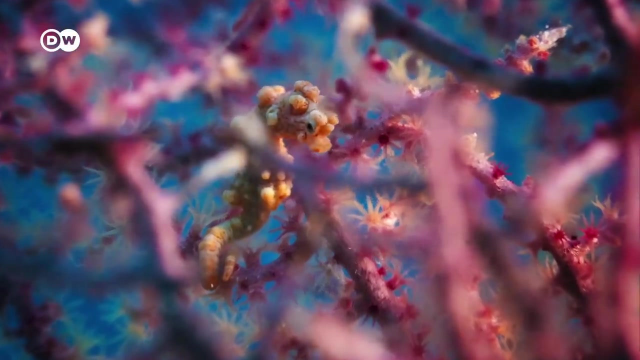 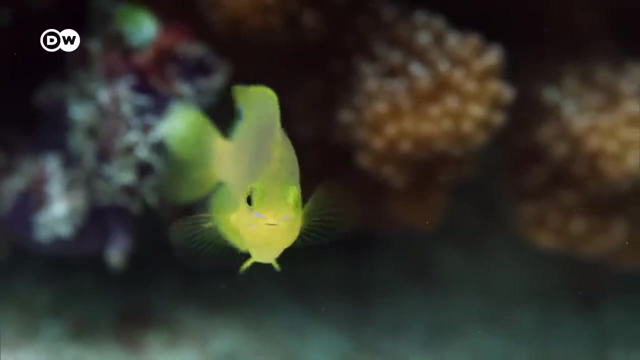 71% of the Earth's surface is covered by oceans. It's the largest habitat on the planet. The oceans serve as an important heat buffer and carbon sink. They absorb about a quarter of man-made CO2 emissions and thus mitigate the effects of climate change. Planet Earth needs the oceans to survive. They regulate the climate, they provide food, they provide the oxygen we breathe- More than 50% of it, by the way- But the oceans are not the only thing. the world's oceans are suffering. 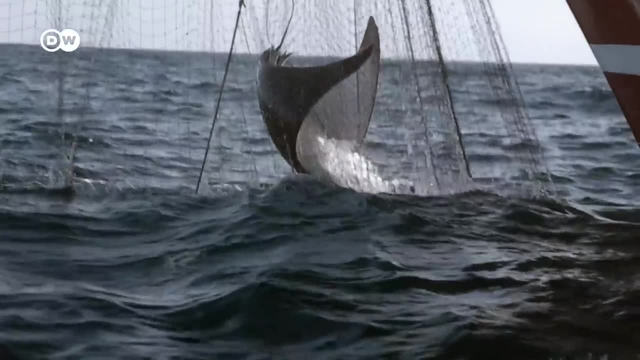 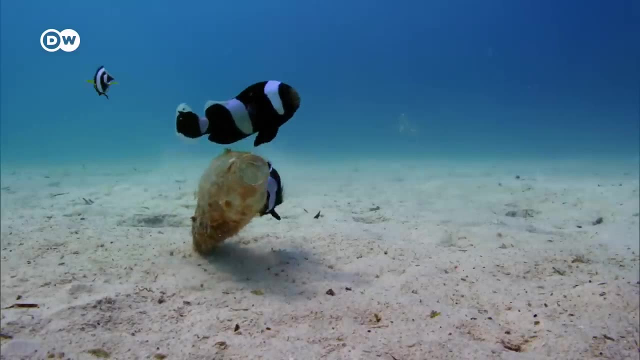 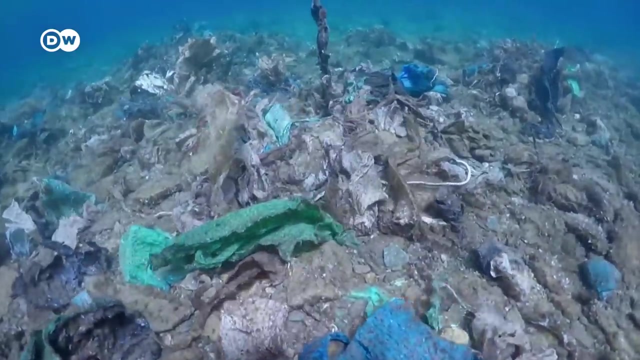 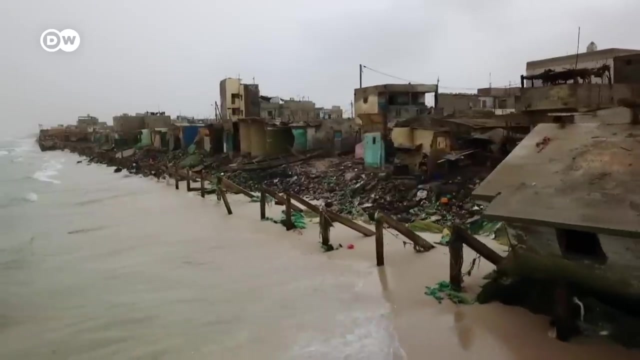 They're ruthlessly being fished bare. The waste produced by an increasingly affluent society is becoming more prevalent in the water. Virtually indestructible plastic waste endangers animals and their habitat. So-called ocean dead zones are getting ever larger. Climate change is also causing sea levels to rise. 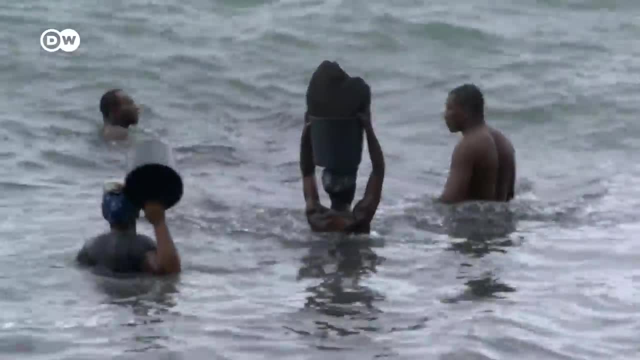 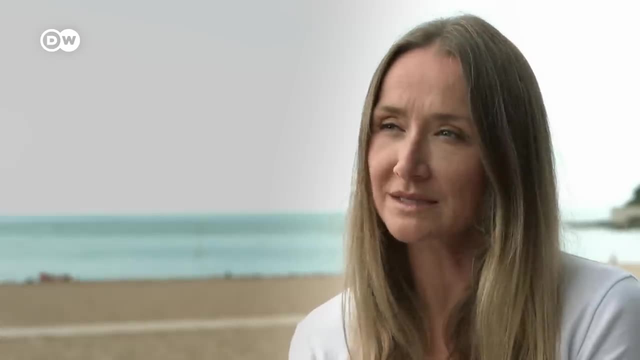 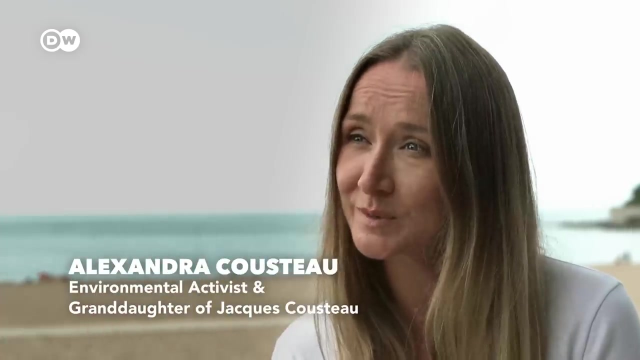 Nevertheless, its exploitation continues. Sand and gravel are being dredged for use as building materials At this point where we've lost 50% of our ocean, 50% of the whales and the fish that lived in the ocean when my grandfather first started scuba diving. 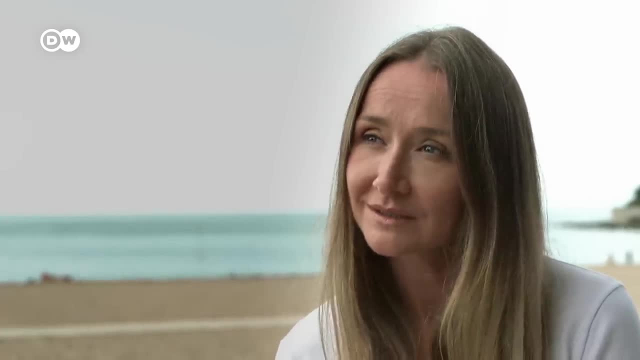 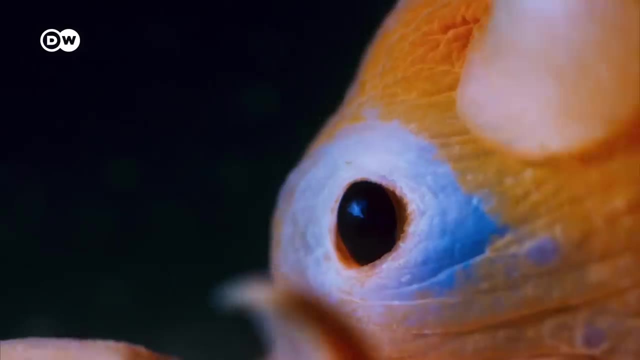 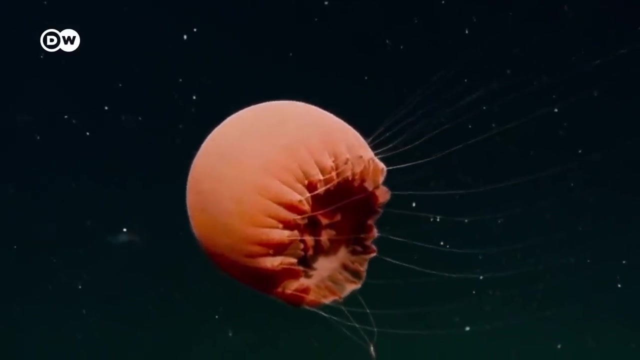 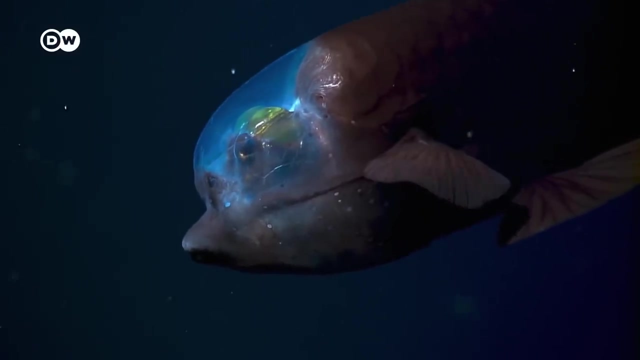 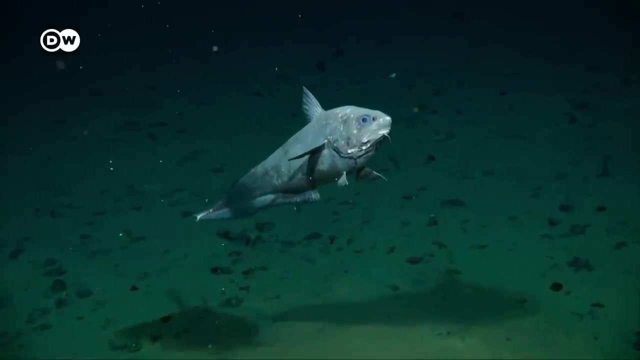 after the Second World War have disappeared. Now we're exploring barely researched places that are still quite inaccessible. We know almost nothing of the plant and animal species living there. Yet we're aware there are resource-rich nodules on the seabed. They're made of cobalt, nickel, manganese and copper. 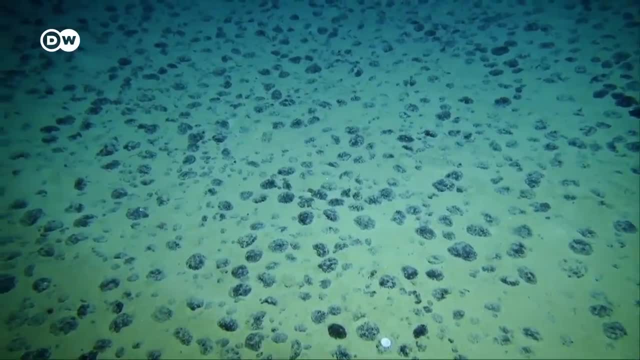 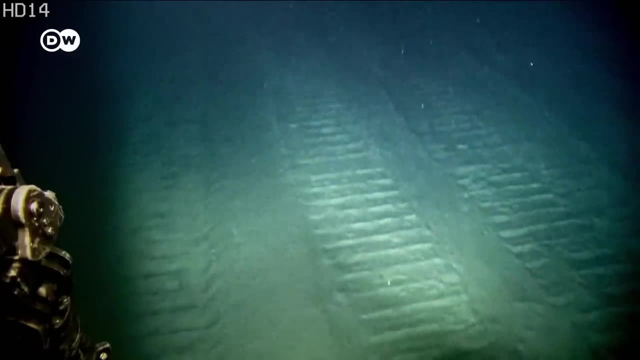 Just the materials to meet the rapidly growing demand for batteries. as the world shifts away from fossil waste, Getting metals from our planet can't be done without any environmental impact, So what we need to be thinking about is how do we make decisions that cause least harm? 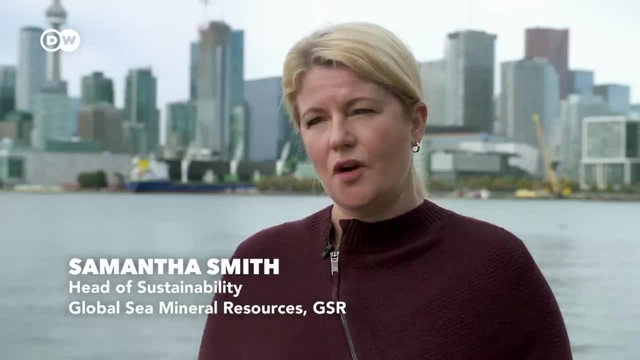 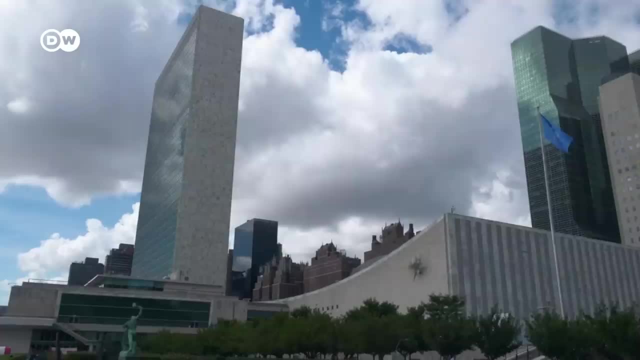 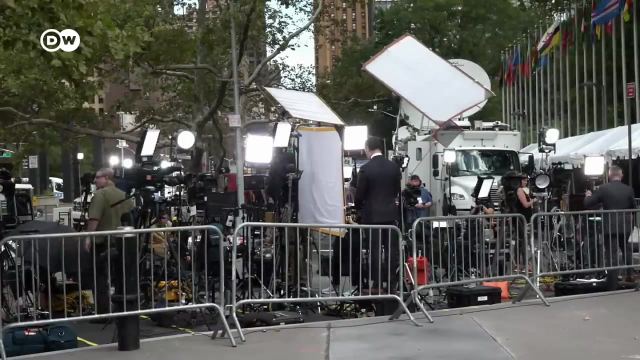 to the planet that we're trying to protect. In June 2021, the United Nations in New York was focusing attention on the highly threatened marine habitat. The UN proclaimed an Ocean Decade to advance the protection and security of marine life in the United States. 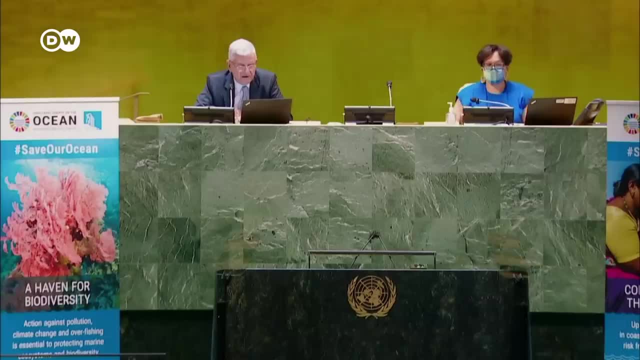 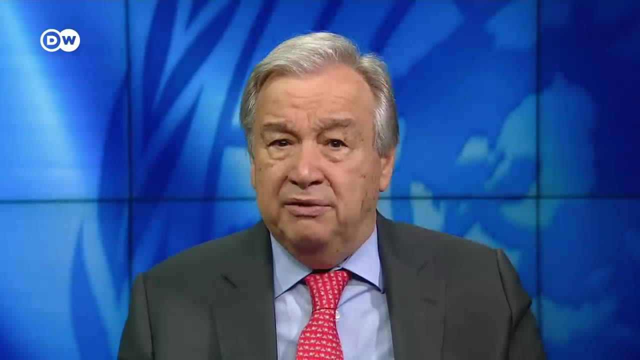 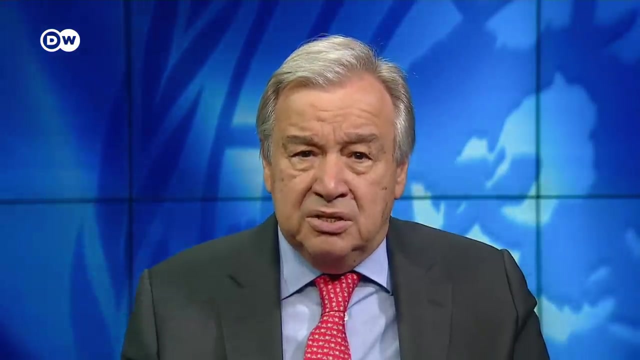 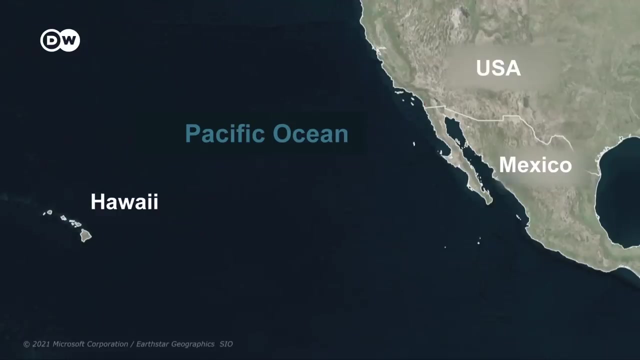 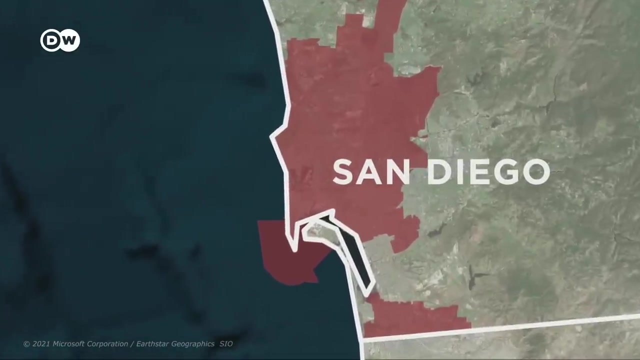 This challenge should be top priority for everyone, everywhere. Welcome to the United Decade of Ocean Science. Together, let us discover the science we need for the ocean we want. Thank you, In March 2021, in the midst of the global coronavirus pandemic. 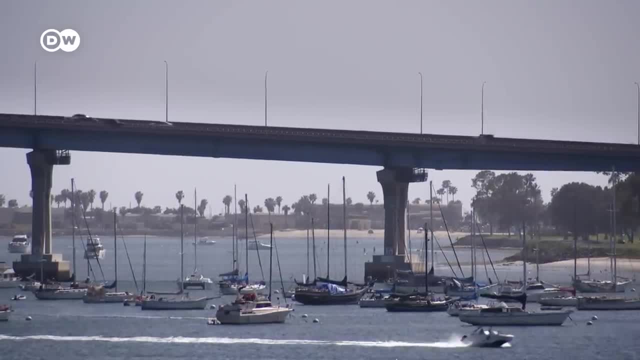 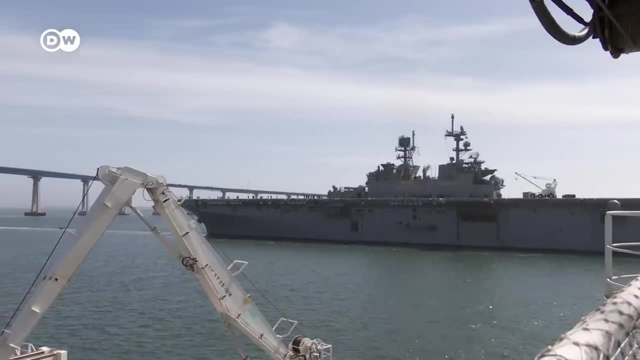 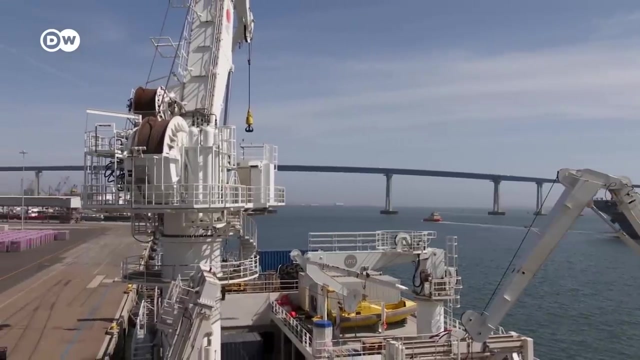 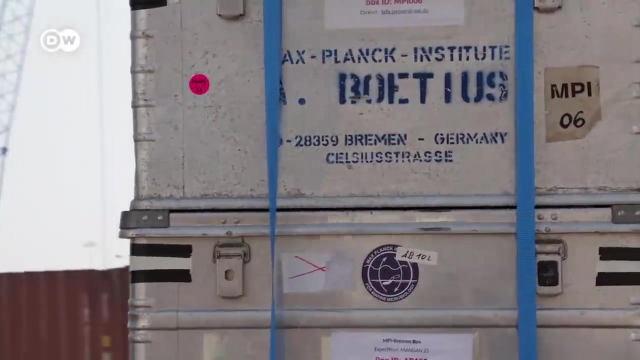 a special ship was docked at the US Pacific Fleet's naval base in San Diego. The vessel, the island Pride, was preparing to go to sea. Its crew and accompanying European scientists were going on a special mission As part of the Mining Impact Program. 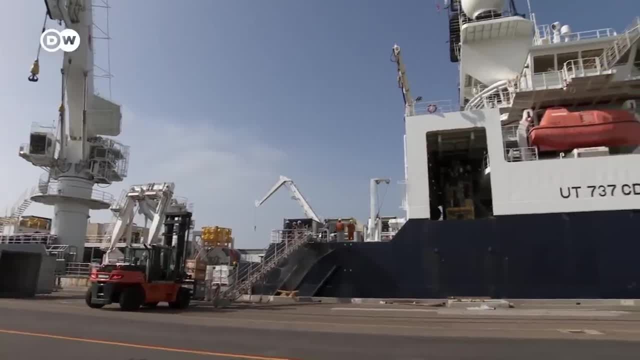 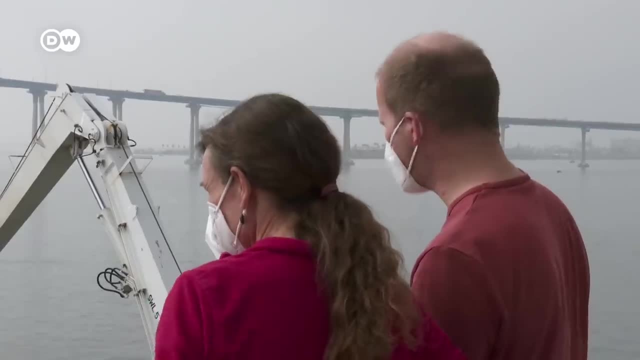 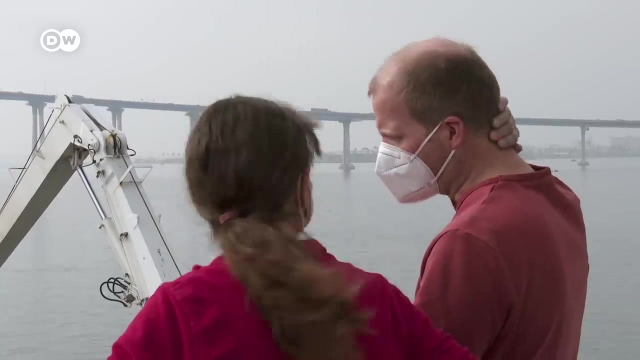 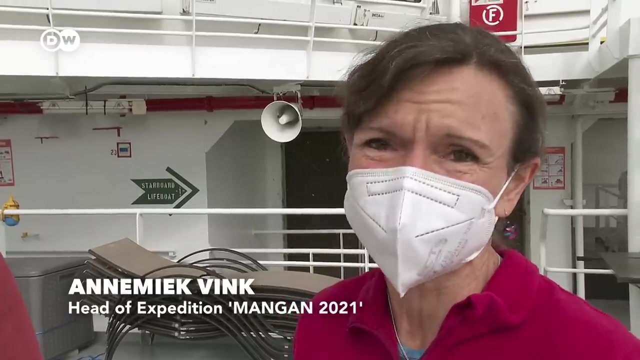 the researchers were heading out to examine what happens on the seabed during the world's first tests of a 35-ton underwater harvesting machine called a Polymetallic or Manganese Nodule Collector. It's a big project. We want to analyze the environmental impact. 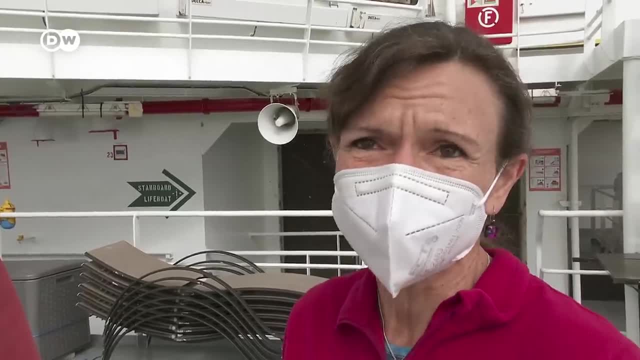 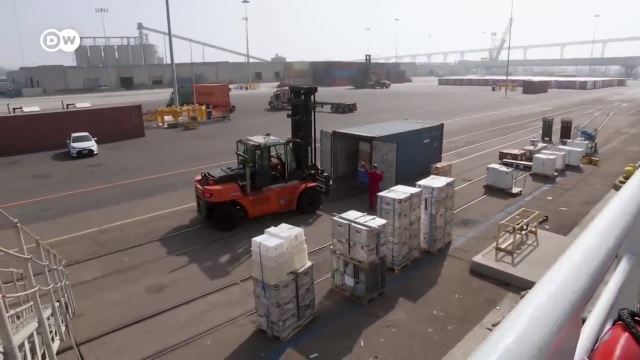 of a Manganese Nodule Collector working in the deep sea. We have quite a few scientific groups on board here. This is the first test of its kind and we're really close to the conditions you might expect from a deep-sea mining operation. 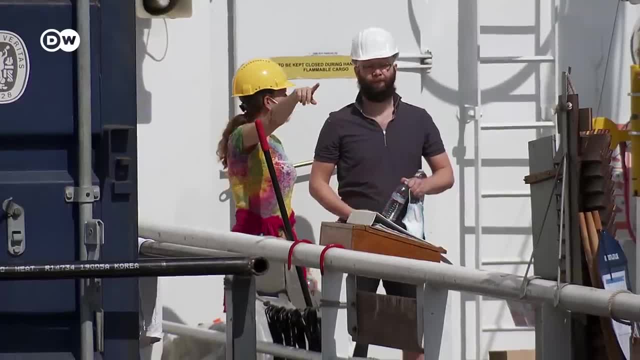 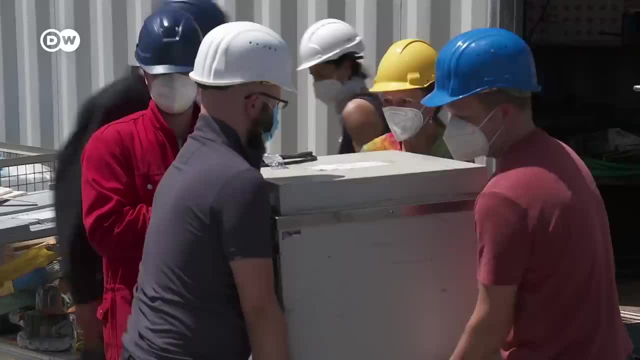 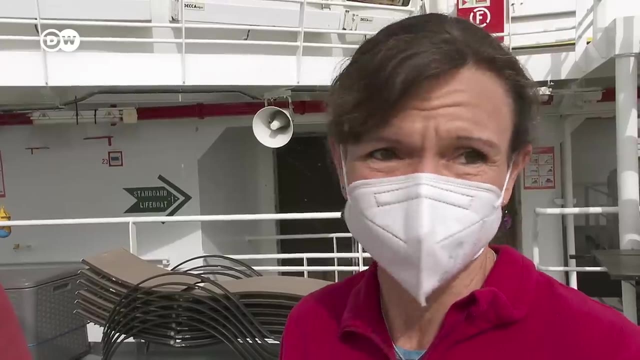 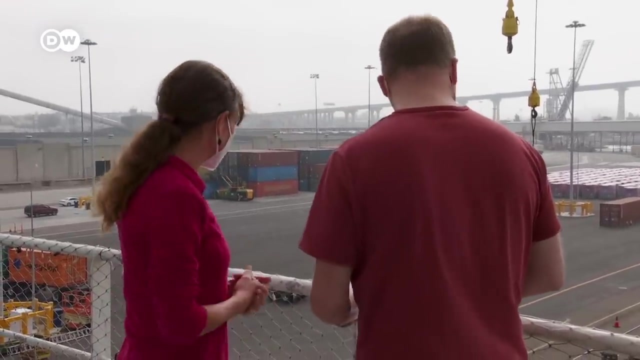 It's a big project. it's very important for the environmental analyses, parameters and standards that need to be developed. That's what we're doing, together with so many great scientific groups here: A concentration of Europe's scientific talent. actually, We have all the technologies. 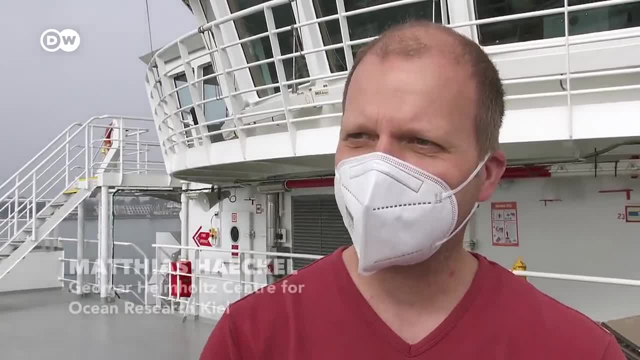 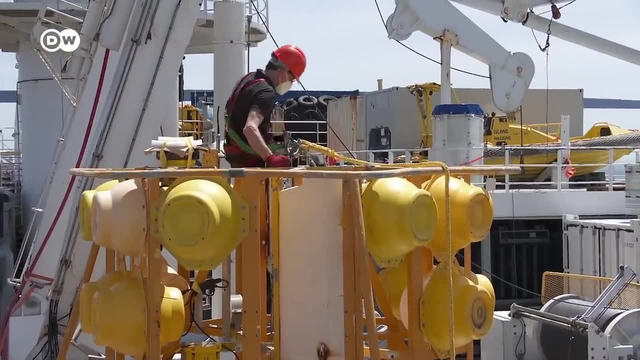 that marine research institutes offer. We've got all sorts of technologies and all sorts of equipment here, all very high-tech. Yes, I'm really looking forward to it now that it's finally getting underway. All kinds of measuring and testing equipment were used during this expedition. 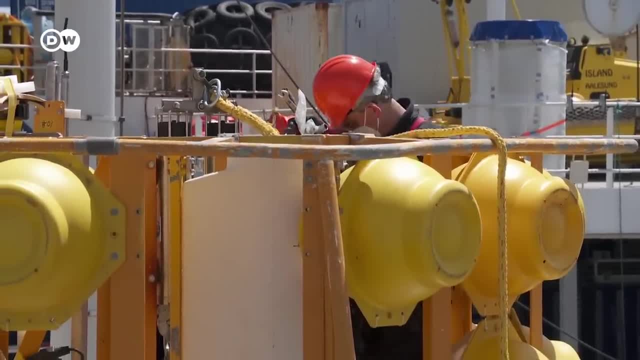 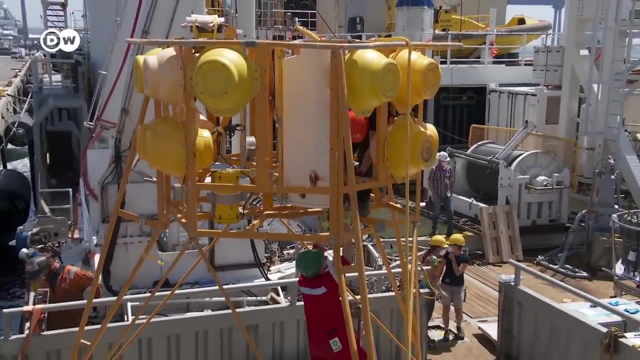 including this giant Bobo lander, which has already been in service for 25 years. The landing gear, that's right, but then not for the moon, but for landing on the seabed. So very much like that. we will drop it from the ship. 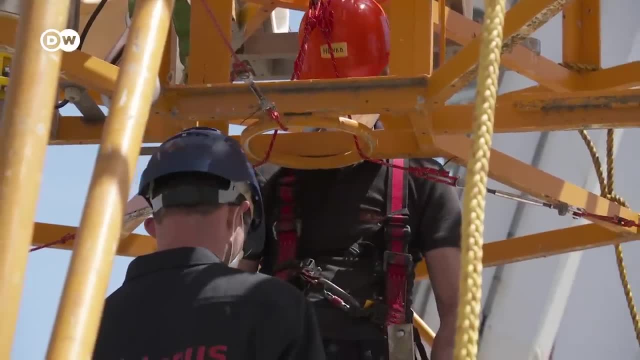 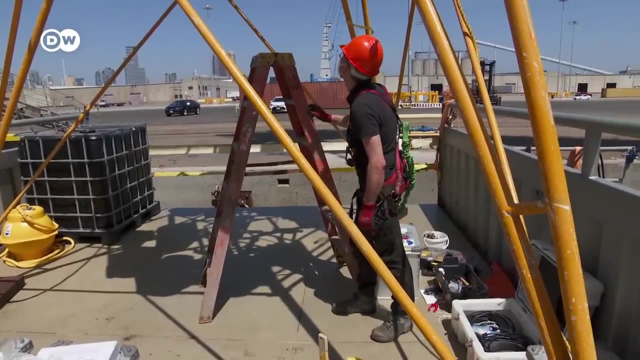 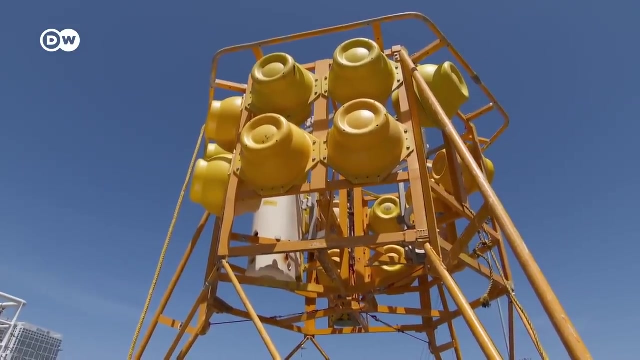 and mount it with some different kind of sensors and then it goes in free, fall to four kilometres depth and then make a quiet landing on the seabed If we want to know what the impact is of deep-sea mining, which is a concern to many people. 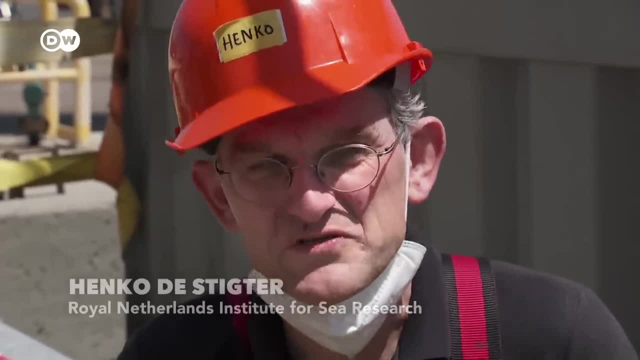 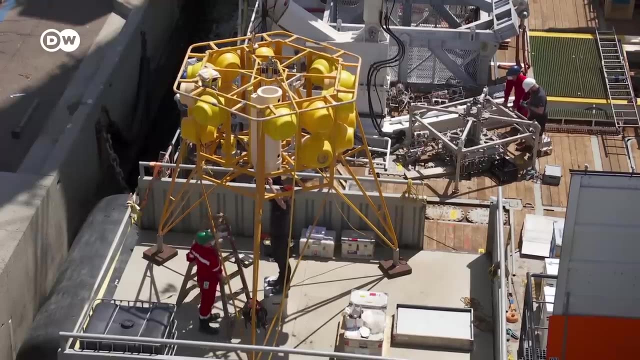 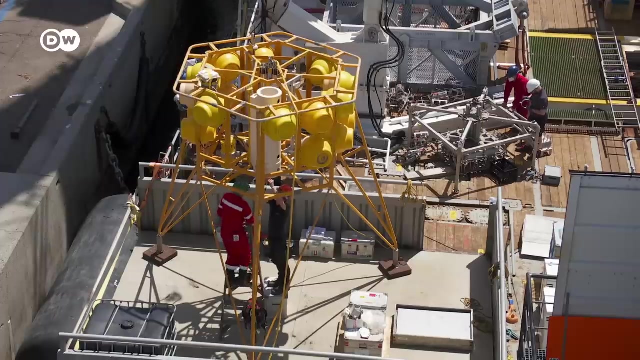 also to myself. I think we need good observations, Observations down there, close to where this mining is going to happen, so that we know better, that we can better predict what the impact will be. Researchers want to investigate first, while industry is ready to dig. 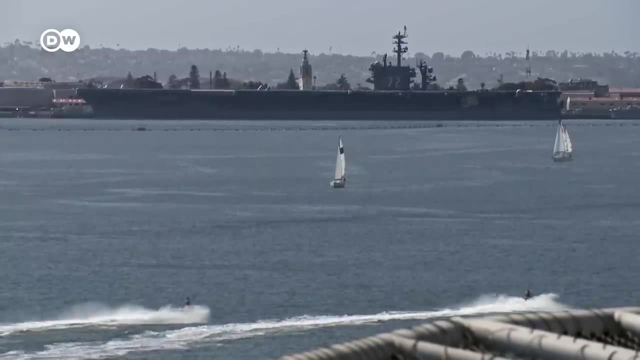 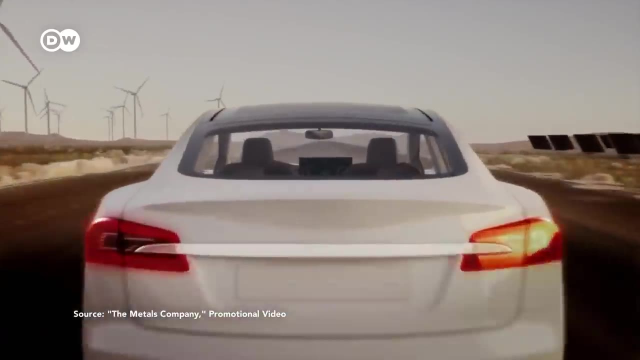 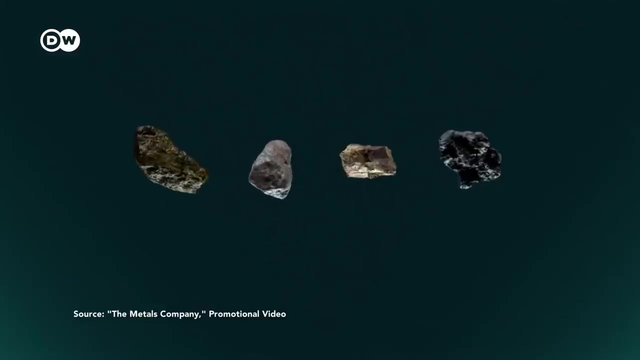 This advertisement for the Canadian mining enterprise, The Metals Company, promises a simple solution: Energy from the sun and wind is replacing fossil fuels. to power the transition to a sustainable future, We need batteries to store this energy. Batteries are made from metals such as cobalt, nickel, copper and manganese. 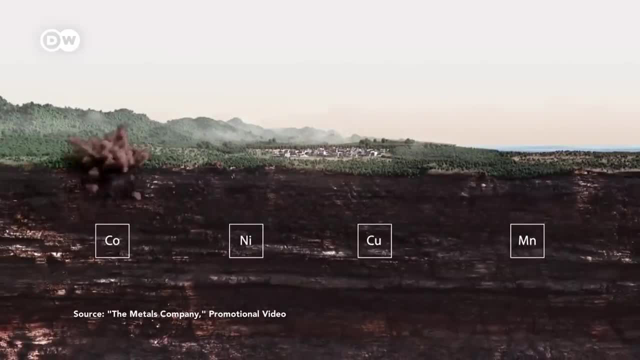 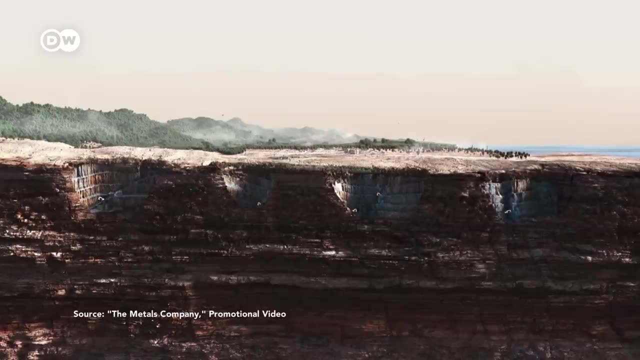 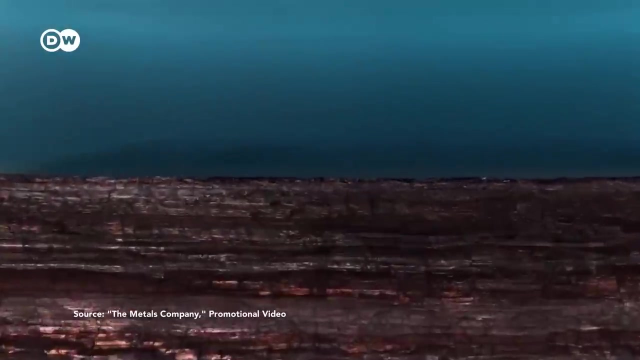 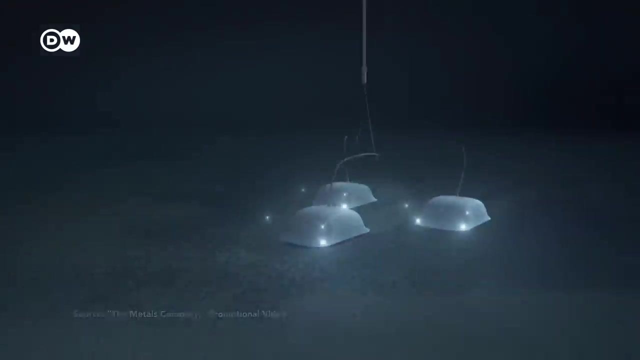 Until now, we've been mining the earth for them, digging deeper and wider for lower quality ores. Nature disappears, Humans suffer, Earth suffers. But there's another way. All that's needed are modern robots. But is it that simple? The Canadian city of Toronto. 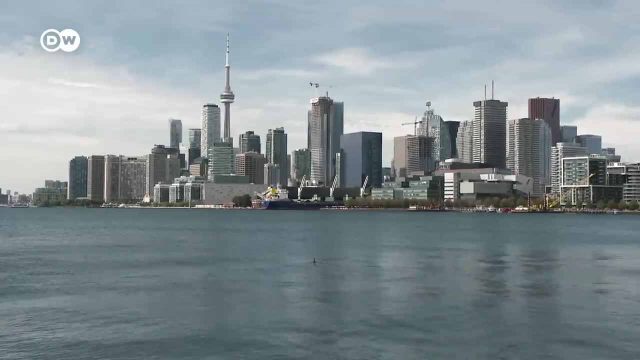 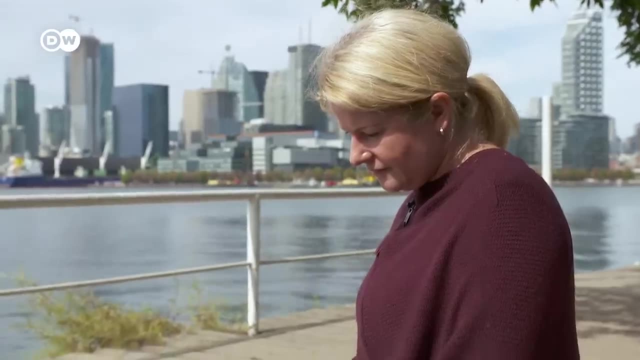 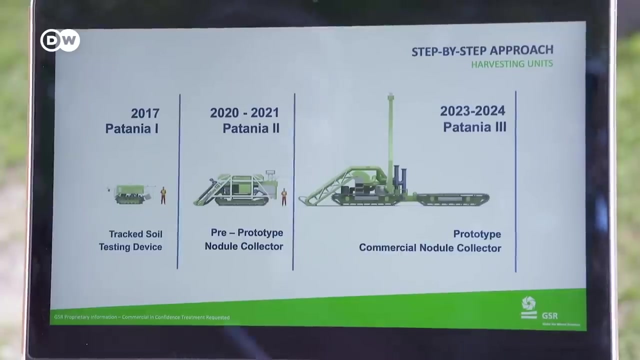 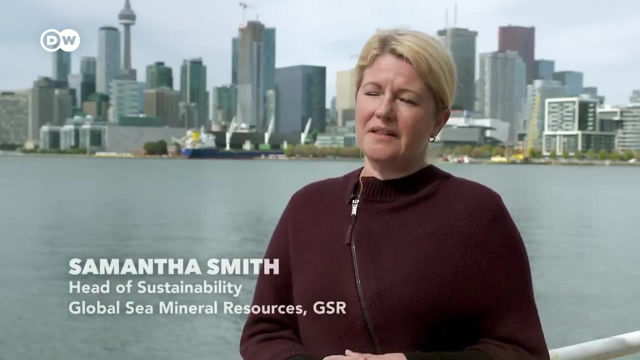 is where Samantha Smith lives. She's the head of sustainability for the Belgian mining company GSR. Their manganese nodule collector is undergoing a series of tests in the Pacific. We are together globally, we are facing a climate crisis And I think 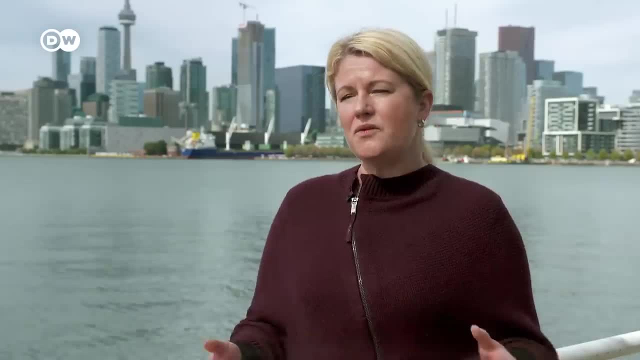 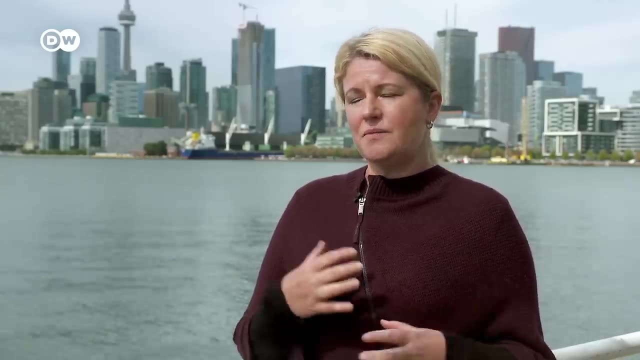 you know, there is this increasing recognition around the world that we need to do something, and we need to do something now That a big part of that is moving towards clean energy, so moving away from fossil fuels, And what that means is that we're moving away. 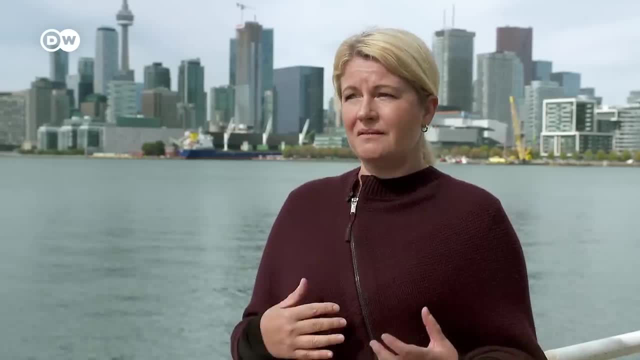 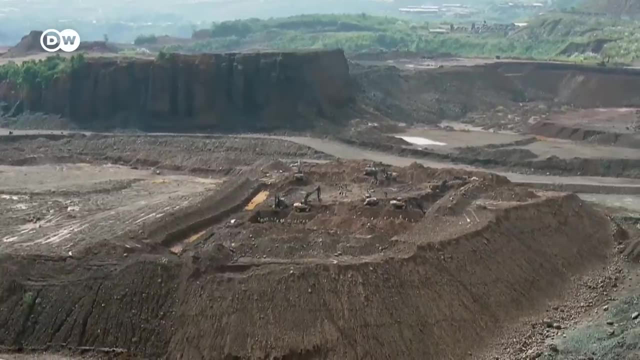 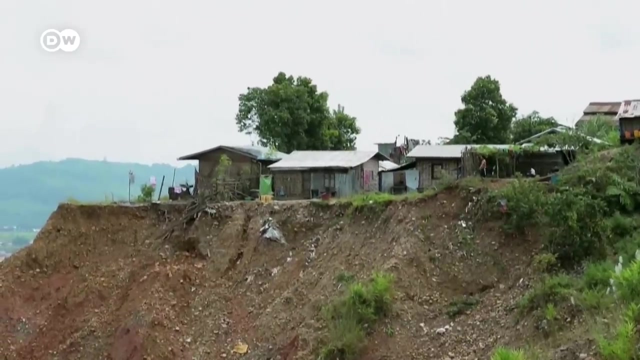 from a planet fueled on fossil fuels to one that is built on metals and minerals, because clean metal technology is so metal intensive. So far, these raw materials have come from mines on land Located primarily in Asia and Africa. the work is often destructive. 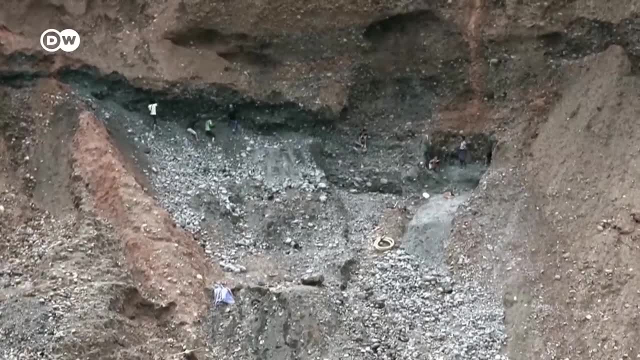 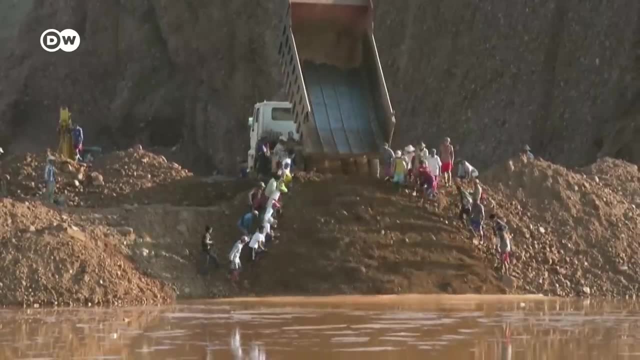 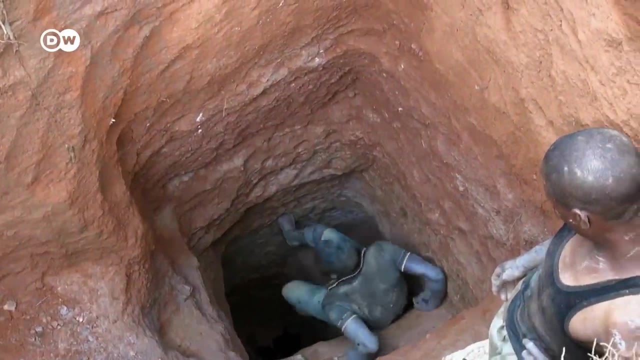 and harmful to nature. The mines are often located in politically unstable countries like the Democratic Republic of Congo, where there's not much respect for human rights. The workers often suffer horrendous working conditions, risking their lives, digging metals that fetch prices far greater. 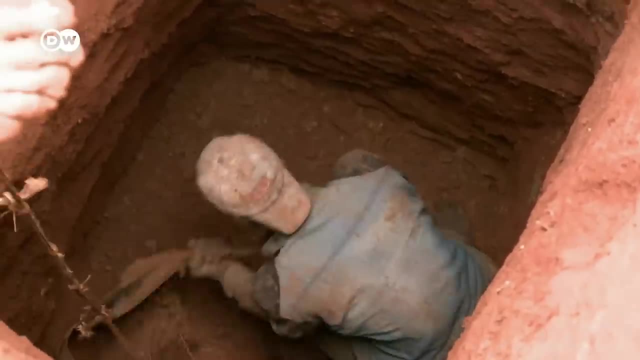 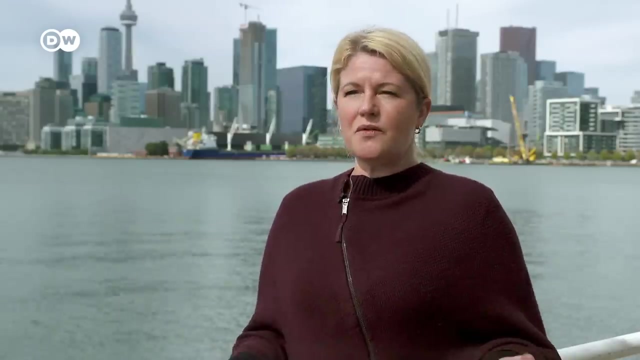 than the wages they earn. Industry says getting resources from the seabed will be far easier. We have options about where those metals can come from and we're exploring one which is going to the seafloor for them, And there's a lot of reasons. 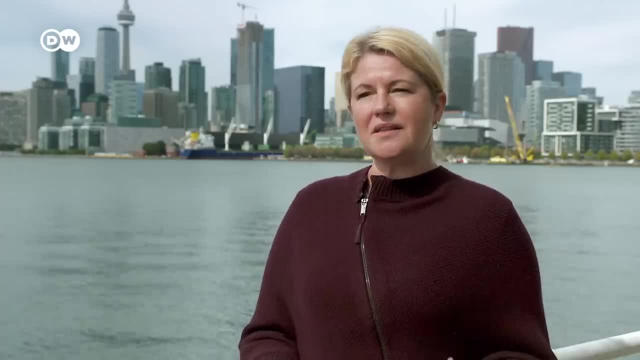 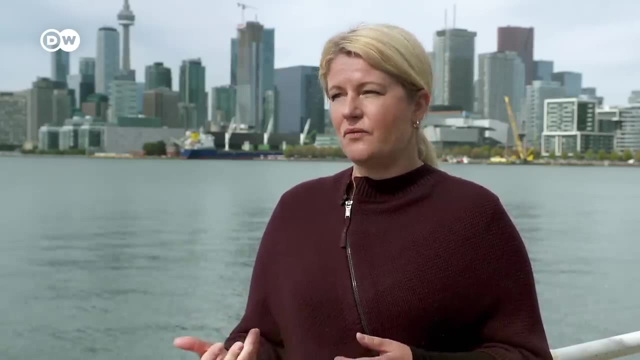 why going to the seafloor intuitively seems to make some sense, And one is we don't need to remove forests, and in some cases tropical rainforests are being removed to get to nickel. We don't need to remove forests. 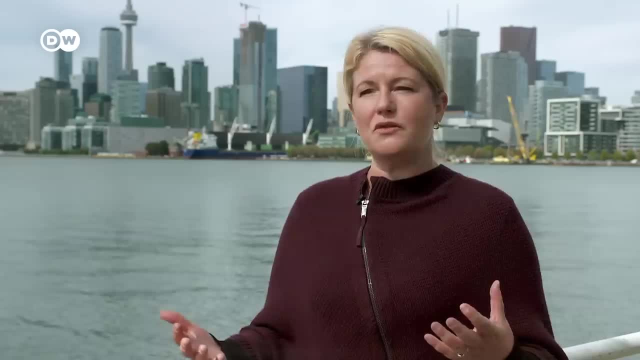 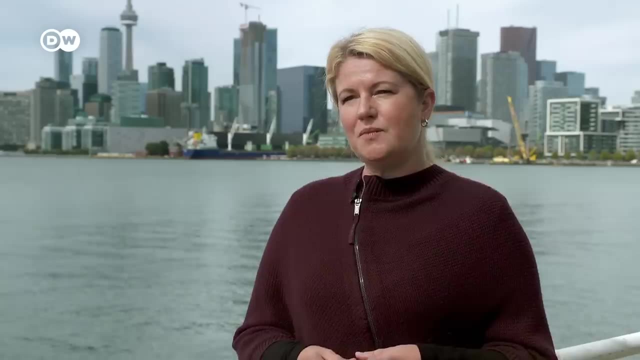 that are being removed to get to nickel. We don't need to remove forests or a single tree to get to the metal that's on the seafloor. Nor do we need to move mountains to get to the ore body, and people don't need to be relocated. 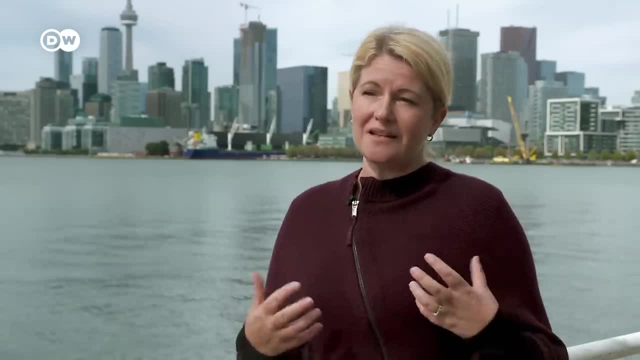 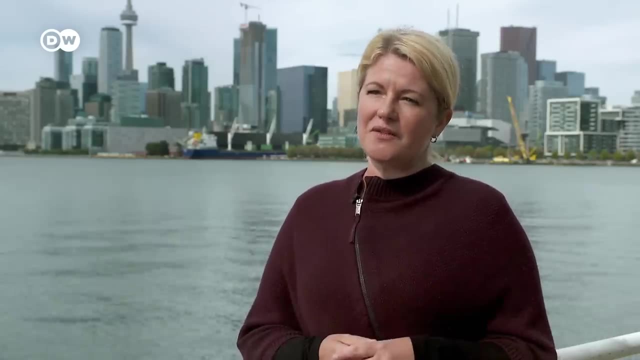 So, right away, those reasons make a lot of sense. Of course, that doesn't mean that we can just dive to the deep sea and not do it thoughtfully. We also have to get the research done so that we understand how to proceed while minimizing our environmental footprint. 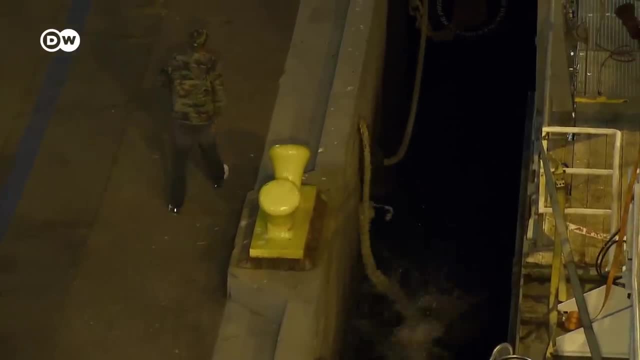 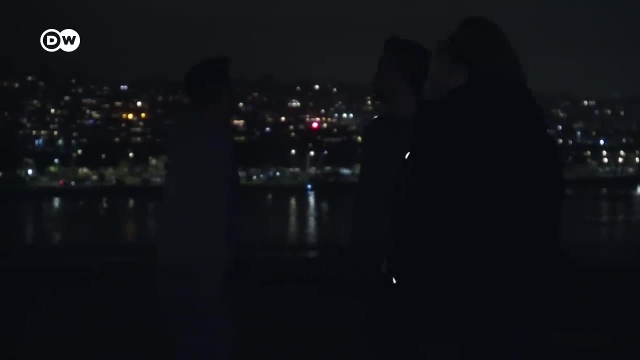 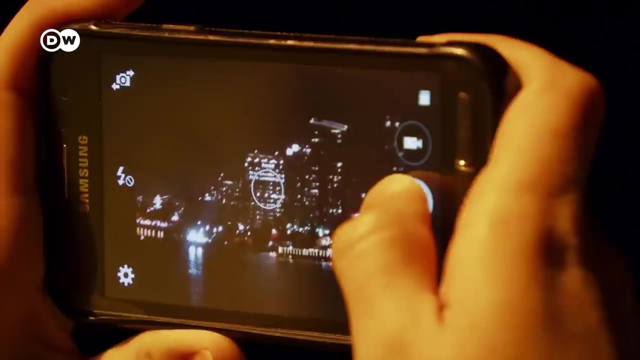 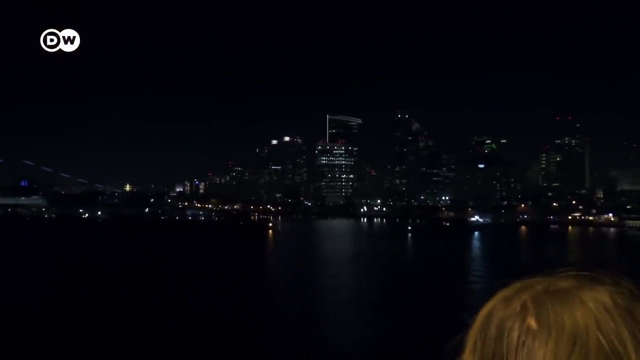 Can there be deep-sea resource collection without causing new environmental problems? The Island Pride departed from San Diego for a six-week expedition to find out. Expectations were high. Our mission is to investigate the environmental impact of all this. We know a lot about this marine habitat. 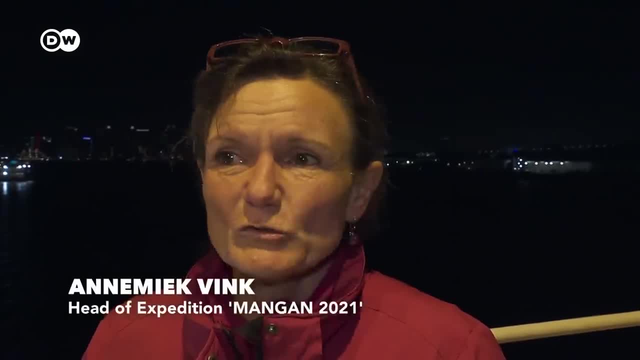 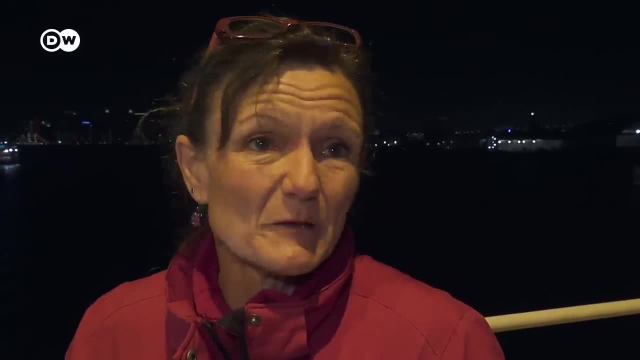 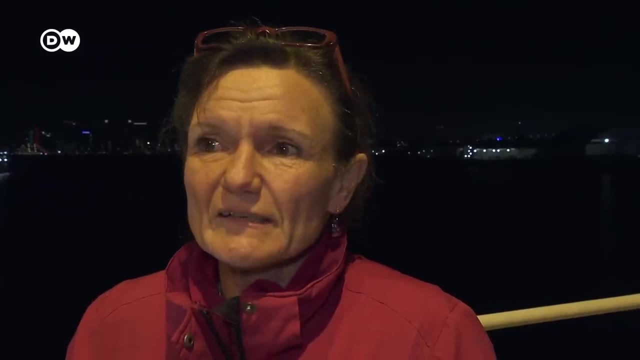 and we know a lot about the environment, its ecology, the animals that live there, but not necessarily what the impact will be when big equipment and machines are driving around on the seabed. Our objective is simply to observe, analyze and neutrally take measurements. 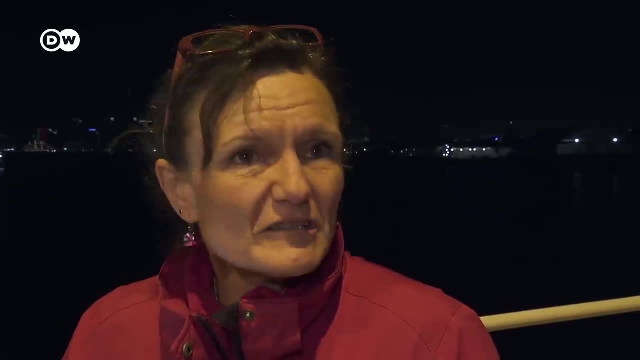 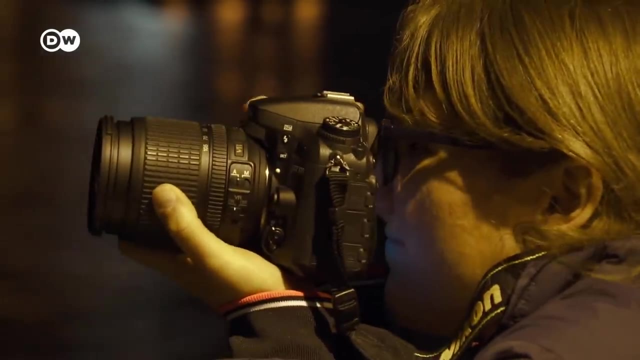 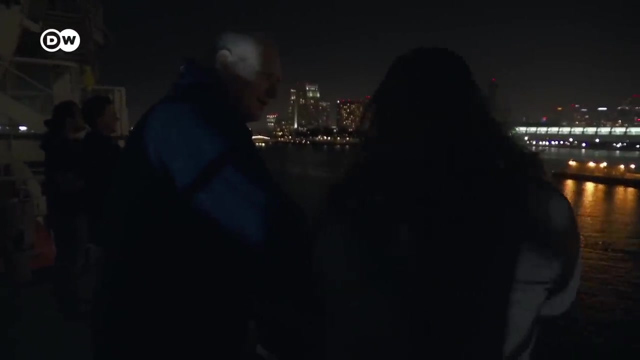 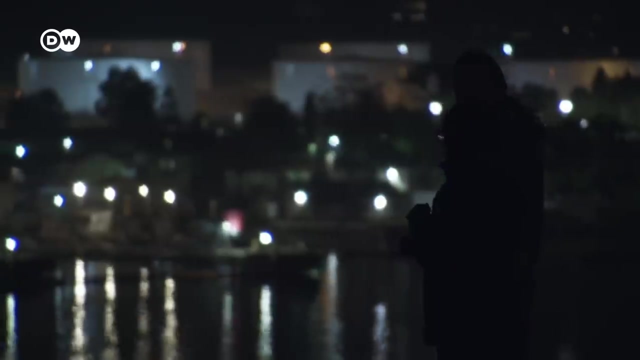 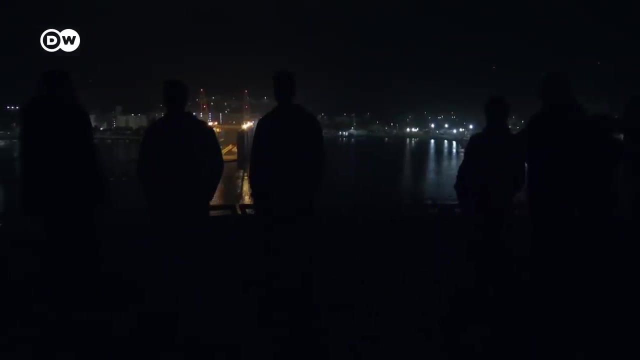 so we can present these findings to the public in a scientifically balanced way. Science, industry and policymakers all watched the expedition closely. The findings could have far-reaching consequences as humans move towards the age of green technology. The crew and researchers waved farewell as the San Diego skyline receded. 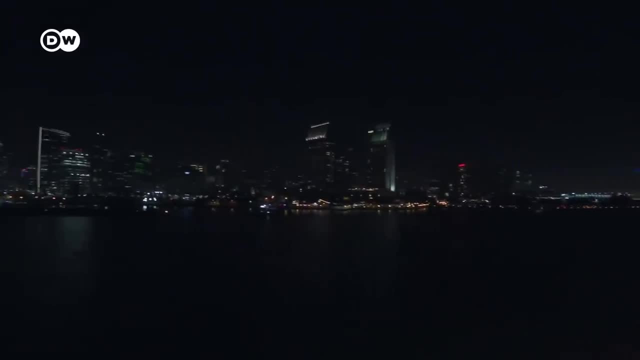 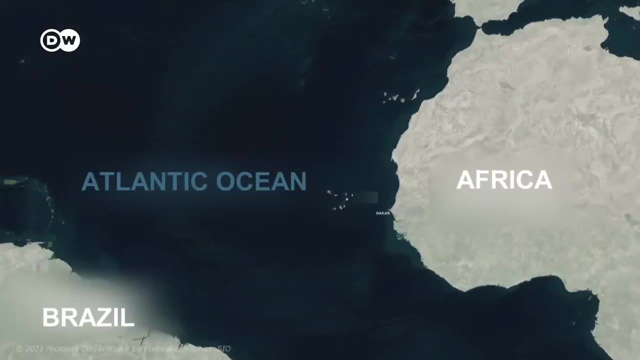 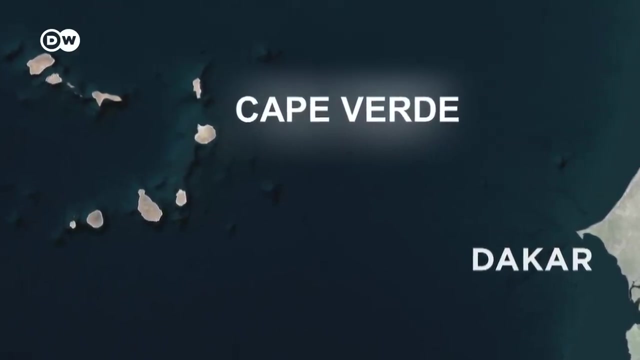 The boat went off into the night, off to where some countries and companies would like to develop new sources for raw materials as quickly as possible to make the ocean a source of mineral resources. Cape Verde's 10 islands are located around 600 kilometers off the West African coast. The country has half a million inhabitants, most of them descended from former African slaves. Once a colony of poor, it gained independence in 1975.. Even though Cape Verde is considered one of the most prosperous countries in Africa, there's still a lot of poverty. 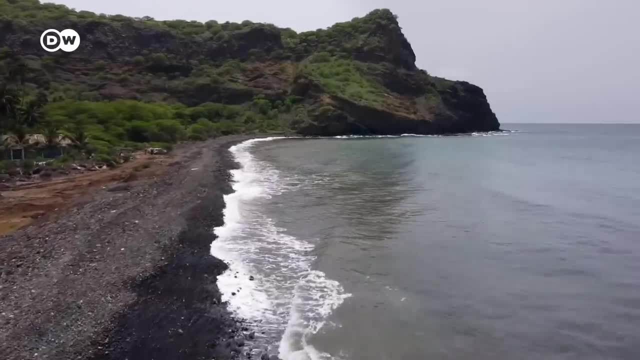 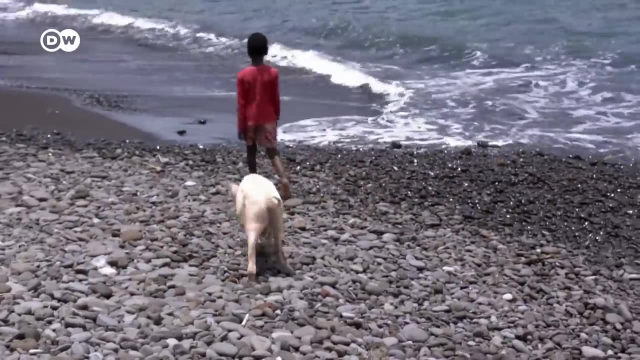 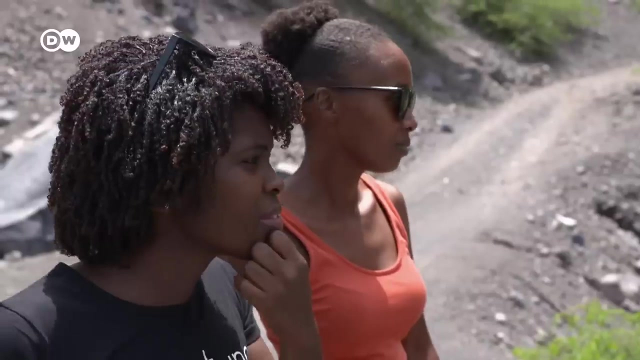 For many, the sea is the source of life, But a look at the coastline in some places indicates something is wrong here. Where there were once sandy beaches are now only sand And now only stones. Ana Vega works for the conservation organization Lantuna. 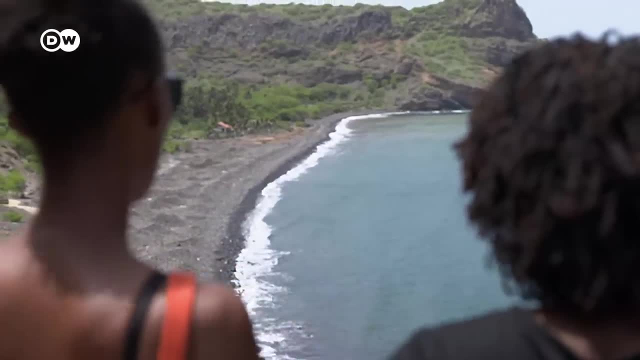 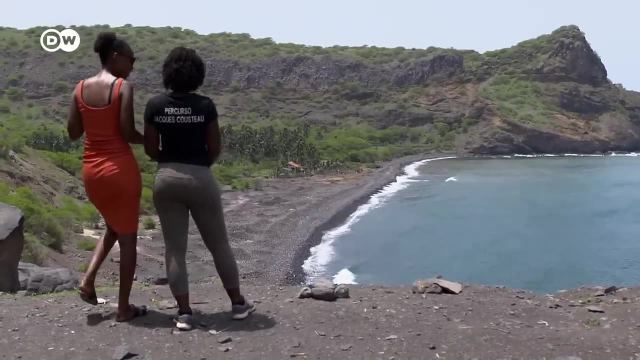 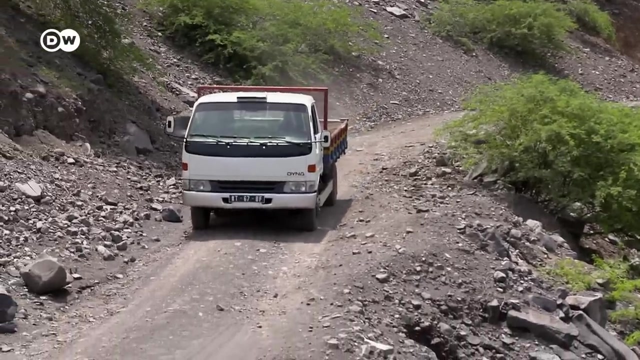 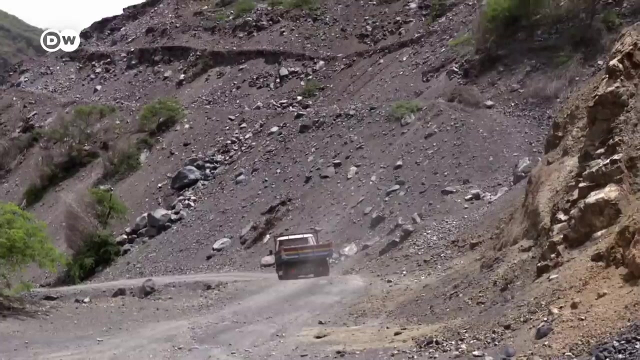 She also takes people on tours. Nature has been mercilessly exploited. here. The women watch a truck go by loaded with sand from the shore. Well, this truck just bought sand and it will resell to someone else. So they come here, take the sand. 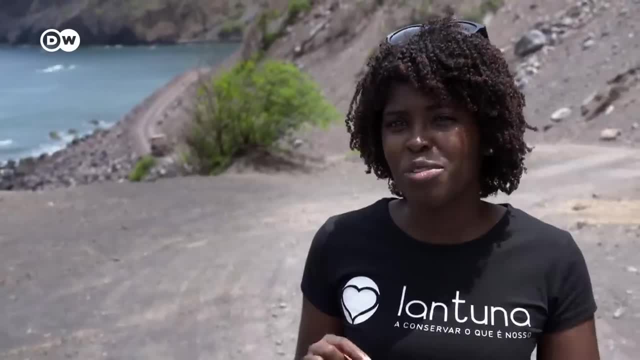 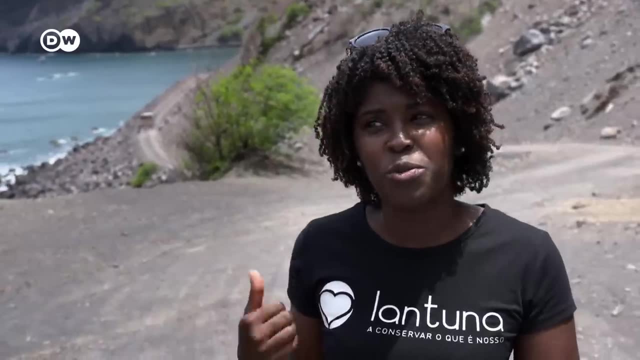 and then sell it to the market. It's like a small business, It's not a really big company. So there are several trucks, It's not just only one truck And, as you see, the beach doesn't have too much sand anymore. 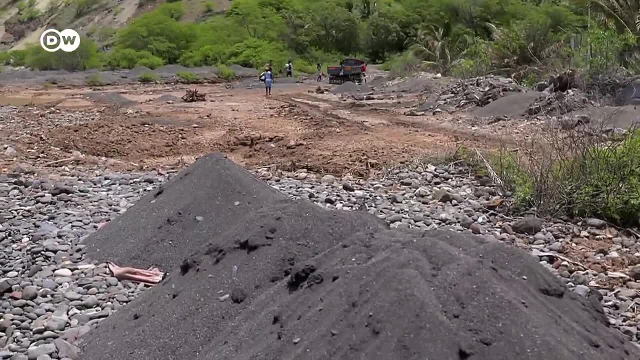 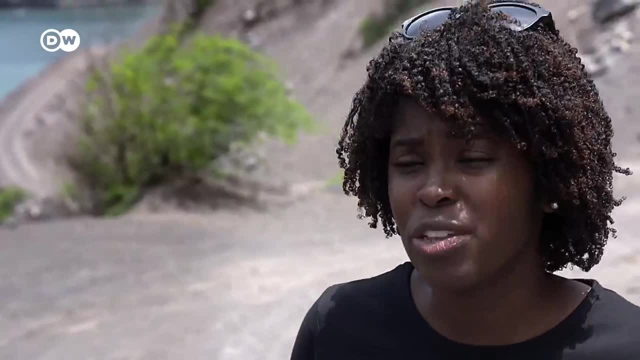 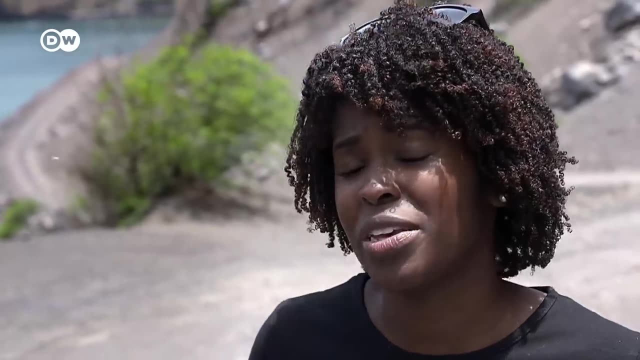 So the little that still exists, it will be sold. It is against the law, It's forbidden to take the sand, But the surveillance is very weak. That's the big problem. It's not allowed to take the sand, Although there is not surveillance here. 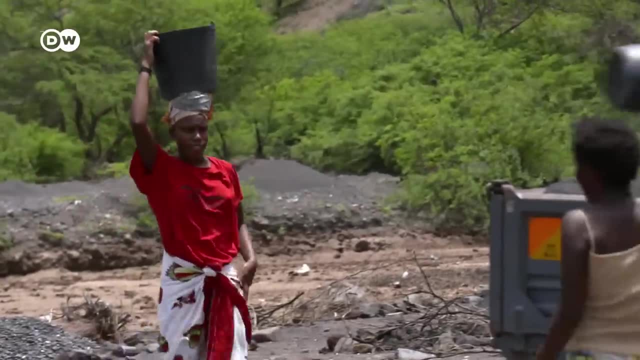 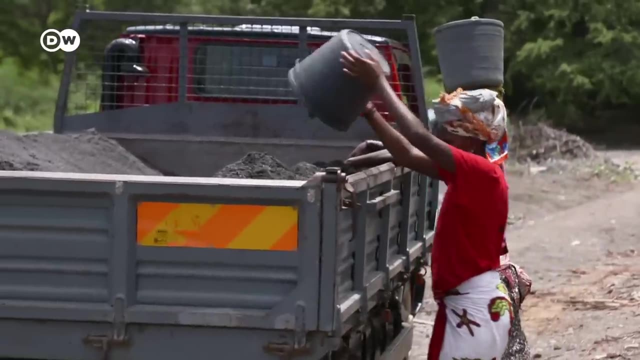 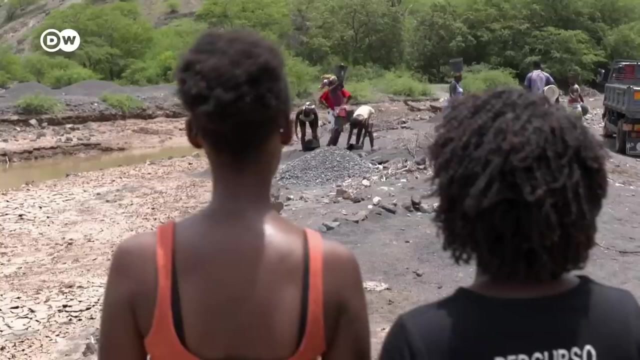 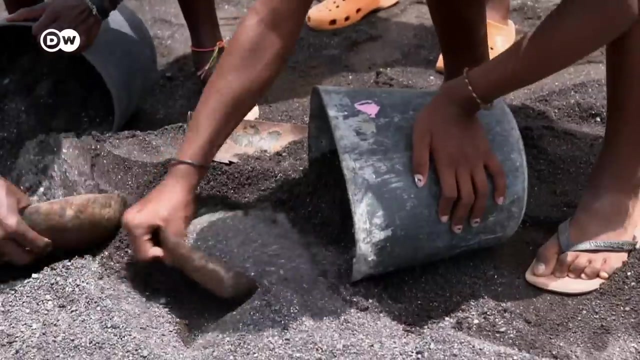 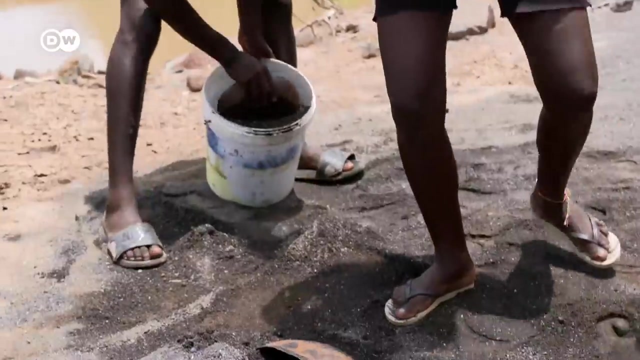 but it could be controlled on the road, But no one does it. So how are we doing here? The two conservationists look on stunned to see how these people are illegally stripping sand from beneath their feet. Another truck is loaded, this time with sand taken from the seabed days ago. 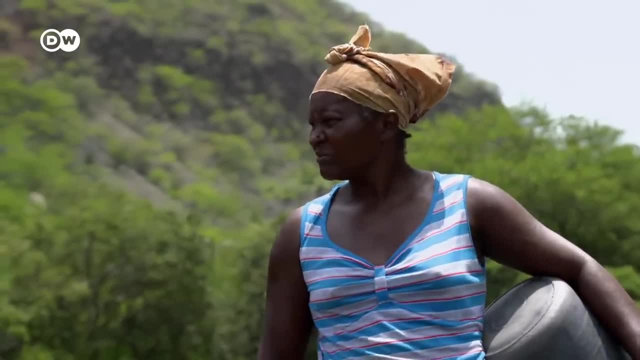 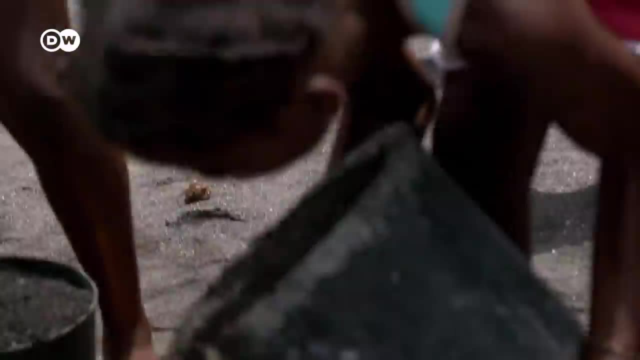 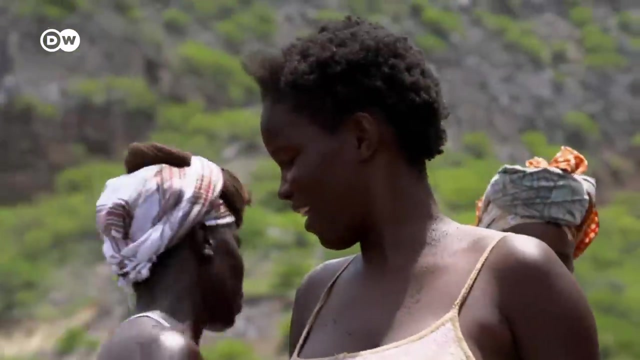 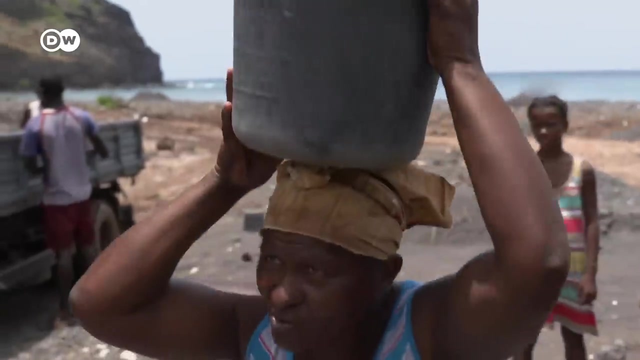 The sand is sold as raw material for the construction industry. For years, this back-breaking job has been the only way for people like Maria to earn a little money. It's very exhausting and tiring. Sometimes there's even a danger of drowning. 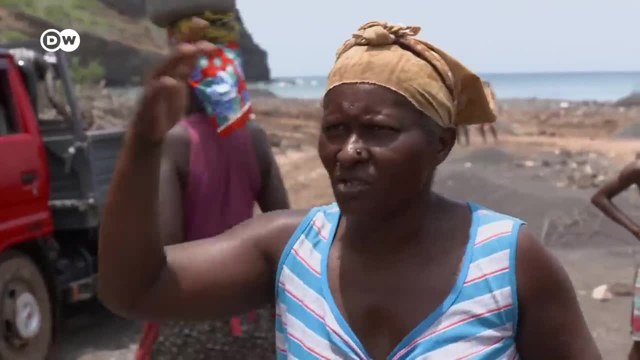 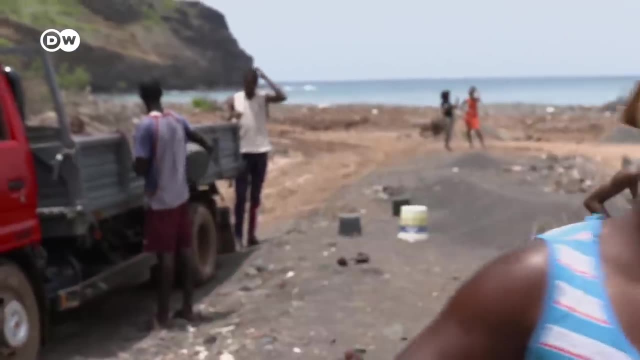 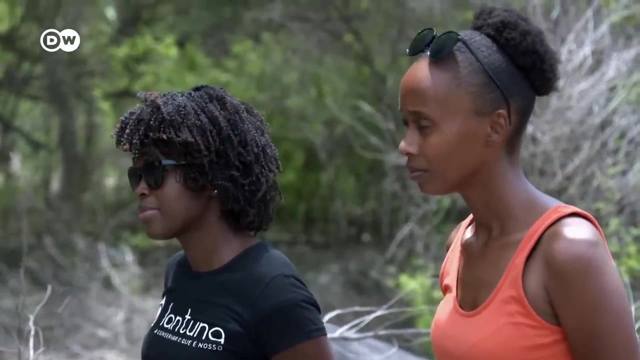 We stand in the water like this. It's dangerous, But if we don't do this, there is no other way for us to earn money. The conservationists seek dialogue. Ana learned that years ago the bay of Riba Radabaca was a sandy beach. 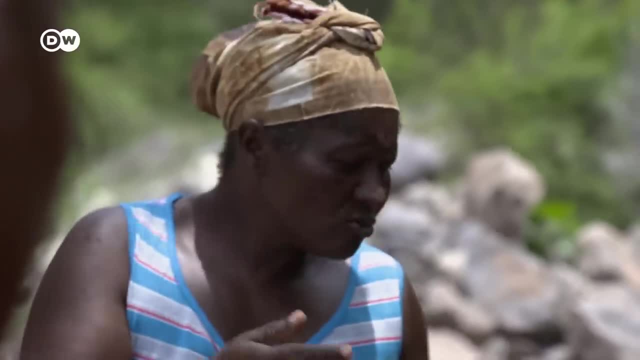 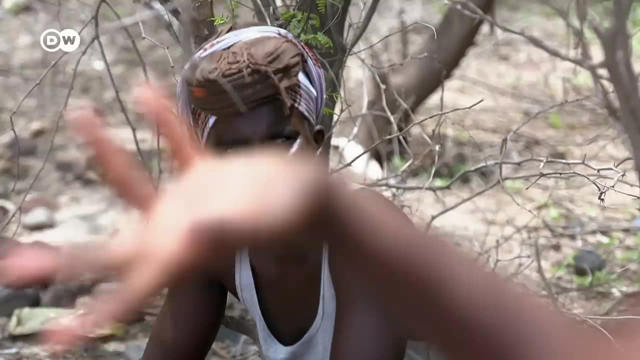 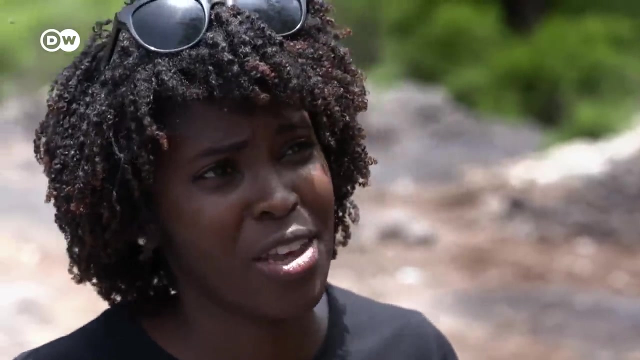 covered with dunes. Nothing of that remains today. Ana says the people digging up the sand know what they're doing here. isn't right. I've asked her how much they earn to do this kind of job and I was shocked because each truck it is around 30 to 40 euros, and if they are desperate to sell even 25 euros, they sell, And the driver will sell it around 120 euros. I even asked if they would like to change their job to do something else. 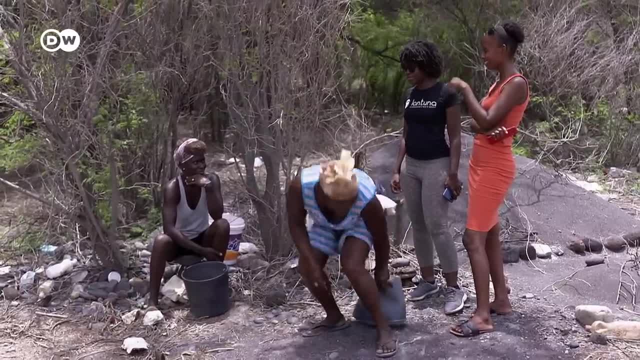 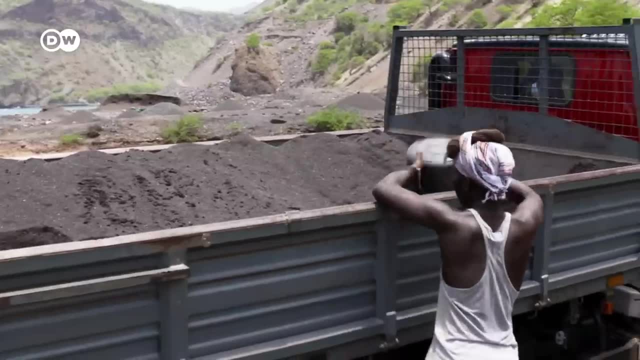 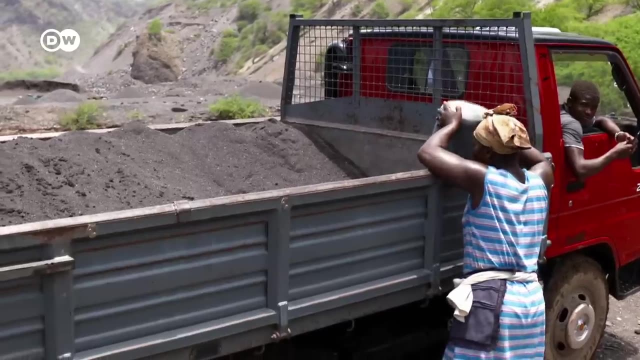 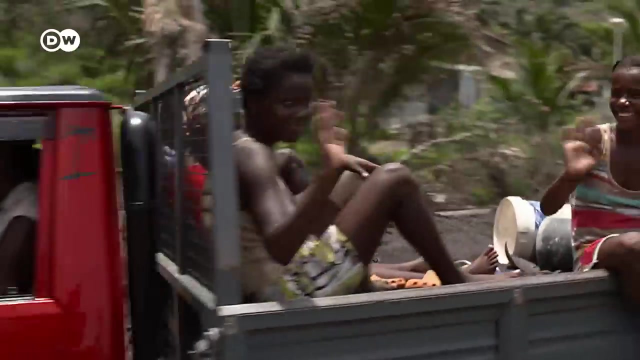 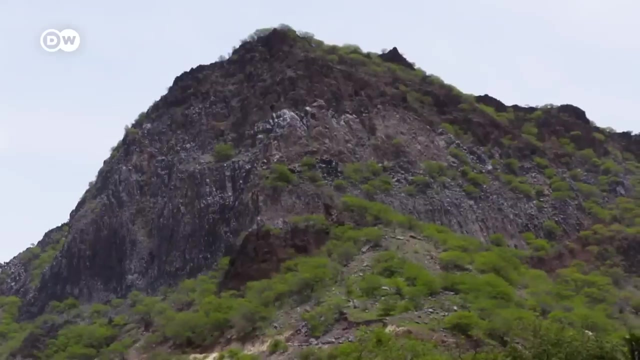 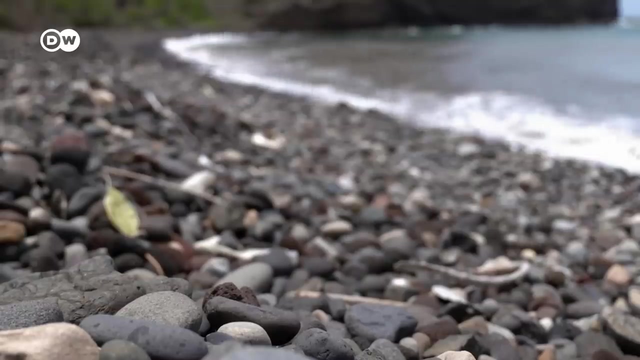 They said, yes, If there is opportunity, they would, But if they don't, they won't. Sand has been taken from the seas for years. Beaches are disappearing, and not just in Cape Verde. The sand is gathered in small bouts. 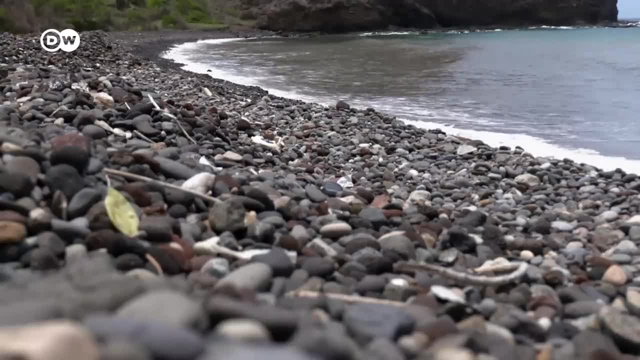 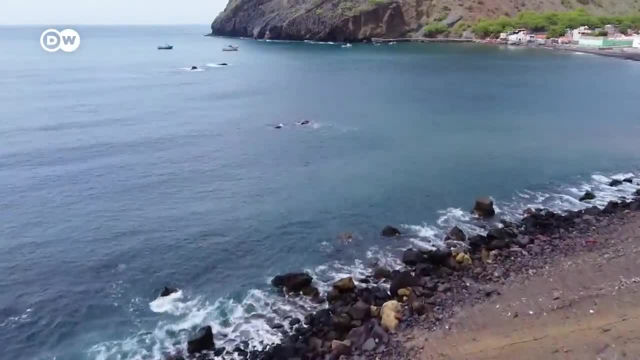 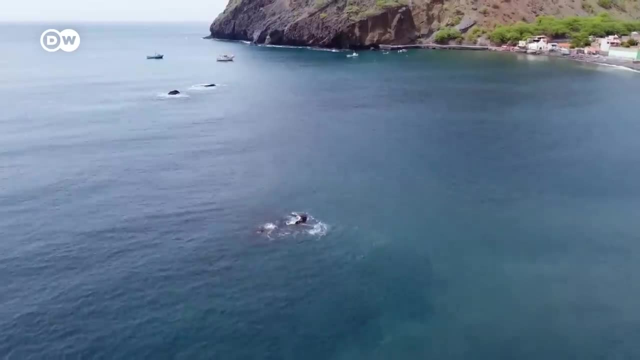 or with enormous industrial ships from many oceans. The impacts are devastating. Scientists and conservationists have long warned of degradation of habitats. We all consume, directly or indirectly, sand or gravel that comes from the oceans. This is also a very big problem in the construction industry worldwide. because so much sand and gravel are being taken from beaches, including right off the coasts, that entire ecosystems are now changing, biodiversity is suffering and entire structures are being eroded. And, last but not least, organized mafia-like groupings are at work behind the scenes. 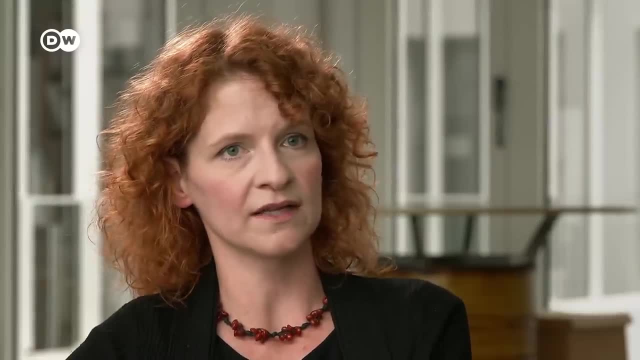 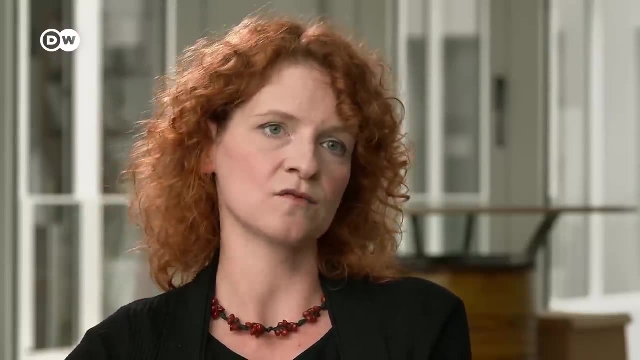 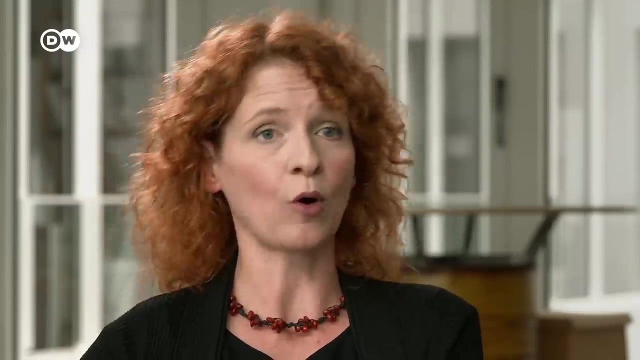 People are forced to transport sand illegally. Entire islands are now almost free of sand in order, it must be said, to enable a construction boom in the globalized affluent West, which should actually have no future at all in this day and age. So this is an issue that is causing major problems. 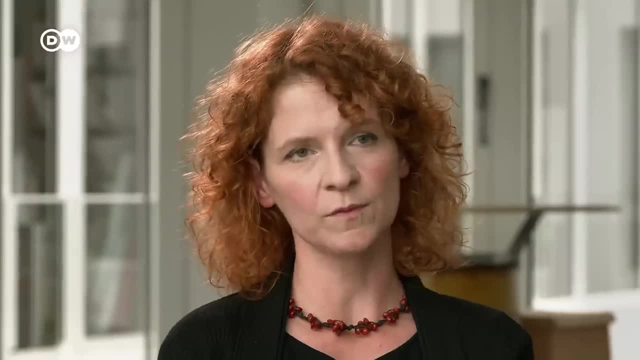 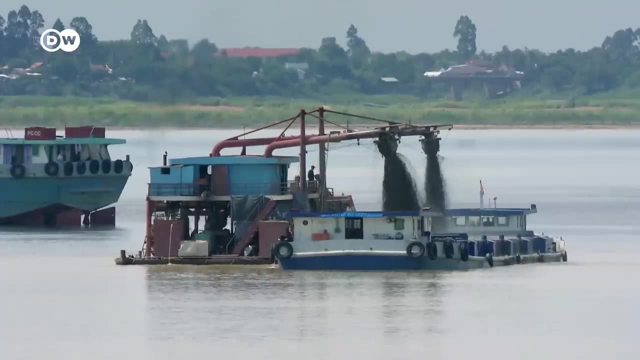 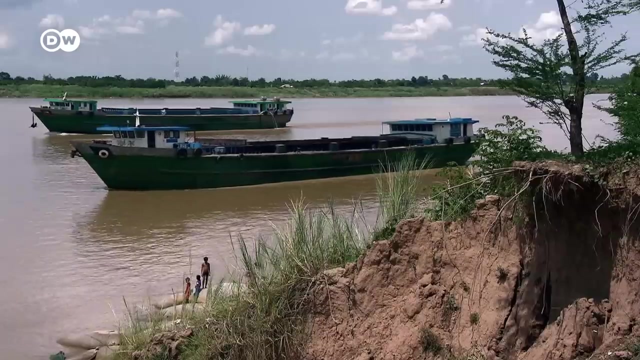 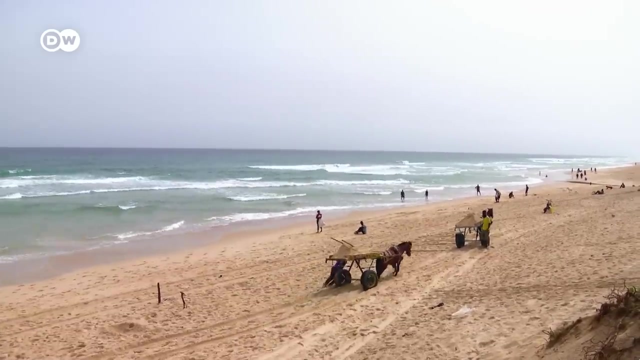 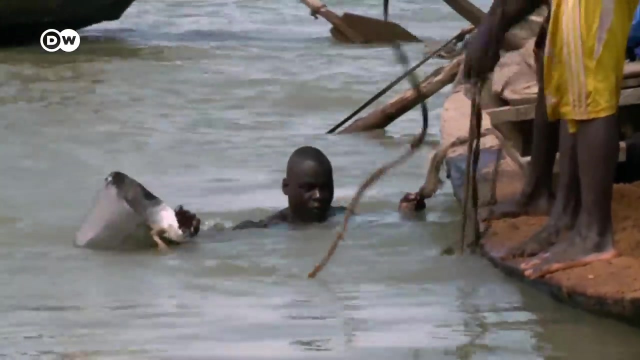 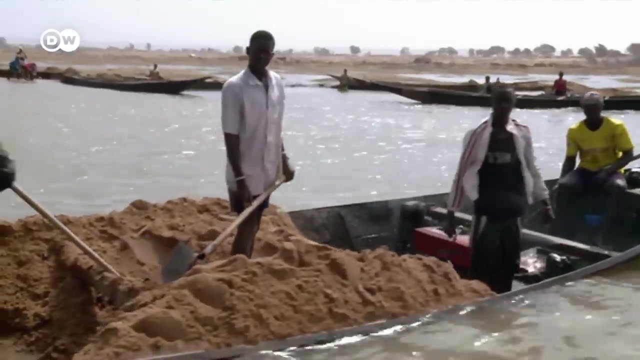 in our seas at the moment, but hardly anyone knows that In India, Africa and all over the world. even in the North Sea, sand is being dredged from seabeds. Descriptions of sandy seashores no longer ring true. Sand typically makes up around one-third of concrete. 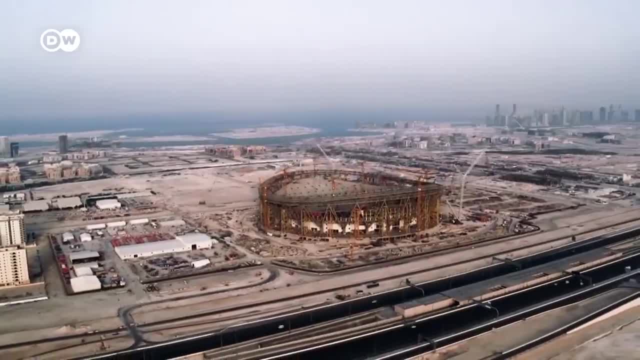 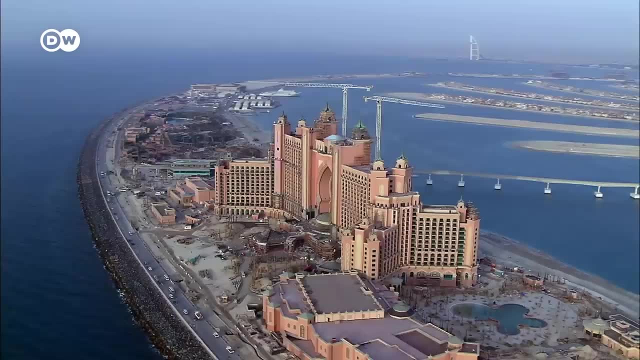 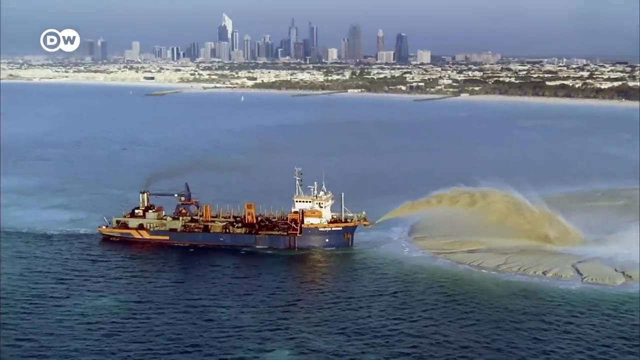 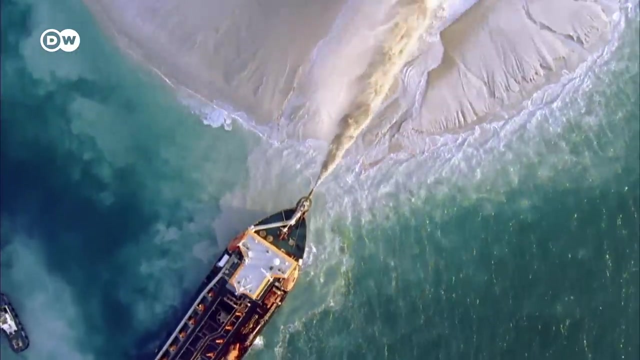 Gigantic buildings in desert countries are also being dredged. Desert countries are also made of sand from the sea, because desert sand is unsuitable for building. Even the sand for prestige projects, such as the artificial islands off Dubai, comes from the sea. Overexploitation has fatal consequences. 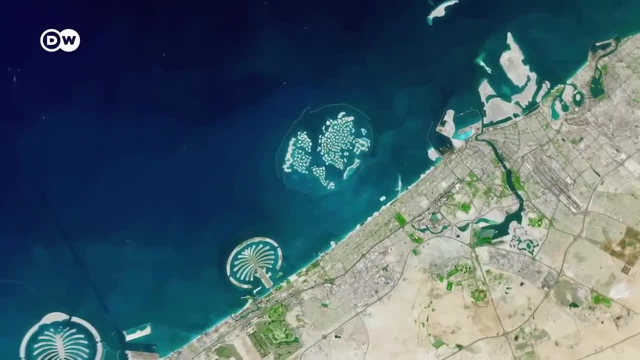 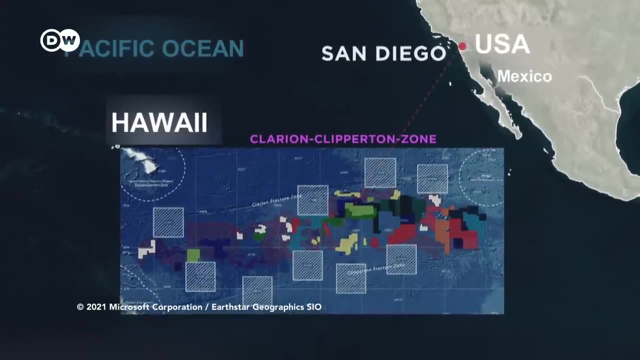 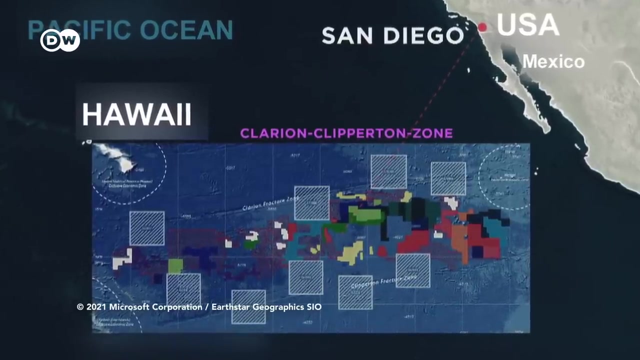 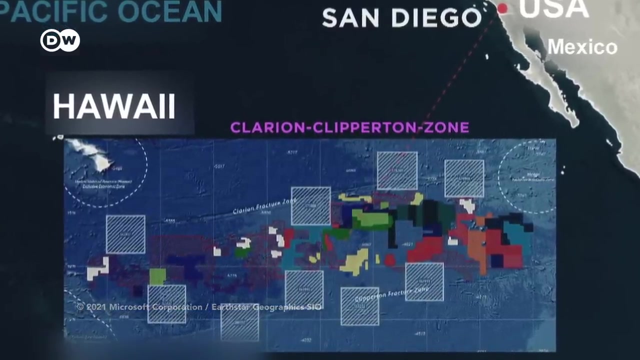 for coastal areas, microorganisms and habitats all over the world. Meanwhile, the island pride has headed for an area of ocean known as the Clarion-Clipperton Zone between Mexico and Hawaii. Here, enormous quantities of polymetallic nodules 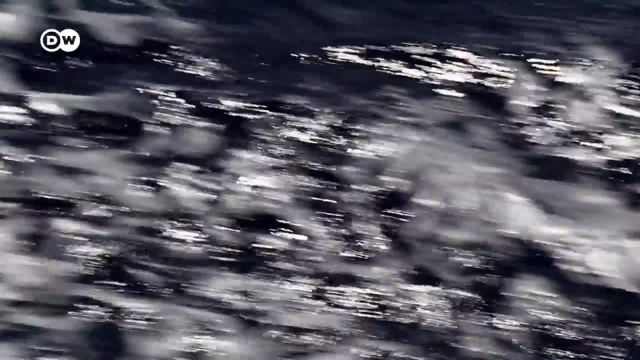 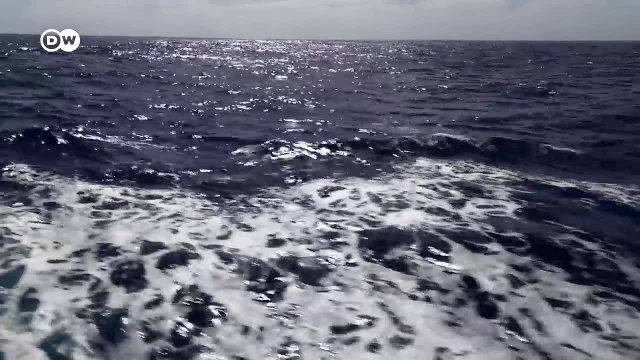 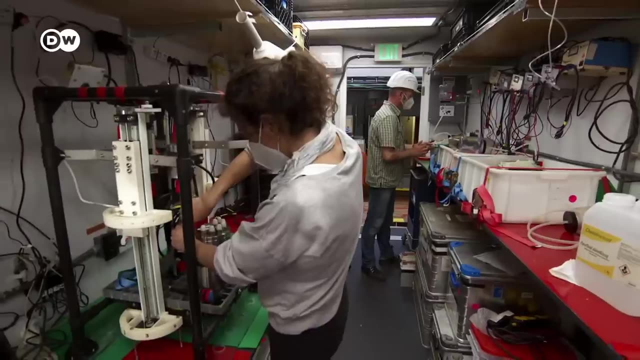 an estimated 30 billion tons lie on the sea floor. It takes almost six days for the island pride to reach its destination. These devices held the keys to the expedition's success. Everything had to work. The tension was palpable. The researchers played music. 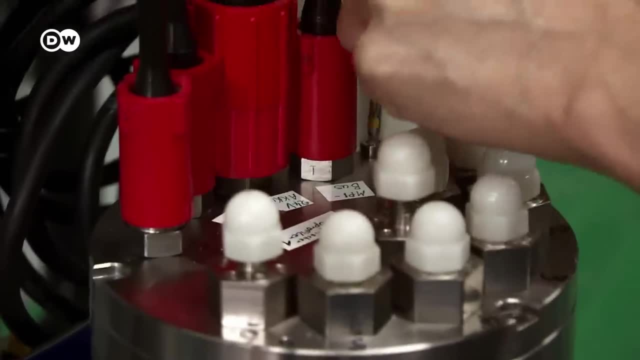 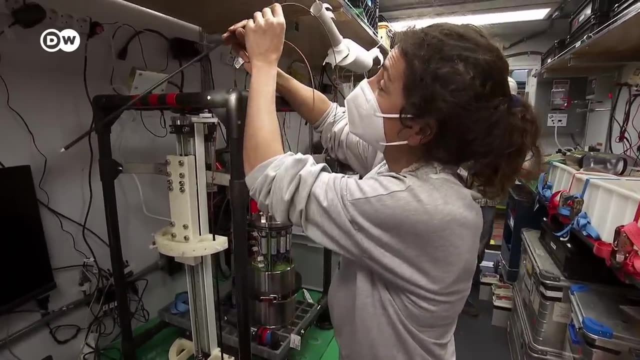 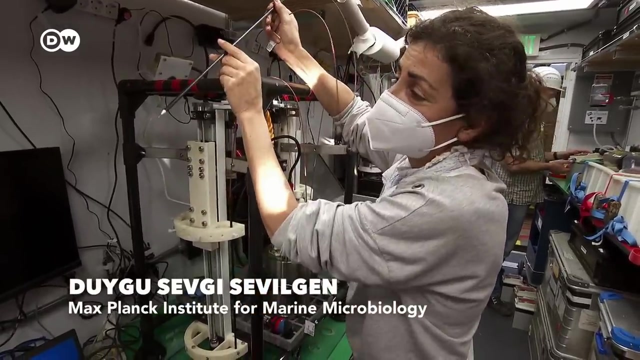 to help themselves relax. This is what's called a deep-sea lander, And inside is a module like this. Optical measuring devices or mini-electrodes are connected to it. They are these rods that we see here. There's a very small tip. 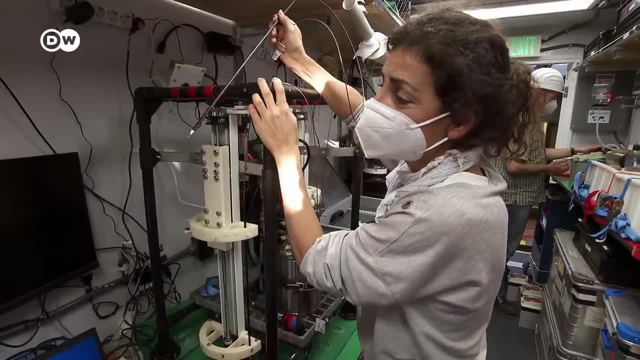 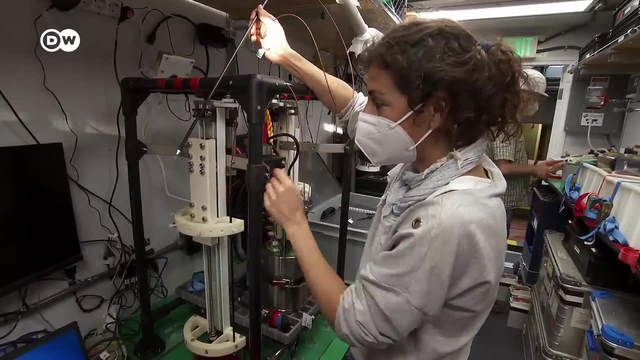 that optically measures the oxygen content in the sediment. So the whole thing is lowered to the sea floor and then there is a motor on it that's programmed beforehand And we then use it to drive these rods into the sediment and measure how much oxygen is there. 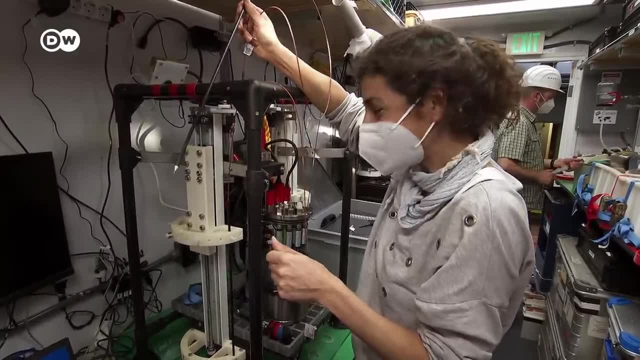 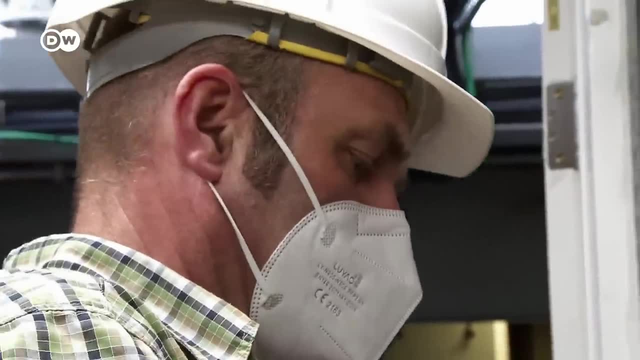 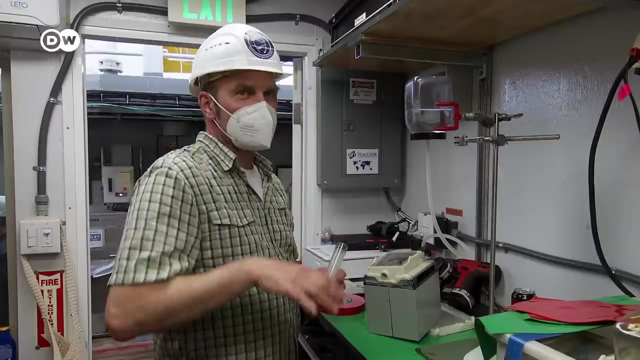 Really high-tech, right? Yes, definitely, It's a challenge for any device. Conditions are extreme kilometers below the surface. Yes, it's just turned out that what we want to measure oxygen levels on the sea floor and their distribution. 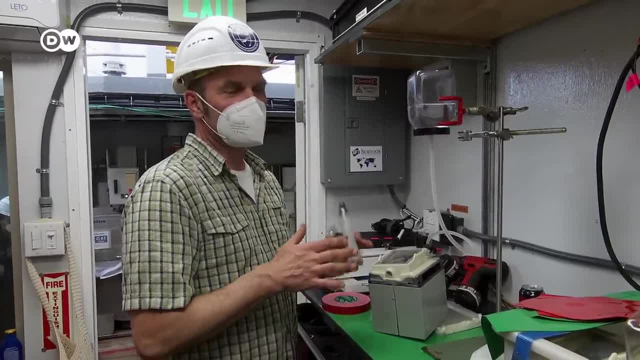 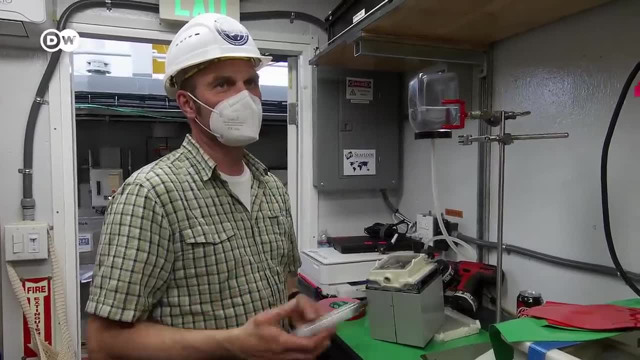 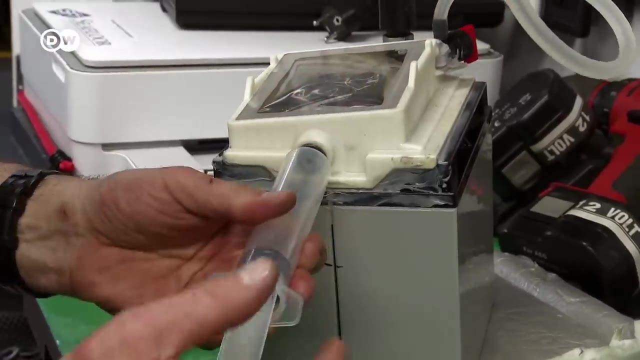 produce different results when you bring them up on deck, And oxygen is something as we know ourselves. that's essential. Many organisms use oxygen and we see that as an indicator of how much oxygen is there. It's an indicator of how much the system is disturbed. If you disturb the substrate a lot or remove it completely, you're taking away a layer that's been deposited over many thousands of years where active processes take place. You've either stirred it up or gotten rid of it, So you already have a chance. 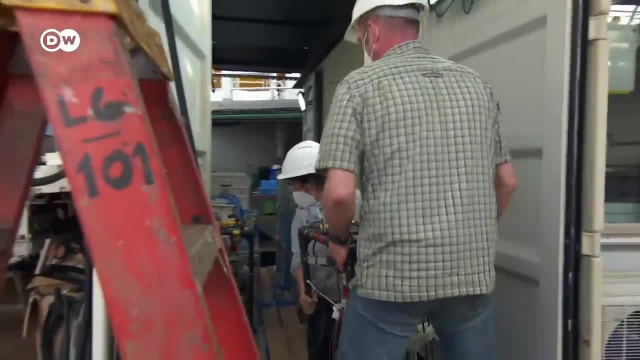 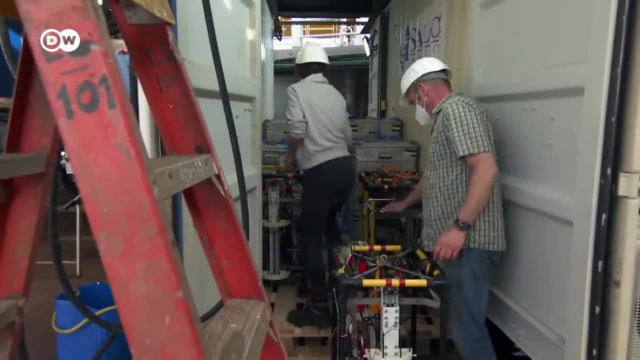 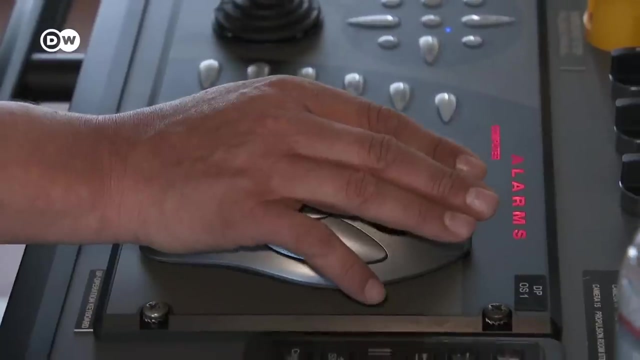 to see now from the measurements. does that have an effect or does it look exactly the same as it did before? The island pride has made its way to the Belgian license area. This is where it was due to join the ship belonging to the Belgian mining company GSR. 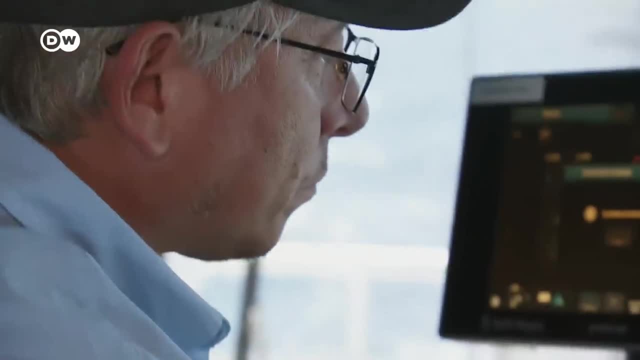 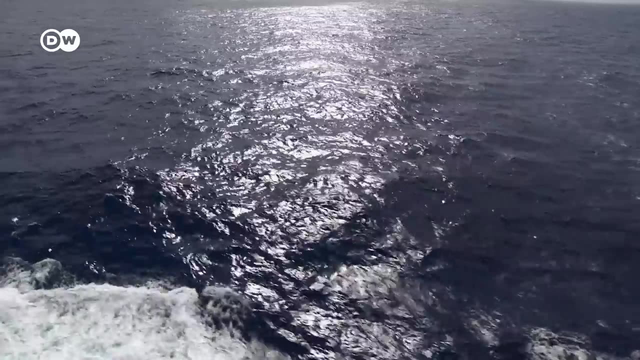 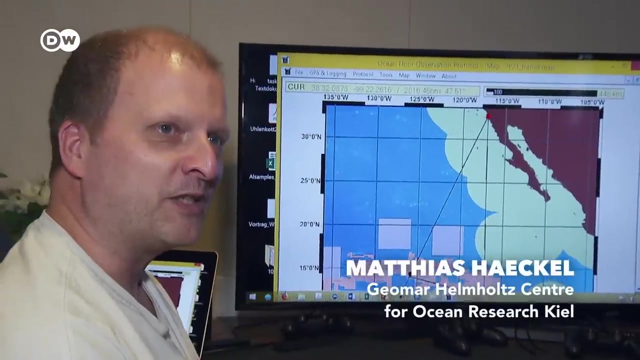 The boat was there to test Pertania, the world's first machine prototype for collecting manganese nodules. There are a lot of manganese nodules here. You can see on the map where the manganese nodules and the marked license areas of the International Seabed Authority. 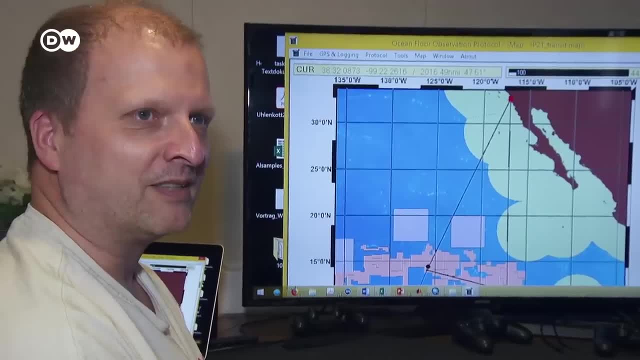 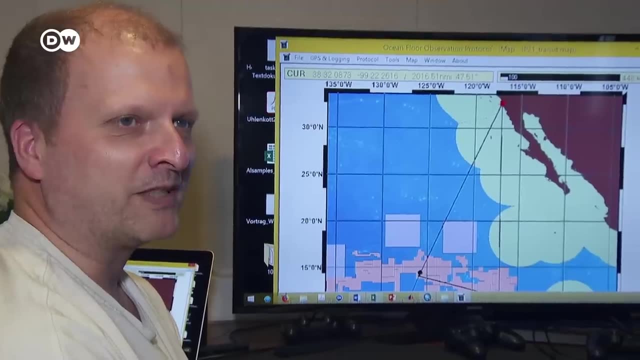 for Manganese Nodules are At the moment. these are all exploration license areas where companies or countries have acquired licenses and are looking to see how many manganese nodules are located there and which parts of the area can be mined. Now we are going to the Belgian license area. 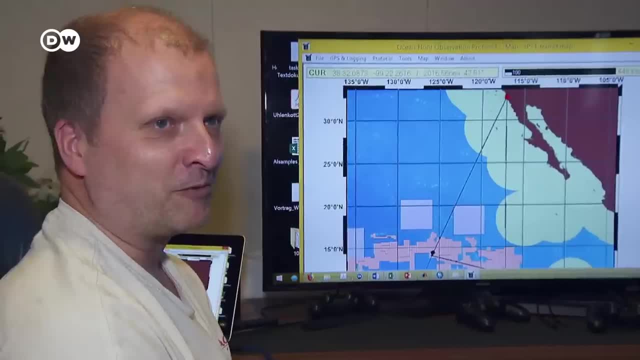 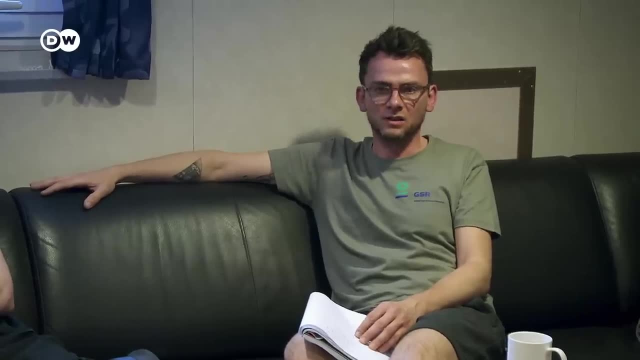 whose license is held by the company GSR, And then in two weeks we'll go to the German license area, which is a bit southwest of there, For any of the operations. GSR's person of contact, François Charlet, was also on board. He was responsible for communication. 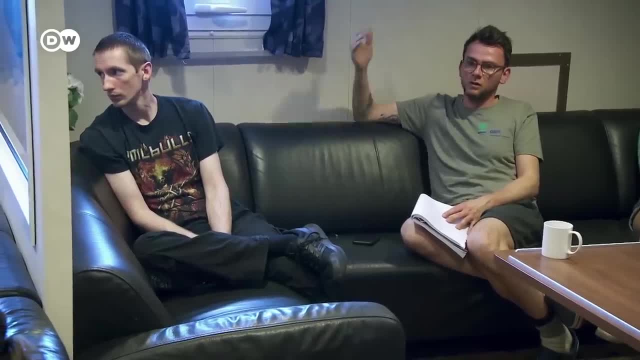 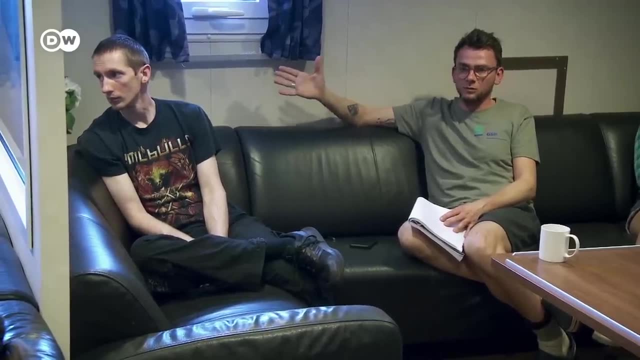 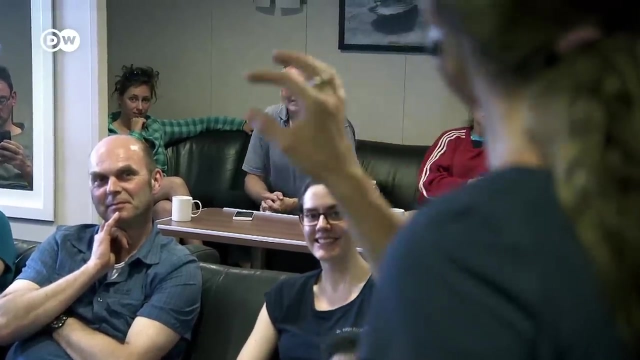 between the industrial vessel and the scientists. as the tests began in the Belgian license area, It's all a bit like the Wild West: Areas are marked out on the seabed that certain nations or companies are allowed to explore, Such as the Belgian company GSR here. 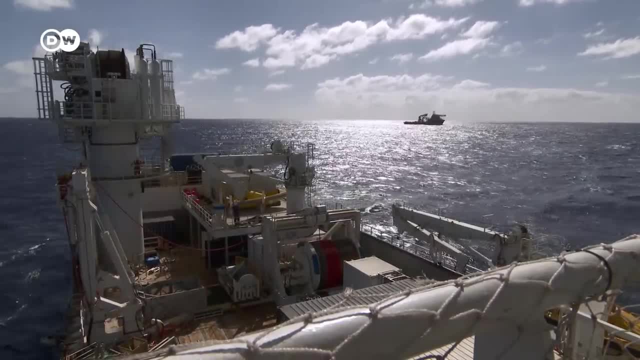 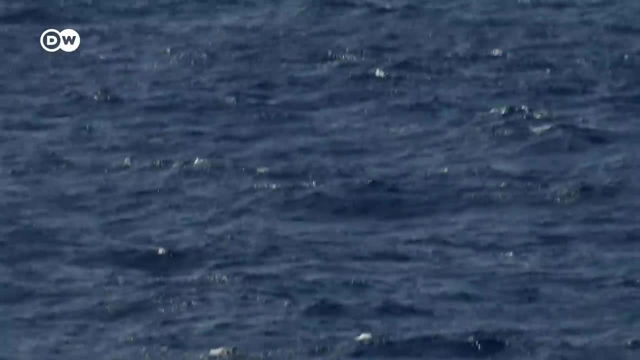 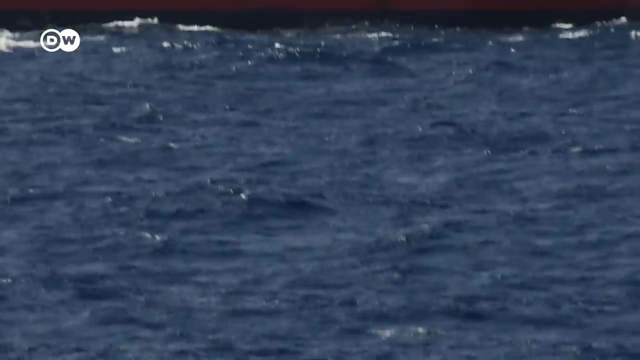 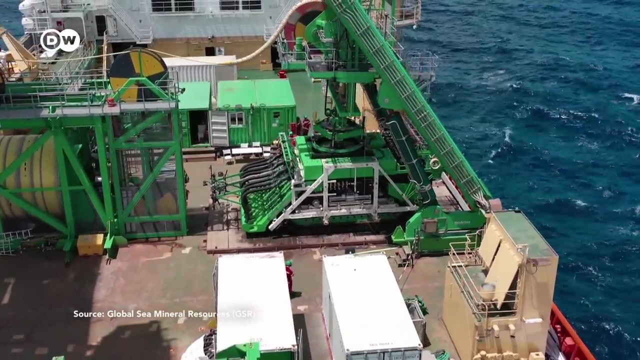 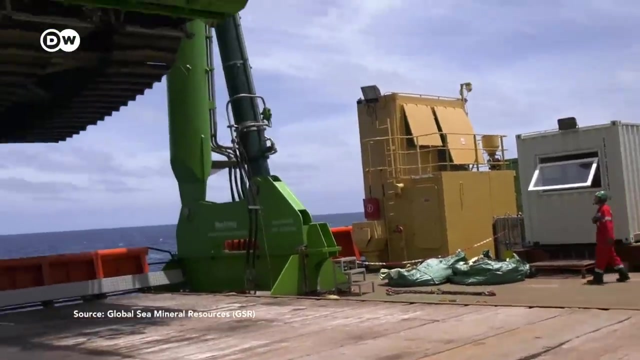 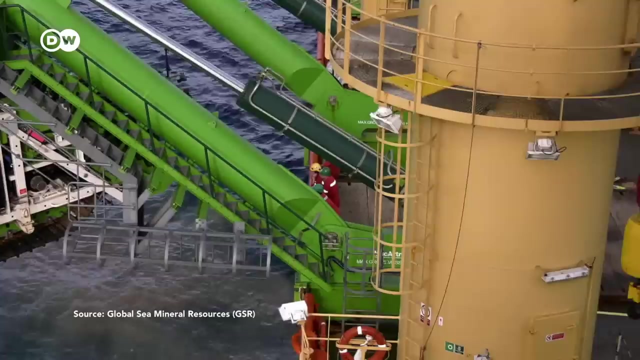 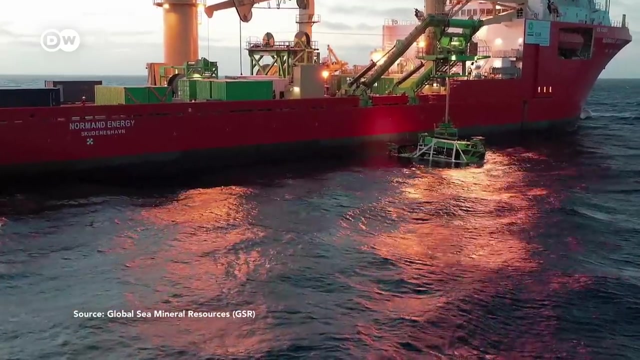 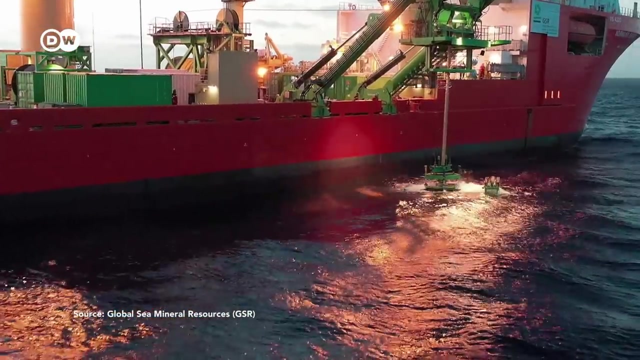 They were already in the working area. This meeting was taking place on the high seas. On the loading platform of the Normand Energy stood Pétania, able to dive to a depth of several thousand meters. It's first dive was being prepared. The technical challenge was formidable. 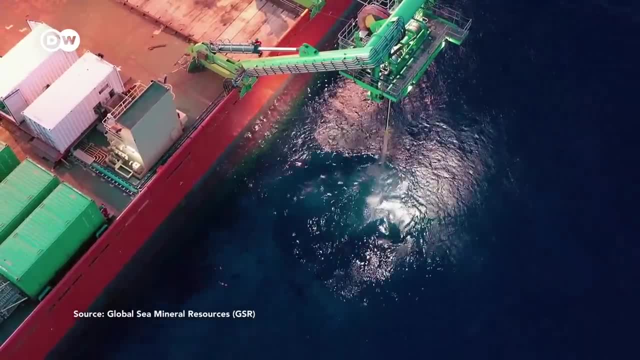 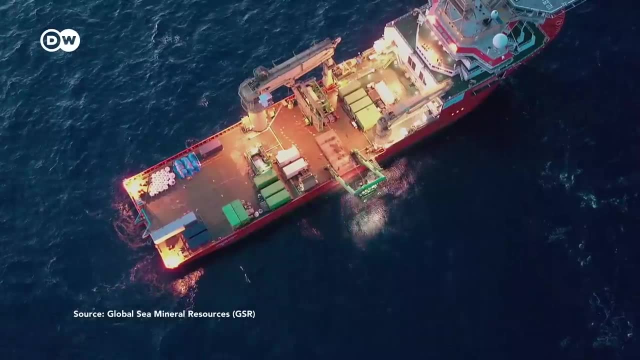 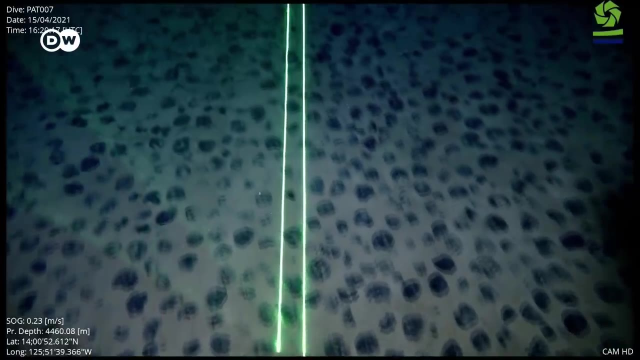 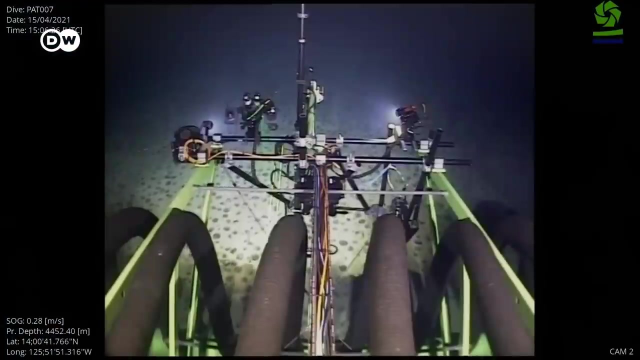 The device had to manage the extreme pressure and maneuver the programmed routes independently, Connected to the ship by a supply line only as thick as a human arm. GSR had been developing the Pétania over many years. This smaller model was built a few years ago. 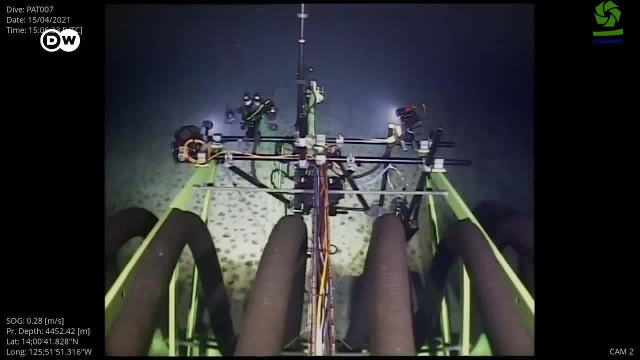 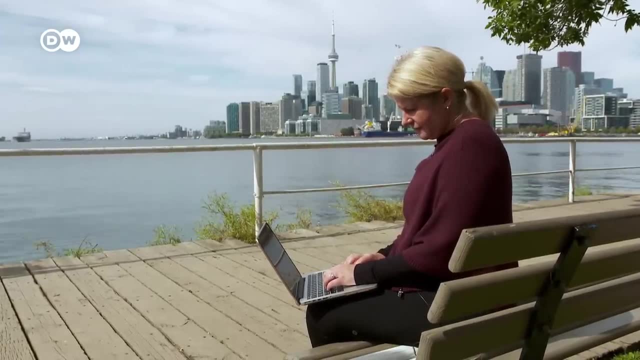 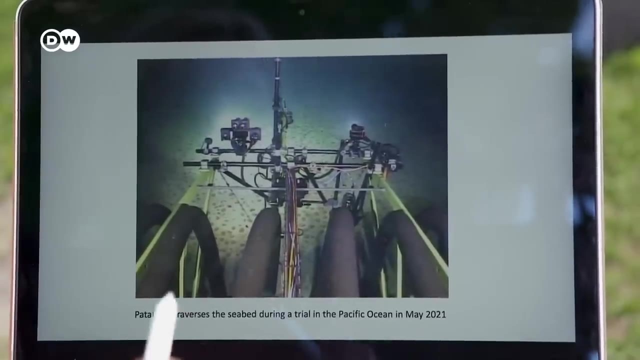 Now Pétania 2 was to face its first real test. If it passed with flying colors, the vessel could possibly become a method for commercial seabed mining in the future. So Pétania 2 is a seafloor nodule collector. 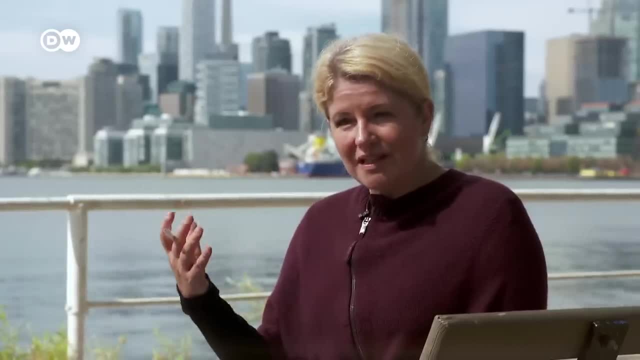 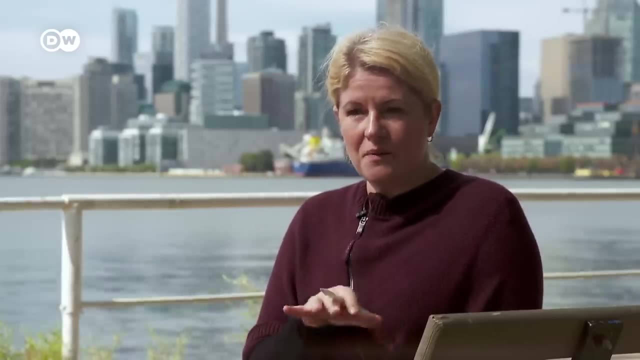 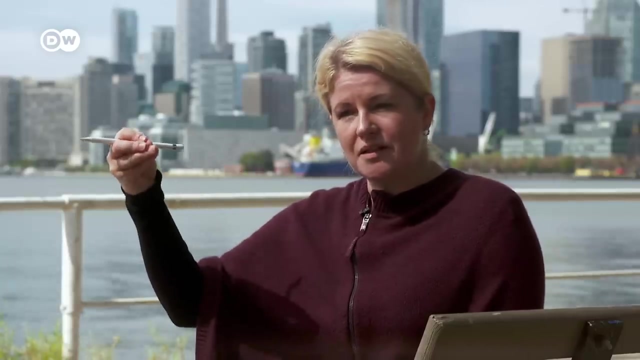 and I think the easiest way to picture it is to think of a vacuum cleaner. So the vehicle's been designed to pick up nodules and leave as much sediment behind as possible, Basically collect them, and eventually that vehicle will be collected to a riser. 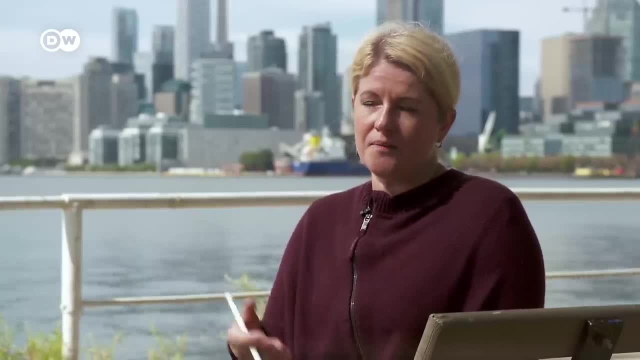 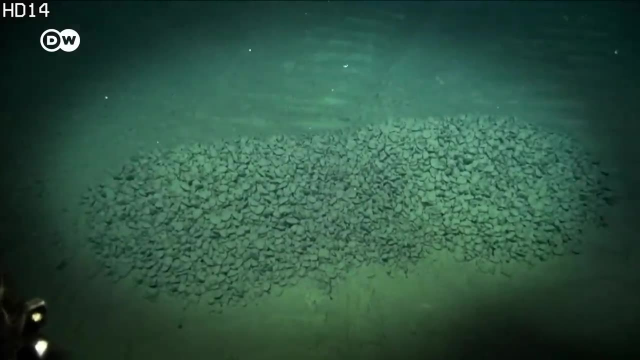 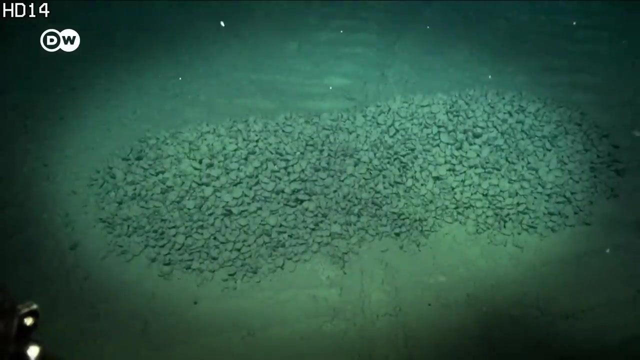 which will bring the nodules to the surface. But Pétania 2 was designed to collect the nodules and initially collected them in a bin at the back of the vehicle and then those nodules were deposited away from the vehicle's tracks at other points in the trial. 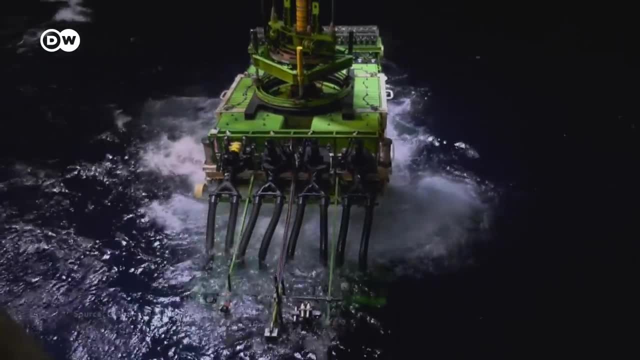 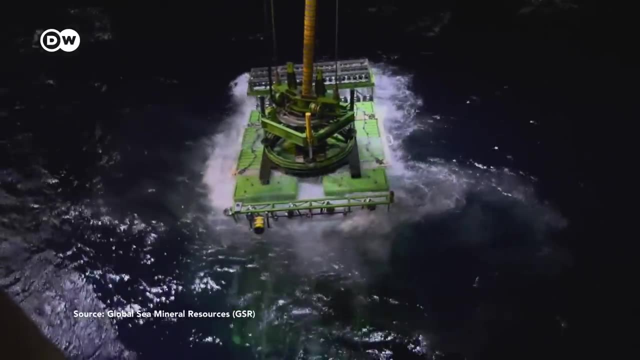 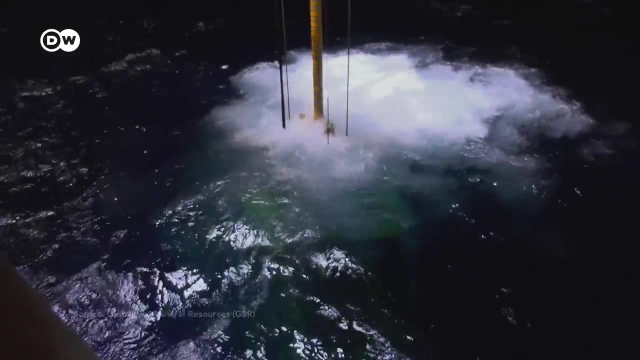 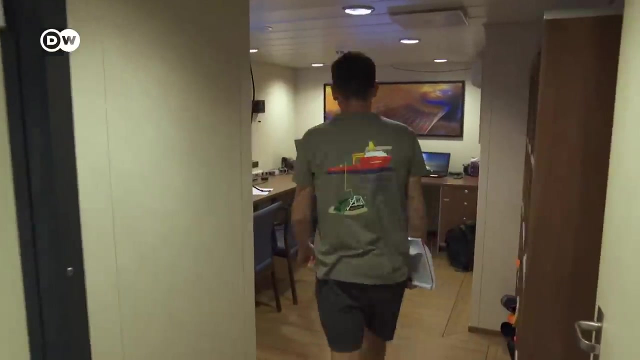 Pétania was lowered several times into the deep sea to test this new technology. It looks like something out of a science fiction movie. Meanwhile, on the island Pride, François stayed in touch with his GSR colleagues on the industrial ship and was briefed how to use. 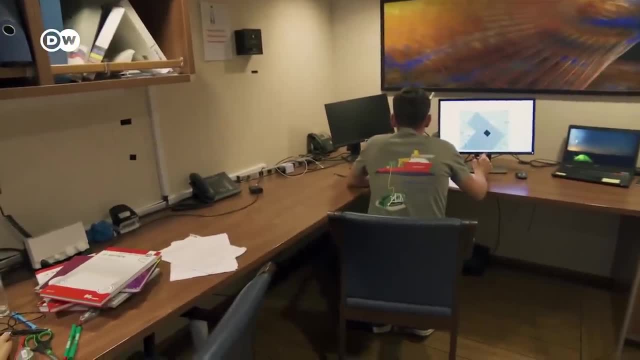 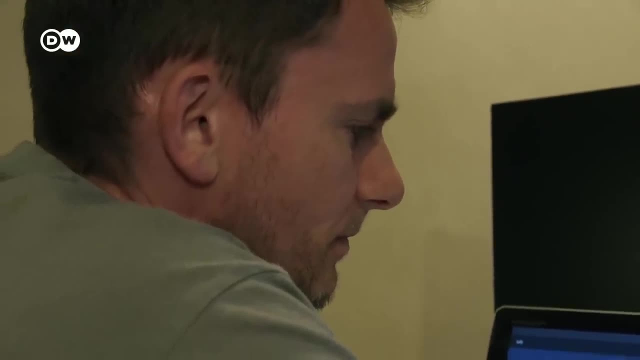 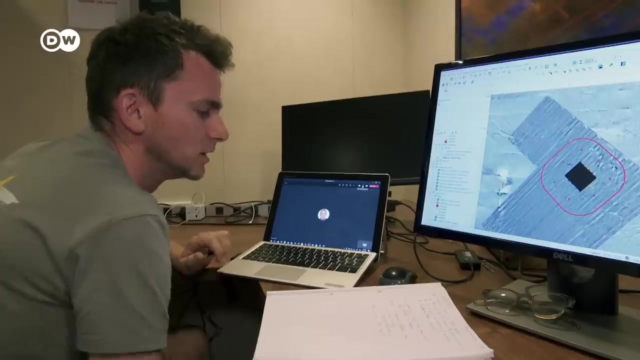 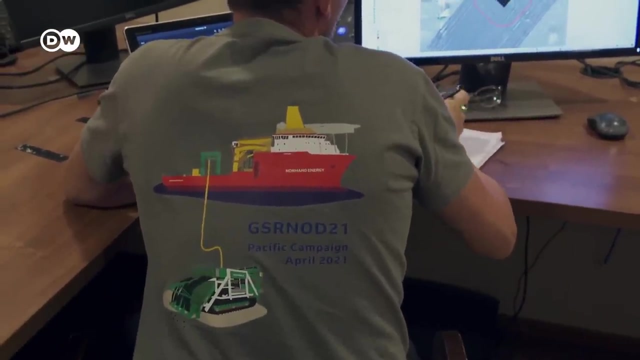 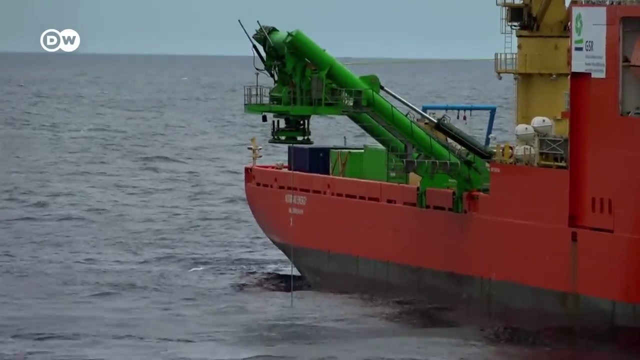 a manganese nodule collector for the upcoming dive. He had to pass this information on to the scientists so that their sensitive underwater measuring instruments would not collide with Pétania. Now, with Pétania, manganese nodule mining in the deep sea is technically feasible. 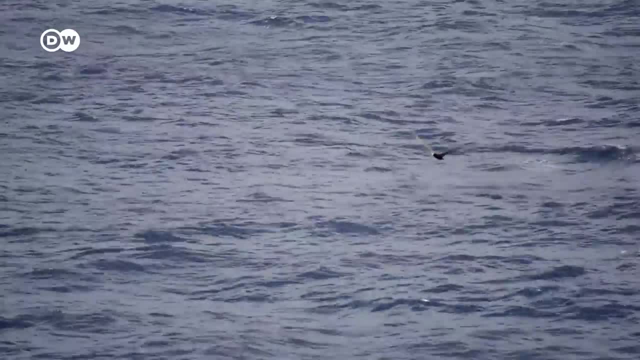 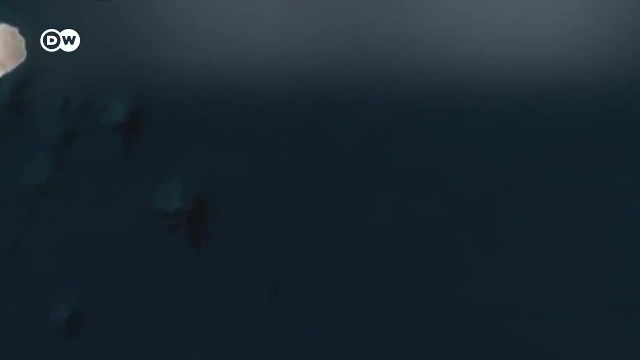 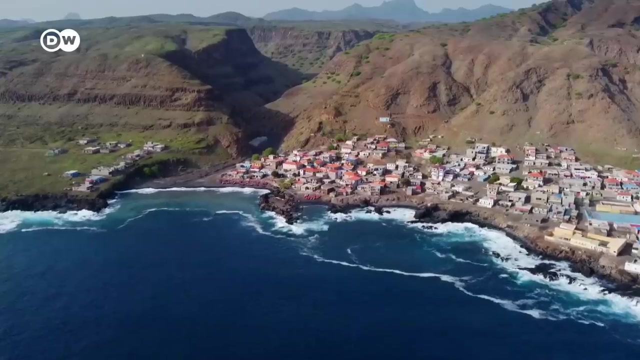 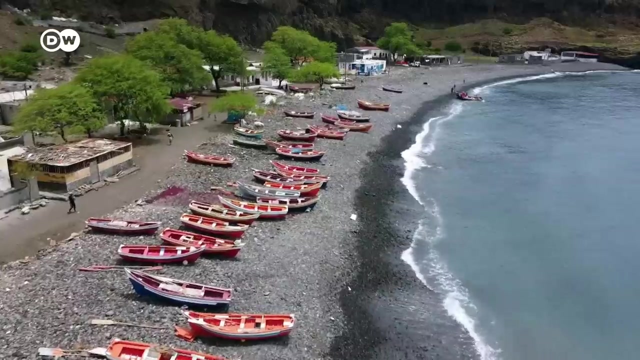 But questions still remained. How great are the environmental risks And are they worth taking? Back in Cape Verde, on the largest island of Santiago, Some of the former sandy beaches are now just barren stones. All of the sand has been gathered up and sold. 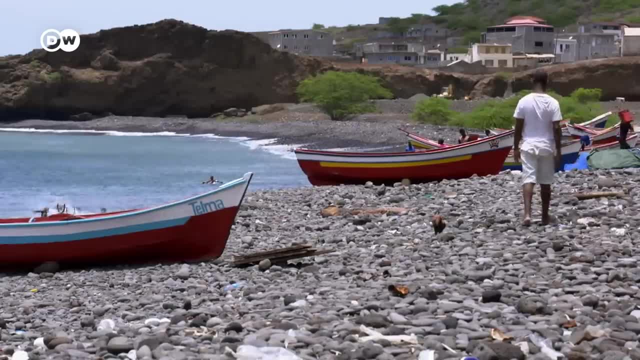 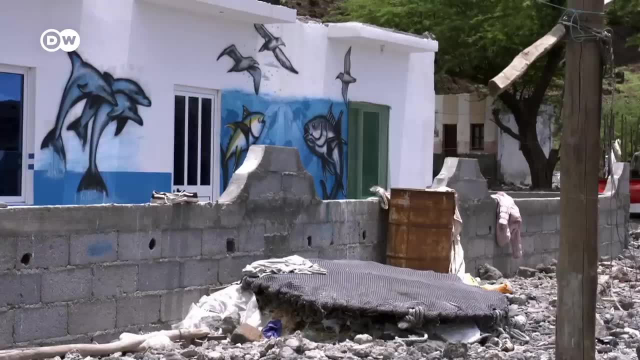 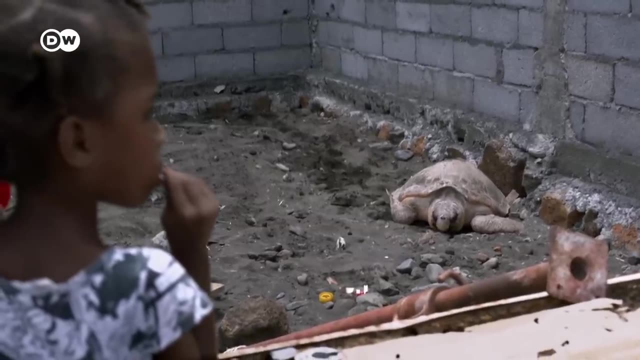 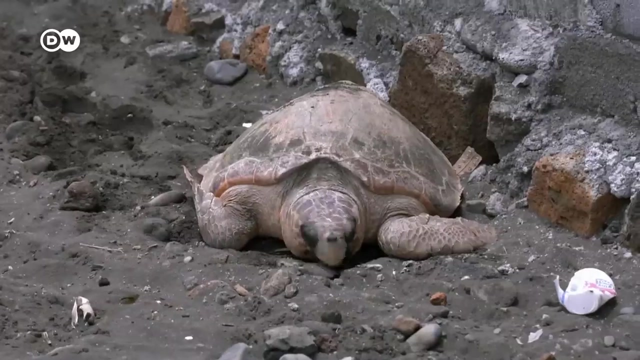 Stones mixed with garbage dominate the bays. This idyllic marine scene has been severely damaged. The world's third largest population of loggerheads- sea turtles- lives around Cape Verde. Today the animal is on the red list of endangered species. It's strictly protected. 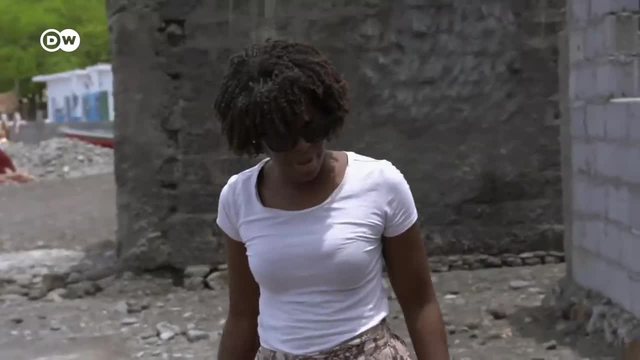 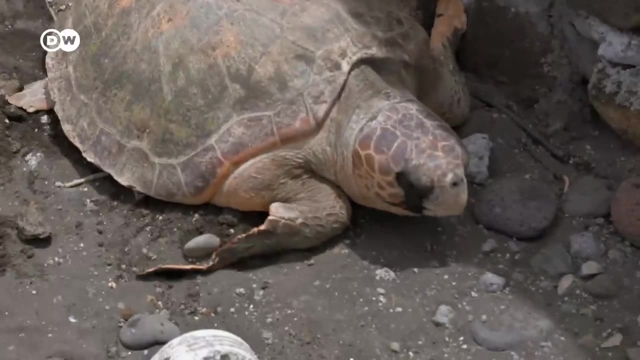 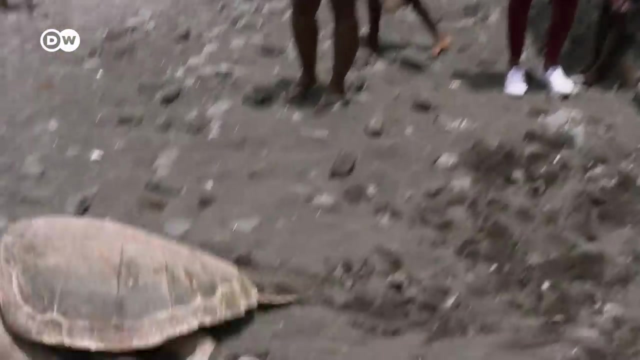 But the removal of the sand disturbs habitat vital for their reproduction. Ana Vega and her conservation organisation are committed to protecting the turtles. For Ana, it's shocking to see a female struggling over the hot stones and finding no place to lay her eggs. Yes, it used to be a sandy beach. 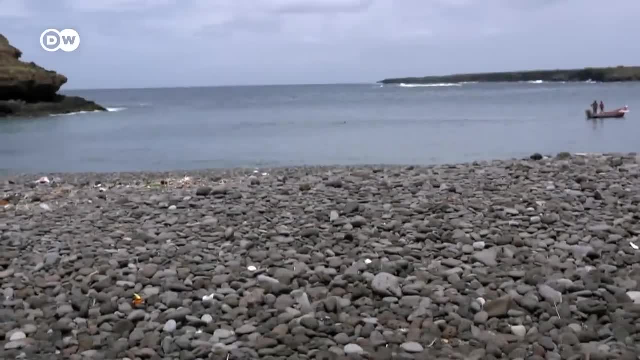 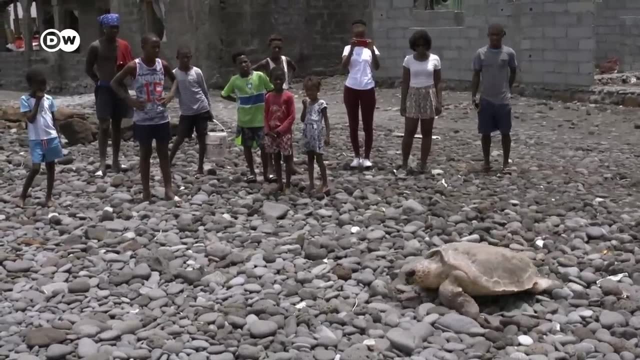 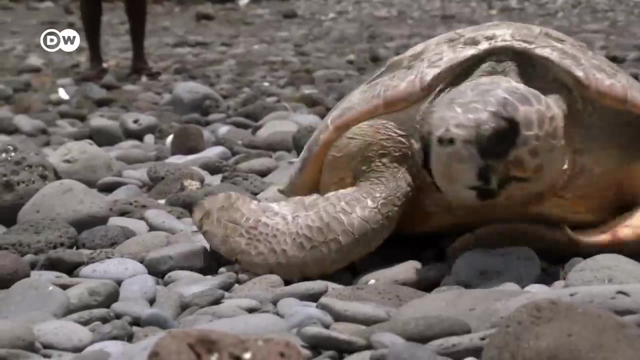 but I didn't know this place before. I've just heard from older people and locals who described the place as a sandy beach. before Turtles return to the beach where they hatched to lay their eggs, Usually it takes 20 years for the animals to reach. 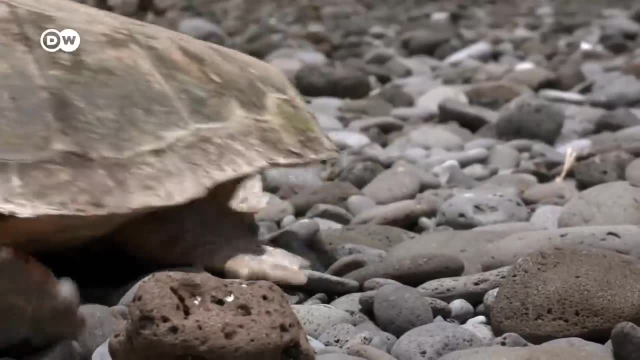 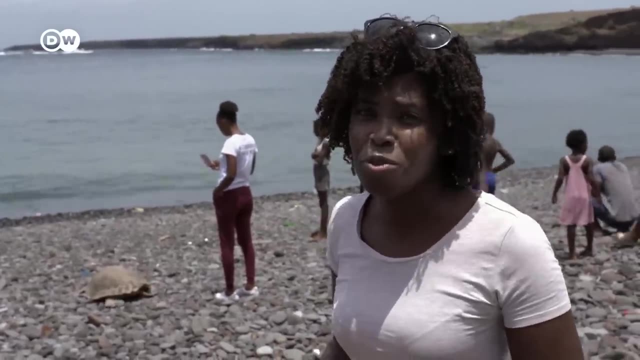 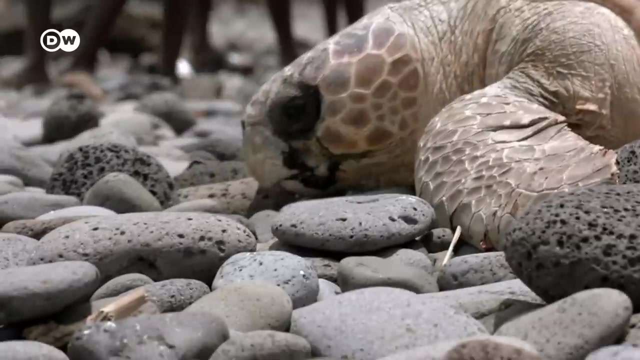 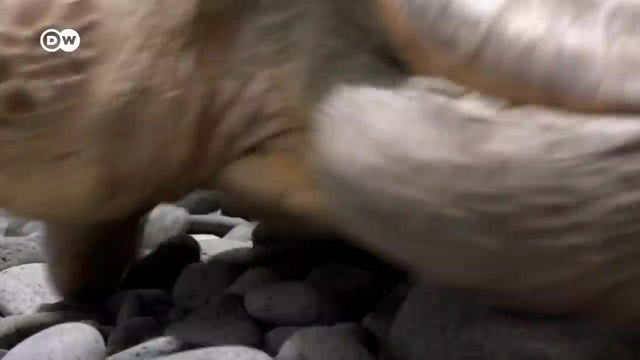 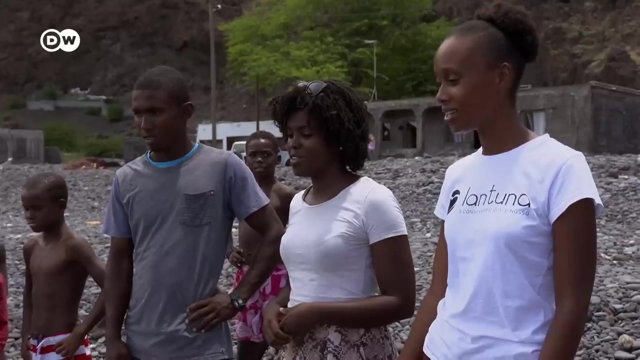 sexual maturity. But much has changed in two decades. We tried to nest here, but there is no sand. so it came out, but unfortunately it has to return to the sea. It came this morning, obviously, Yes, 7 am. It's really, really sad. 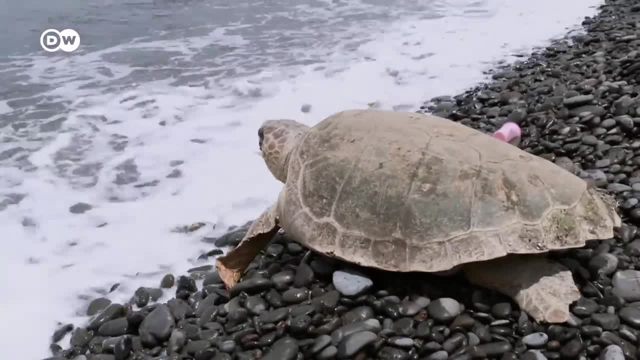 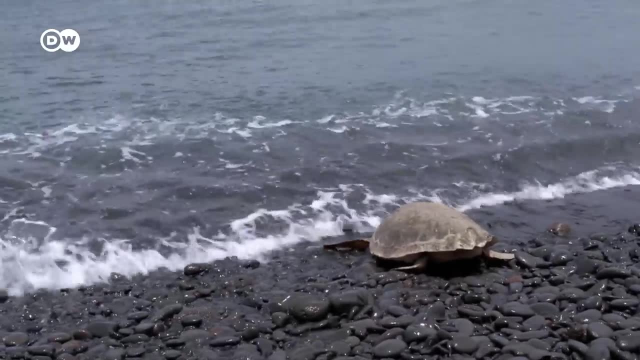 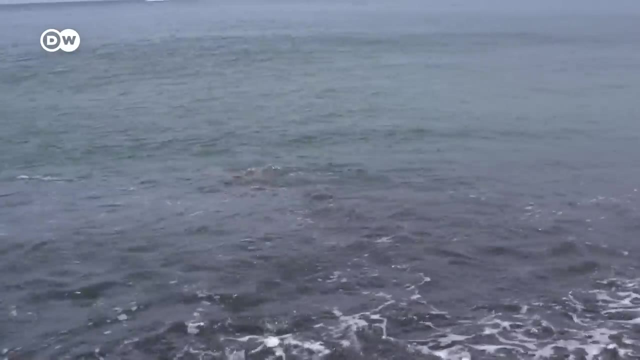 because an animal that has been born around here maybe spent 20 years more trying to nest and when it came out his house has been completely destroyed by human beings. So this is really sad. so I think we have a duty here to try to restore this place. 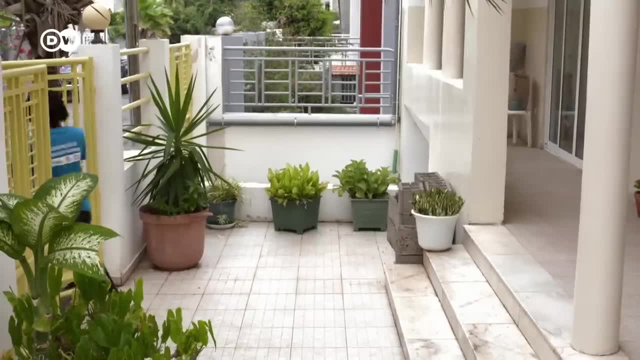 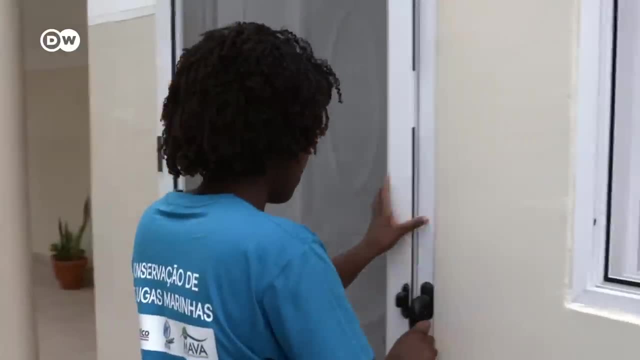 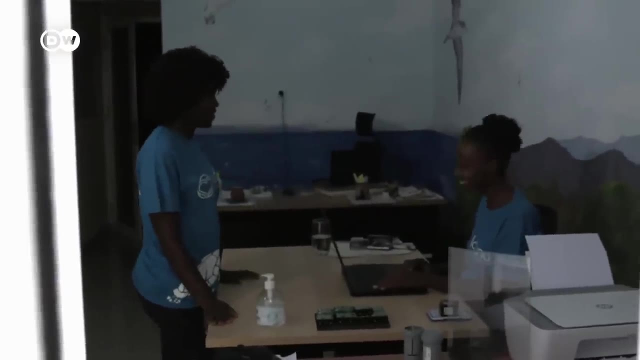 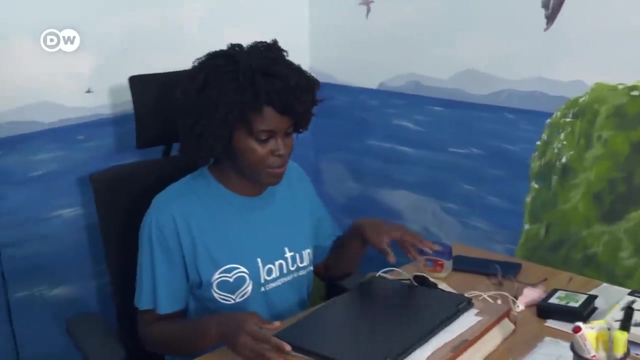 in order to promote the sea turtle conservation. Emma has a degree in marine biology. She's spent time abroad and realized that something must urgently be done in her home country to protect the oceans and nature. She founded the nature conservation organization Lantuna right here in 2013.. 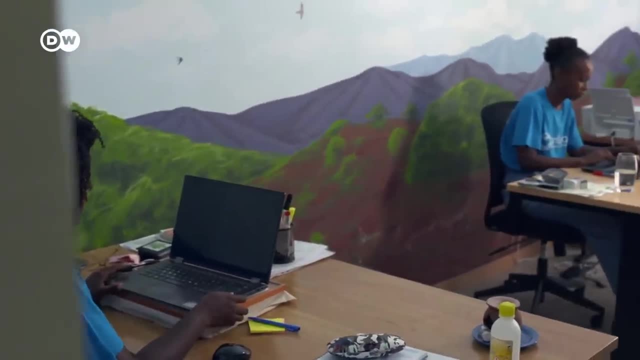 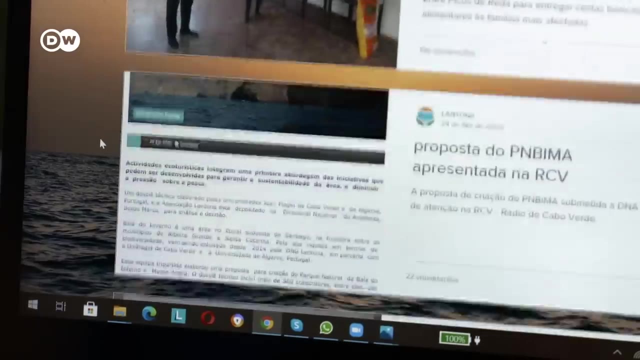 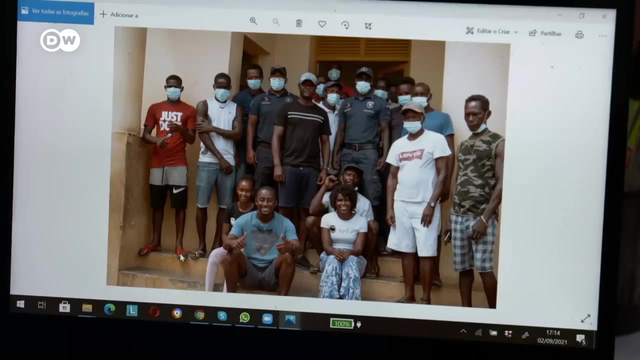 But now dozens of helpers are working on projects on the beaches. Things are really taking off. If we want the conservation to continue, we have to get them involved, to create them to have, like, a passion for the nature, for the species, and they try to conserve. 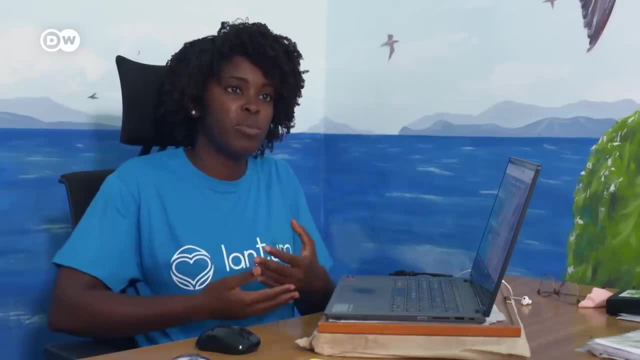 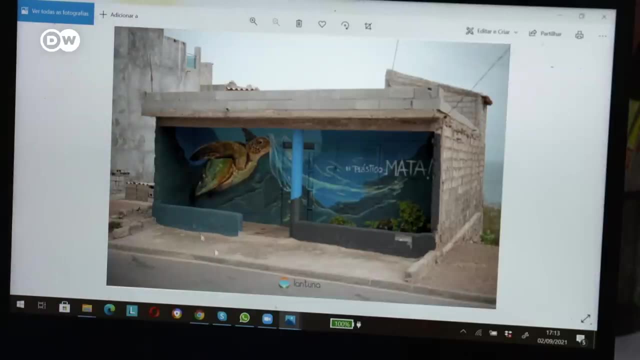 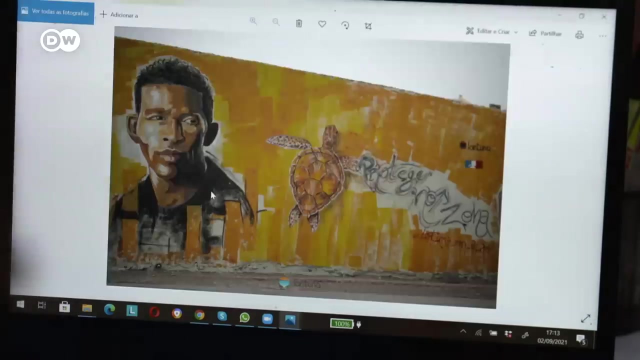 At the beginning it was more difficult, but now it's easier and every time it's easier because we start to have trust of the community. They participate and also we try to improve this by adding a bit of color. for example, Porto Mosquito is the name. 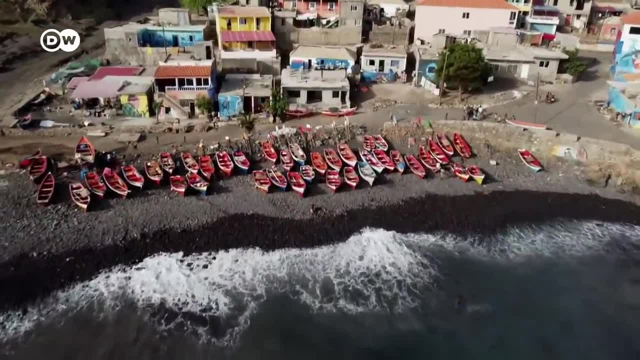 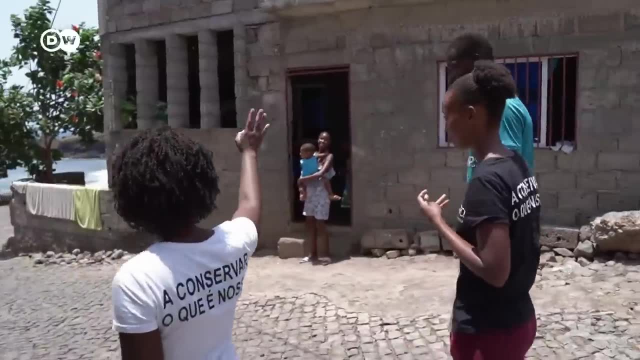 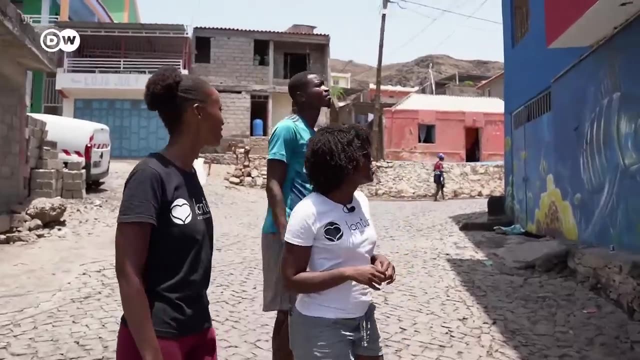 of this fishing village on the Baia do Inferno Hell's Bay. The fishing boats are beached on stones. the sand long shipped away. Anna now walks through the village and she's proud. A lot has changed here in the last few months. 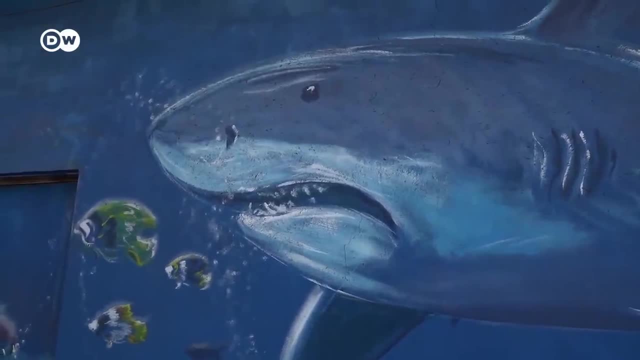 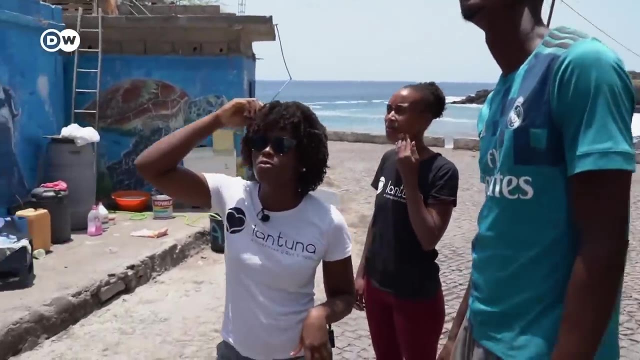 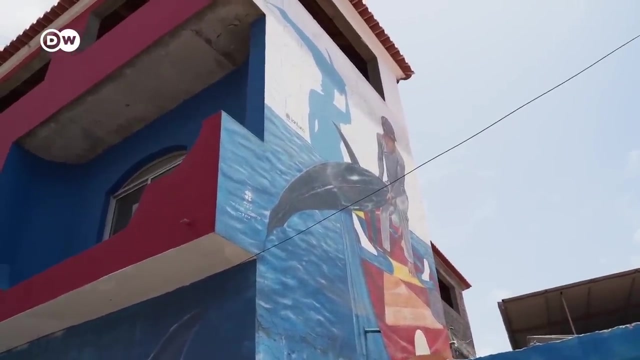 The place has a new look In the painting. it was to do awareness activities regarding the fishing and sea birds And the locals. they like it and we saw it as a positive way of making people more aware about the nature conservation. So we started doing the paintings. 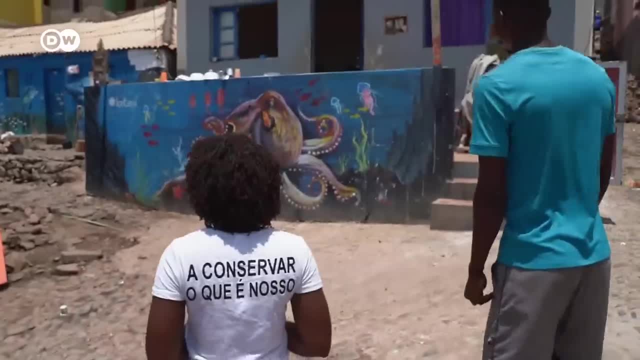 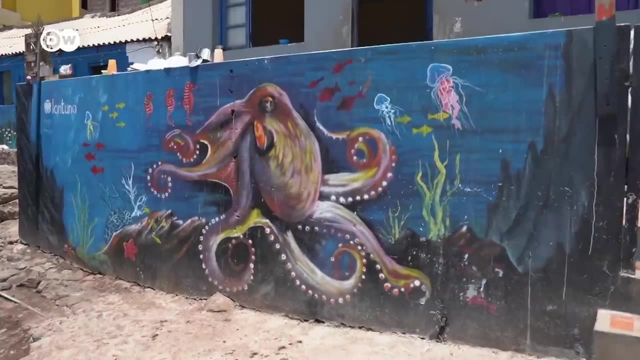 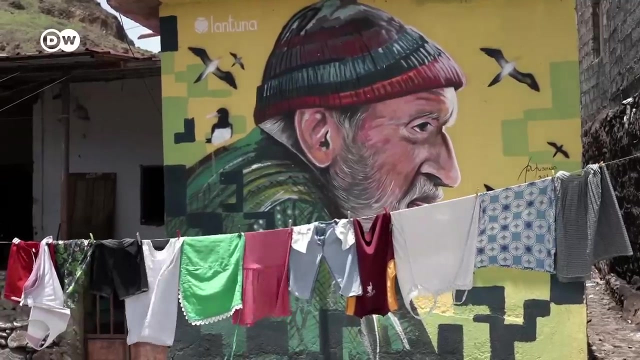 about the local biodiversity. and we didn't stop yet. So we plan to do more paintings, to cover the village with beautiful paintings and associate this visit with ecotourism activities. Now, ocean flora and fauna decorate the facades of the houses. They're a constant reminder. 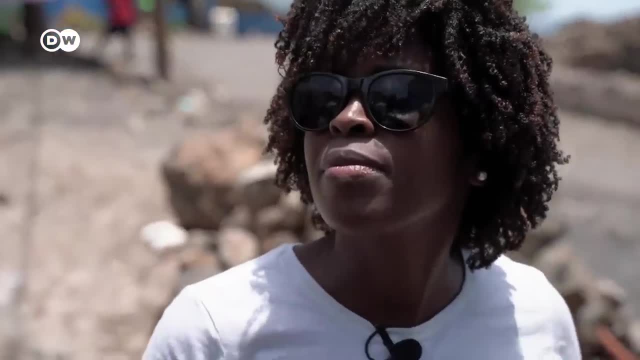 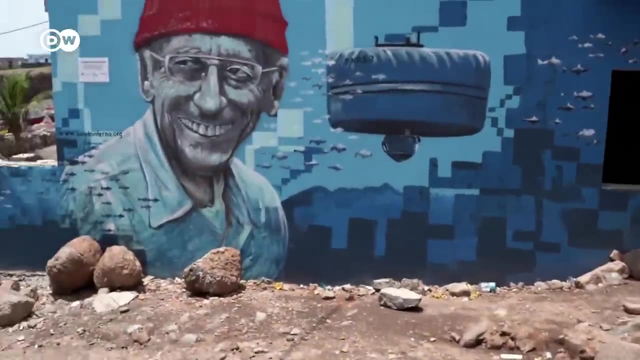 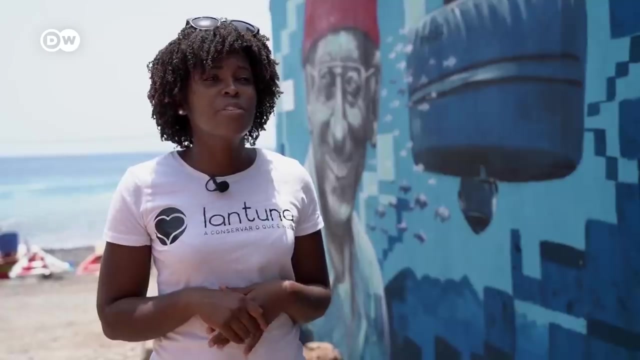 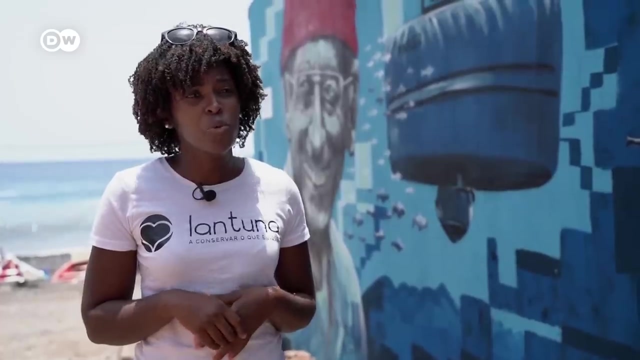 of the importance of preservation, And this famous marine explorer plays an important role. Jacques Cousteau visited Bahia do Inferno in 1948 with two other colleagues, Theodore Monod and Auguste Picard, So they came here to test an equipment. 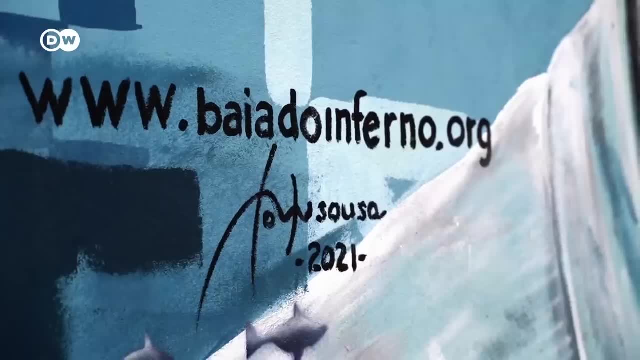 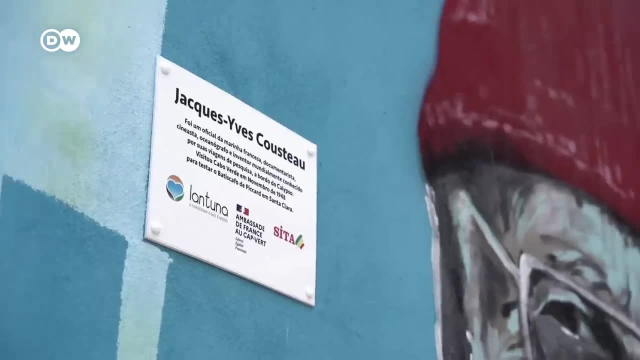 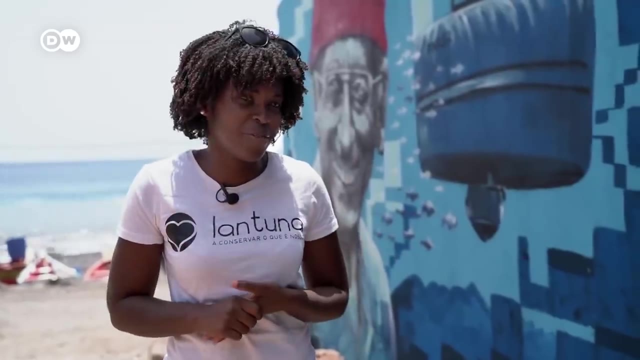 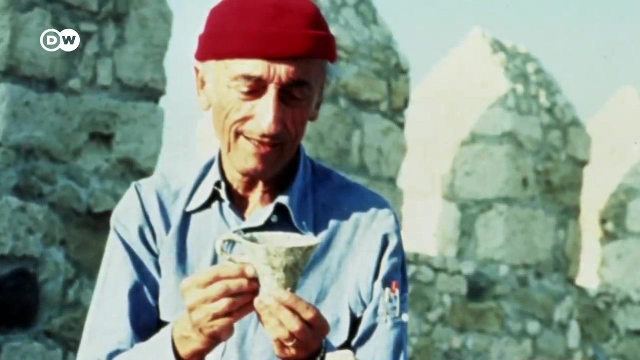 They wanted the equipment to do some recording in a very deep ocean, So we decided to bring back this memory that was almost lost, because the majority of the locals didn't even know if he was around here. Jacques Cousteau was a legendary ocean explorer. 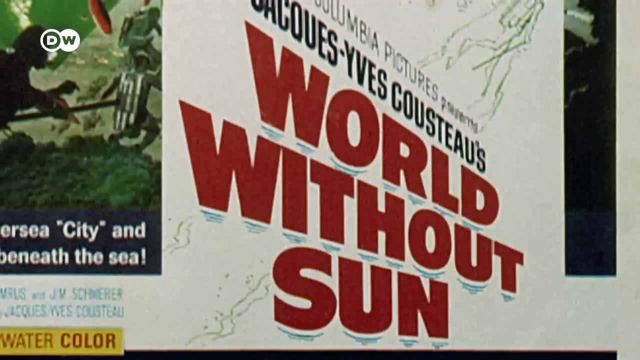 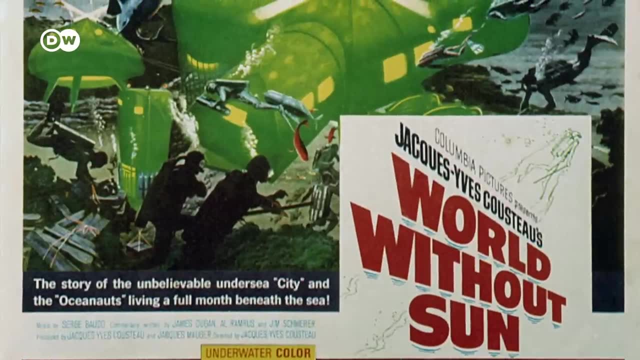 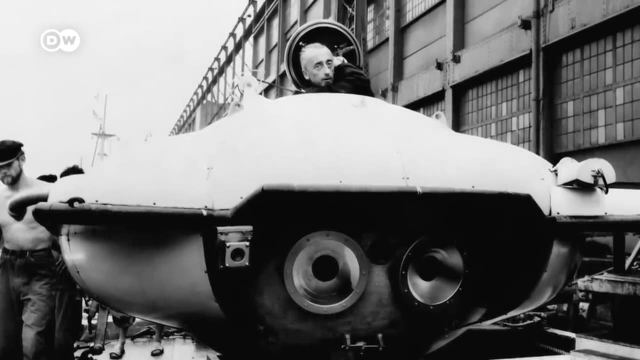 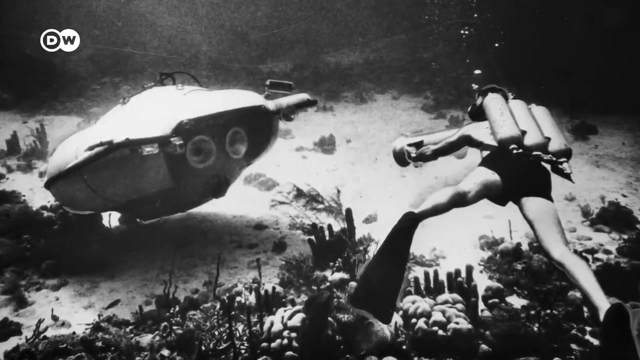 The French diving pioneer and documentary filmmaker, introduced people to the underwater world like no other. He brought images of the depths never seen before into the world's living rooms. Cousteau wanted to explore the unknown world under the sea and called for the oceans to be protected. 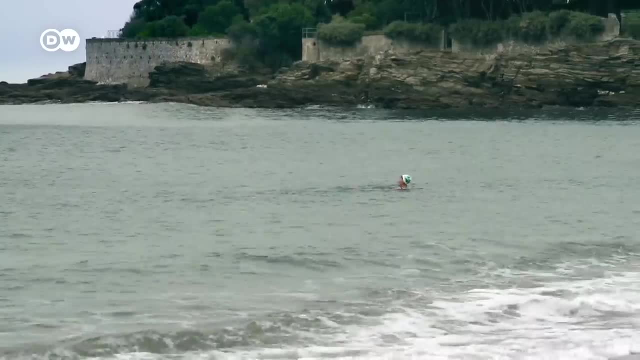 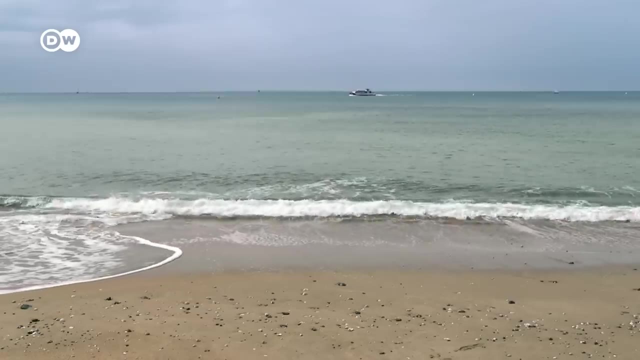 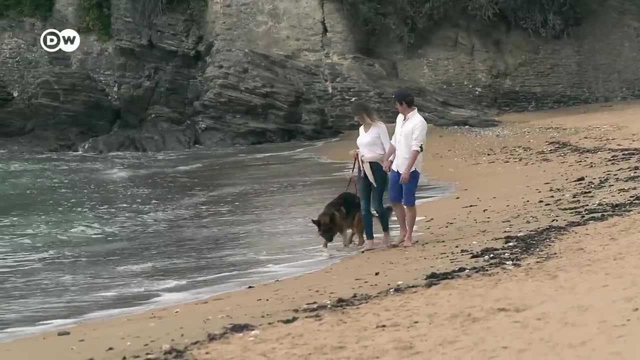 This is the French Atlantic coast, not far from the mouth of the Loire River. The granddaughter of Jacques Cousteau and her family live nearby. After her father's early death, Alexandra Cousteau spent almost her entire childhood with her grandfather. 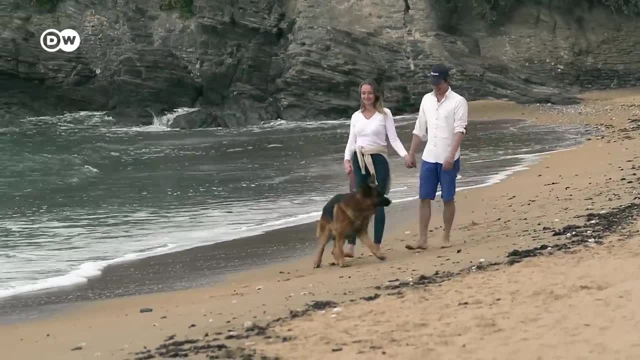 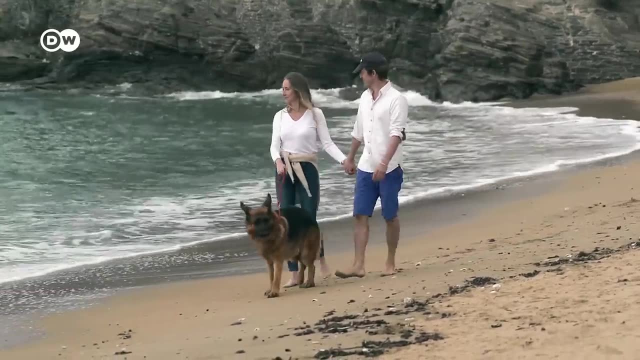 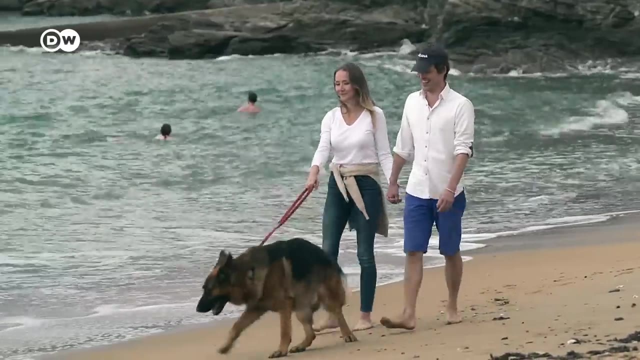 That left its mark. She's very concerned about the state of the oceans. I think if we continue with business as usual, where we're overfishing, we're polluting, we are advancing with ideas like deep-sea mining- we're going to see. 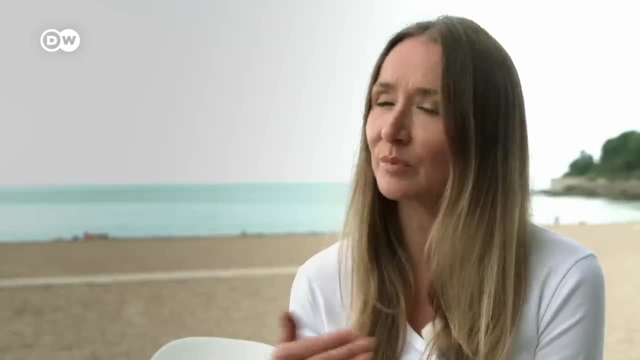 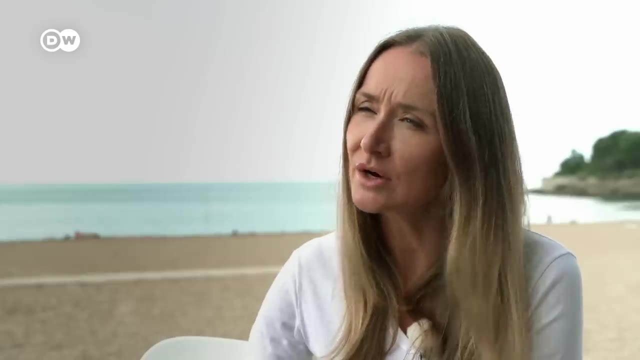 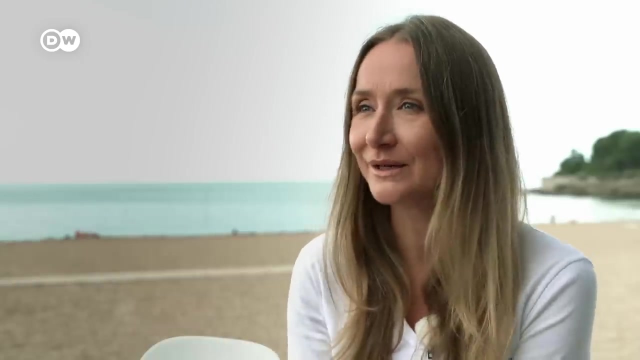 our oceans disappear, We'll continue to see a decline. At a certain point you reach tipping points where you have exponential loss And that's hard to come back from. You can't really come back from exponential loss. The damage is done. 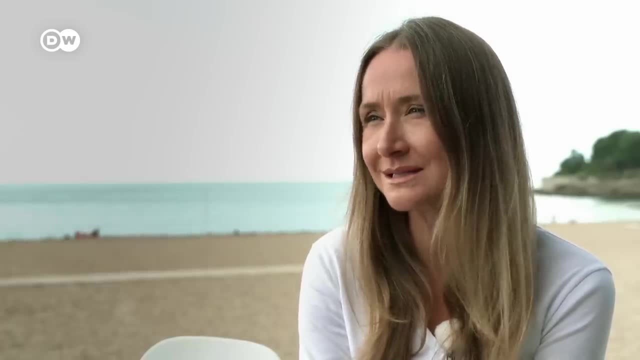 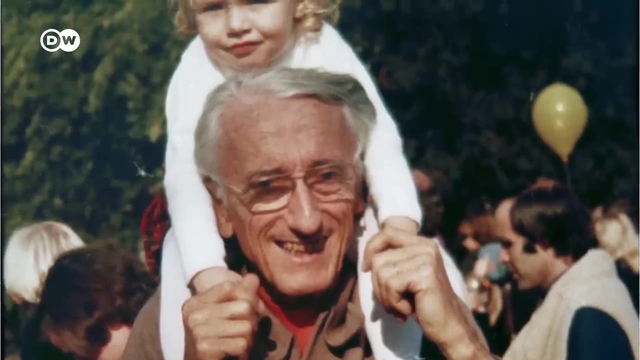 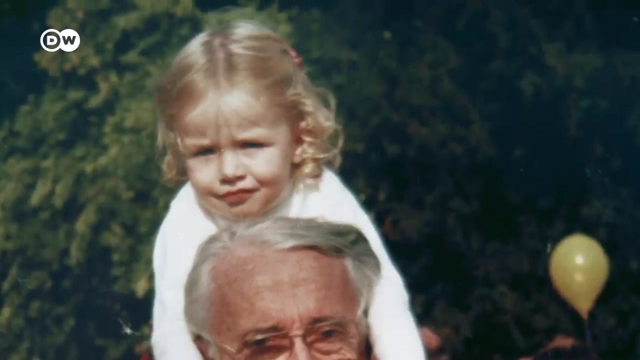 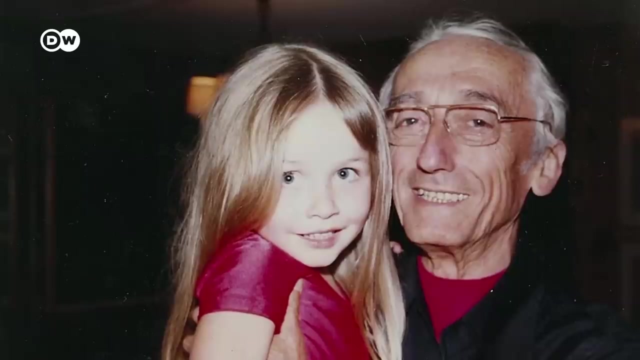 Once we reach those tipping points with the ocean, the damage will be done. We won't be able to reverse it. Alexandra says that her grandfather taught her to dive before she could walk. Her love of the oceans is his legacy. Like him, she makes documentaries. 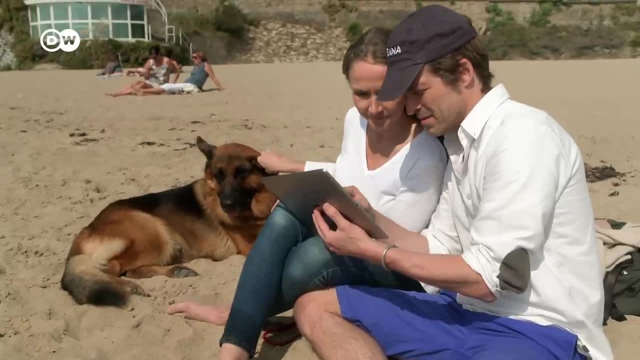 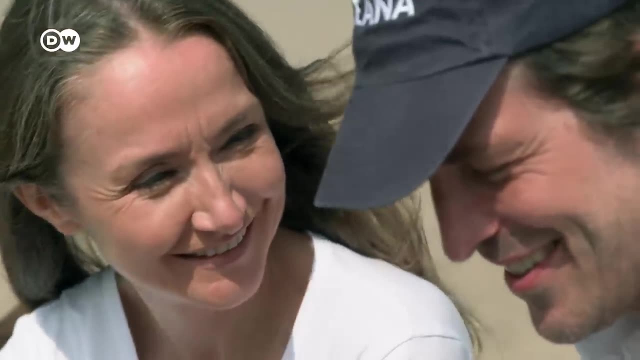 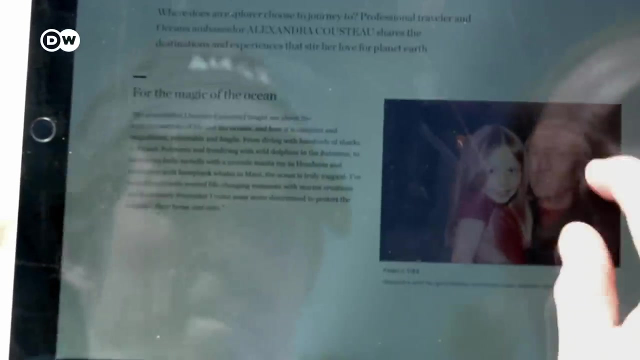 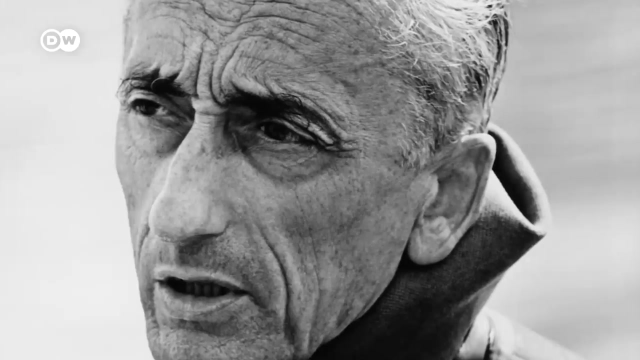 advocates for the preservation and looks for ways to save the oceans. She wishes she still had her grandfather at her side, in addition to her husband, who's there now. My grandfather passed away 20 years ago and left a huge void in the world, Not just for me. 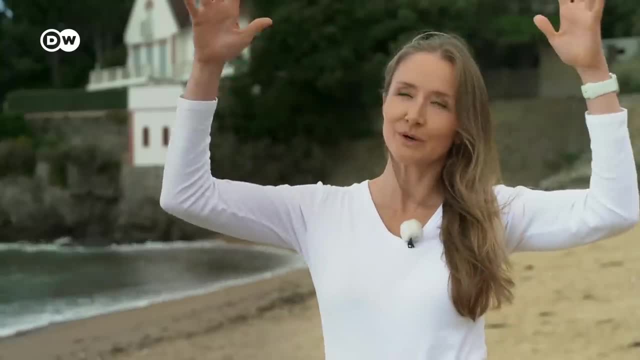 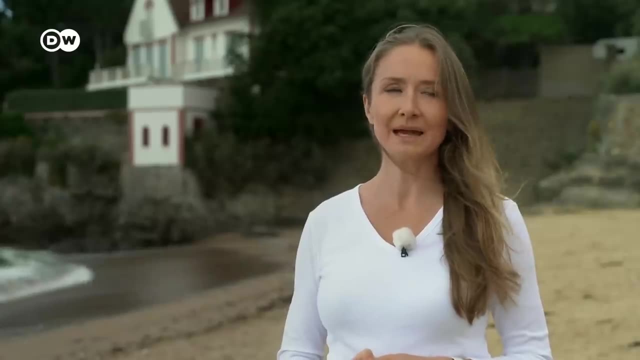 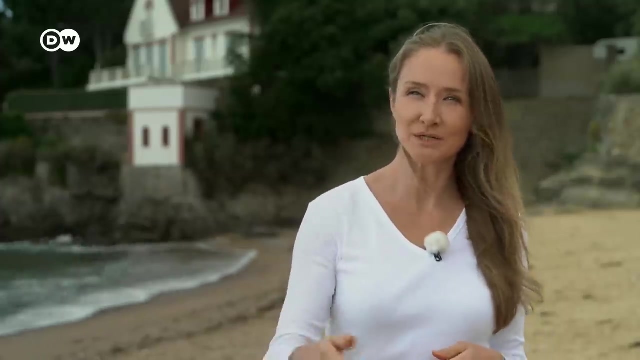 and my family. but I think there was this huge Jacques Cousteau shaped hole in the universe after he died that no one can fill. But what I realized is that every time someone tells me I grew up watching your grandfather, he really inspired me. I love the ocean now. 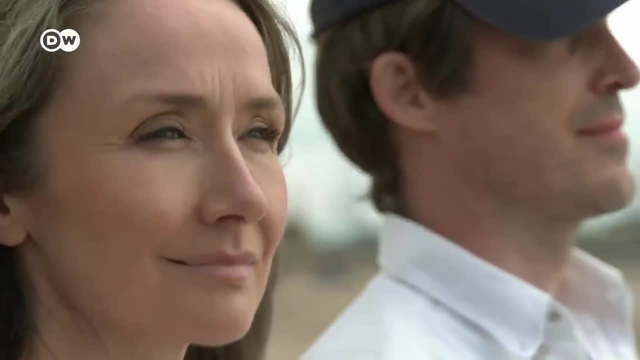 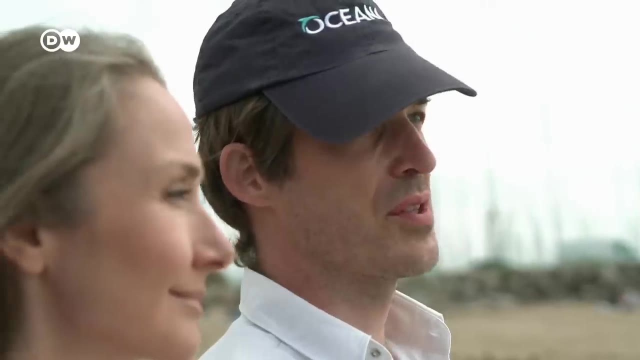 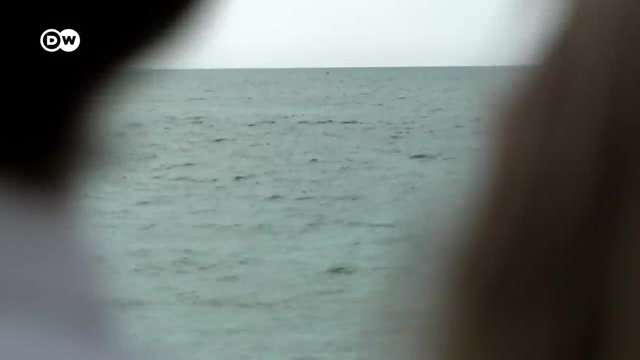 and I want to do something to help protect it. We are finally at a point in time where we can. Maybe 10 years ago, 20 years ago, we weren't. We didn't have the technologies, we didn't have the solutions, we didn't have the urgency that we have today. 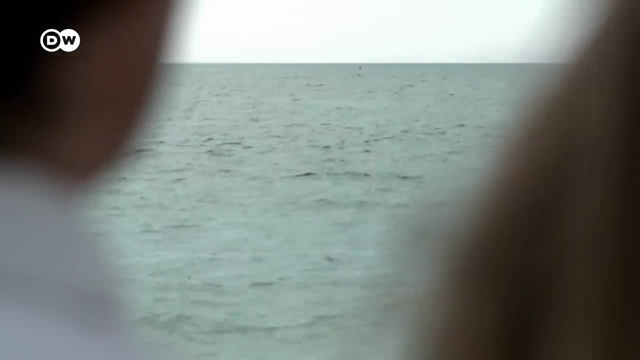 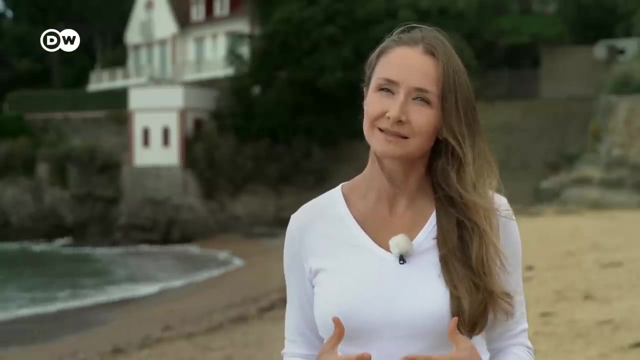 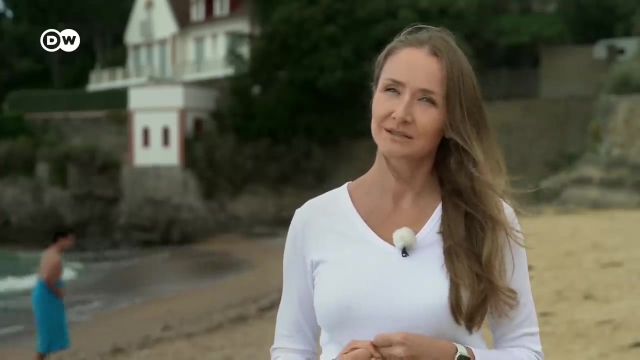 And so my hope is that, for everyone who loved him and loved his films and loved exploring the oceans with him and that discovery and sense of awe and wonder that he brought, my hope is that they will harness that and use it to create change, Because that is the best legacy. 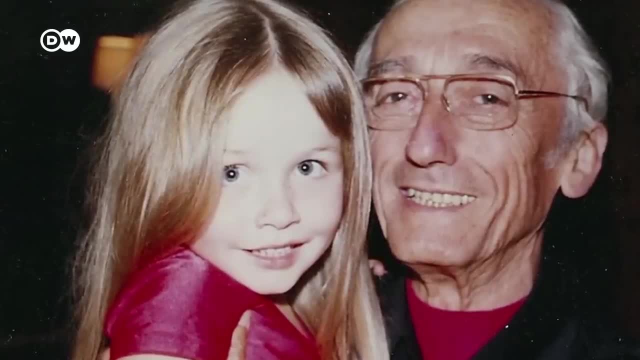 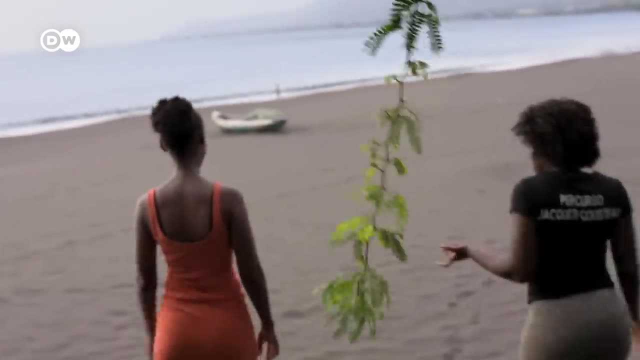 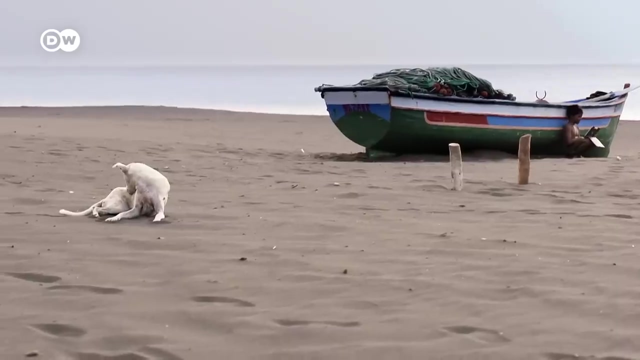 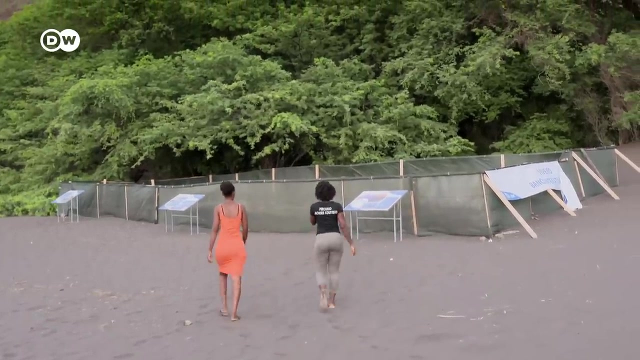 he could possibly have left us. On the Cape Verde Islands, Anna and her group of helpers have built a protection area for turtle clutches on one of the remaining sandy beaches. Educational signs show passers by the importance of the oceans and the life in them. 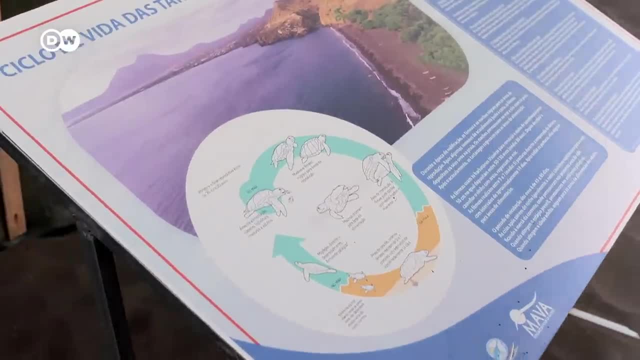 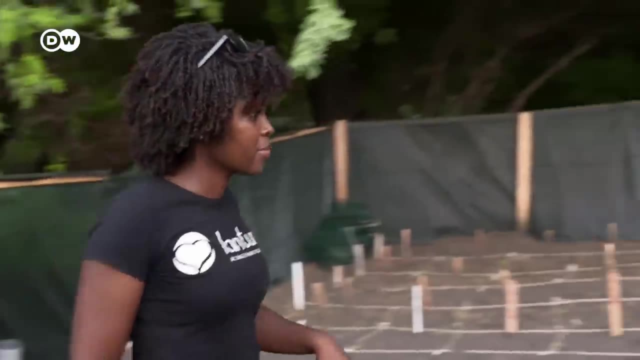 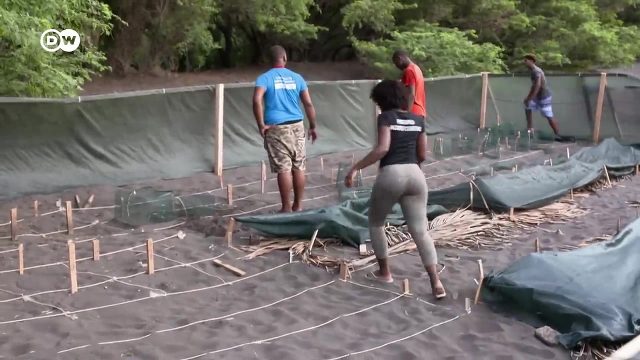 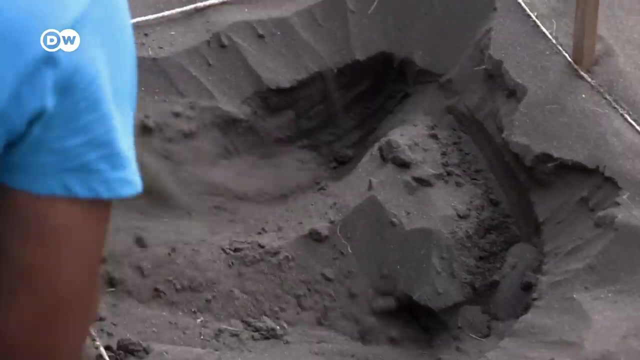 This is where the turtles lay their eggs For weeks. Lantuna watches over the clutches of eggs that have been collected Here. the organisation ensures the baby turtles can hatch safely. We are checking which nest already hatched, because this is actually where we put the nest. 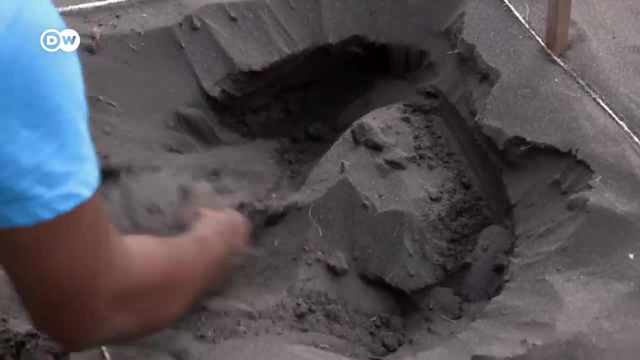 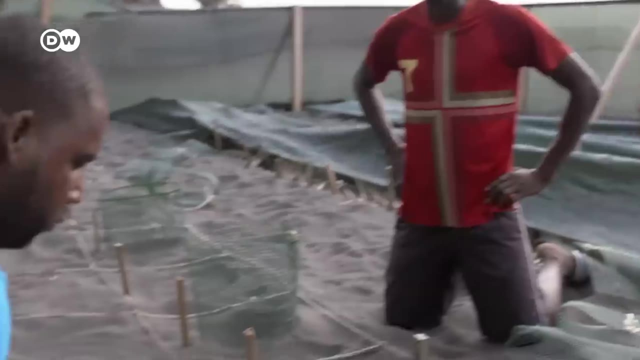 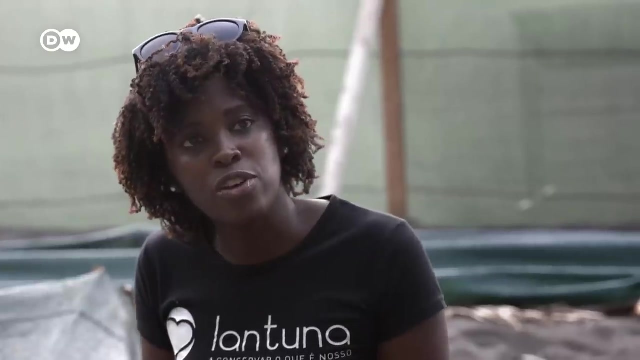 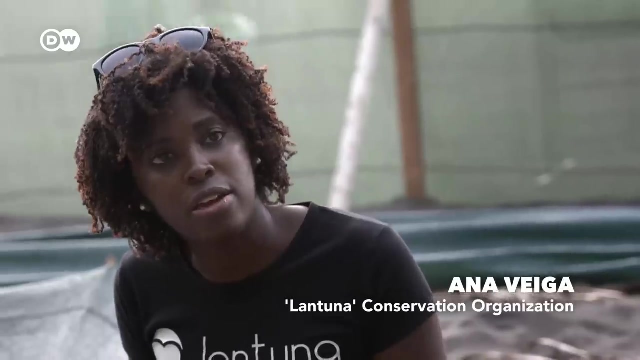 they are at risk. By now we have seven nests here, so the team were checking if they are about to hatch. Through the conservation we create opportunities for people to have a job so that they can earn some money for their families and also try to create. 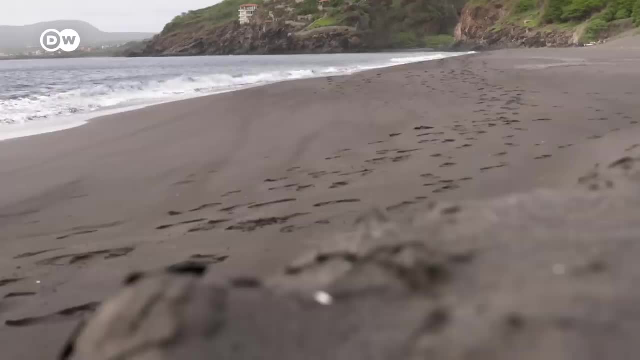 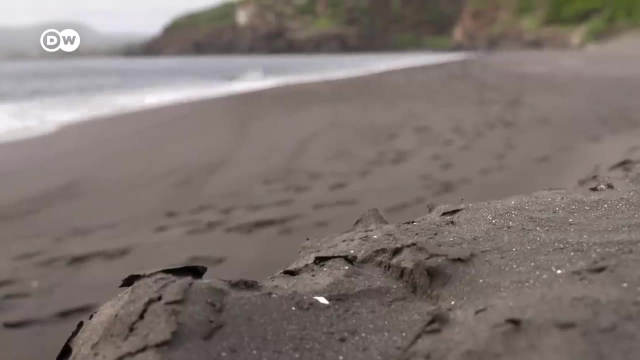 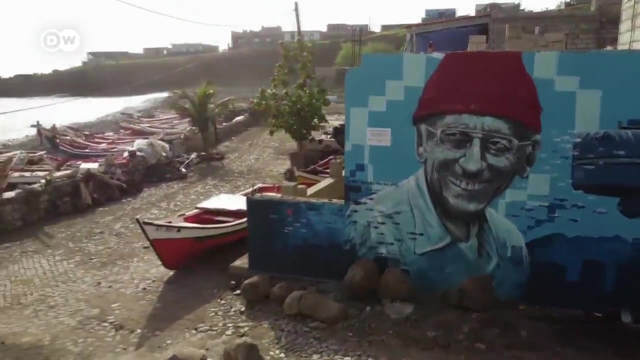 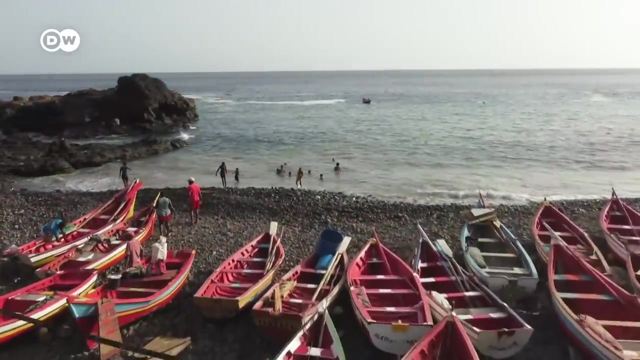 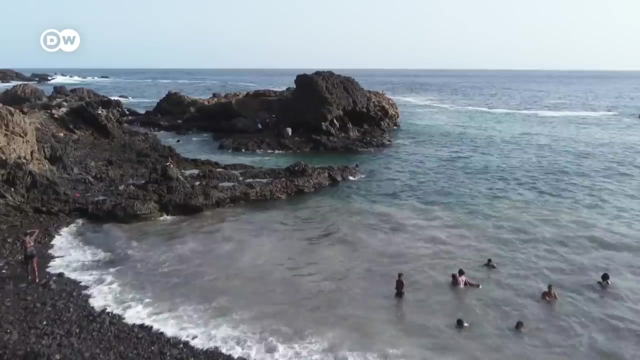 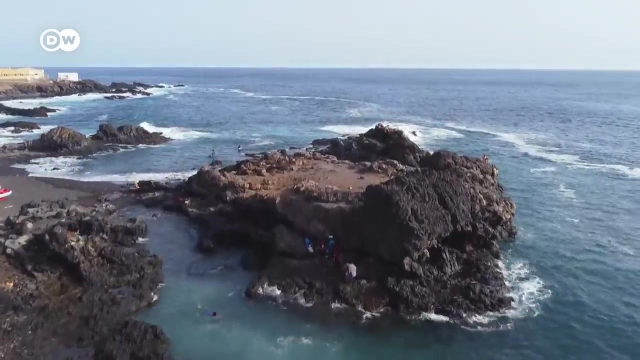 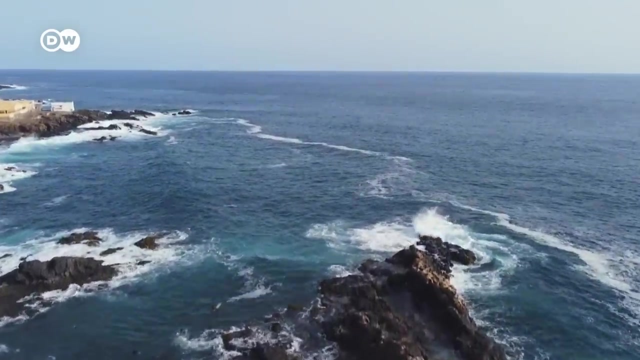 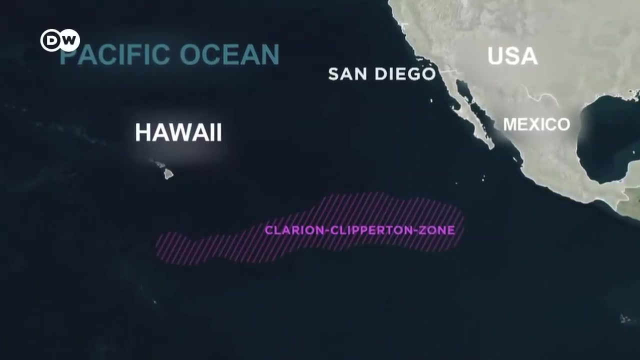 this passion for nature conservation. Small steps, but they make a difference. Jacques Cousteau would likely be happy to see these efforts to conserve marine wildlife. The Nets are the first to have a baby turtle in the wild. The Nets are the first to have a baby turtle. 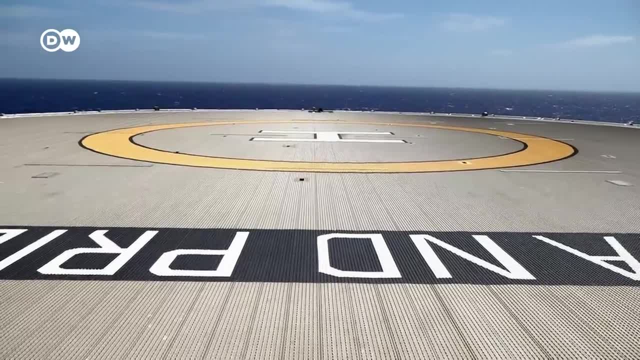 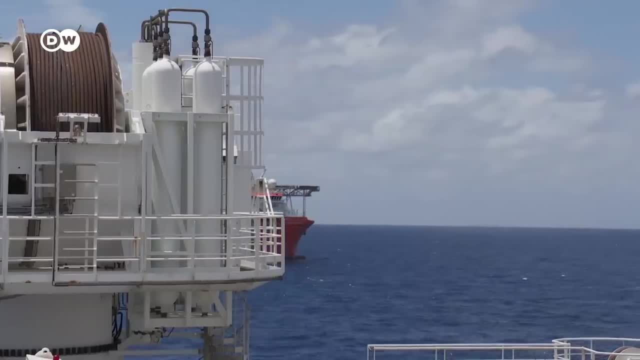 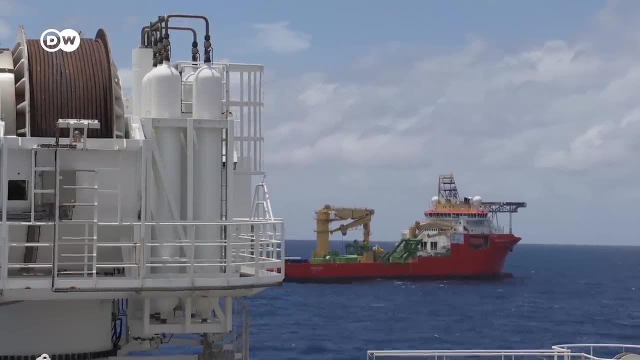 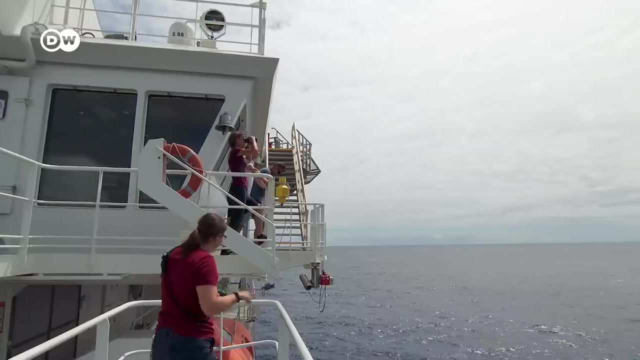 in the wild. The Nets are the first to have a baby turtle in the wild. Jacques Cousteau would probably have a child, only a three-month-old. try to get one baby, and the baby is standing right by the right lid and we can't. 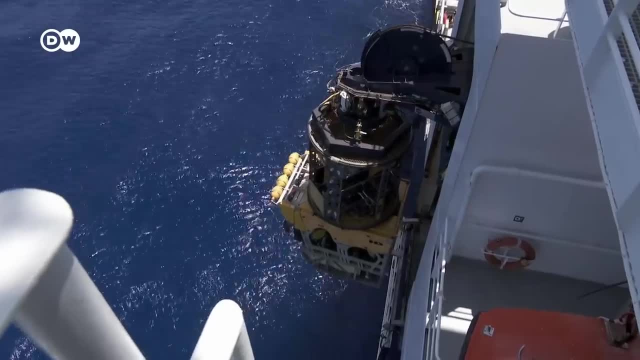 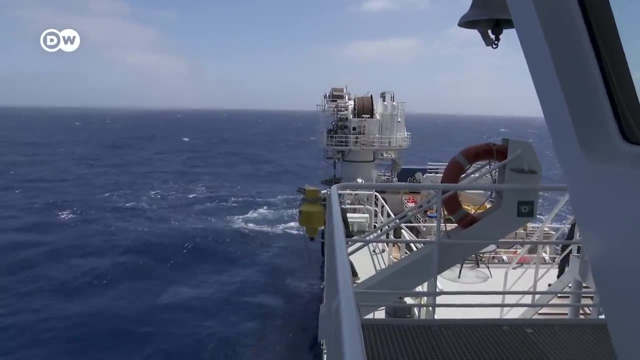 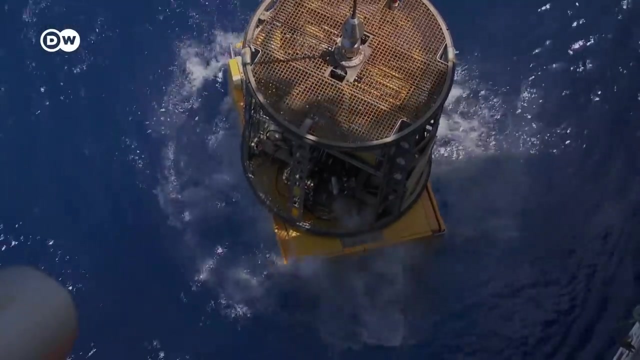 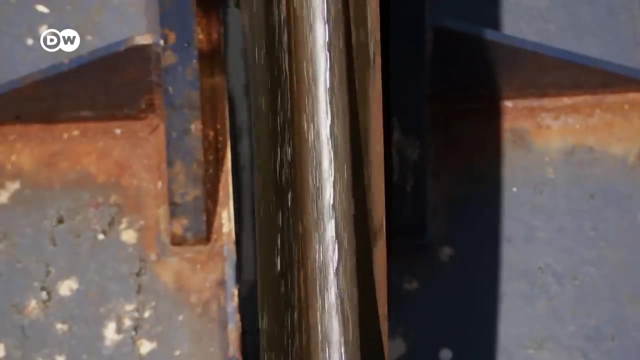 really tell slices on each part of the лет. Now the researchers' many measuring instruments and sensors and robots, known as ROVs, were coming into play. Lowered four and a half kilometres down into the depths. they were positioned around the deployment area on the seabed where Petania was making its way. 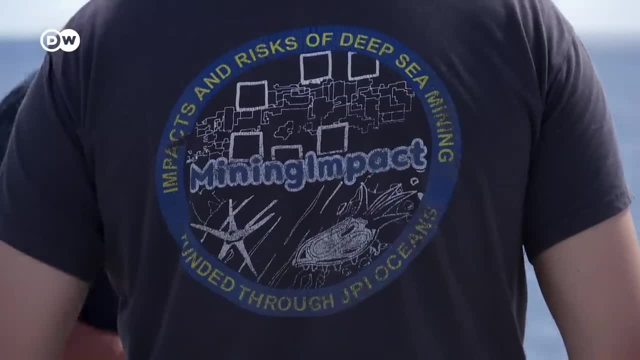 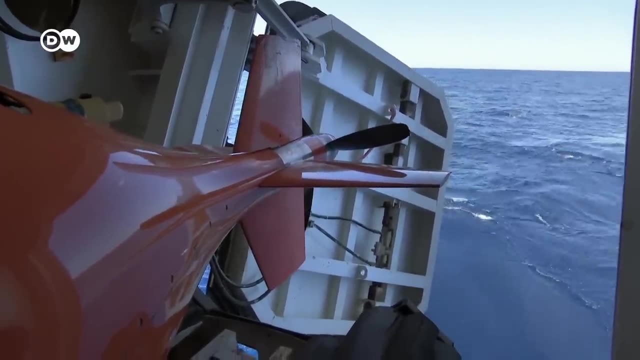 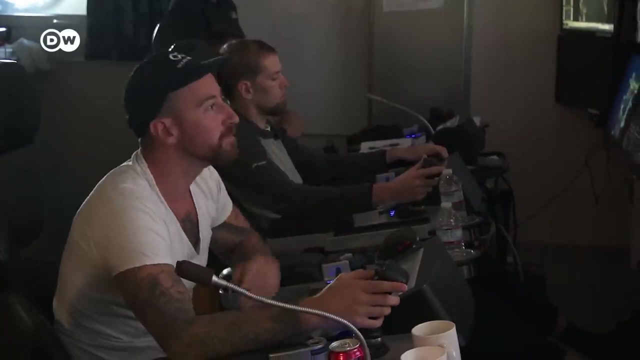 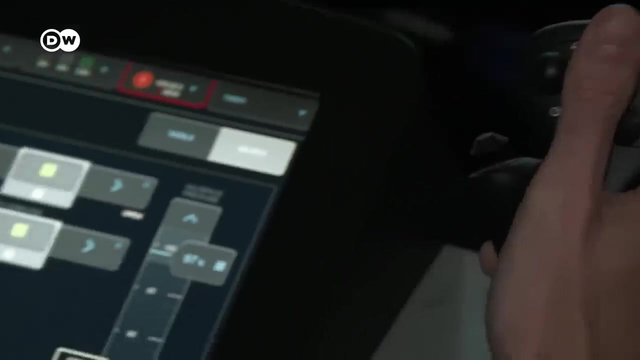 The scientists wanted to know the impact that Petania would have on nature. The control room is located on one of the lower decks of the island Pride. Here the pilots were sitting staring at their monitors for hours as they controlled the robots on the deep-sea floor. 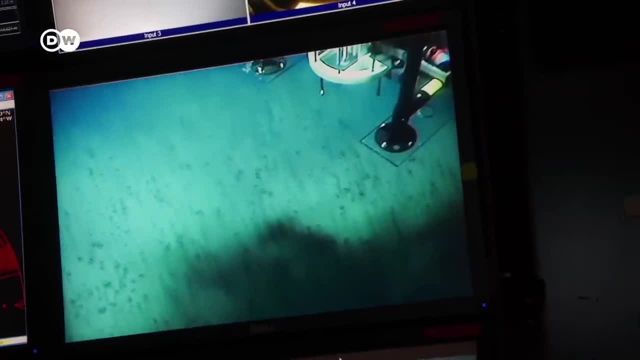 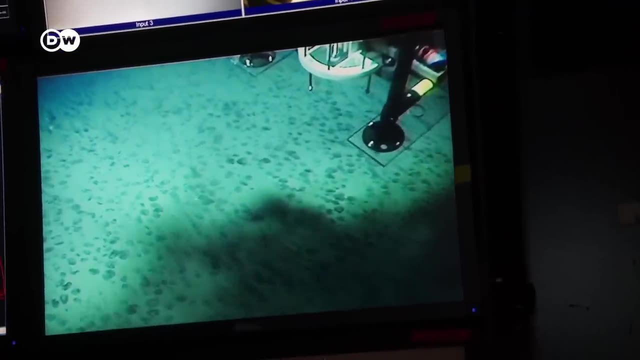 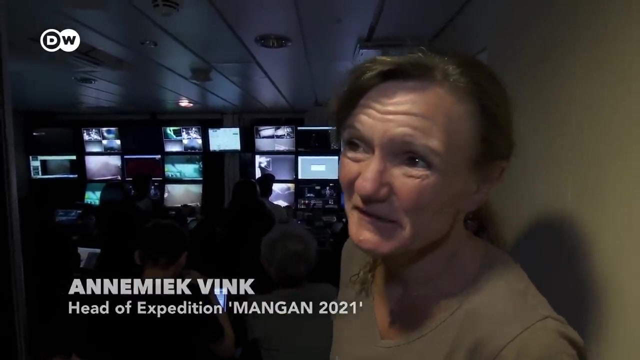 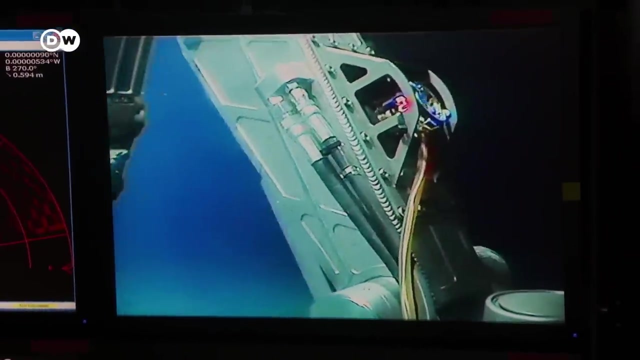 … There was an overwhelming feeling of being in a different world. Of course, it actually is a corner of the world that we barely know, And everything we're seeing here nobody else has seen before, So naturally that's always exciting. Scientific history was being made at that moment. 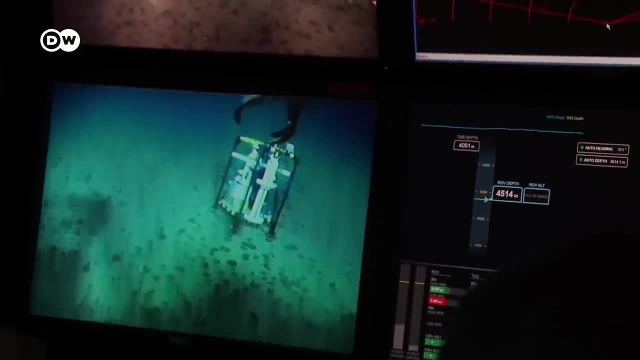 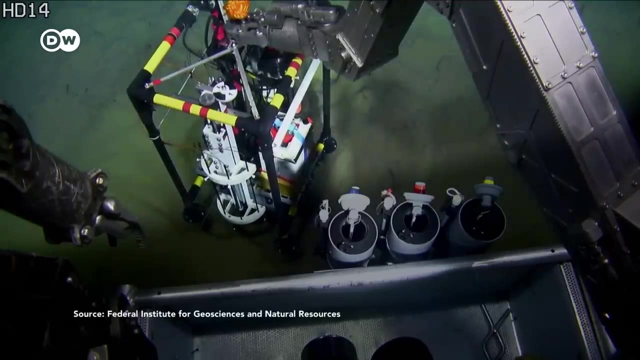 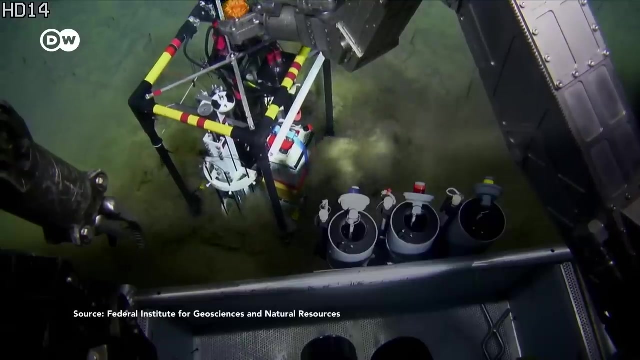 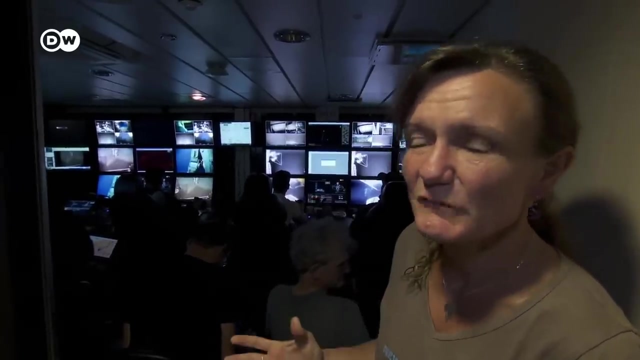 Four and a half thousand metres away. It's below the ship. Extremely important research was taking place under extreme conditions. We're now in the process of deploying many sensors- Oceanographic sensors, turbidity sensors and current sensors- on the seafloor. 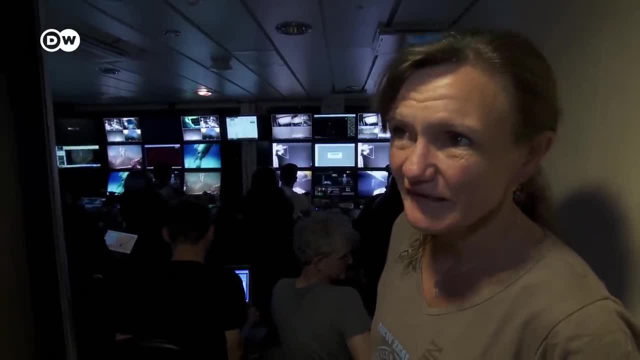 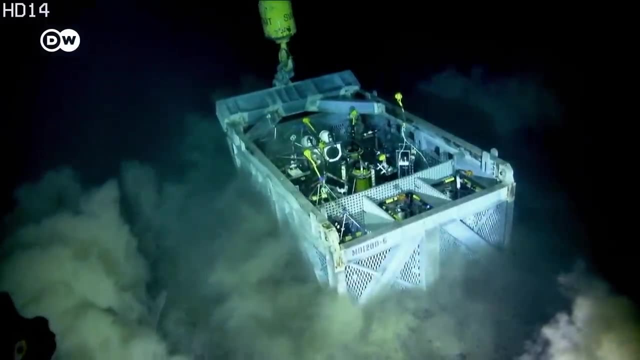 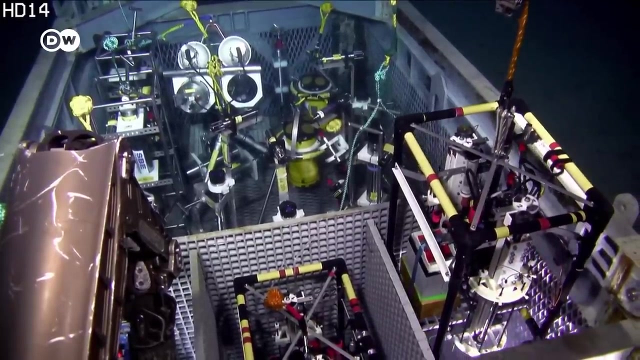 These were brought down in the huge sub-sea basket last night And they're now with the two ROVs, Or ROVs- Remotely-operated vehicles That are now moving along the seabed. The sensors are being taken out now and positioned along the seabed at various locations. 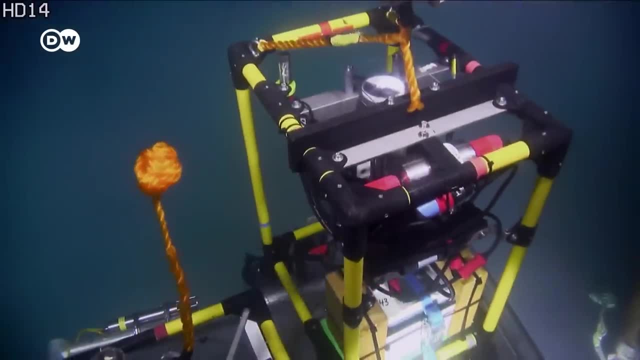 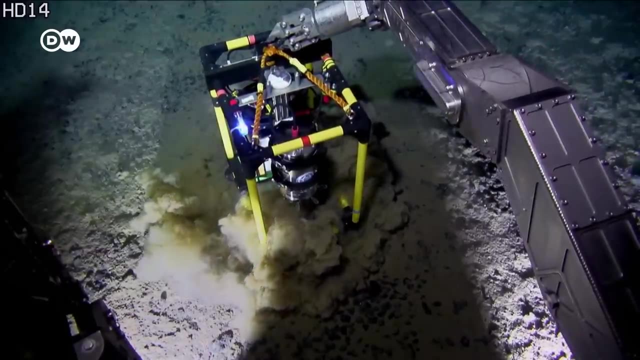 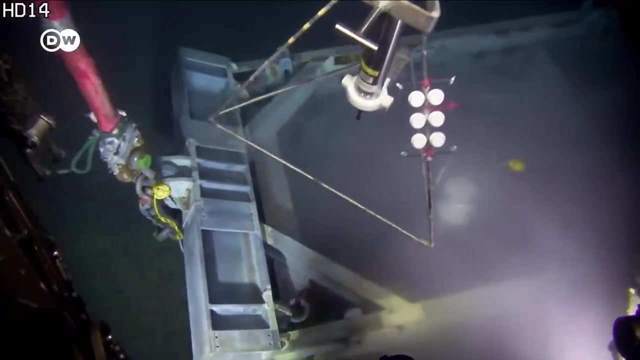 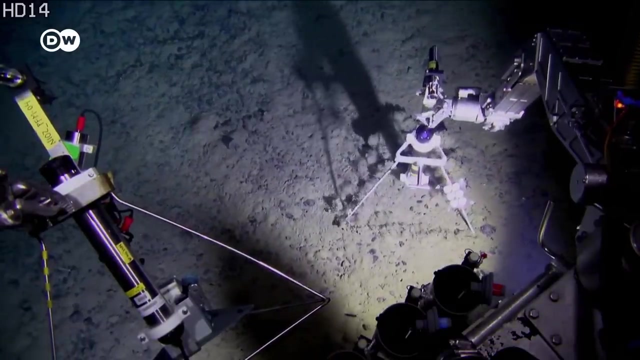 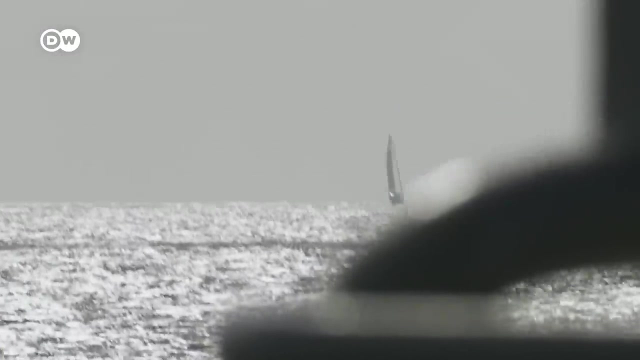 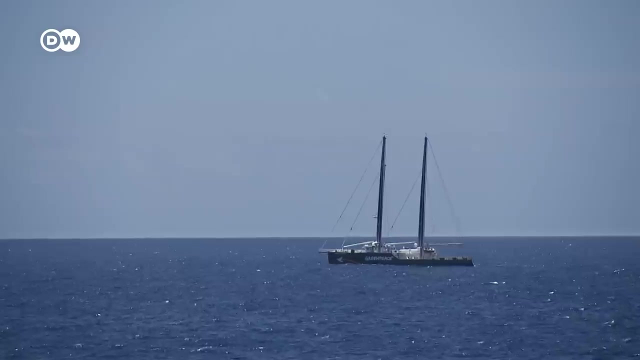 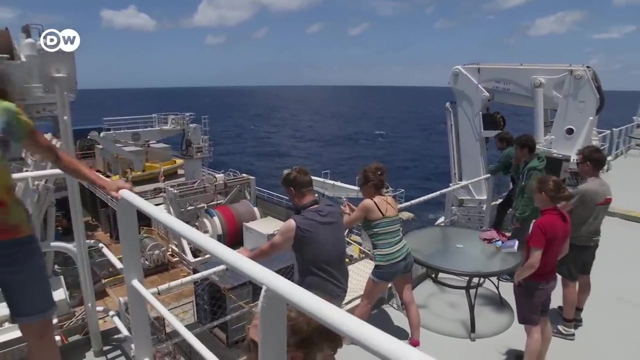 Hopefully, when Petania gets to work, they will measure the sediment cloud it creates as well. The sail has appeared on the horizon. Greenpeace's Rainbow Warrior was approaching the Norman energy. The scientists were slightly unnerved. Everyone was wondering what would happen. 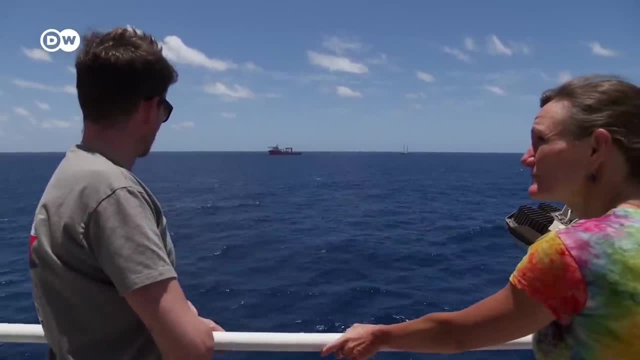 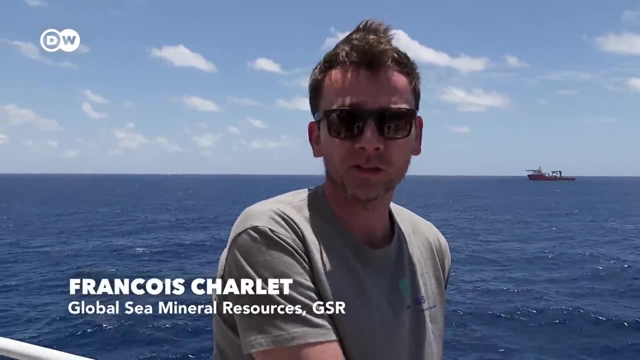 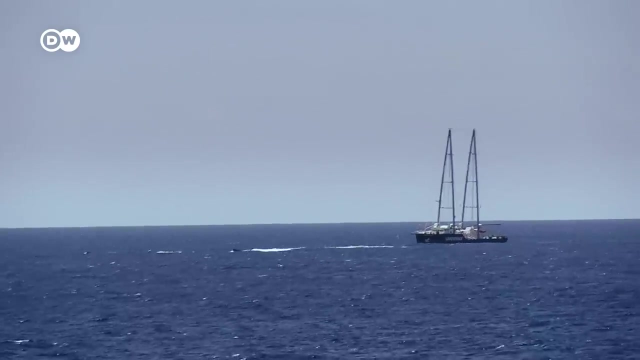 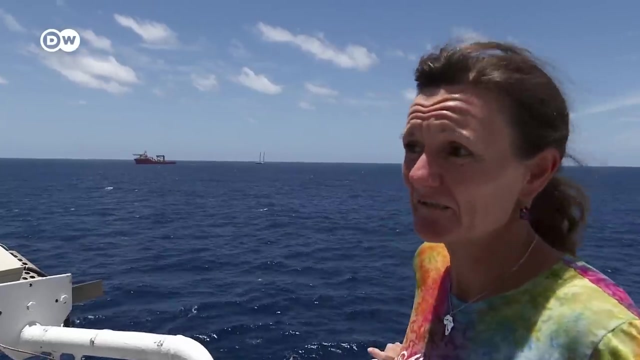 Do you have information? what is happening? Not that much, except to say that they make an action, so hopefully it's peaceful. We don't know. The only thing Greenpeace has emphasized is that it's peaceful, A peaceful program, A peaceful program. 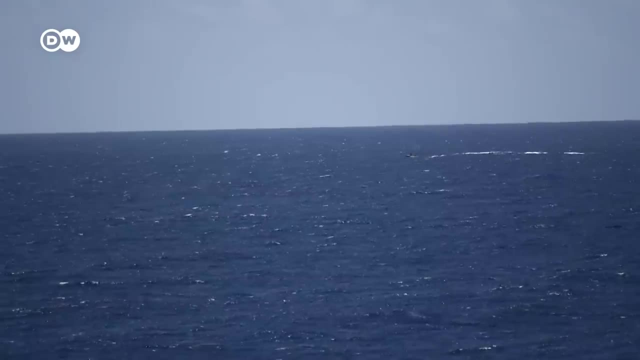 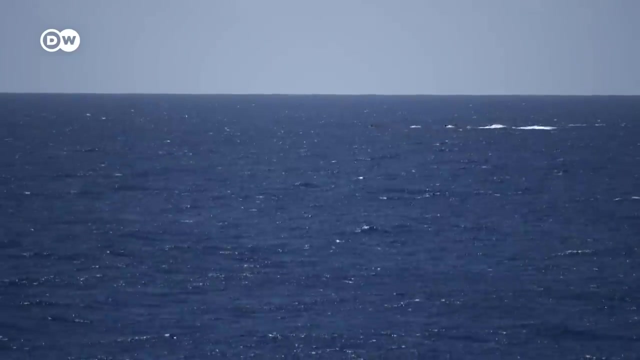 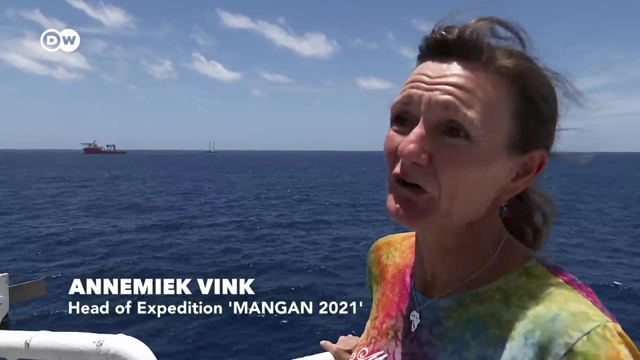 We can only hope that's what's going on. Obviously we're not the target, that's for sure. As soon as we moved away a little bit, they raced away. We don't know what they're doing. Something is happening on the starboard side and unfortunately we can't see it. 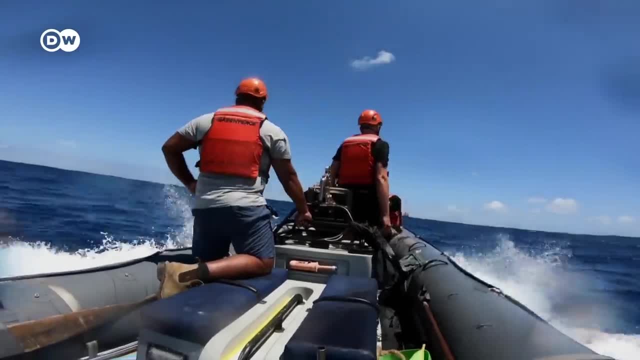 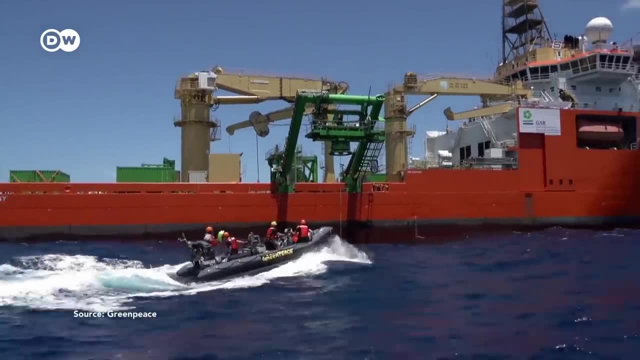 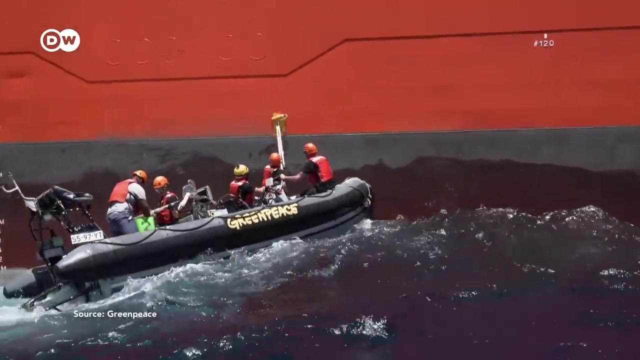 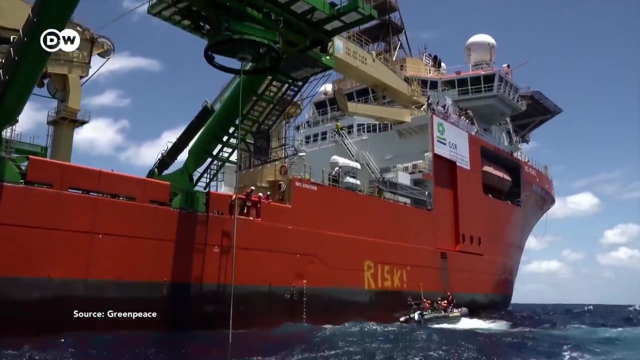 We can't do anything. I thought maybe that knows where it actually is. We're here to speak For us. of course it's spoke clearly of what's happening. It's saying something. The Greenpeace activists filmed and documented their actions themselves. 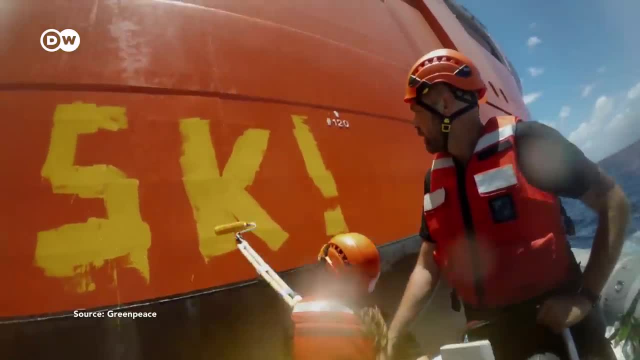 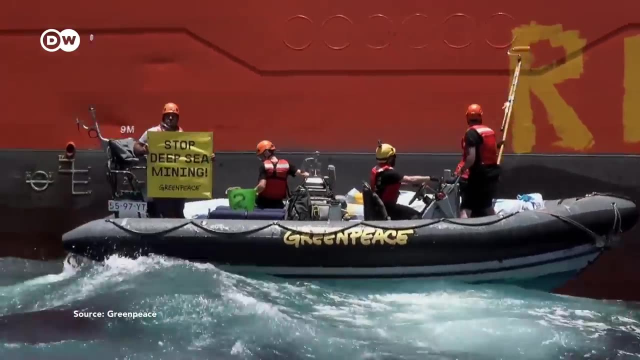 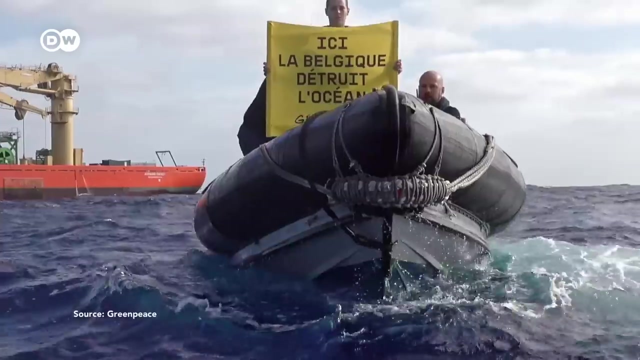 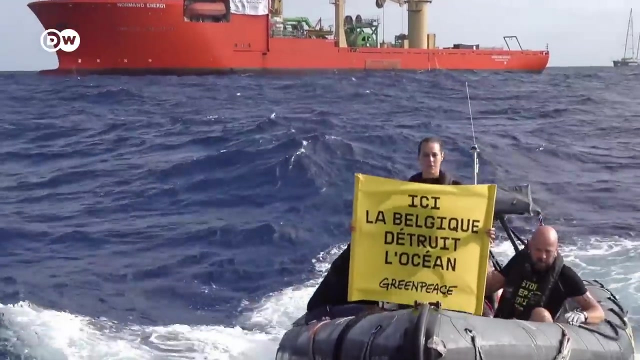 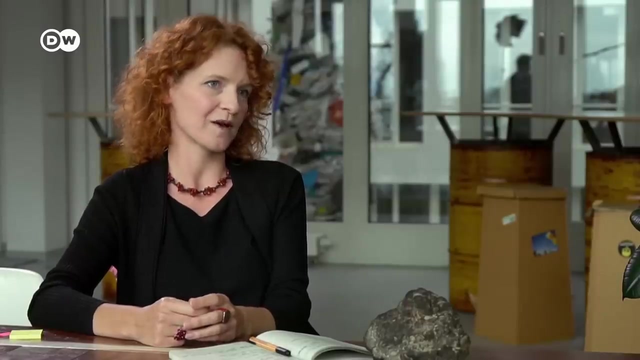 They approached the industrial ship and painted RISK on its side relies on striking images and messages in many languages to galvanise support. Greenpeace considers the commercial exploitation of the deep sea to be a fatal misstep. It would be an absolute crime to assume that the deep sea is a barren desert. 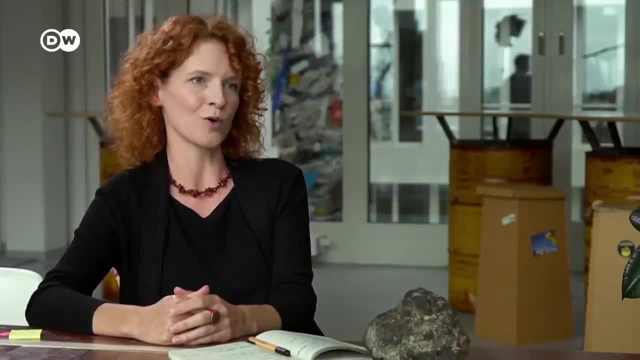 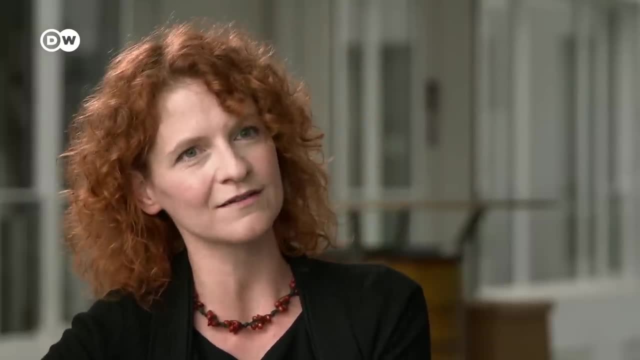 where you can do a bit of digging for manganese, nodules and other ores without having any impact on this planet. That's what people would like to tell you, And I don't think the general public would like that. The general public is aware that the deep sea is teeming with life. 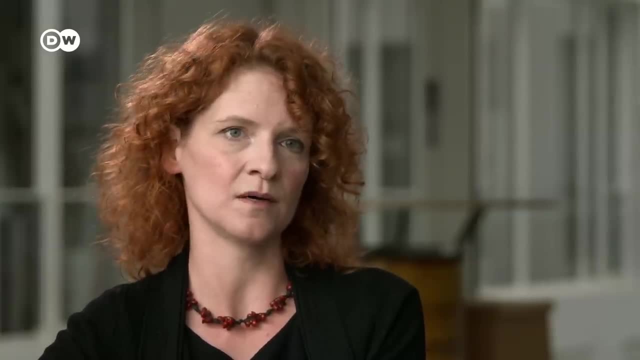 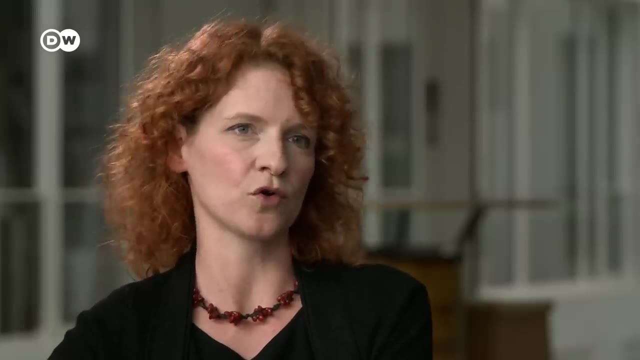 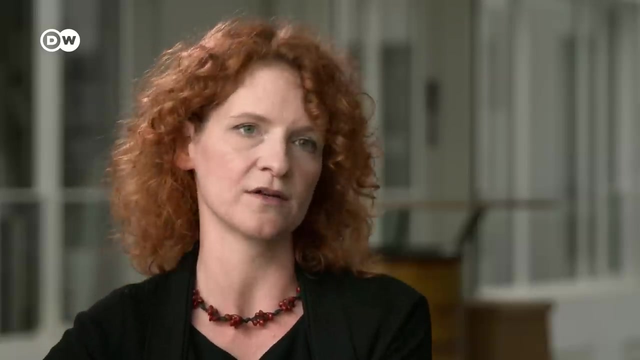 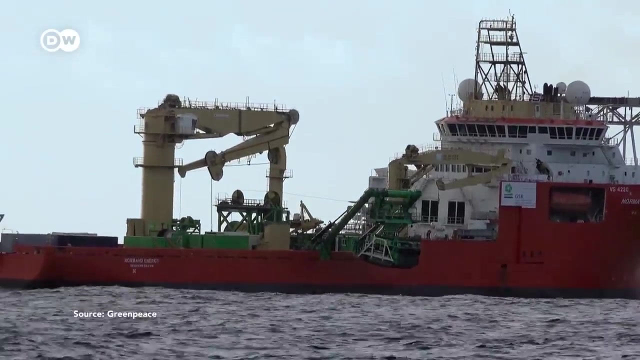 The companies involved in deep sea mining aren't necessarily interested in revealing the damage that's taking place down there, including in the long term, and which animals, and ultimately, plants, such as plankton, are being affected. It's already been proven that CO2 has been bound in the sediments. 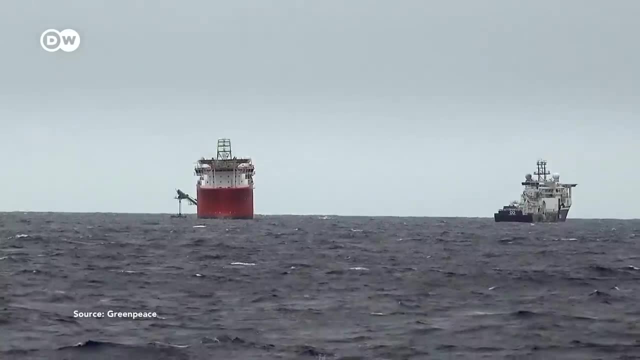 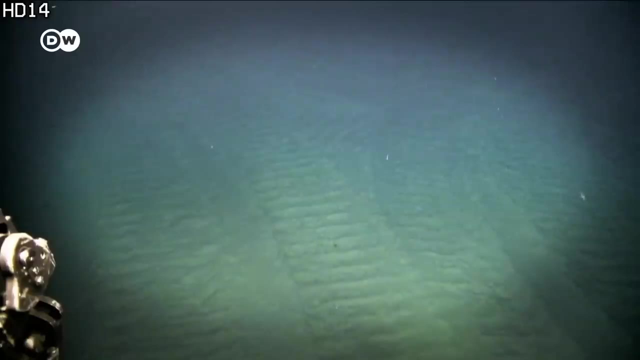 deposited on the deep sea. That means carbon that originally came from the atmosphere. If we disturb and stir up these sediments, then there is definitely a risk that this CO2, this carbon that is currently sequestered down there, could also be released back into the water and ultimately into the atmosphere. 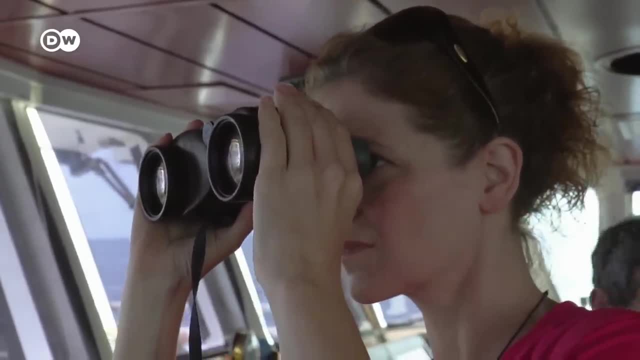 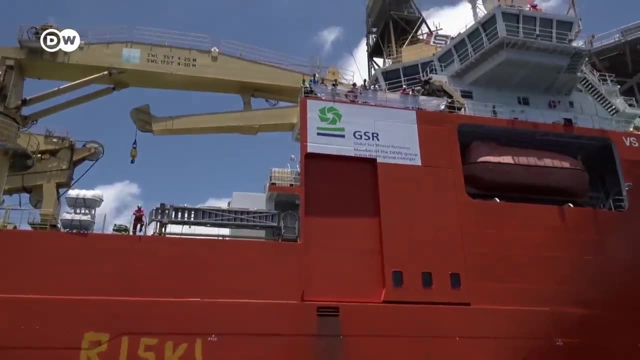 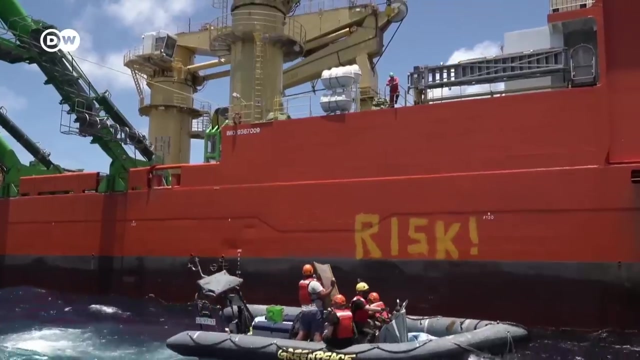 Greenpeace's Rainbow Warrior tracked the Normand energy for weeks with the aim of producing images to generate support. Let's make the point right now: We want to make sure the oceans continue to have the possibility in the next years, the next millennia, to be climate resilient. 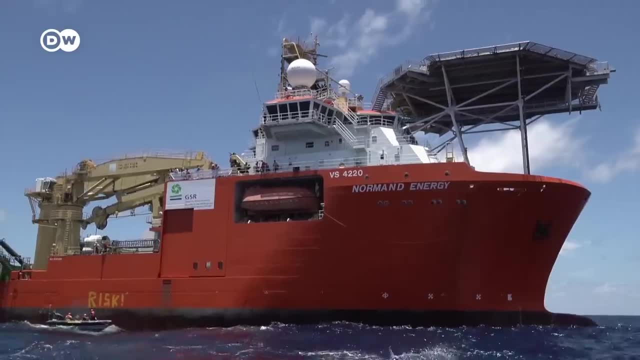 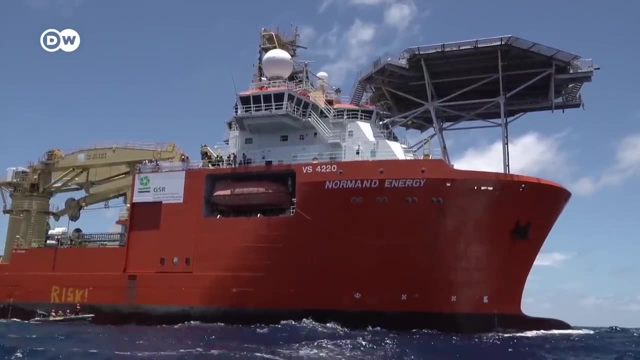 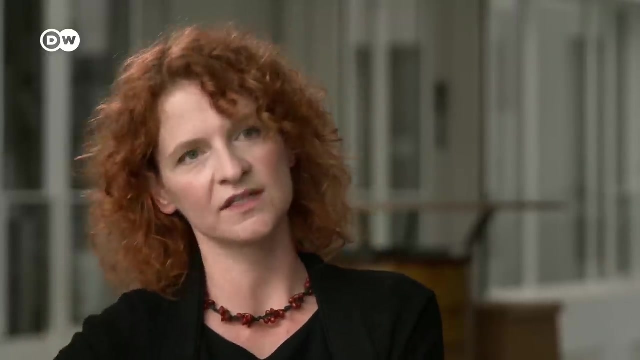 Something they can't be if we start digging and destroying the deep sea floor, Not just taking out rocks, ores and metals, but also the biology, the life forms, and destroying their habitat, Because all of this is involved in the climate stability of our oceans and our planet. 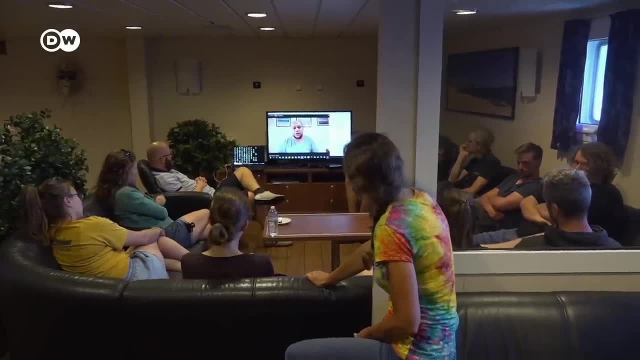 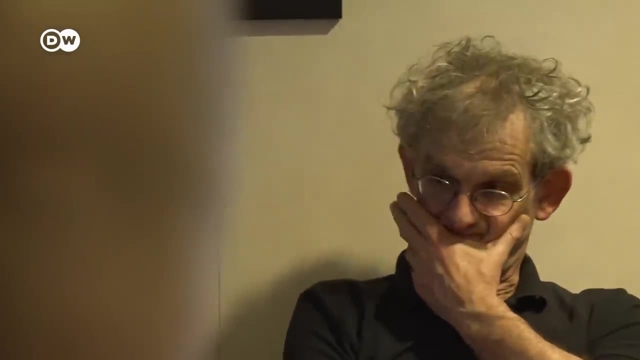 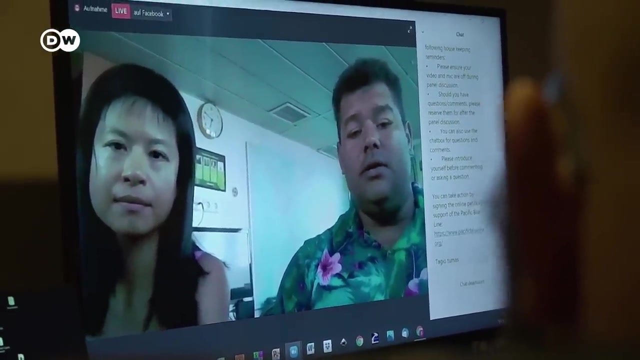 A meeting was held in the conference room on the island Pride. The occasion Greenpeace had issued an invitation to a worldwide international video conference. The NGO's objective was to prevent possible deep sea mining. It reported on its concerns, giving arguments why disrupting the depths must be stopped at all costs. 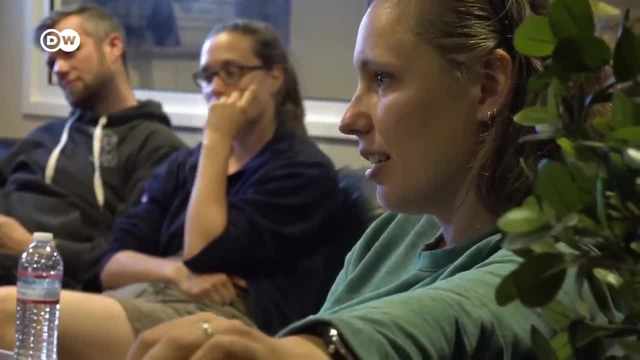 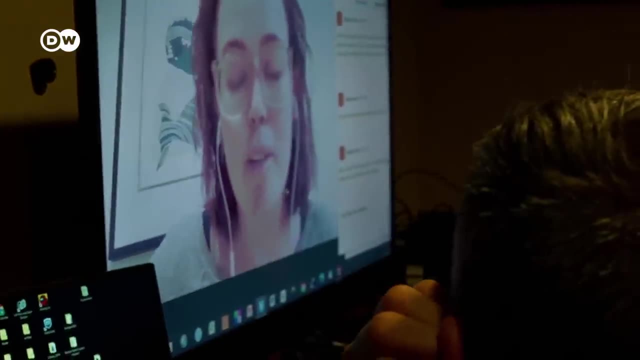 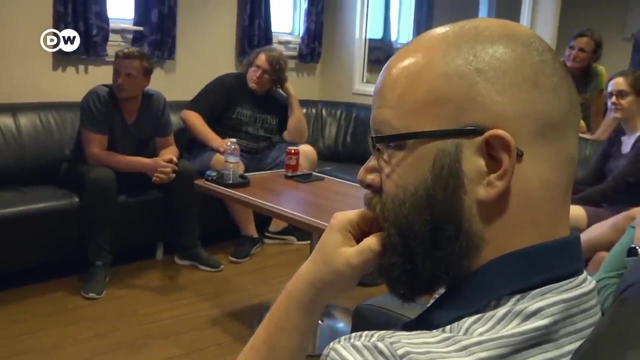 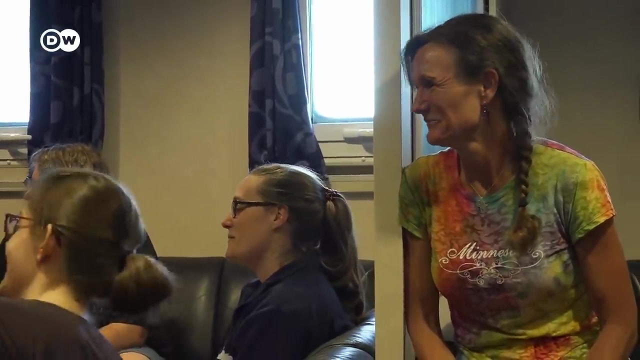 before it really gets underway. They also took a swipe at the scientists who were then researching the effects such an intervention would have. Greenpeace said it wasn't genuine science. The best science that is being done is the right science. That outraged the scientists. 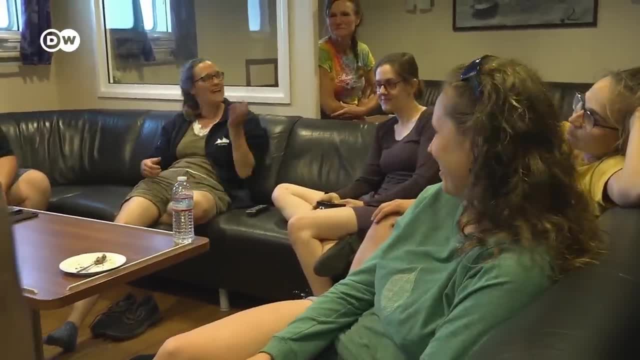 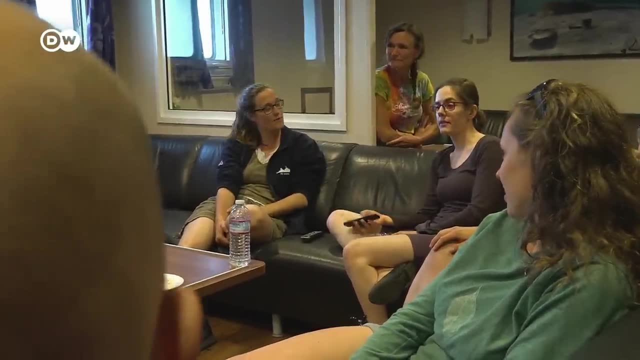 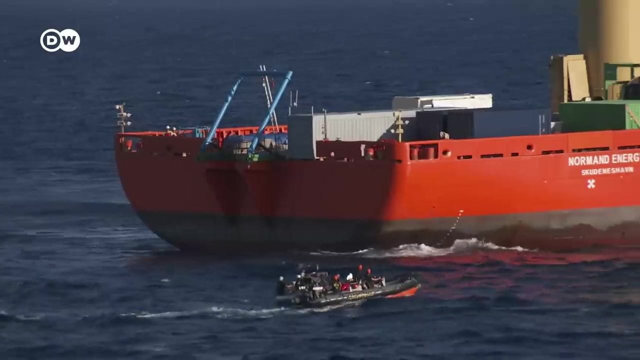 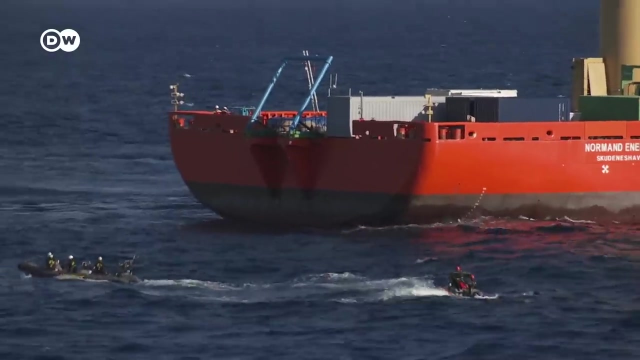 They said they would continue to carry out neutral research in order to ultimately provide data and findings that are also used by environmental protection organisations. No, but he's a real scientist and he worked on that stuff, and so, OK, Some of the researchers showed understanding for the protest on the high seas. 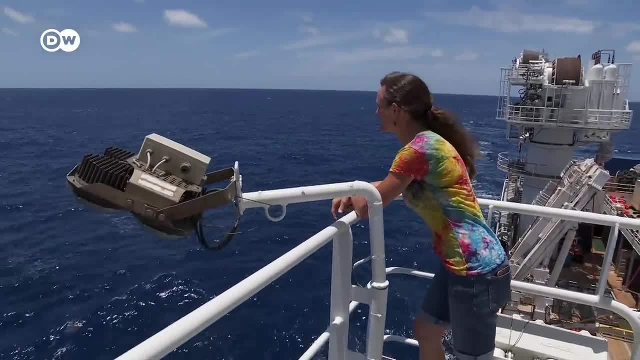 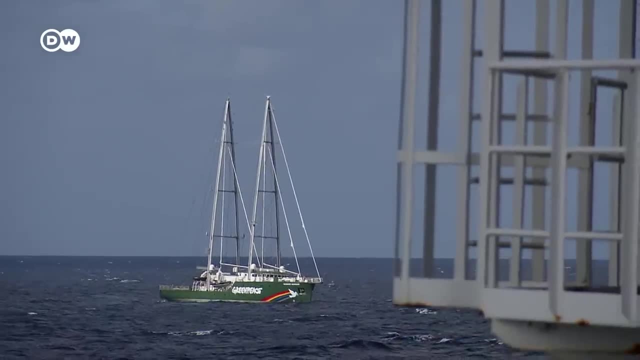 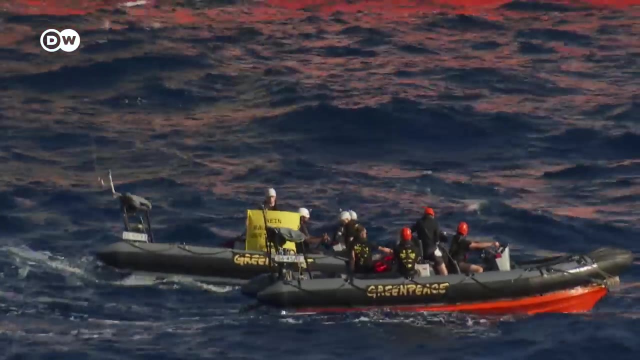 and the concerns of the environmental protection organisation. This is a very sensitive issue and everyone has the right to be concerned and also to protest. Of course, we all try to be very neutral in our analysis, and that's certainly correct, But there's always the question of what the science is used for. 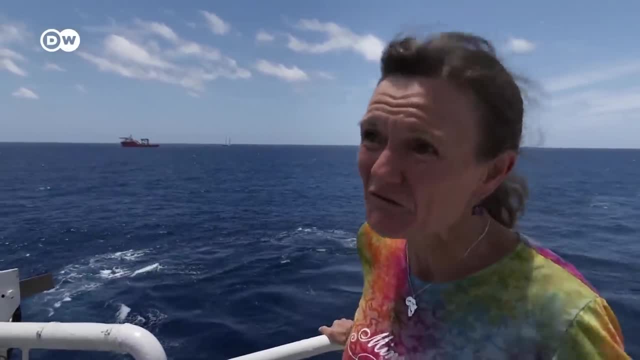 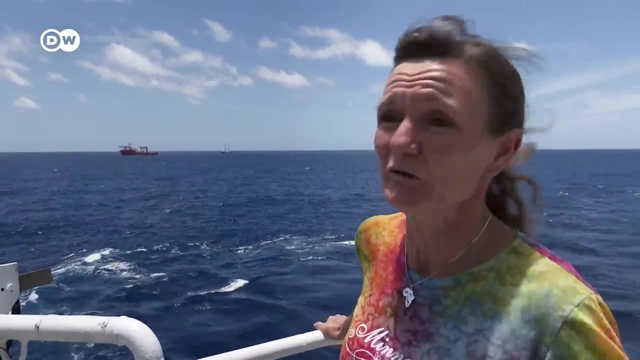 Deciding that isn't our job. That will be done by the policymakers who will have to develop the regulations. What we're trying to do here is record what could potentially happen if a device like that were to drive around on the seafloor. 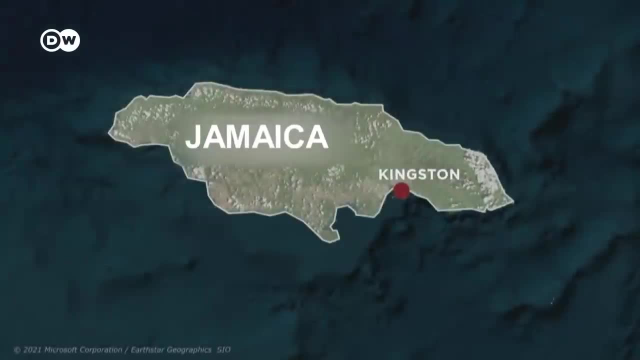 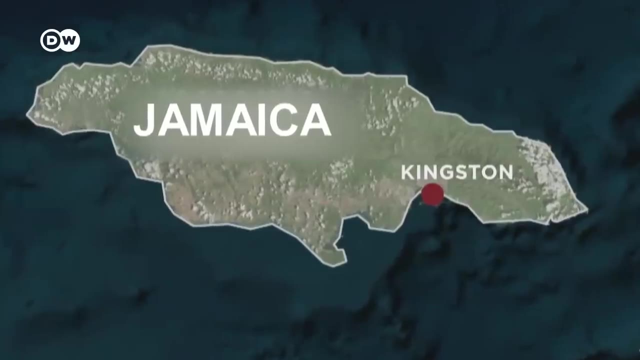 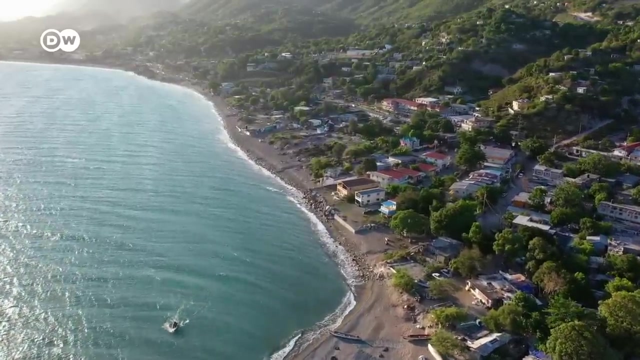 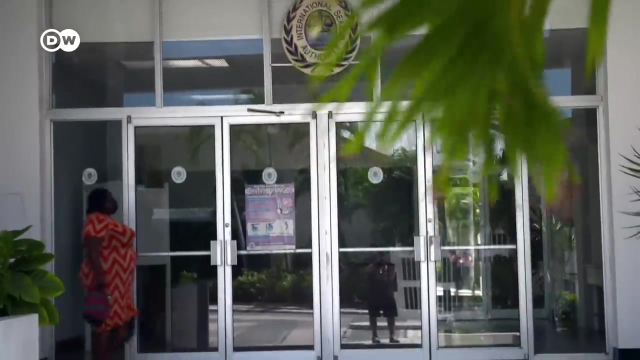 Located in the middle of the Caribbean Sea, the island country Jamaica is home to the institution that will decide whether deep-sea mining is permissible. The International Seabed Authority, or ISA for short, has its headquarters here, Founded in 1994 by the United Nations. 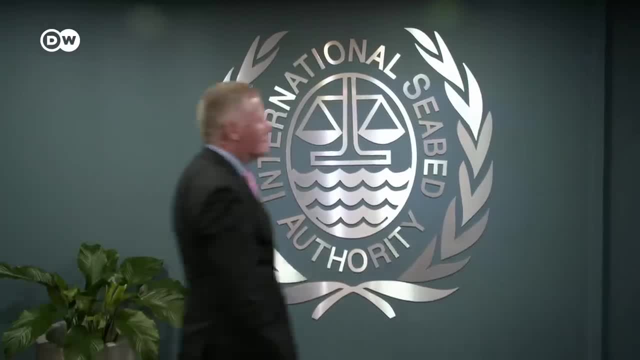 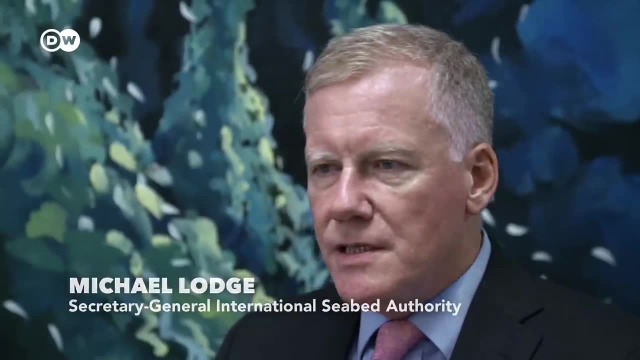 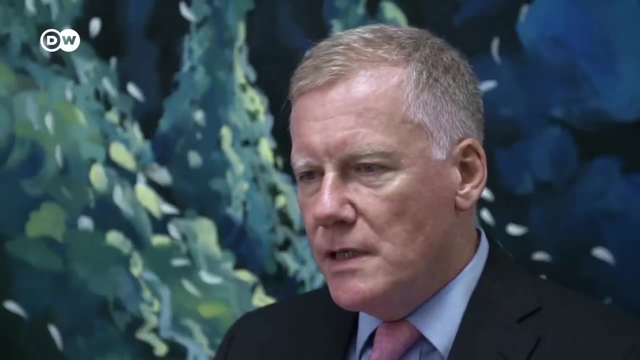 it's the overarching body that decides what happens beneath the waves. So all the ISA contractors, which are a combination of different entities- some are governments, some are private sector, some are state research organisations- all of them have in view, eventually, the sustainable exploitation of deep-sea mineral resources. 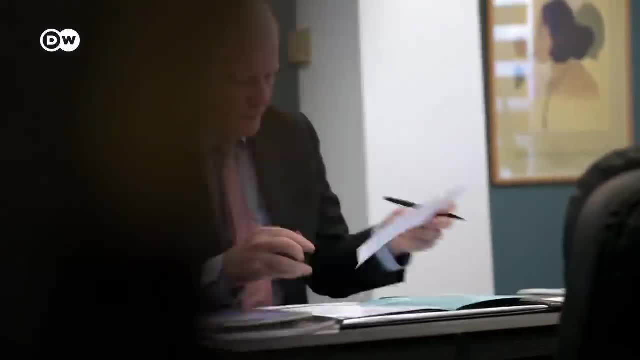 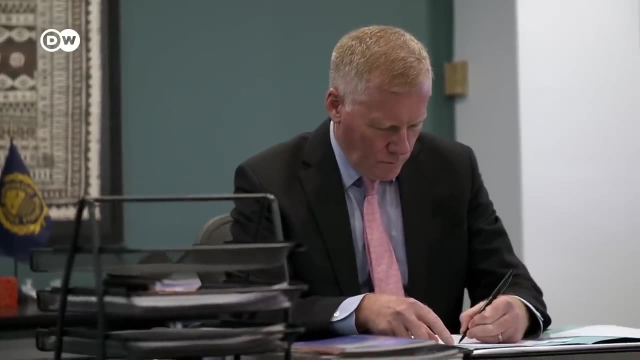 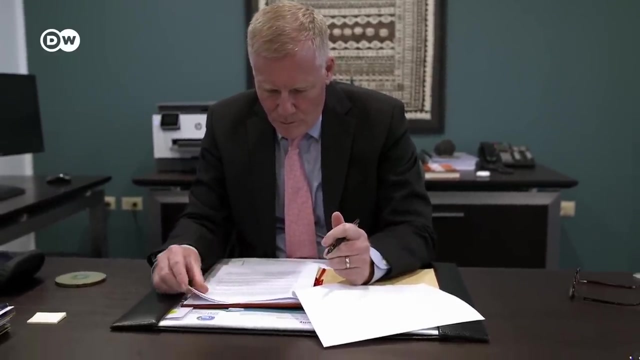 ISA must proceed on the basis of two fundamental conditions: One is that we act on the basis of the best available scientific advice, through extensive consultation, and the other is that we act on the basis of the best available scientific advice through extensive consultation, and the second is that we act on the basis of consensus. 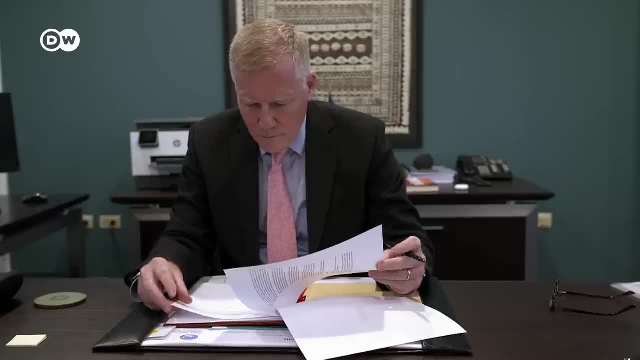 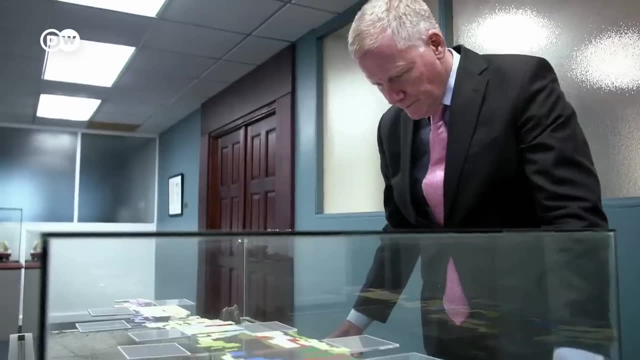 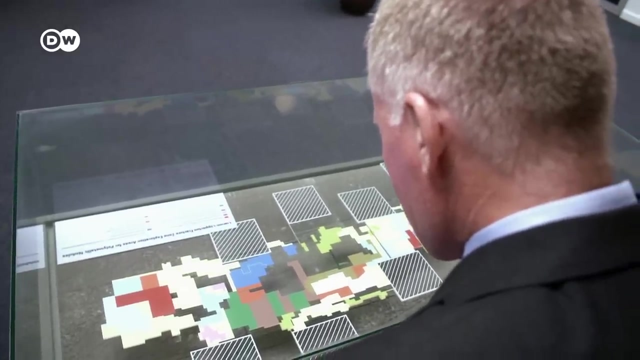 amongst the member states that make the decisions- That's currently 167 countries, including Germany. They develop the guidelines, known as the Mining Code, according to which deep-sea mining would be possible. We have a very unique opportunity here that actually has never been done before. 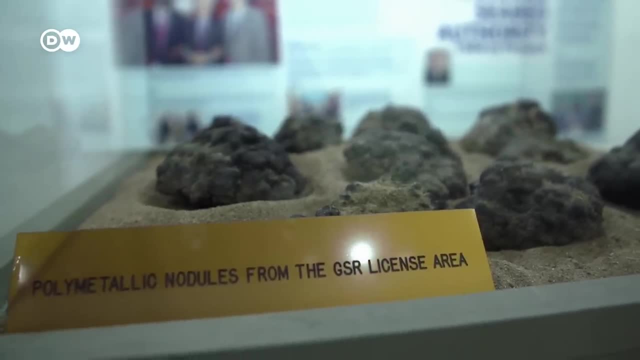 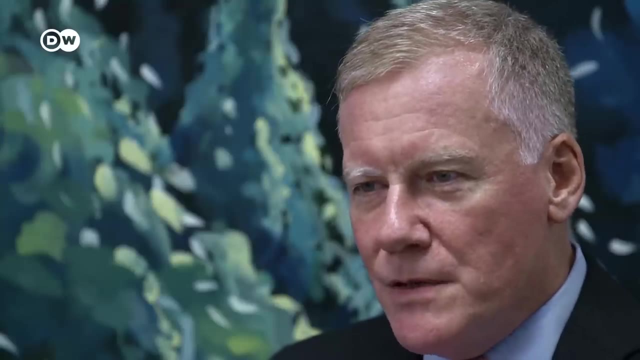 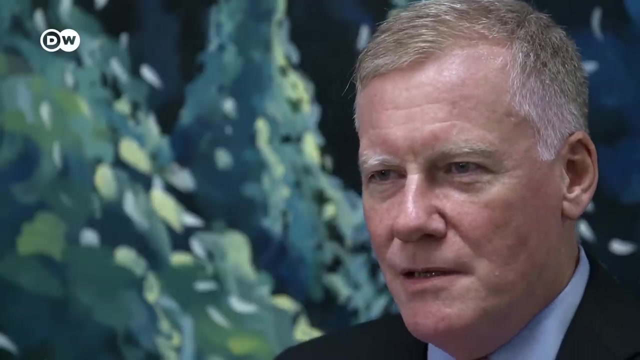 which is that we have a whole new industry that will proceed only when regulations have been put in place. Usually it's the other way around: Industry starts and then people start to react by trying to find a way to regulate it or to stop bad things from happening. 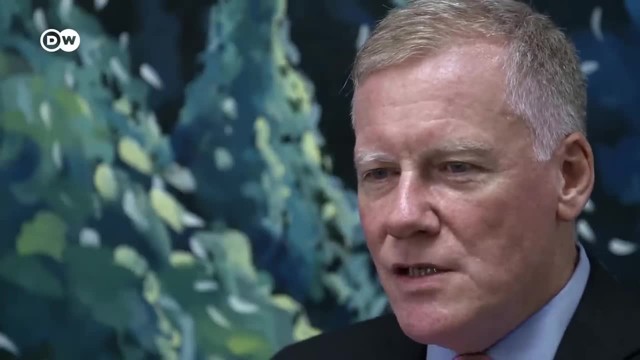 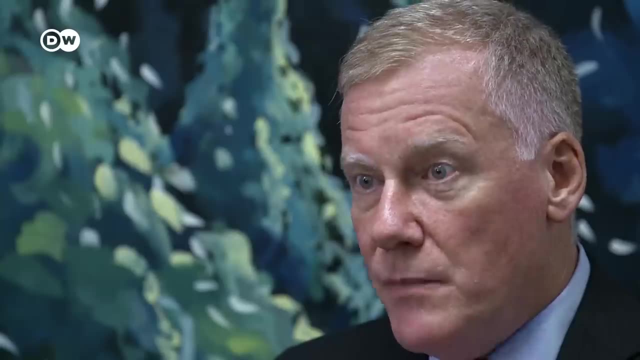 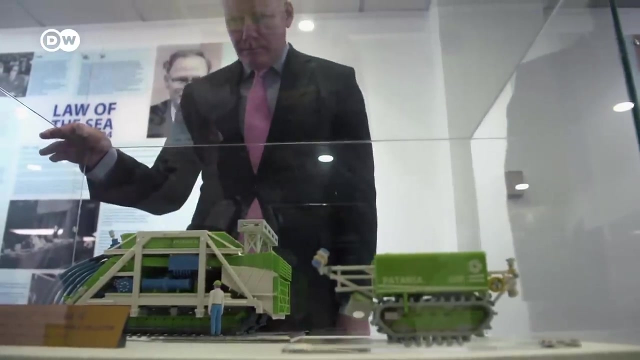 or to ensure that good things happen. Here it's completely the other way around. We have an opportunity to get it right before we even start, which is unprecedented. It's a really great opportunity. So really, it's a very highly transparent organisation. 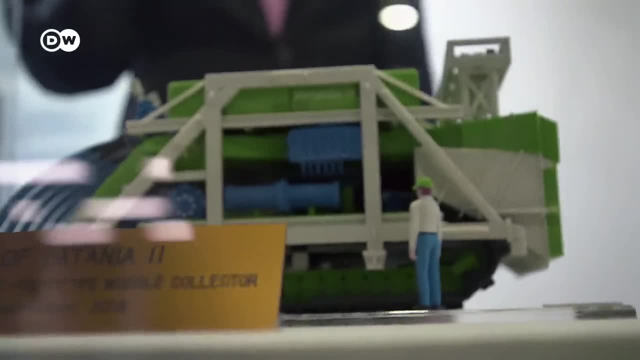 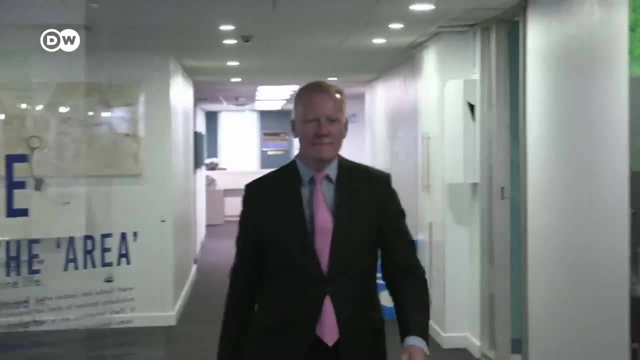 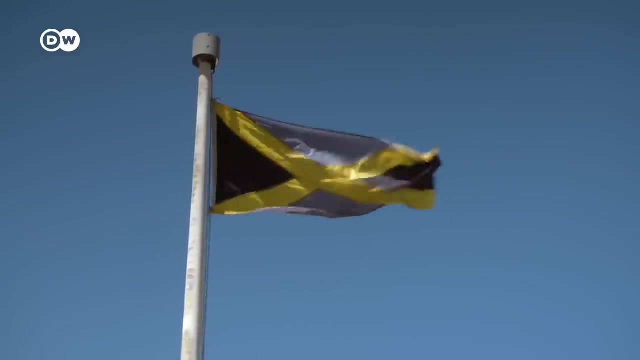 where everybody has an opportunity to have their say and provide input into this emerging new industry. So this is where the decision is to be made, Taking into account the interests of industry, the findings of science and the concerns of environmental protection organisations. Nature conservation versus a billion-dollar business. 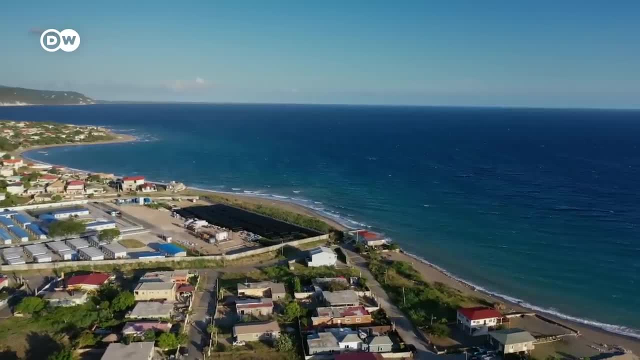 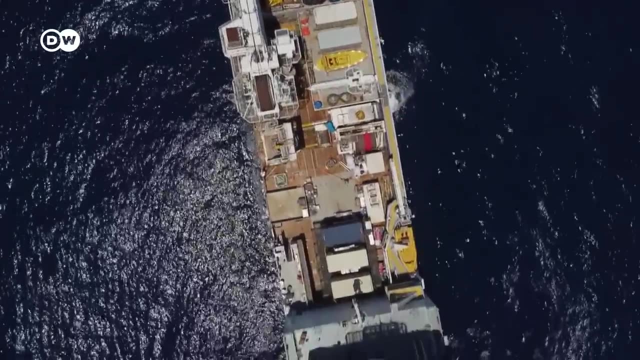 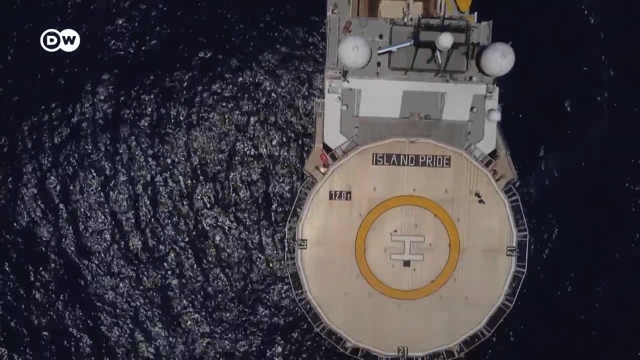 Who'll win in the end. The Island Pride was sent out to work in the Clarion-Clipperton zone. It's an area the size of Europe. More than 30 billion tonnes of manganese nodules are said to lie on the ocean floor here. 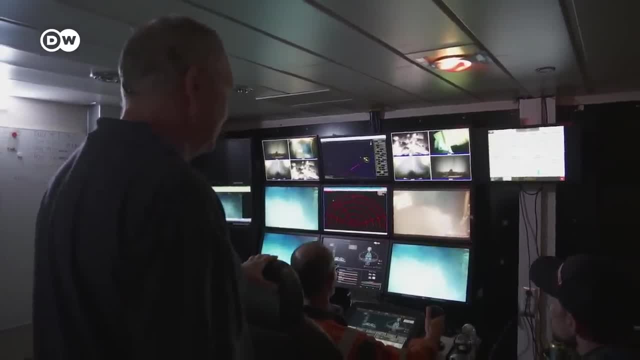 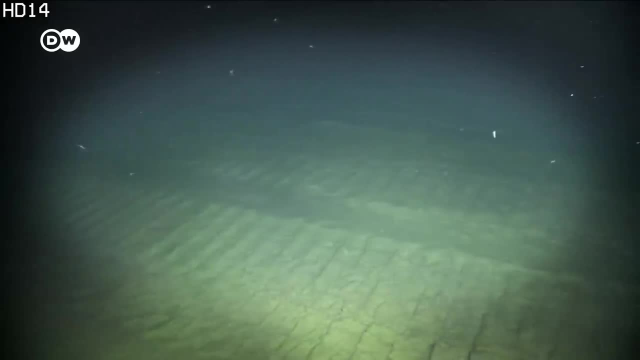 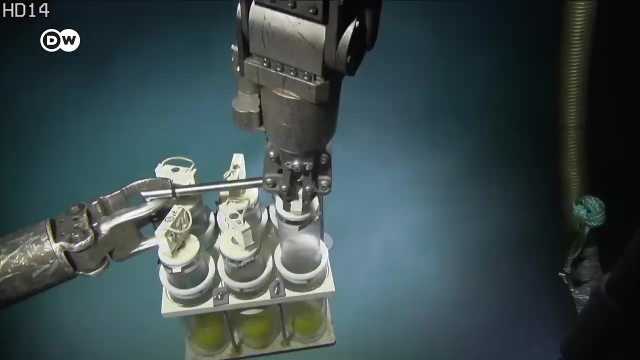 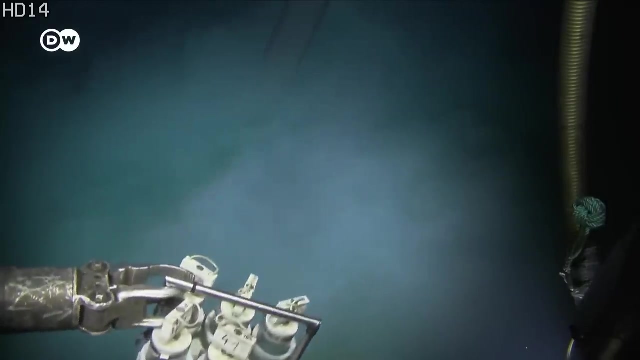 It's an enormous treasure and there is no way retrieving it will happen without disturbing the deep sea floor. These are the results of Pétania's work. The heavy machine has stirred up large plumes of sediment. What does this mean for the environment? 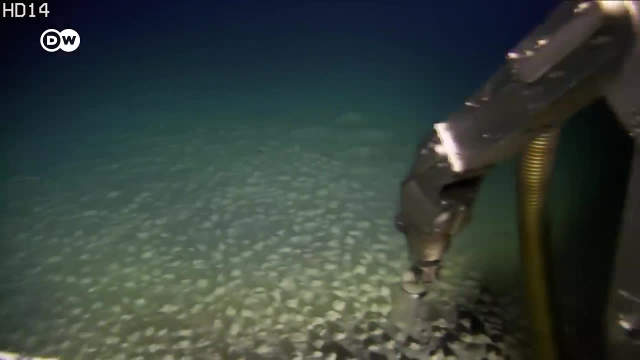 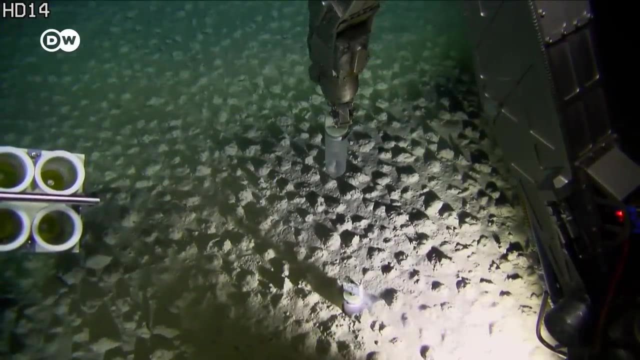 Yes, the one we see here is the manganese nodule habitat next to the tracts of Pétania, where the disturbed sediment has already settled. It's completely covered the manganese nodules and fauna, And what we want to find out now is at what thickness the sediment does negative, permanent damage. 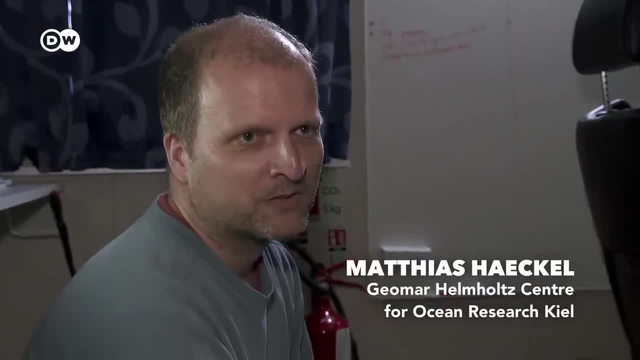 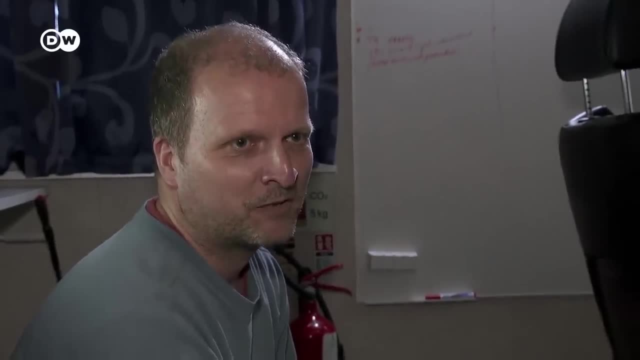 and what thickness the fauna can possibly tolerate. And what we want to find out now is at what thickness the sediment does negative permanent damage and what thickness the fauna can possibly tolerate. and what thickness the sediment does negative permanent damage and what thickness the sediment can possibly tolerate. 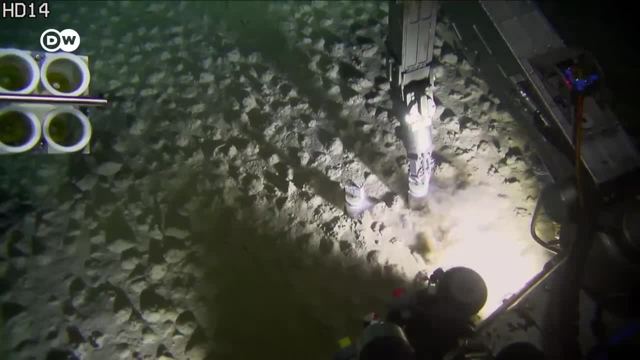 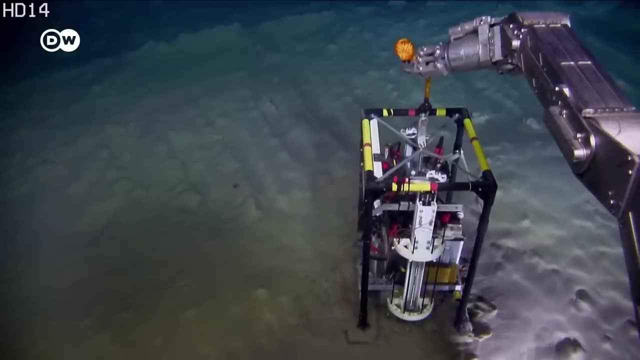 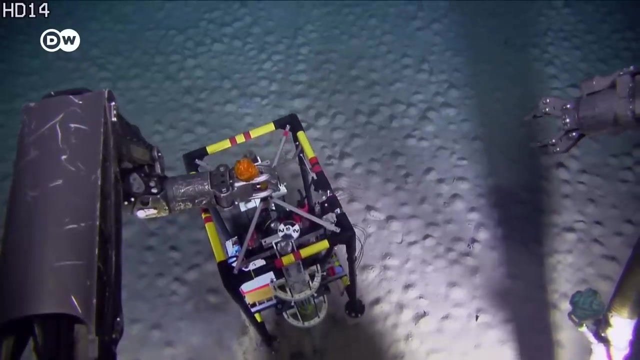 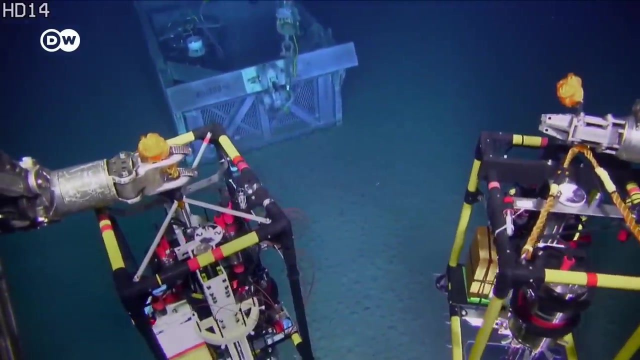 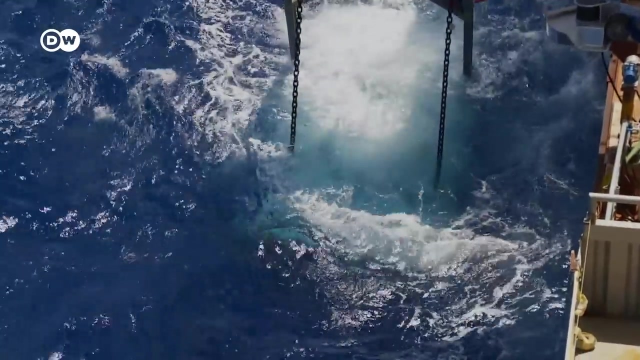 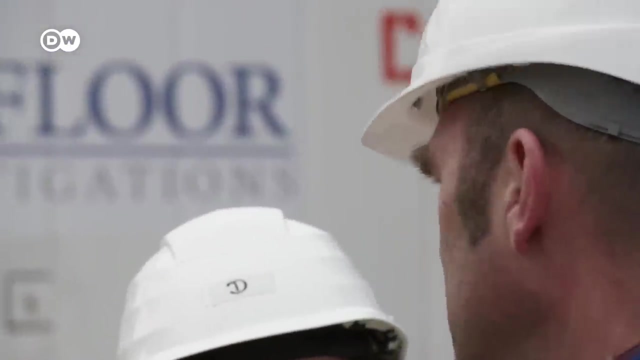 It looks as if a snowstorm had passed over the landscape and covered everything in its way. The measuring devices then needed to be brought up to deck for evaluation, a process that took many hours for evaluation- a process that took many hours. The researchers were eager to see what had been brought up. 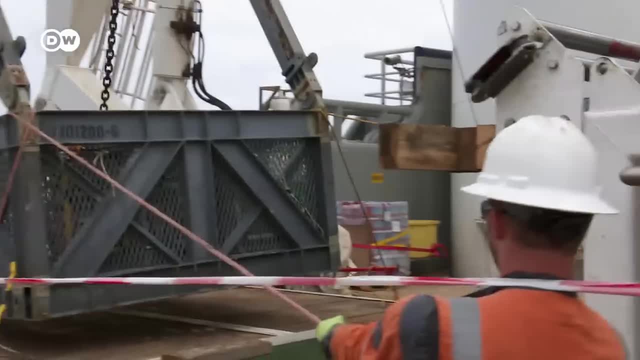 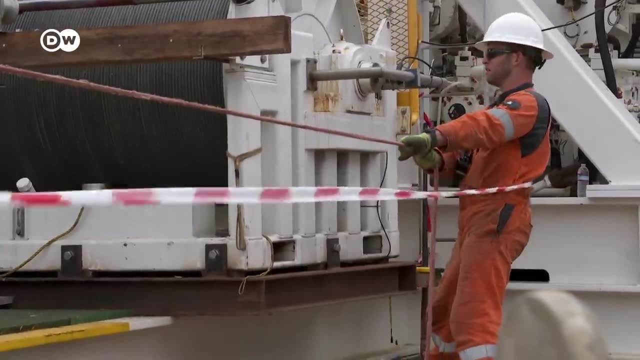 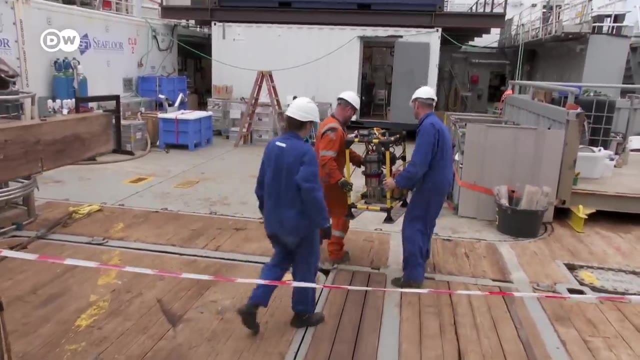 Even though the results of the analyses would likely remain unknown for months, until they were fully assessed in the laboratories of the institutes in Europe. First we've got to rinse them, because salt water is very corrosive to the electrical components. Then we'll download the data and take a look. 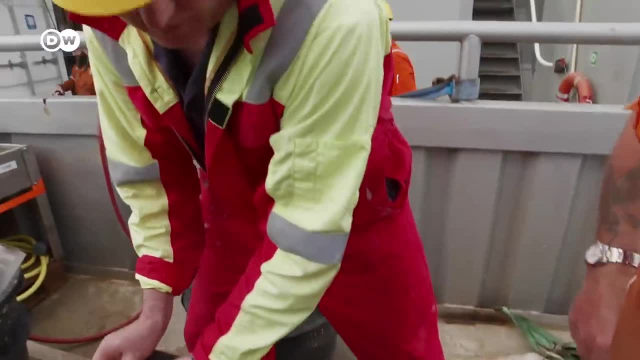 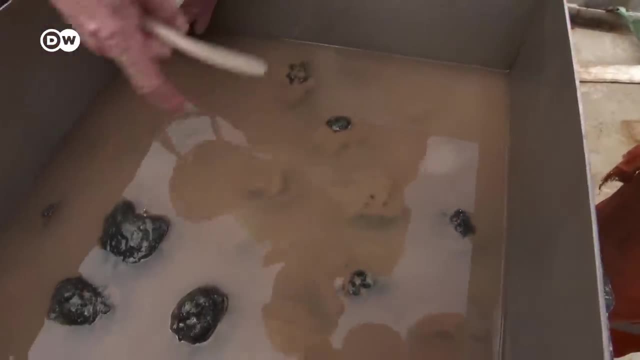 These are the manganese nodules and you can see that they were actually covered with deposited sediment. But because the water is now sloshing back and forth here, the sediment just washes away. But it doesn't matter, because we have to free the nodules from the sediment anyway. 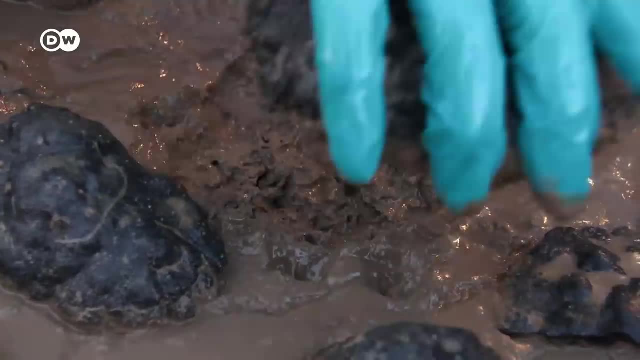 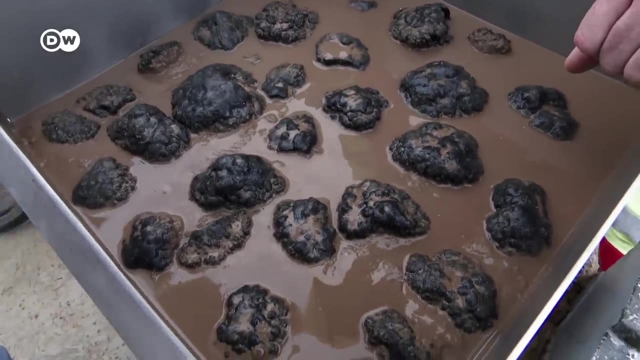 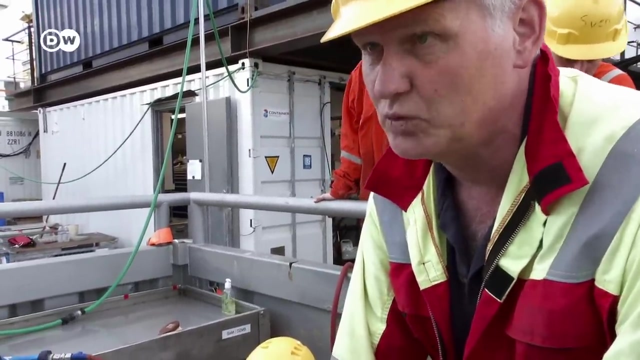 in order to collect the sediment, In order to collect the animals that live on them. You see, when you cut the manganese nodule open, there's a core material around which it forms. The nodule is made up of metal oxides, manganese oxides. 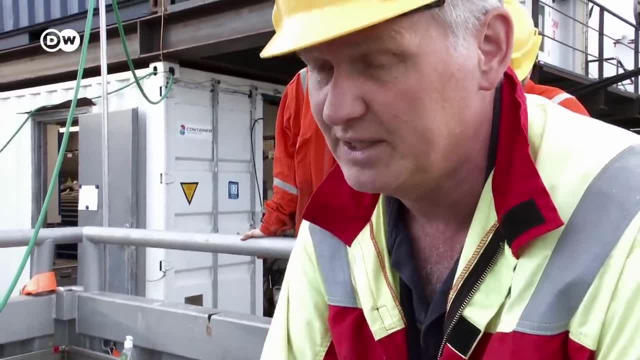 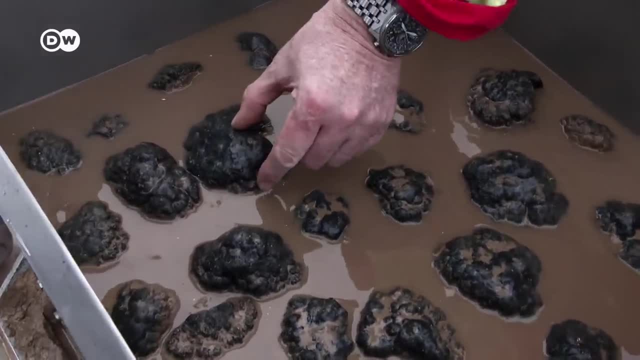 and then there's copper and nickel and cobalt in it, as well as traces of other metals, And that slowly builds up around the core material That is. such a nodule with a radius of around four centimetres would be close to two million years old. 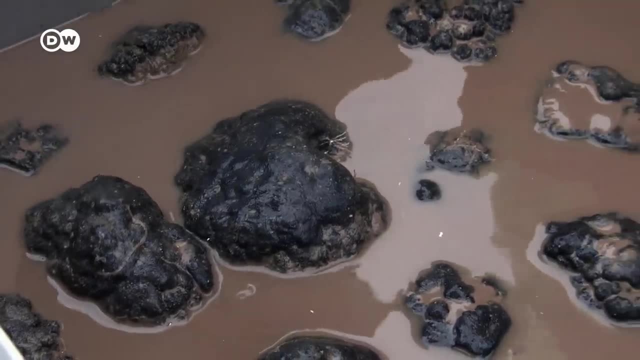 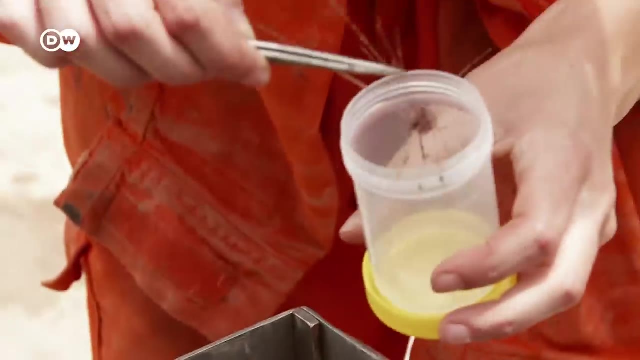 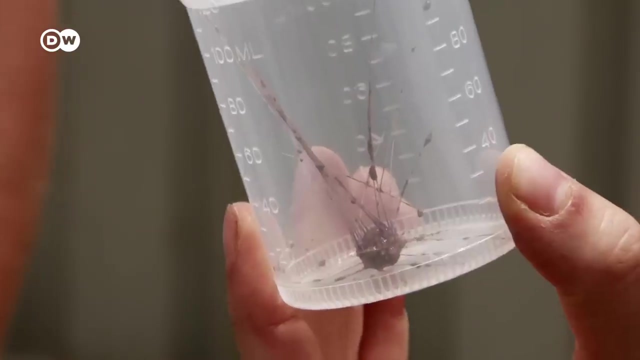 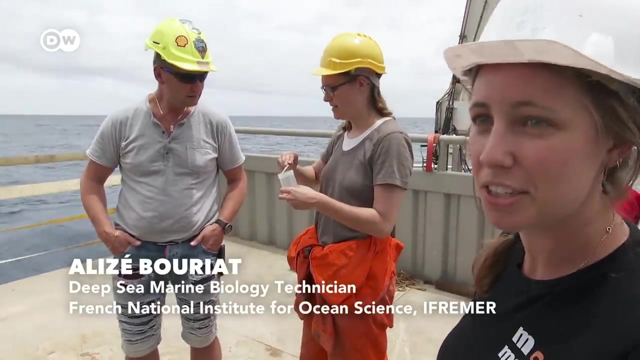 So the nodules are prehistoric stones And much of the deep-sea fauna in the Clarion-Clipperton zone are still unknown. Yeah, to have a big sample of a sea urchin is the first time that we have a sea urchin in the box core. 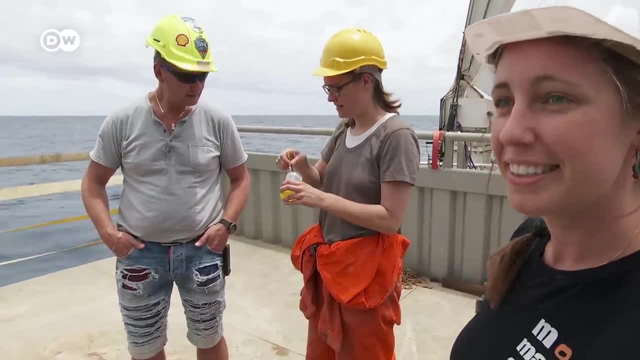 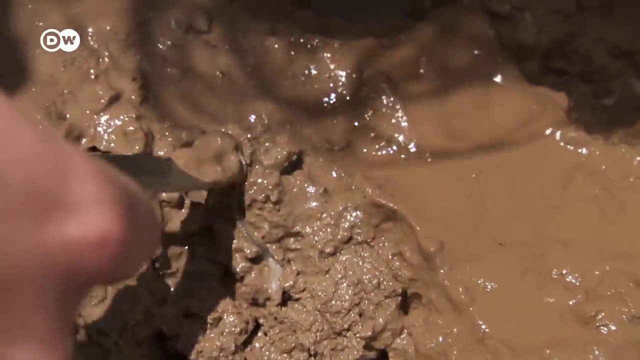 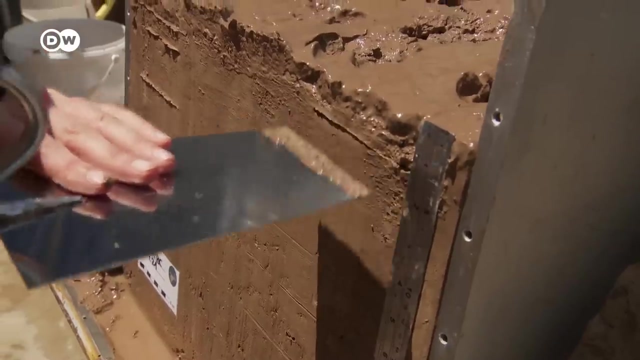 So that's nice. and it's in good shape, so it's nice. We're going to have a good analysis with that. The biologists and geologists meticulously examined their soil sample from the deep sea. For them, it's a real treasure. 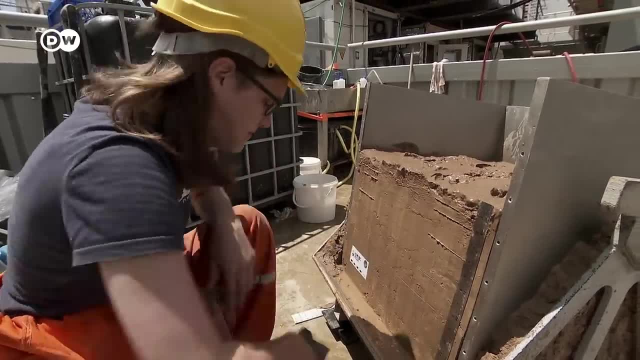 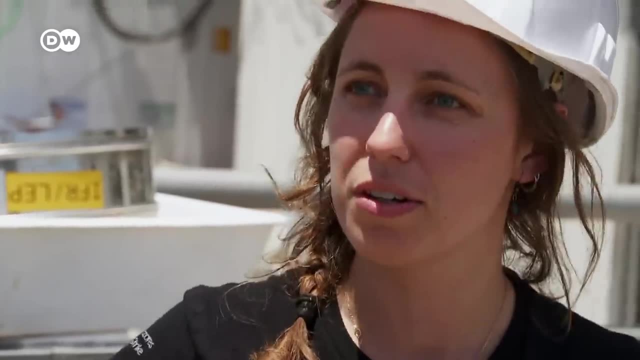 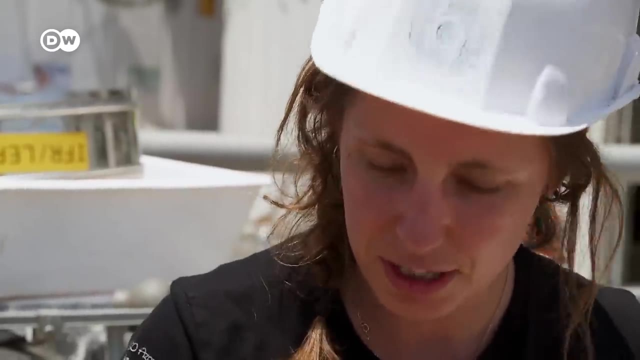 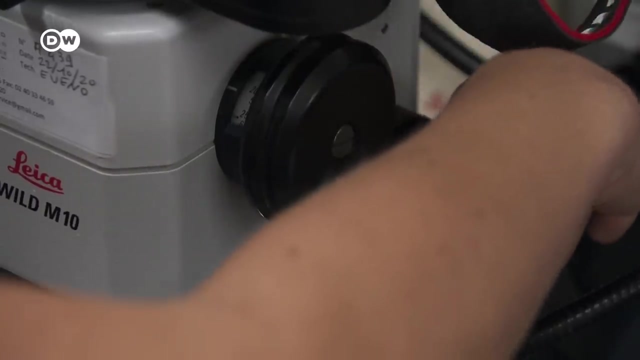 That's not just mud and stone, as you can imagine, because that's a very big view of our heritage. So that's amazing and there is a lot of life inside that you cannot see just by your eyes. You need a microscope. The French scientist loves looking at the microfauna. 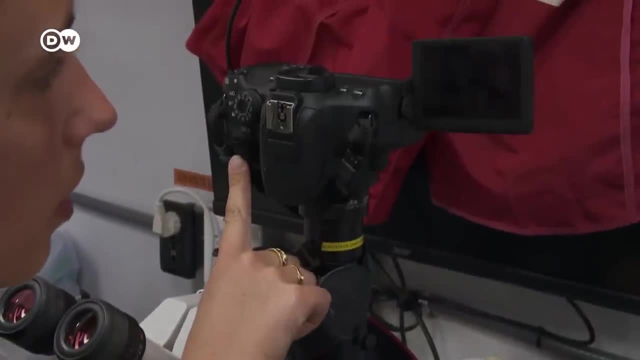 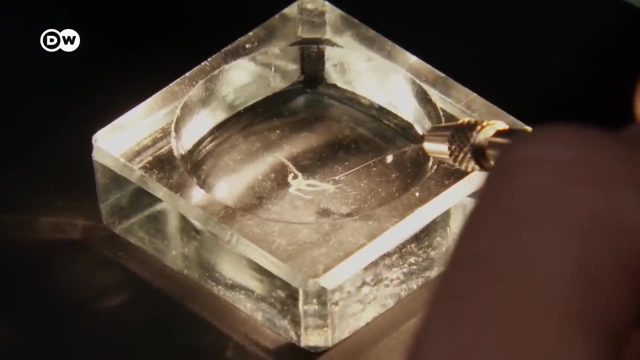 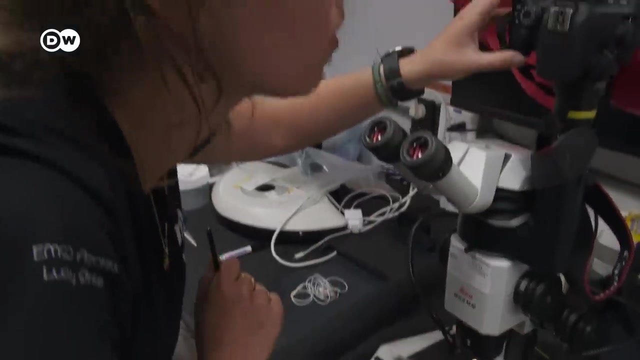 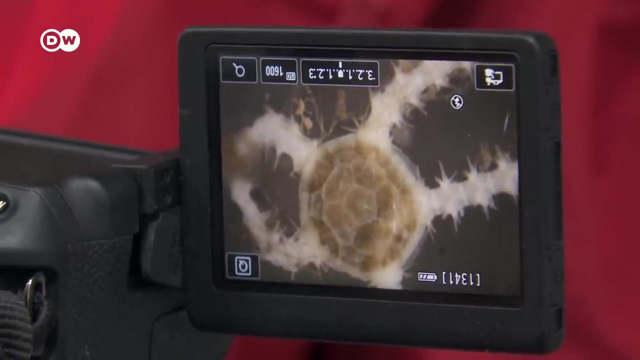 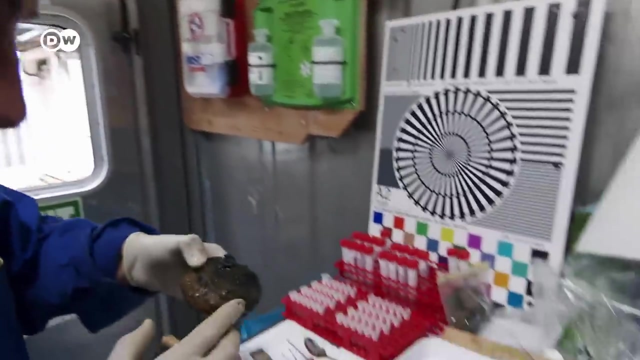 from the deep sea. In fact, she found several tiny animals and was delighted with every single one. All over the ship, tests were being carried out in the laboratories as well as in the sea. She was here in the cold room. 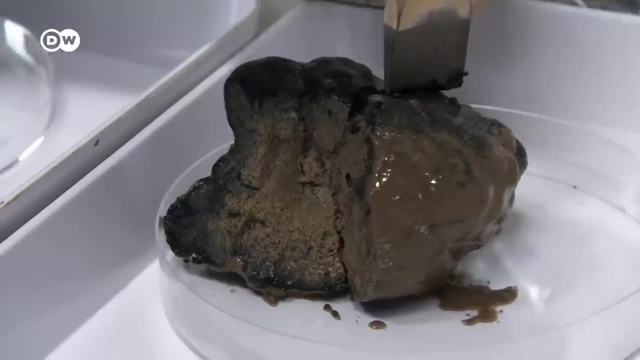 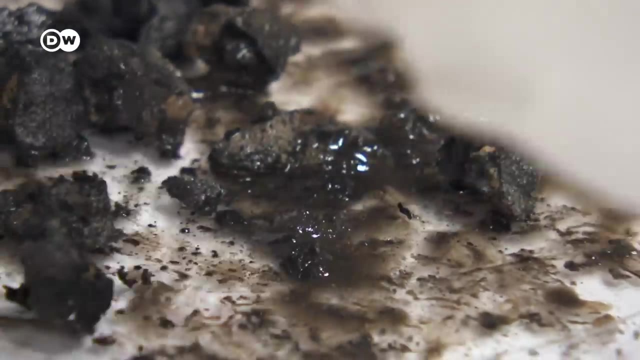 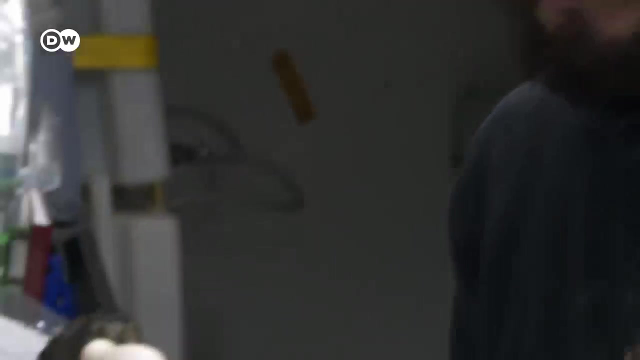 Everything that had come from the depths was analysed in detail. Studying the structure and activity of microbial communities in the sediment samples is the work of Turkish researcher Batuhan Yapan. In human history, we start to exploit and then see the results, and they are generally, unfortunately, bad for nature. 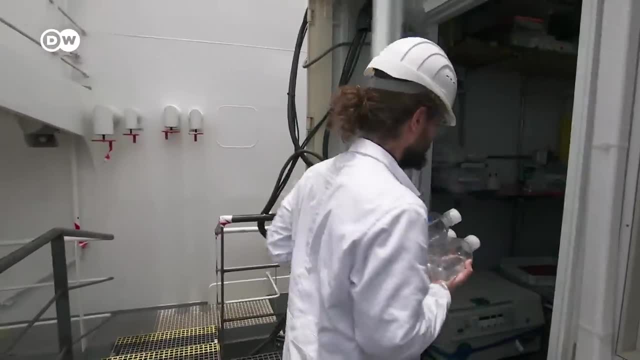 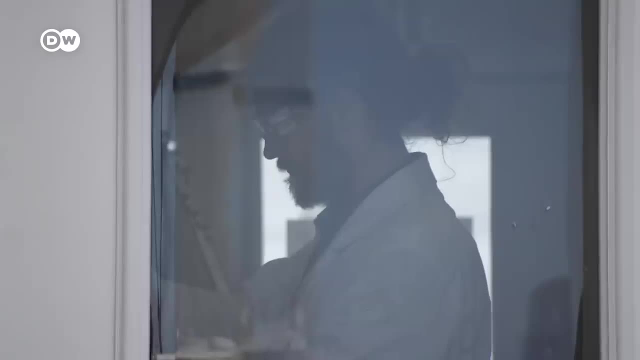 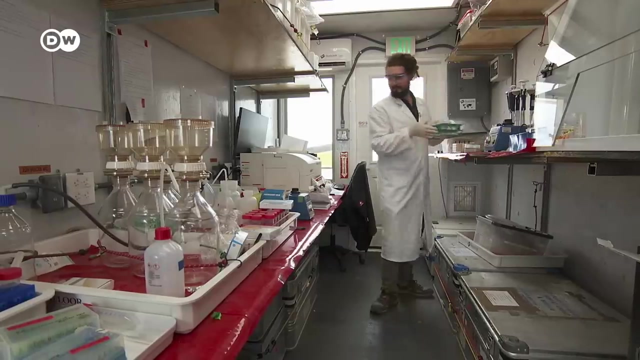 and in the end, for us, We are so excited because we need those resources. It looks so because we consume a lot and this time we will see impacts and maybe this time we can restrain our impact on nature and use those resources in a more sustainable 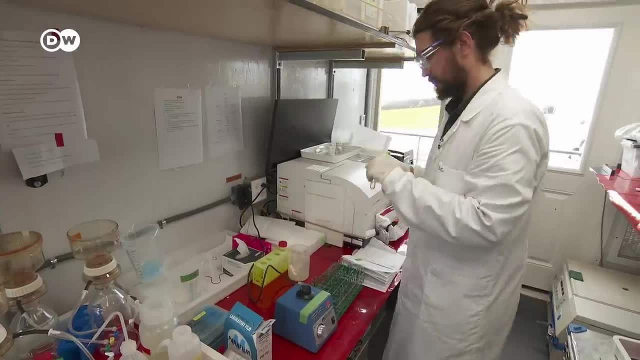 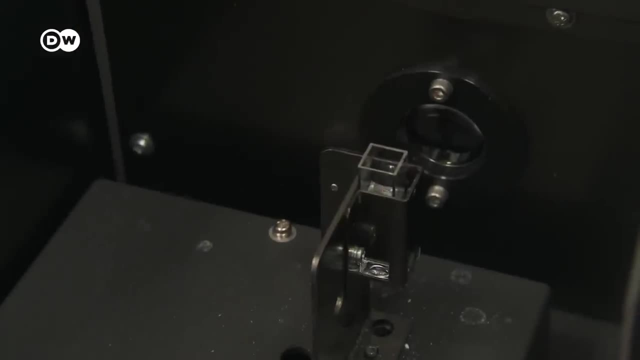 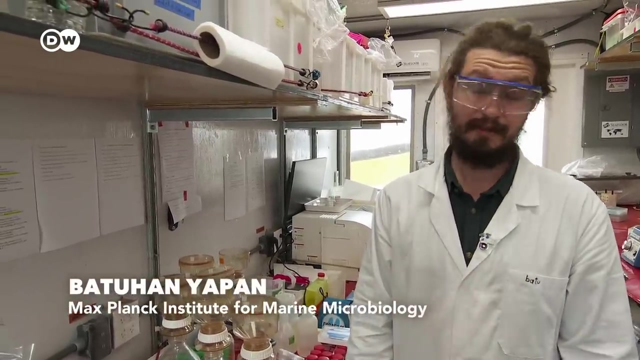 and environmentally friendly way. Personally, I would rather choose to consume less, and I don't buy a telephone every two years, for example, So I would prefer to reduce if possible, reuse and recycle in the end and not touch the sea floor as much as possible. 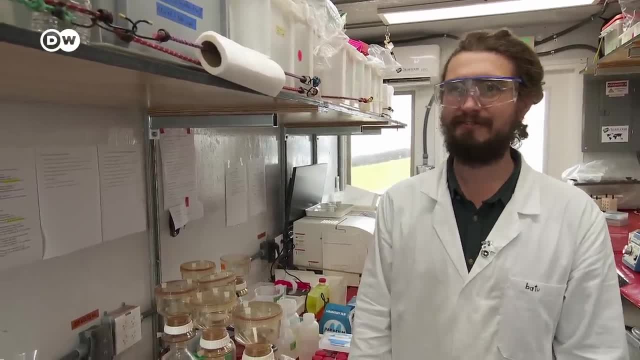 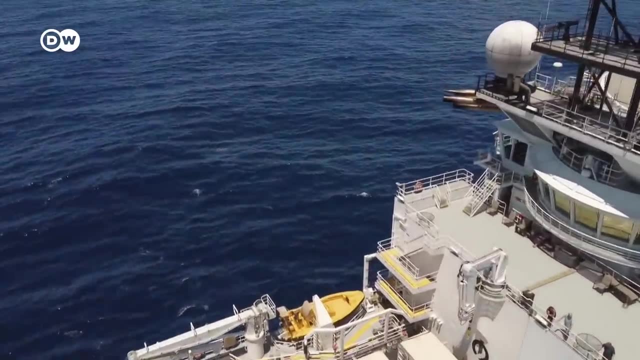 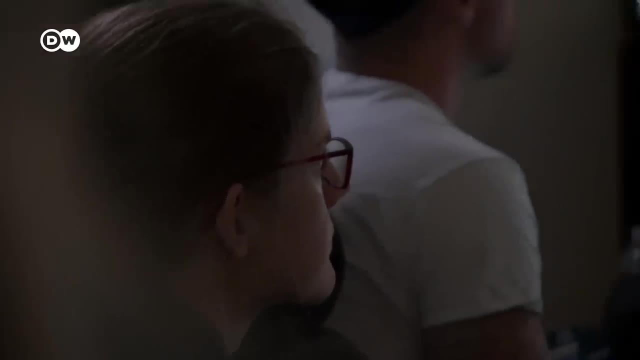 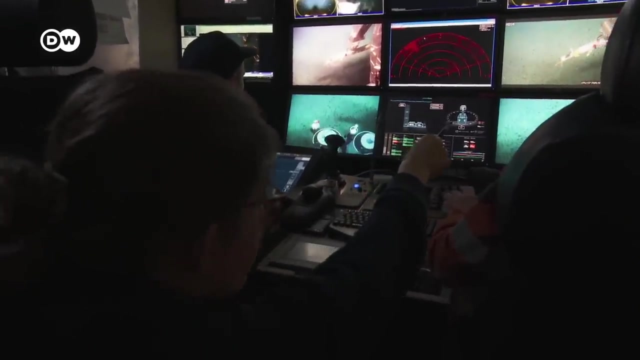 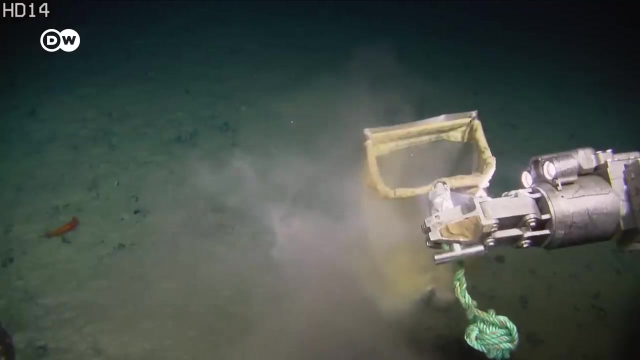 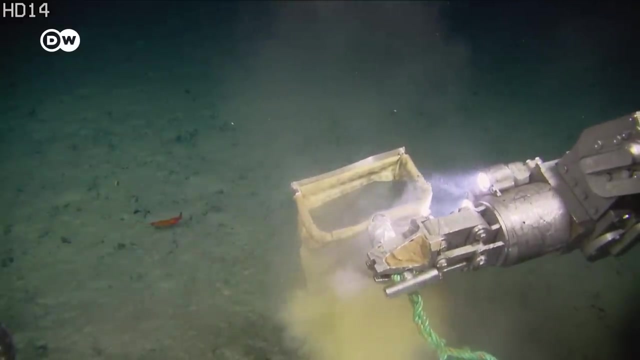 But yeah, we will need it. it looks so. Tanja Stratman has taken her seat in the control room. As a biologist, she was getting the chance to search the deep sea floor for larger animals working with the robot pilots. A shrimp drifting by didn't arouse much interest at first. 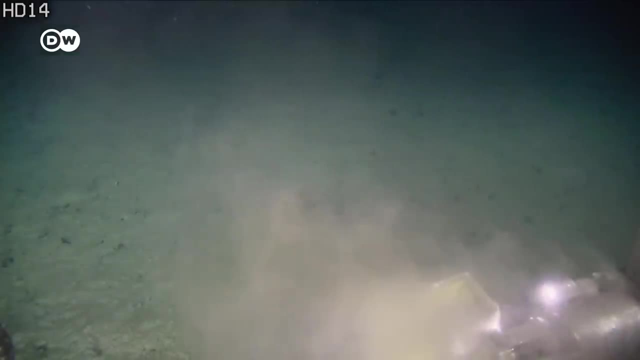 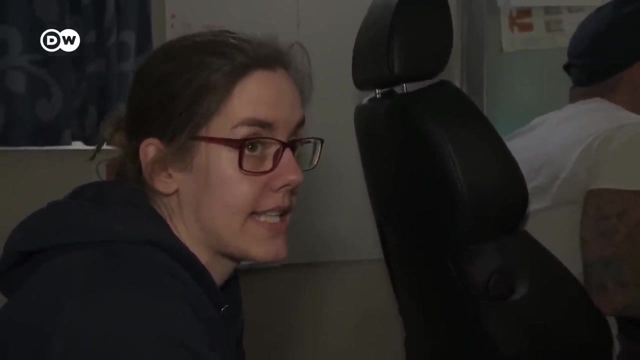 We've got a specific list of animals that we should gather first. We still have about an hour. We need to find a few more starfish and a few sea anemones. We'll take them too, Suck them up just like a vacuum cleaner. 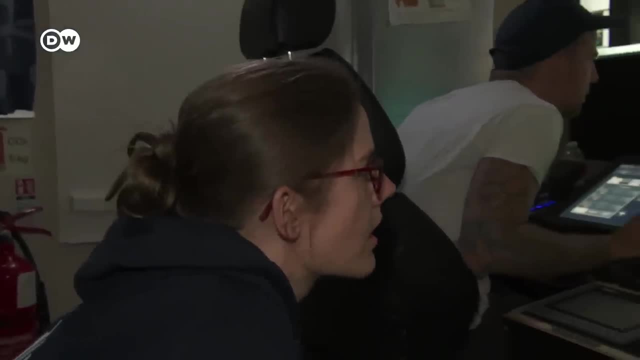 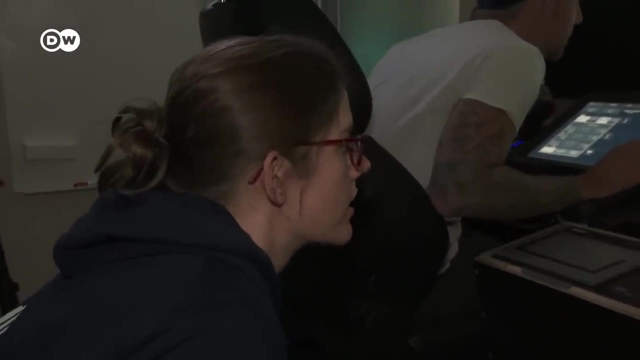 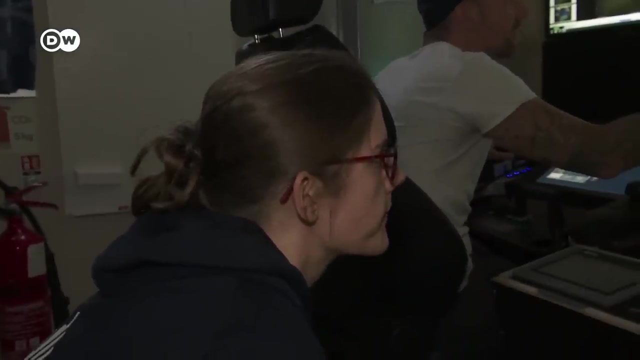 Something's happening over there. This is a sponge, I think. Do you want that? No, I think we will just thrust it if we try to suck it in. You can put it in an egg. Yes, you can. I mean, that's a perfect idea. 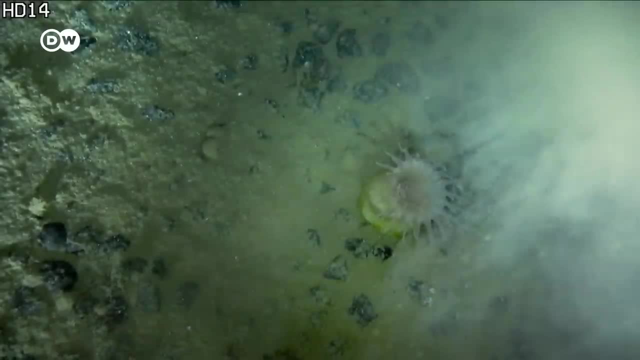 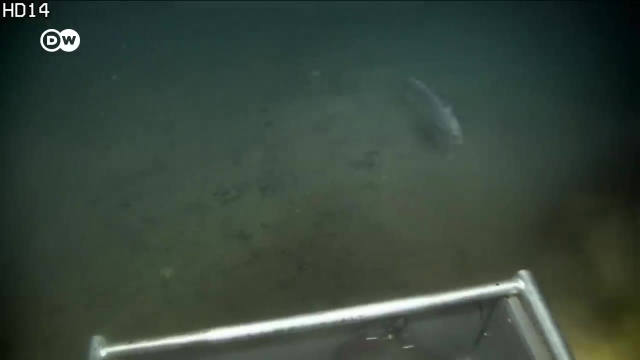 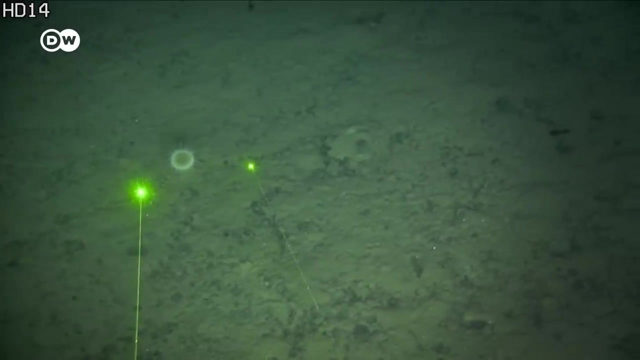 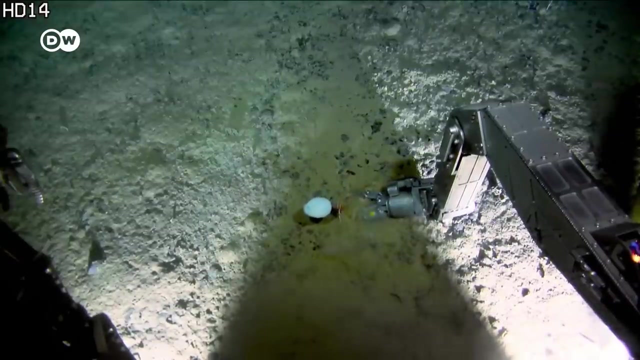 We can try to have it in a net. Tanja had her eye on the sea. anemone The robot found some other animals on flatter seabed. They looked strange. It's amazing that animals can live here at all, where the pressure is many hundreds of times higher. 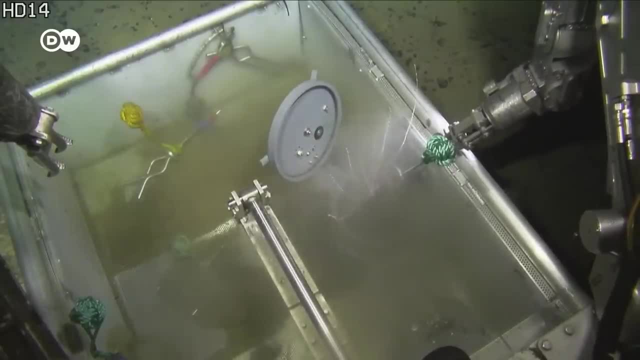 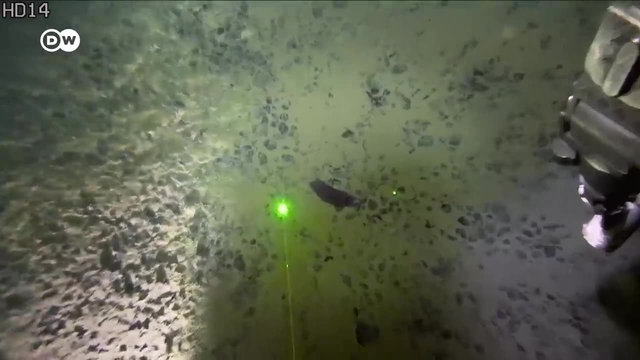 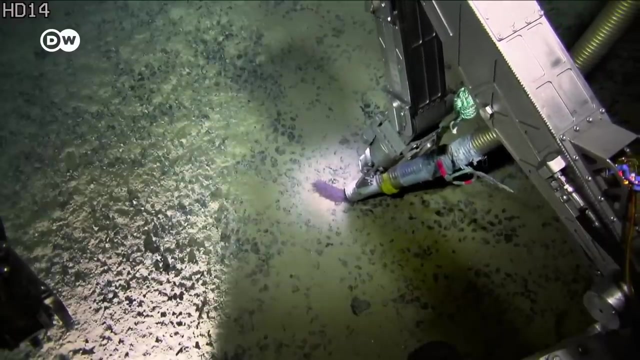 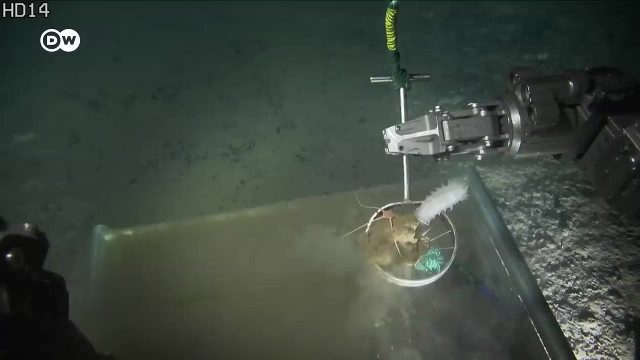 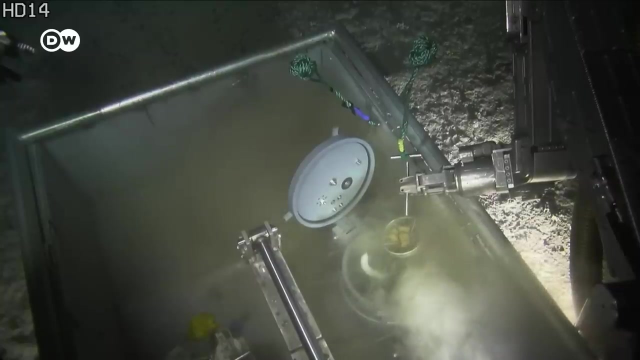 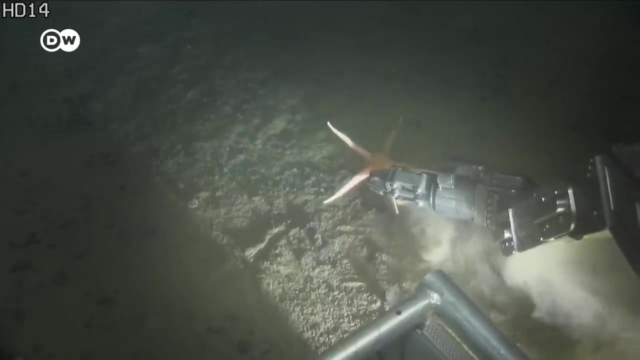 than at the Earth's surface. A large sea cucumber was sighted. The robot's sampling vacuum packed it away. He said one of the most beautiful things about the Earth is the fact that it's got a lot of stars in it. And then the robot found an unusually large starfish. 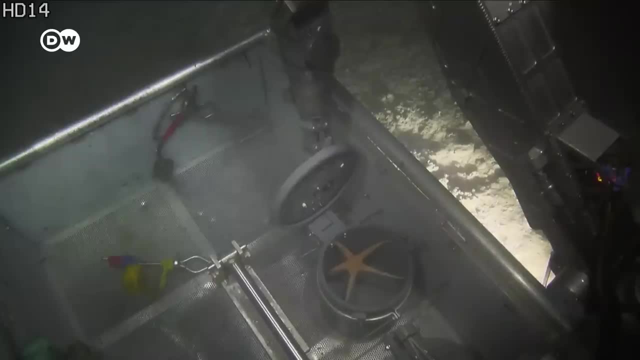 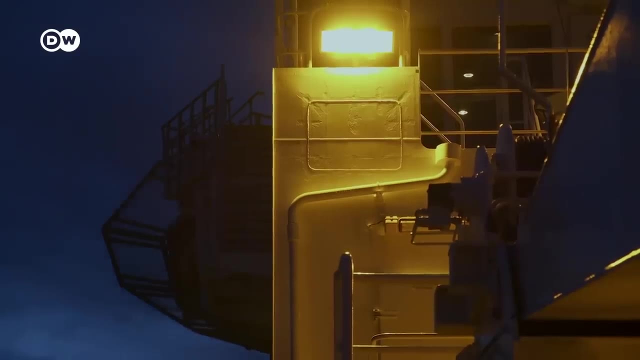 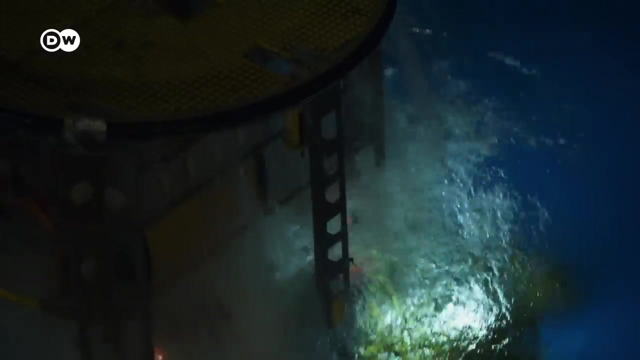 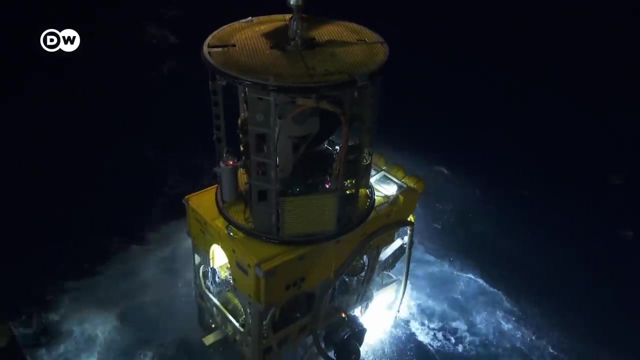 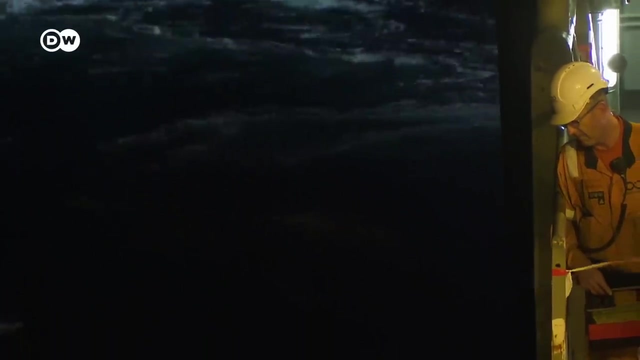 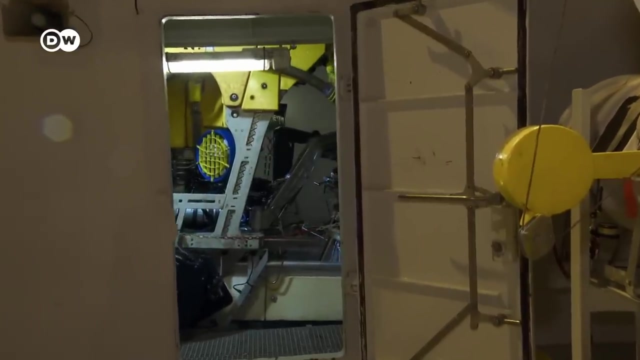 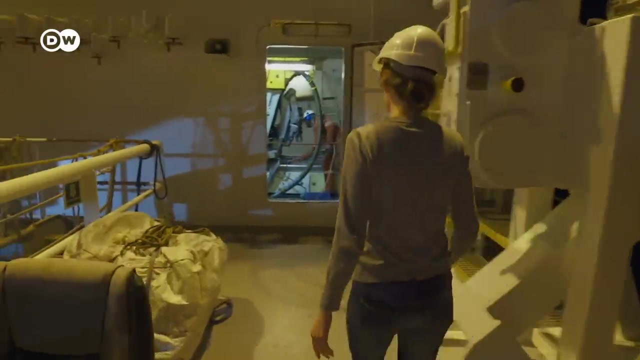 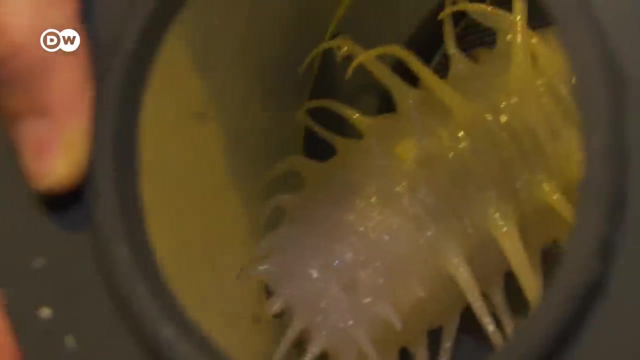 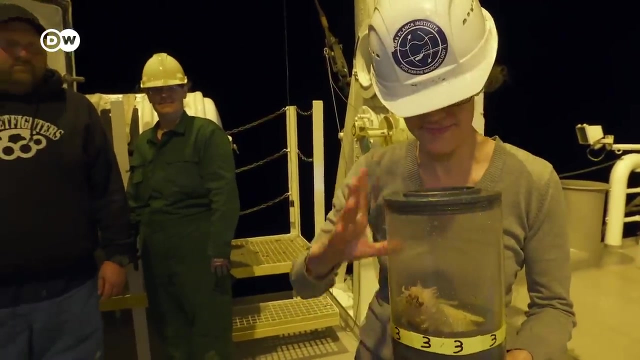 It, too, landed in the sample bucket, destined to find its way on deck. Hours later, the robot had finished its search on the seabed and was brought back up. Along with it came the collection of animals. The biologist was quite excited. I'm happy about the sea cucumber, even though I am probably the only one. 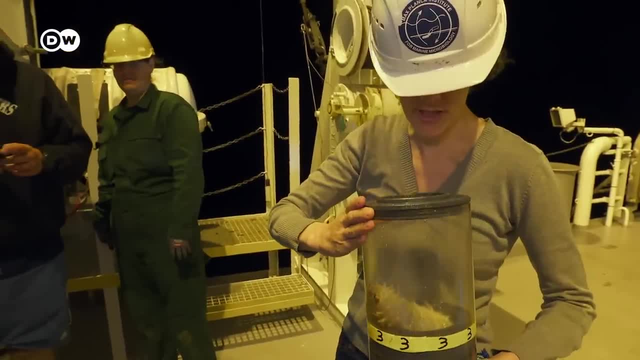 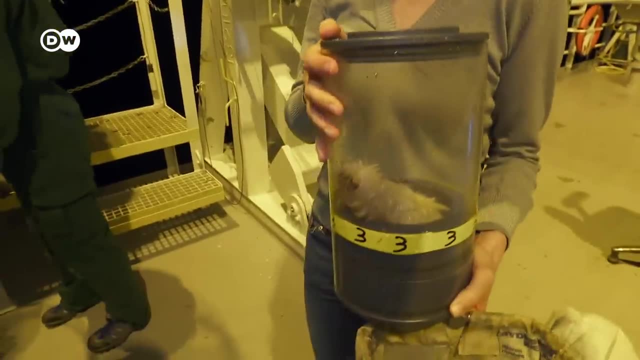 Now the sea cucumber goes into the cold room so that my colleague can dissect it tomorrow morning. Is it still alive? No, I don't think they can handle the pressure difference and especially the temperature difference of over 20 degrees. They die on the way up. 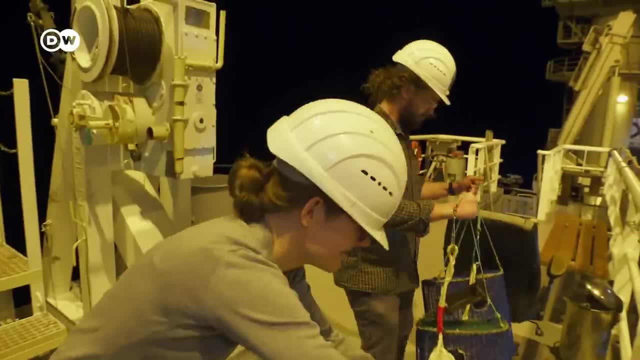 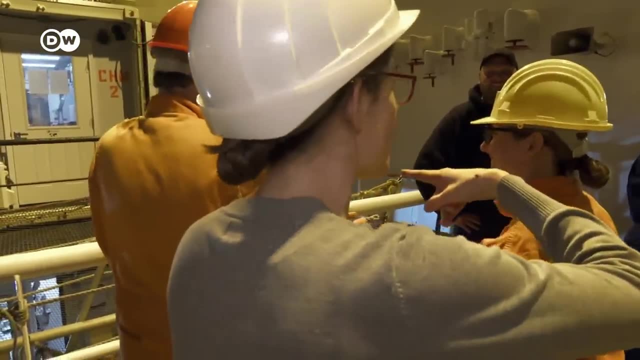 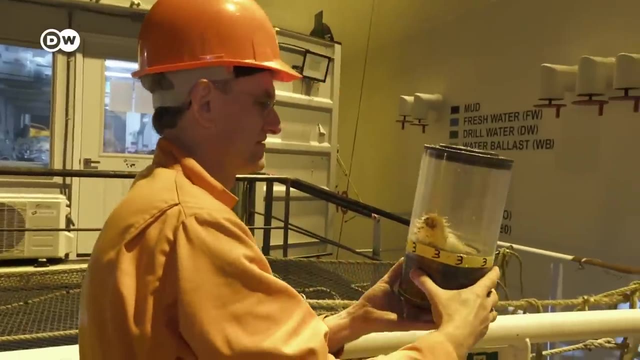 Don't touch them, guys. they are mine. It was a special moment for the other scientists too. They were thrilled to hold these life forms from the depths so close to them. I like it. It's beautiful, It's strange. 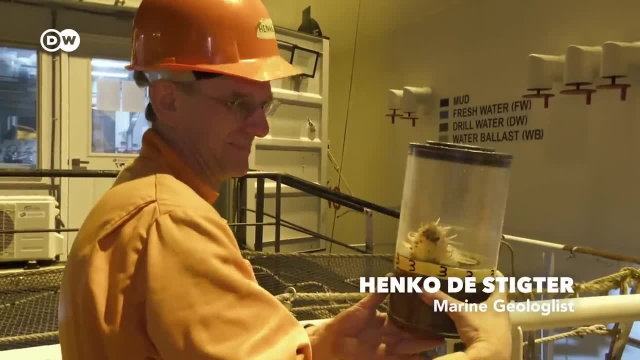 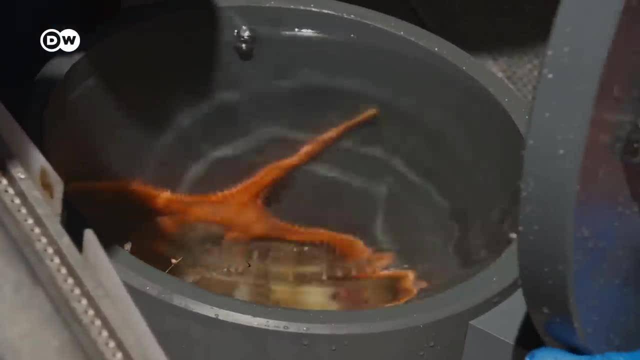 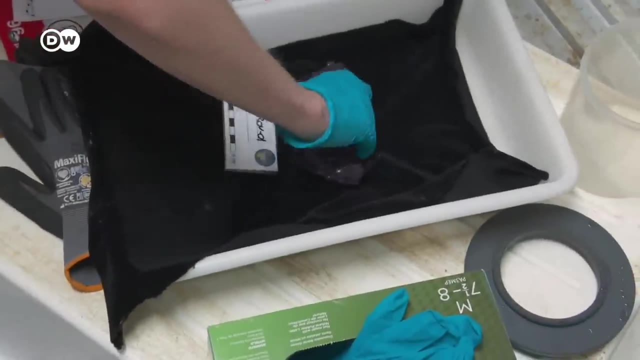 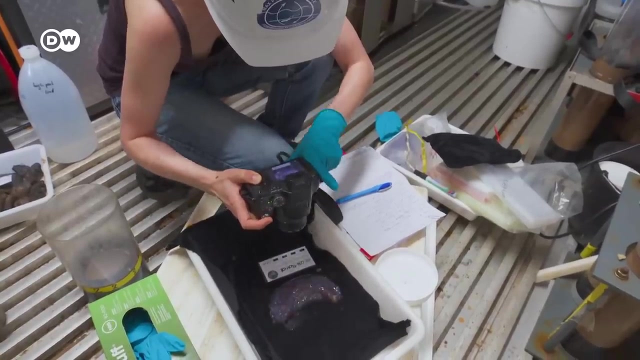 It's weird. It's It's From now to a world that An other world. This is awesome. We have everything that we collected. It must be up there. Tanya Straatman knows that humanity barely has a clue about what lives deep below the. 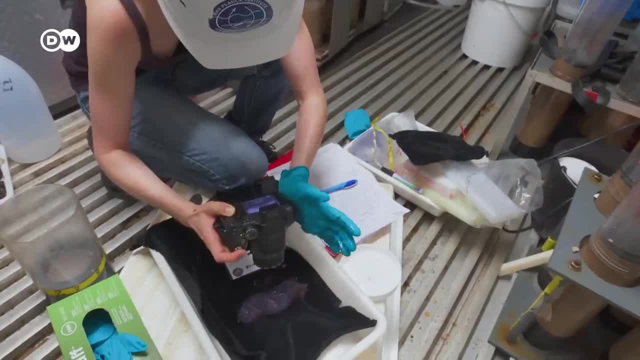 waves. But it's not all that simple. Tanya Straatman knows that humanity barely has a clue about what lives deep below the waves. Tanya Straatman knows that humanity barely has a clue about what lives deep below the waves, But it's not all that simple. 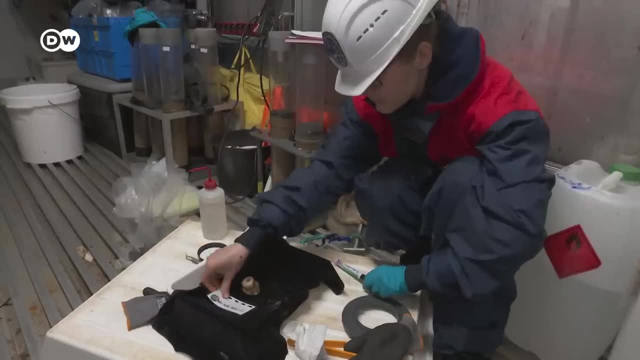 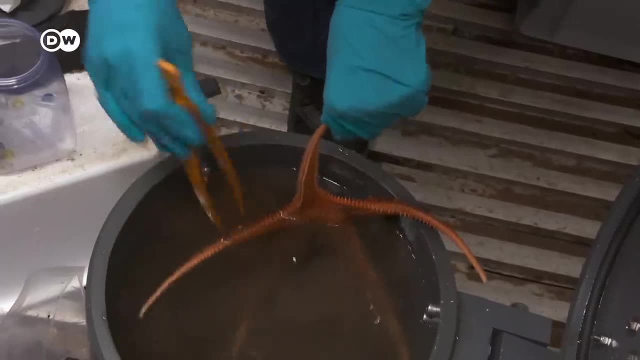 All that they knew at the time of their mission was that biodiversity is high in the depths of the Clarion-Clippatant zone. But it's not all that simple. All that they knew at the time of their mission was that biodiversity is high in the depths. 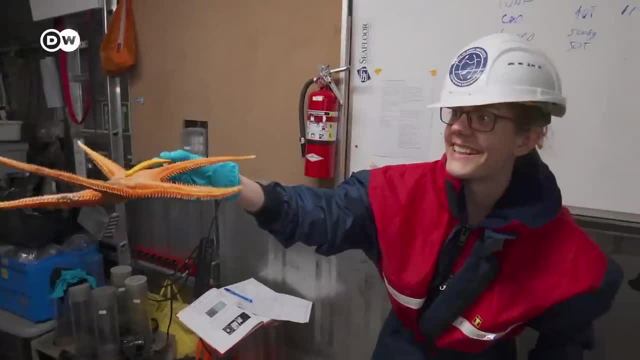 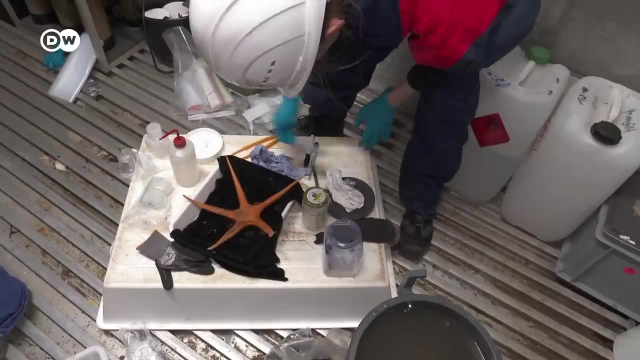 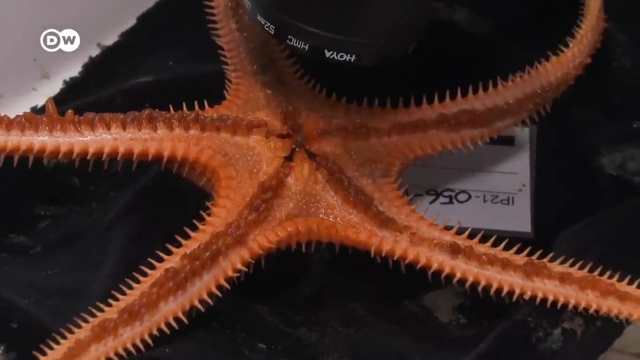 Some experts suspect that, despite the adverse conditions, deep below the surface there could be greater species diversity than even on land. It's possible that Tanya Straatman had brought the most scientific scientific evidence. it's possible that Tanja Stratmann had brought a previously unknown species up on deck. 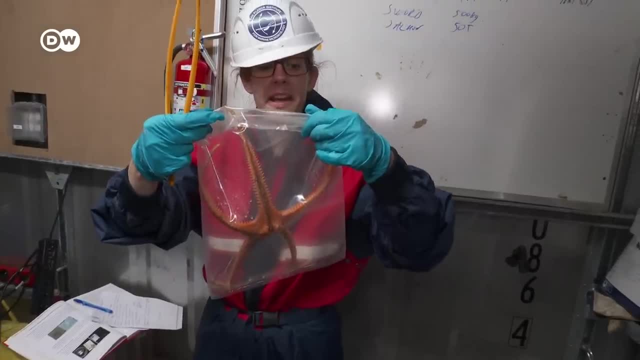 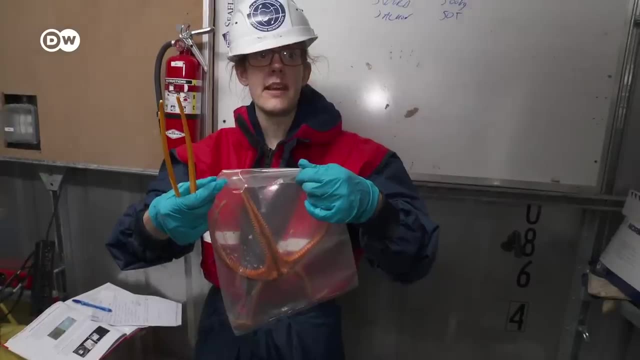 Honestly, I'm not sure if this is a new species. That's why we're freezing it right now at minus 80 degrees, so that my colleagues at the Senckenberg Institute can determine if it is a new species we've just discovered or if it's only one still unfamiliar to me. 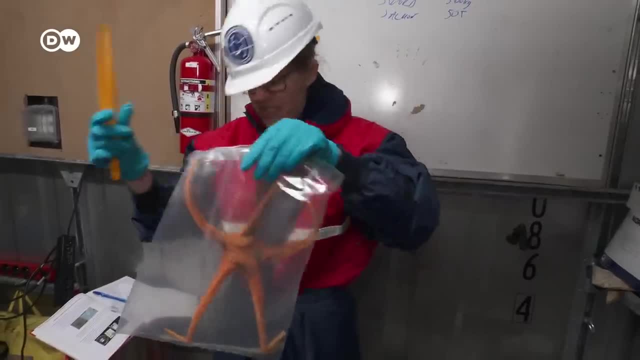 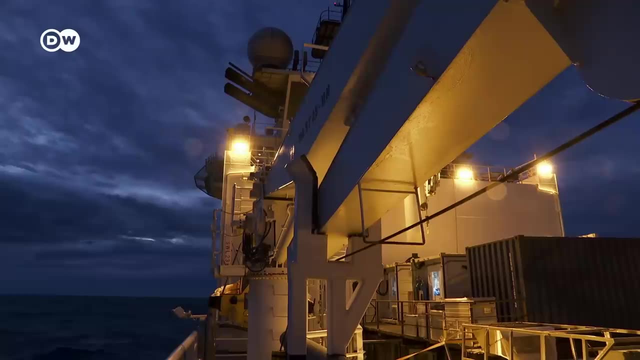 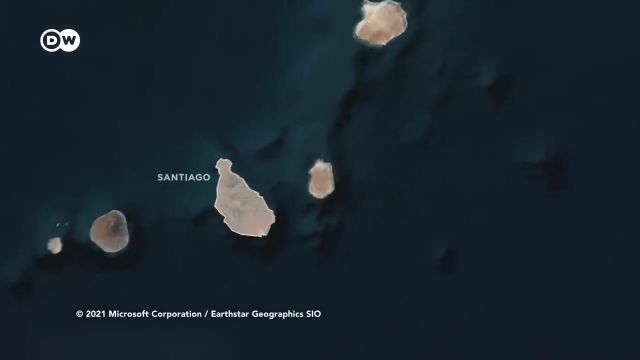 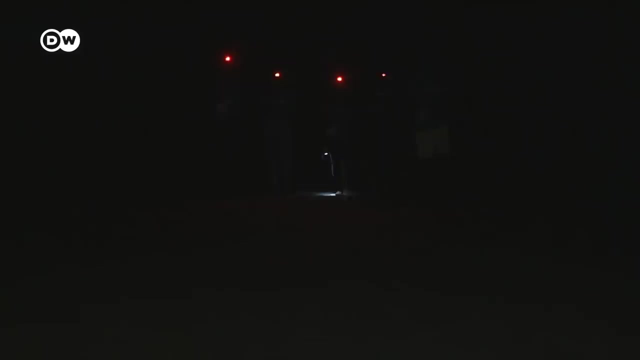 It's possible that this one only lives in the deep sea, or I just don't know it. yet It was a time of wonder and joy aboard the island Pride. Far away on the islands of Cape Verde in the Atlantic, the conservationists of Lantuna were celebrating their small success. 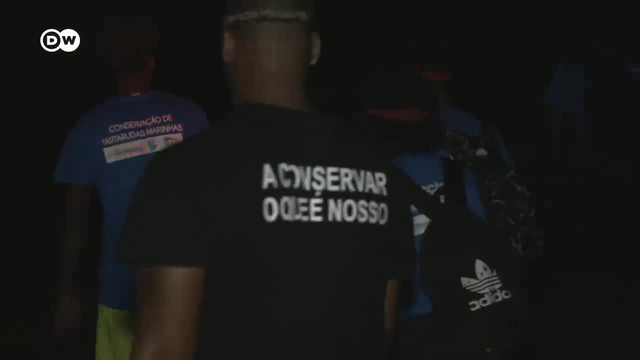 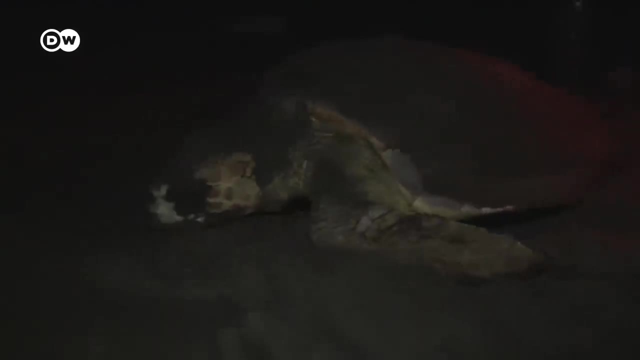 In summer, during the night time, sea turtles come on shore to lay their eggs. They usually begin reproducing at the age of 20.. That's when the females find their way back to the beaches where they were hatched to lay their own eggs. 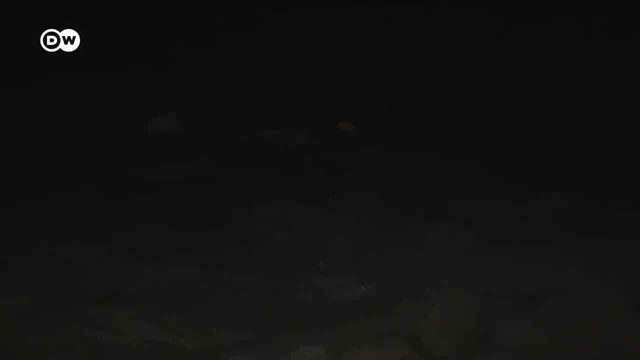 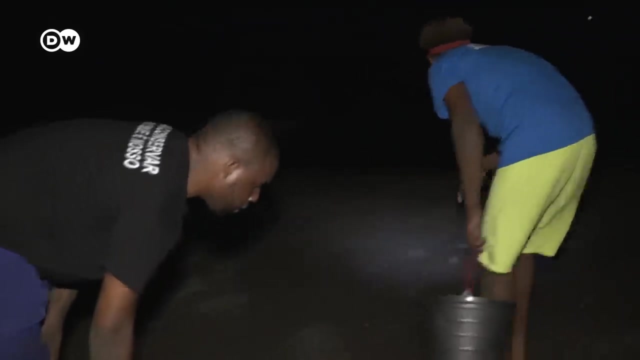 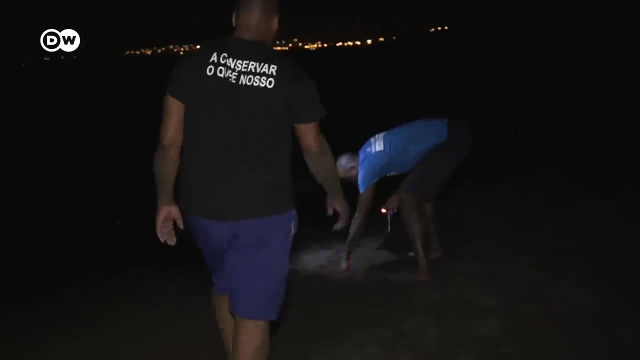 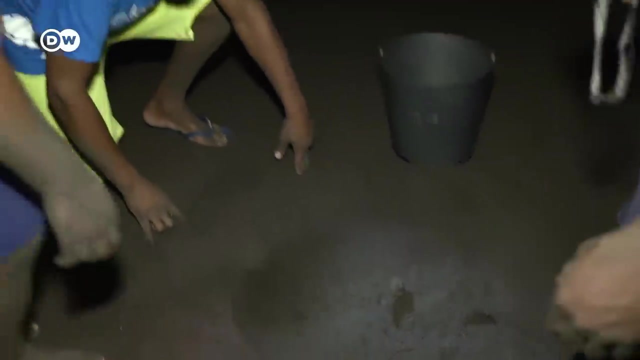 If they're lucky, they'll find sand to dig a hole for their nest. The team from Lantuna is spending every night there for three weeks. They find the nests, dig them up and take them to their protected nursery. There are too many nest predators, both human and animals alike. 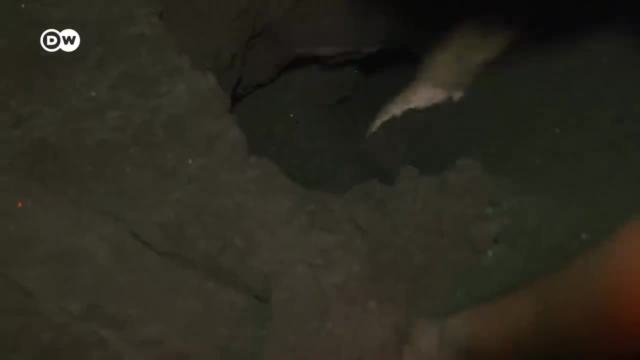 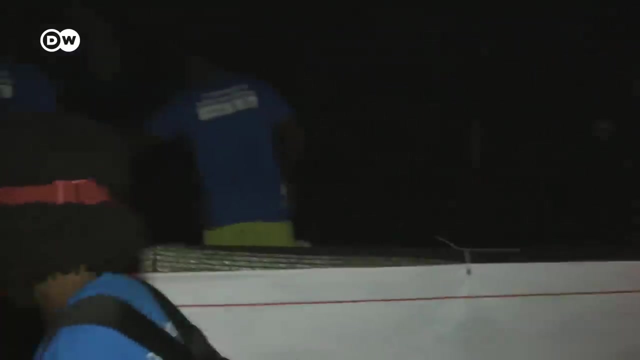 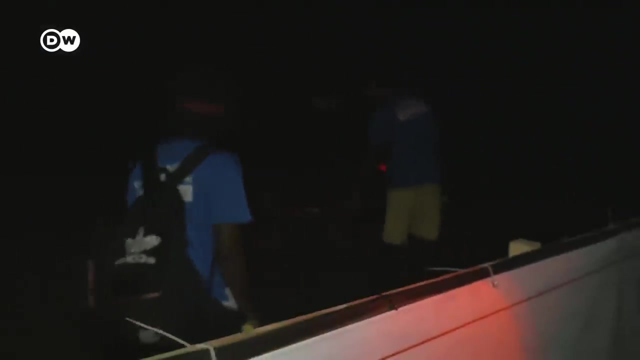 to let nature take its course. Without the help of the conservationists, the turtles would have an even greater struggle to survive, given their shrinking habitat. There are moments of wonder. every night now at the small nursery, Baby turtles are emerging, digging their way out of their sand nests. 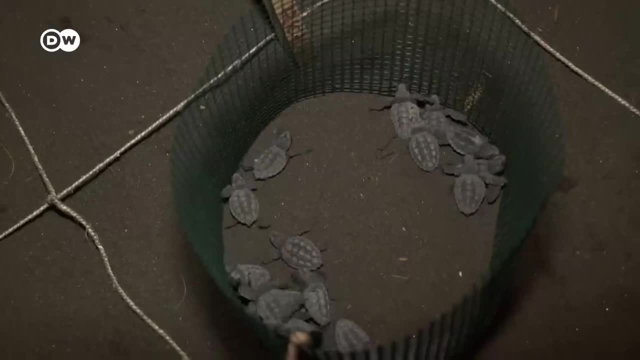 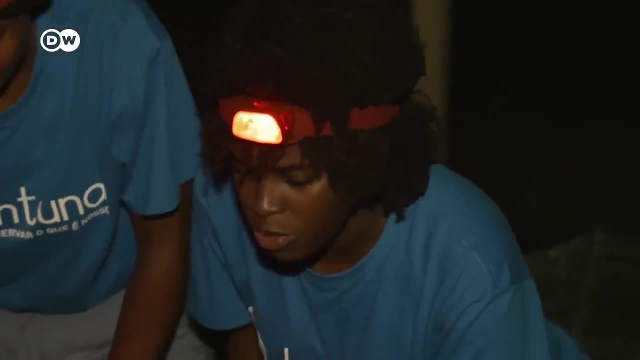 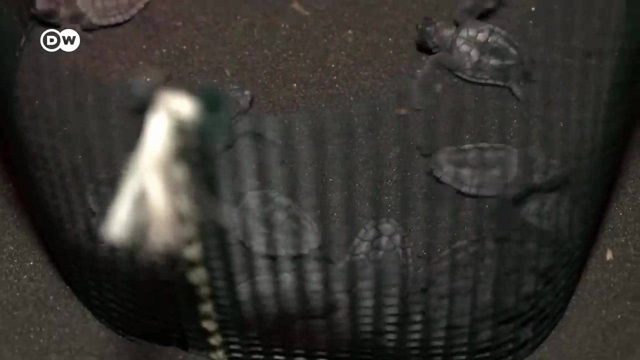 It's a time of joy and satisfaction for Anna and her team. Well, it's happening. The turtles are happy. They're watching, so you can see the baby turtles. So now we are going to test the baby turtles to see how strong they are grown. 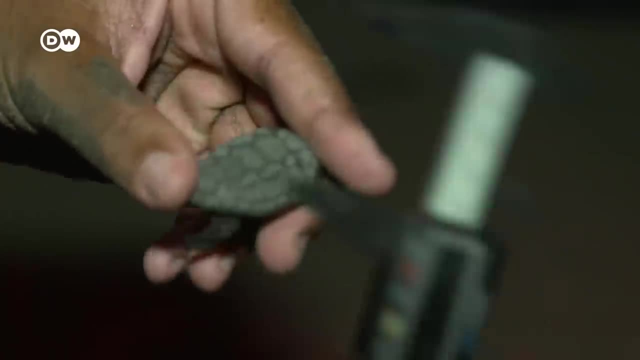 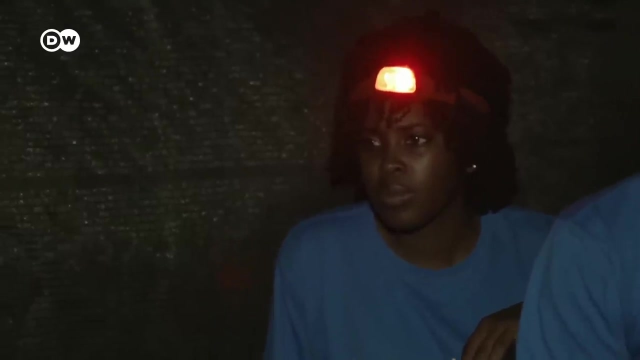 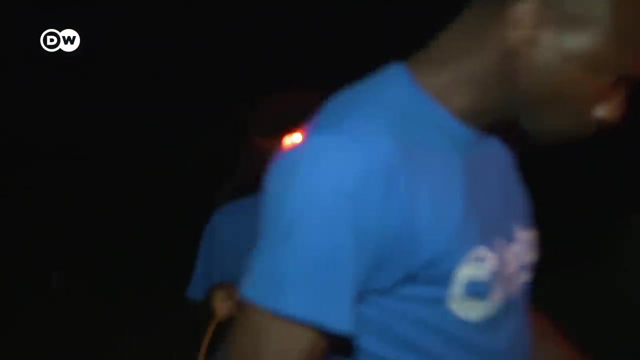 They're weighed, measured and counted, Precise records are kept And then they're given a little head start. The offspring are carefully carried close to the sea so they won't fall prey to anything or anyone on the beach. How many are there? 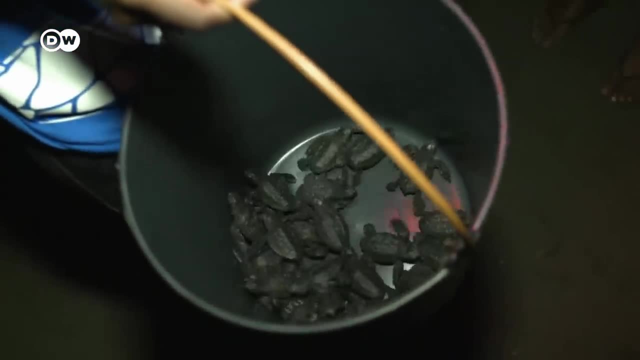 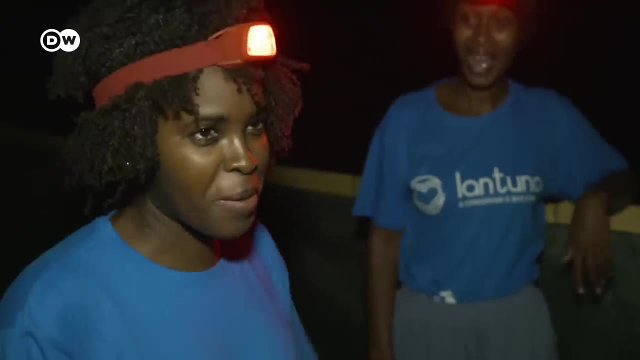 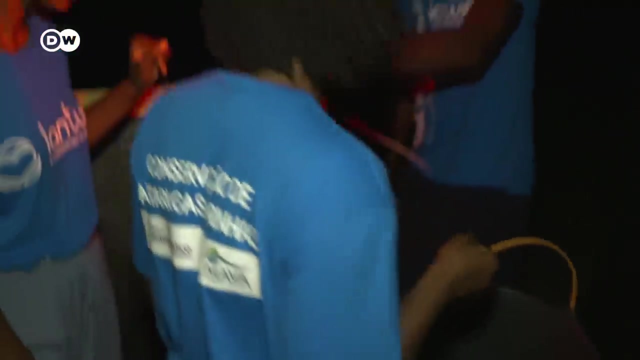 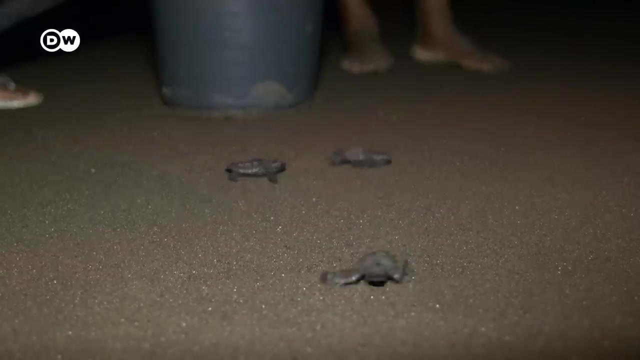 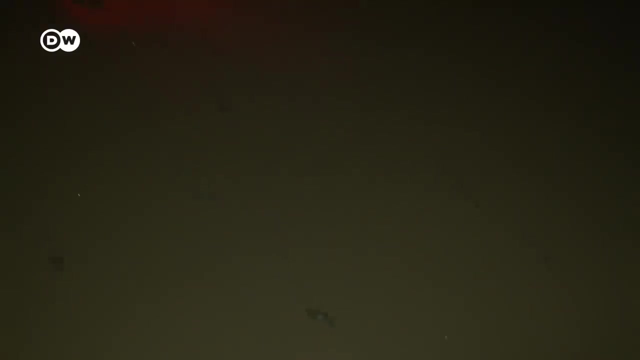 Here 28.. And now we release them. Yes, we are going to release them And wish them good luck. Yes, we are going to release them. Yes, we are going to release them Without the dedication of conservationists like Anna and her team. 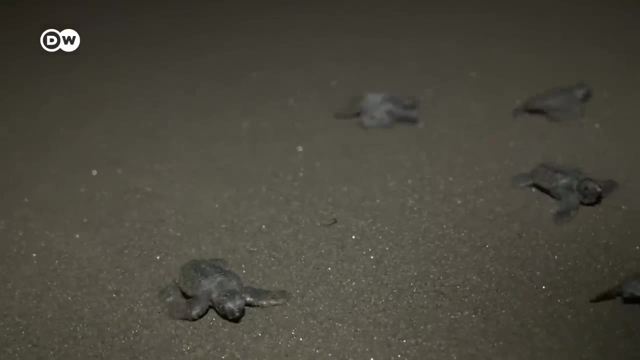 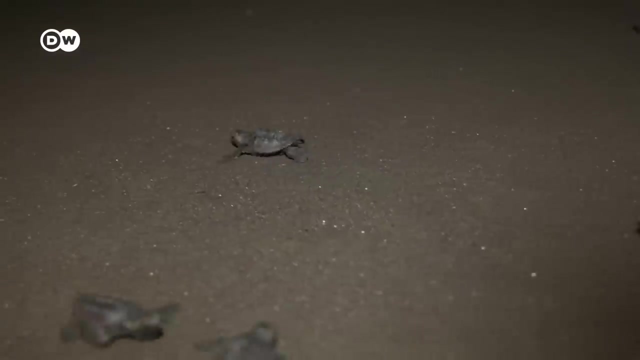 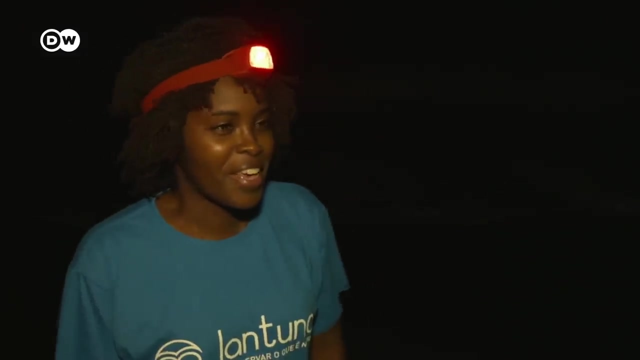 things would be much worse for the turtles in the Atlantic Ocean around Cape Verde. We're going to leave them in the water. We're going to leave them in the water. They're going to be very happy. They're going to be very happy. 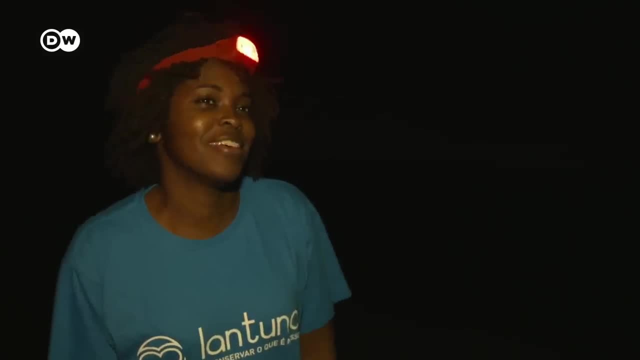 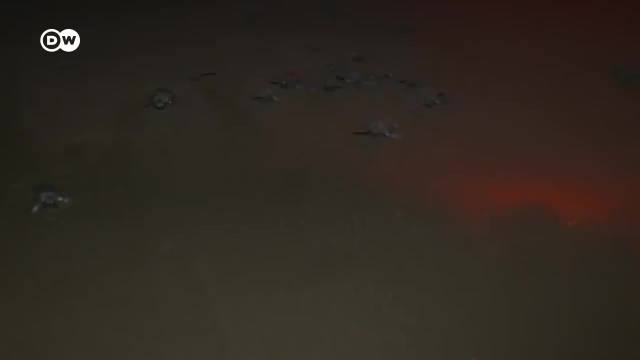 Really happy is always an emotional moment and also a moment of hope. We hope that in 15,, 20 years those little turtles will return to lay their eggs. So this gives us the strength and hope to continue this conservation work. So this gives us the strength and hope to continue this conservation work. 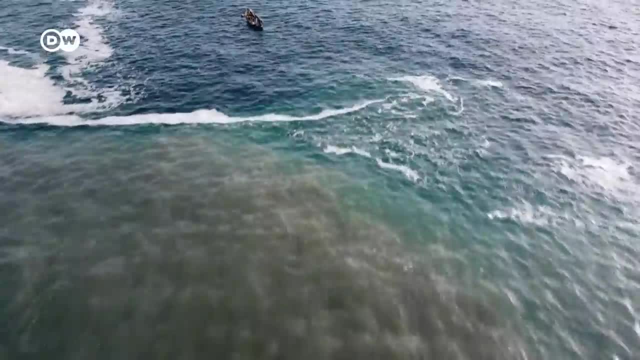 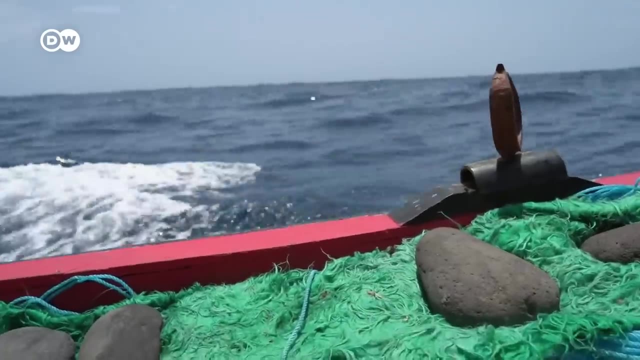 But Anna says there is much more to be done to improve the condition of the oceans. The stripping of sand from so many beaches has also affected marine life just off the coast. Food sources for fish have dwindled. Food sources for fish have dwindled. 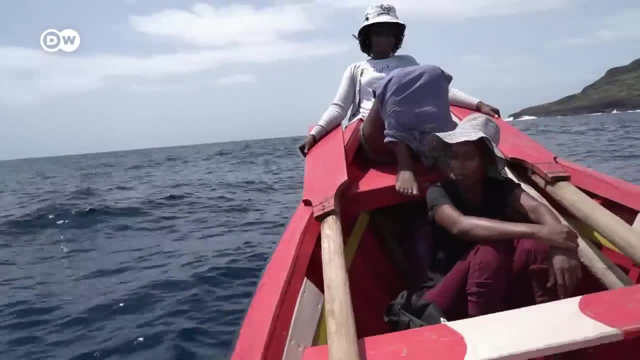 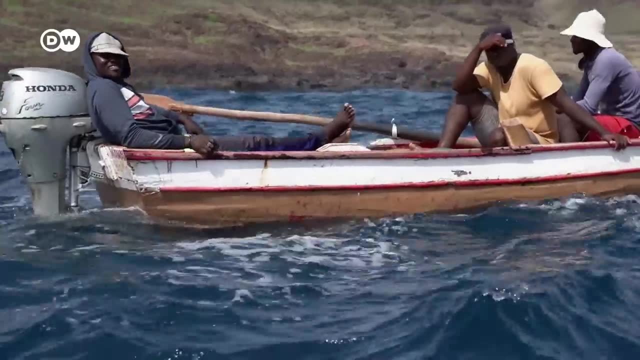 and there are fewer opportunities to spawn and there are fewer opportunities to spawn. The fishers catch less and less and need to go ever farther out, But Anna is proud of the fact that fishing here is sustainable. It's all about people's individual needs. 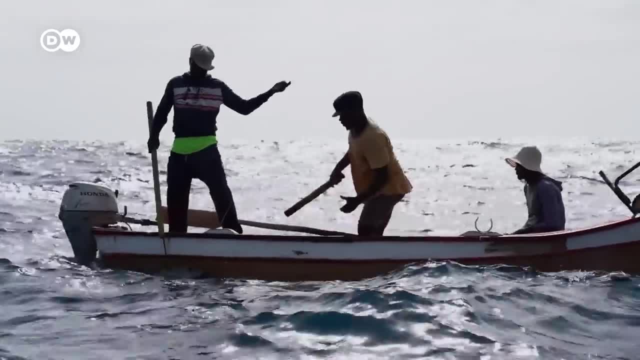 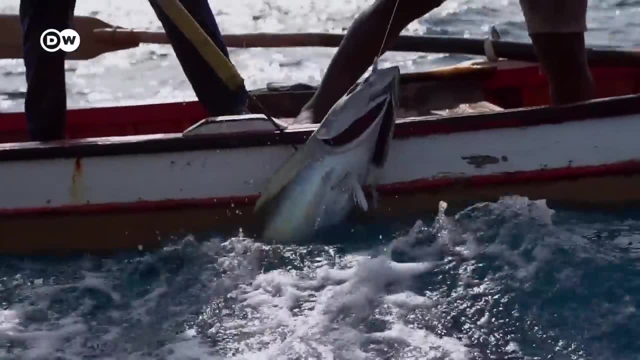 rather than industrial bottom trawling and hooked lines that extend for kilometres. There's no bycatch either. This boat takes in its catch of the day. A tuna this size is enough to feed several families. A tuna this size is enough to feed several families. 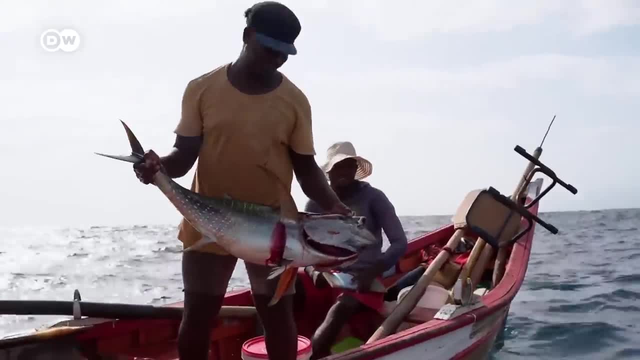 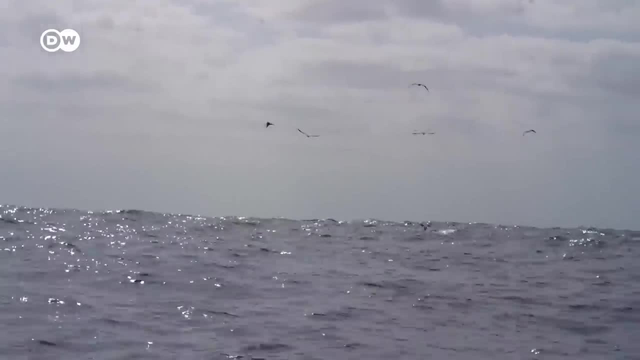 Fishing like this doesn't harm ocean biodiversity. Fishing like this doesn't harm ocean biodiversity, But that's not the case everywhere on the high seas. But that's not the case everywhere on the high seas, According to the UN Food and Agriculture Organisation. 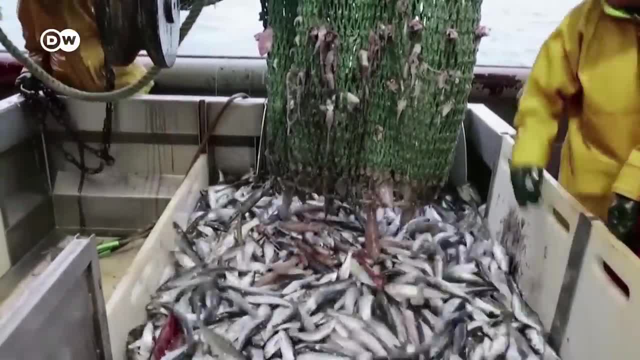 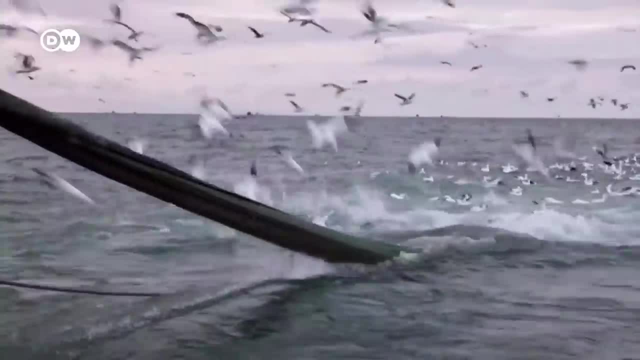 one third of all fish stocks are overfished. One third of all fish stocks are overfished. Technically sophisticated large fishing fleets are scouring the oceans bare. are scouring the oceans bare. Catch quotas set by politicians often miss their target. 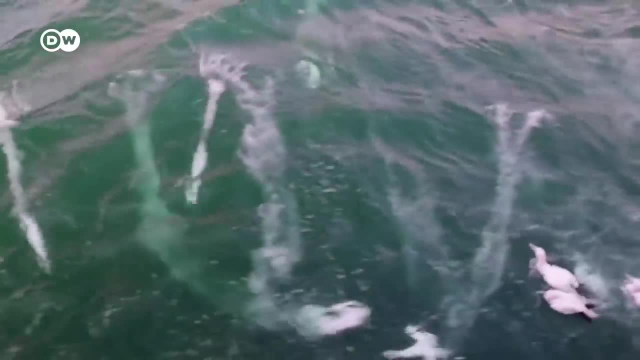 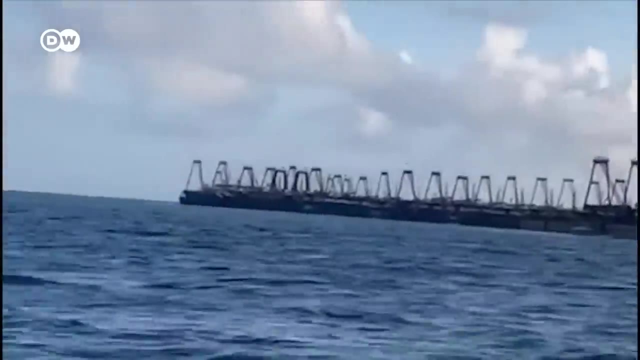 Catch quotas set by politicians often miss their target. A huge fleet of Chinese industrial fishing vessels. A huge fleet of Chinese industrial fishing vessels works around the world round the clock, works around the world round the clock At sea for months. they load their catches directly onto cargo ships. 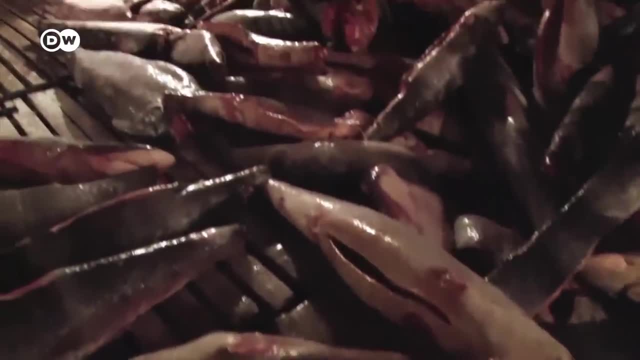 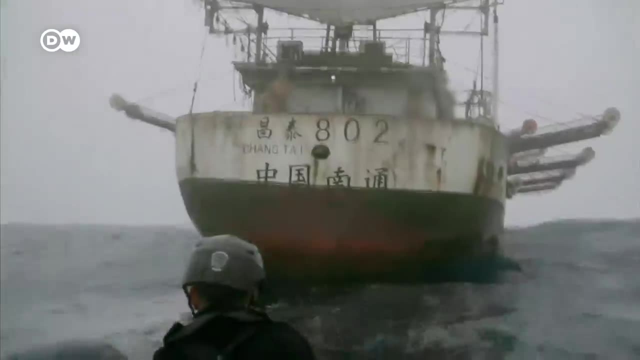 At sea for months. they load their catches directly onto cargo ships. Many billions of dollars in subsidies, Many billions of dollars in subsidies, fuel this harmful plundering of the oceans. fuel this harmful plundering of the oceans. fuel this harmful plundering of the oceans. 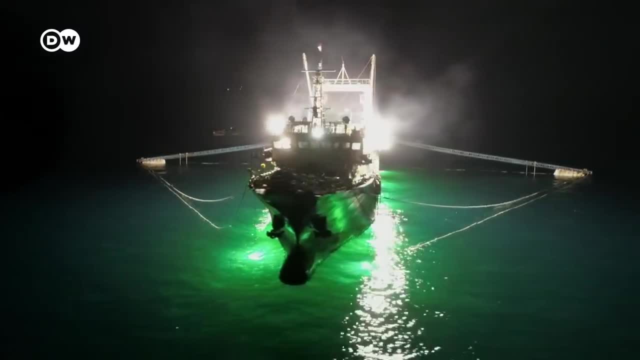 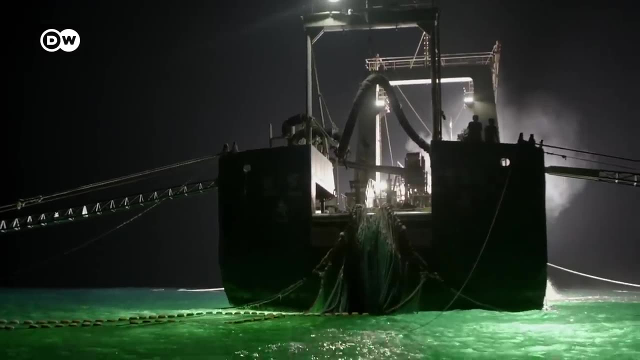 Chinese ships like this one are specially designed to catch squid. Chinese ships like this one are specially designed to catch squid. The animals are attracted by powerful lights at night. These boats ply the waters mainly in the Indian Ocean. These boats ply the waters mainly in the Indian Ocean. 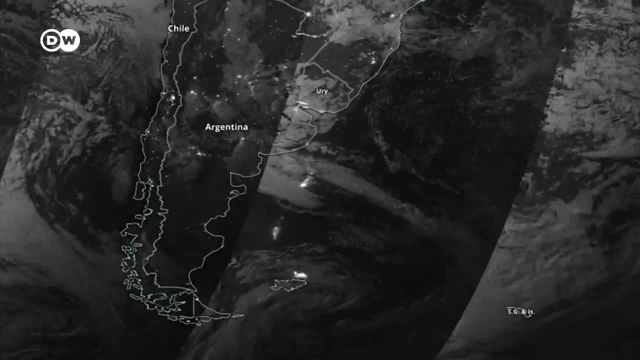 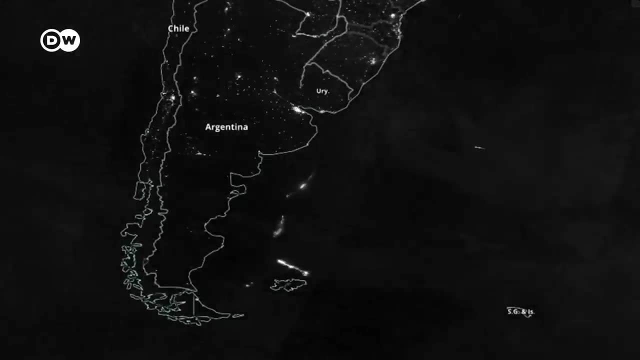 or work off South America. These images taken from space show light sources off the coast of Patagonia. These images taken from space show light sources off the coast of Patagonia. These images taken from space show light sources off the coast of Patagonia. 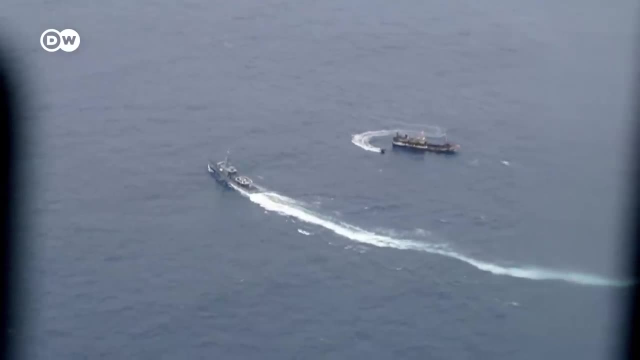 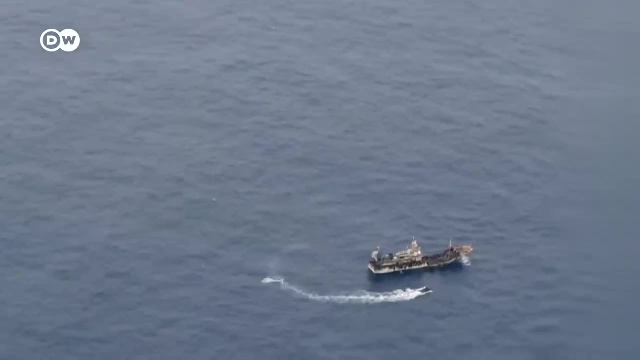 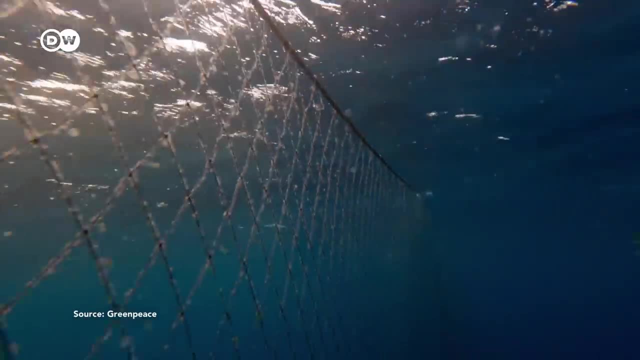 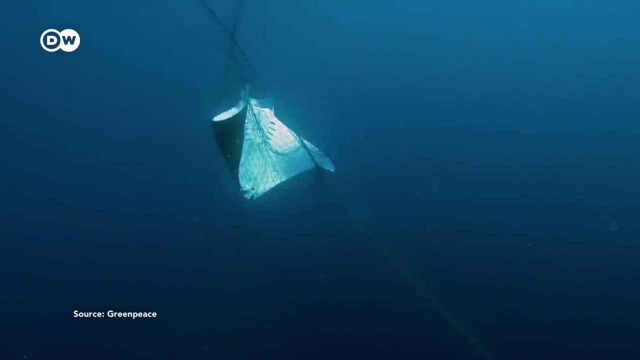 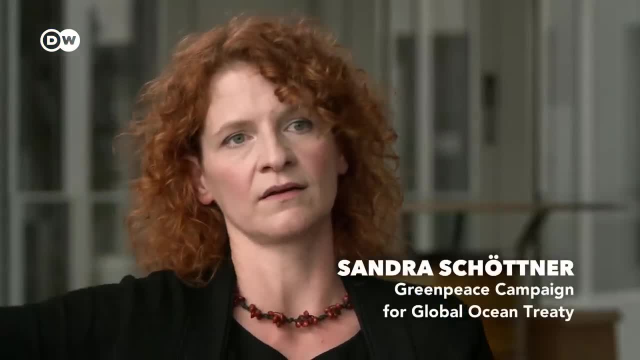 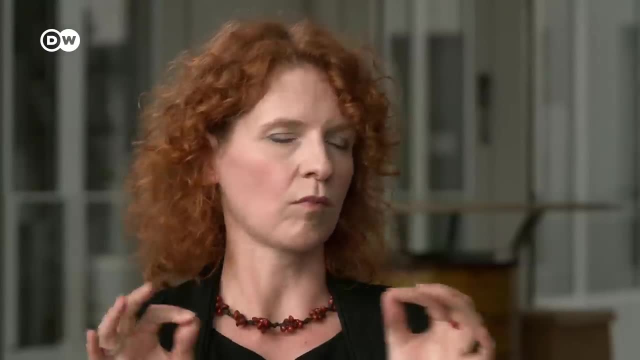 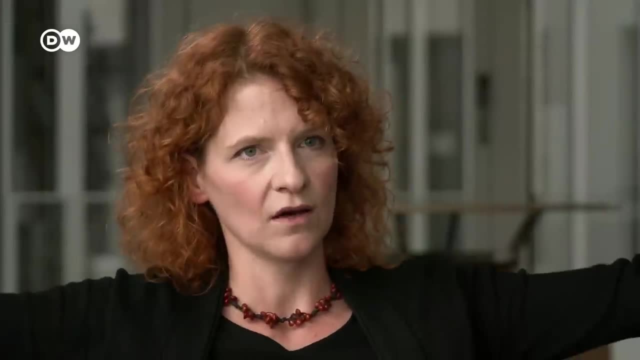 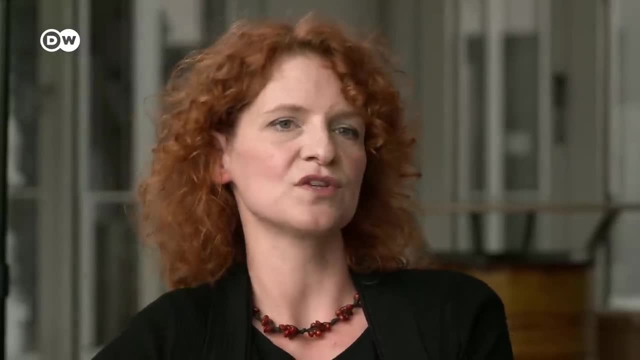 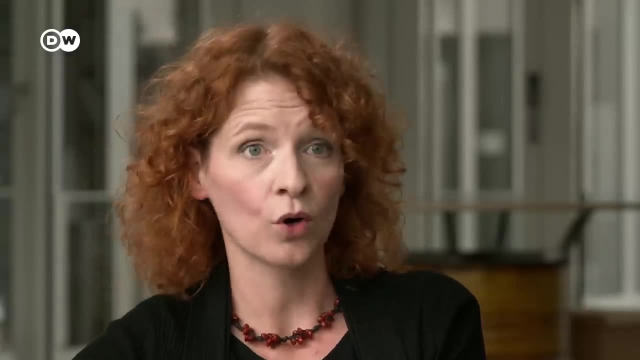 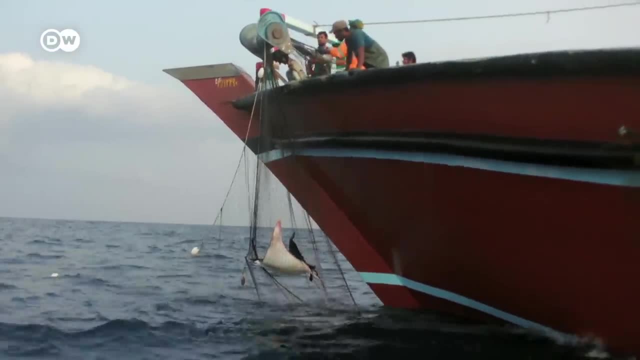 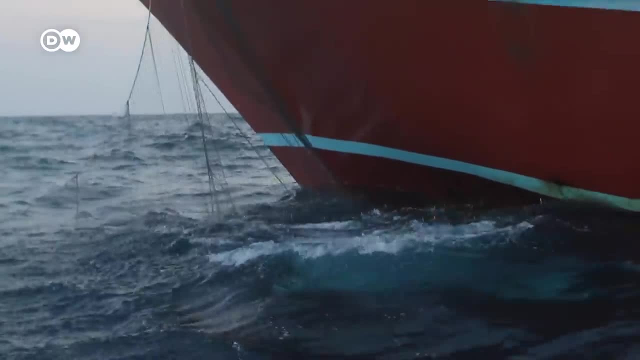 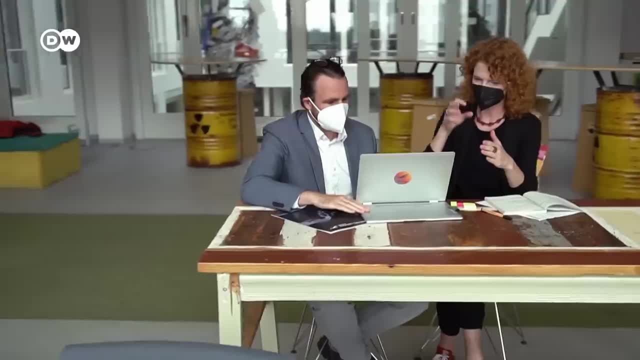 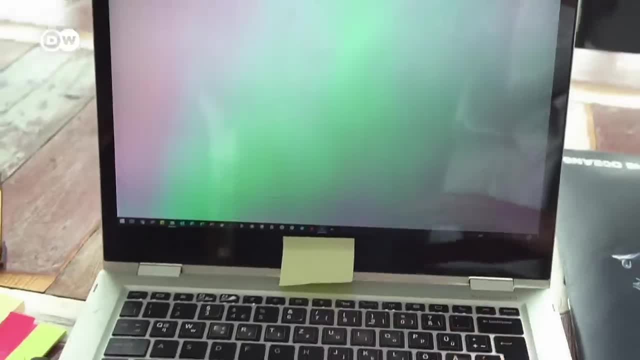 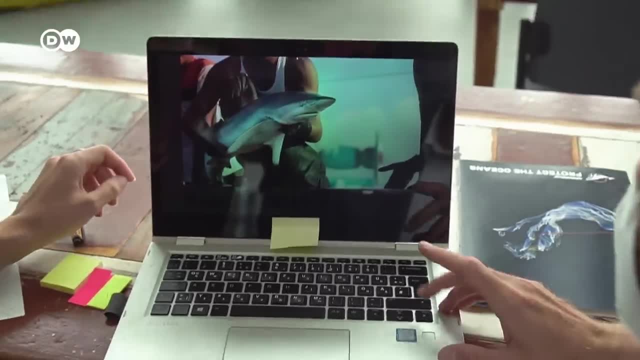 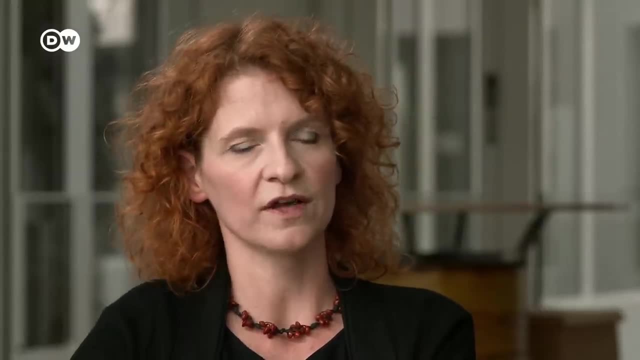 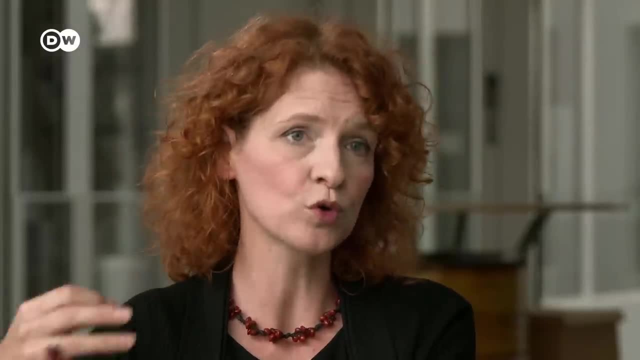 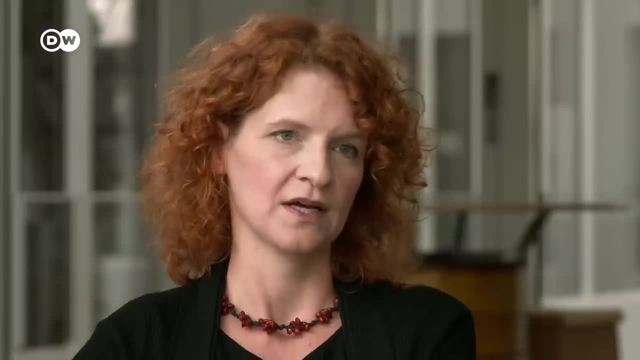 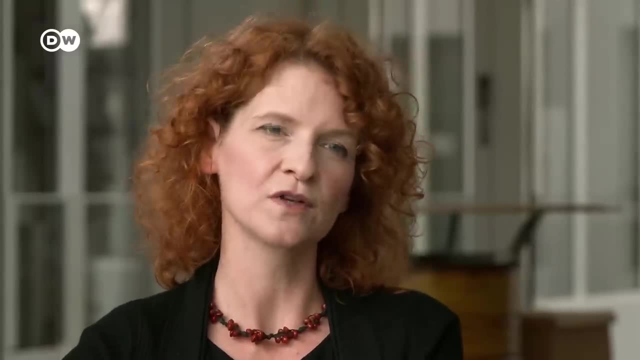 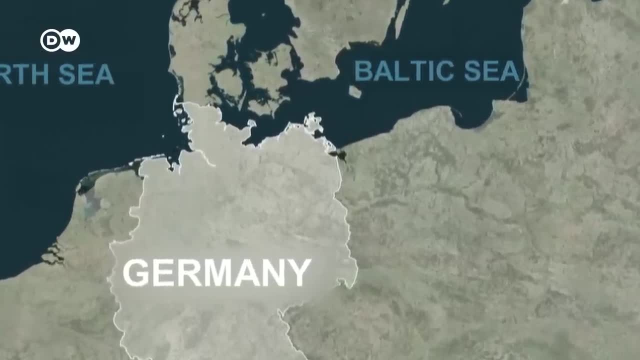 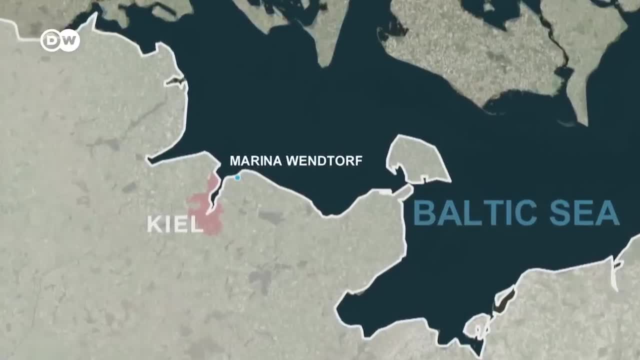 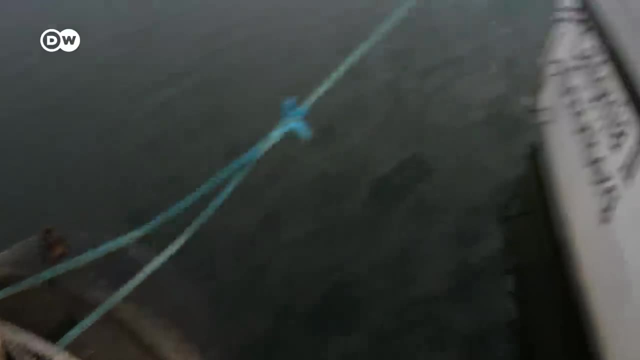 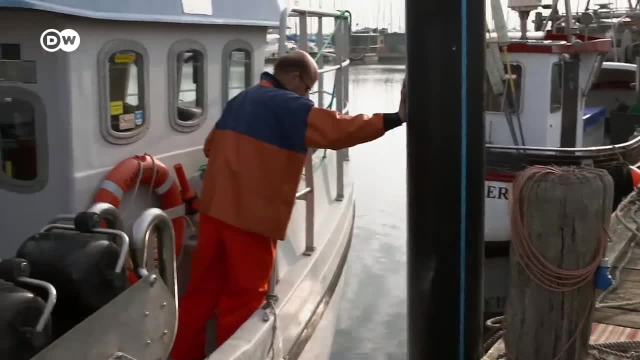 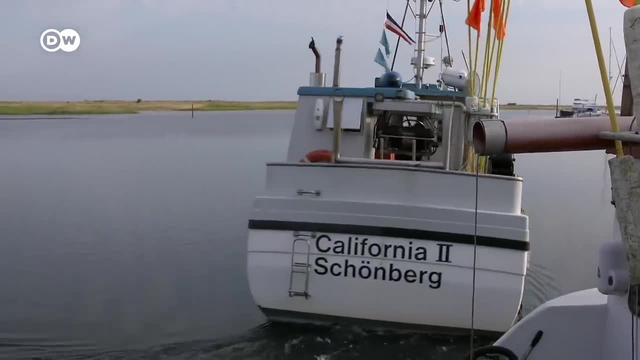 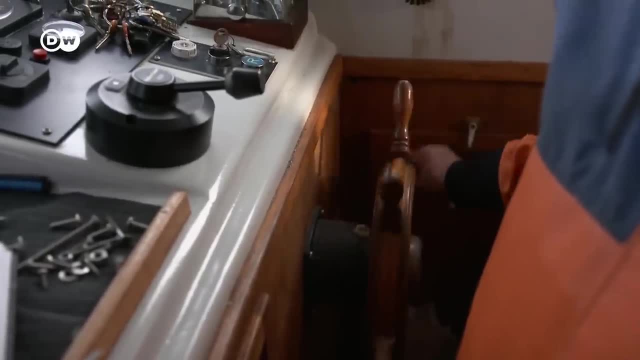 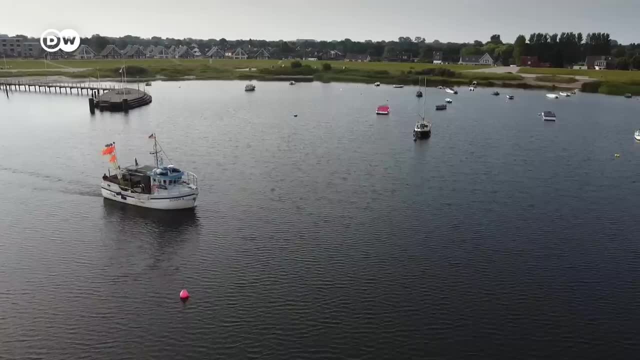 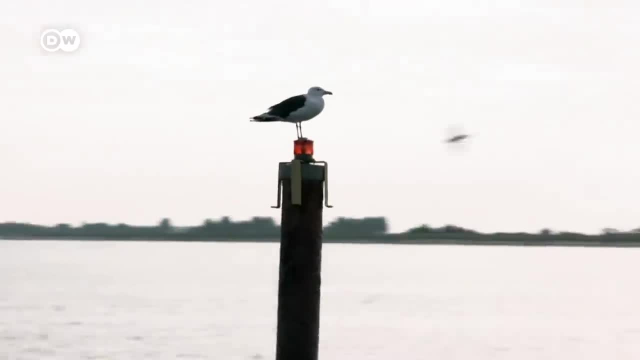 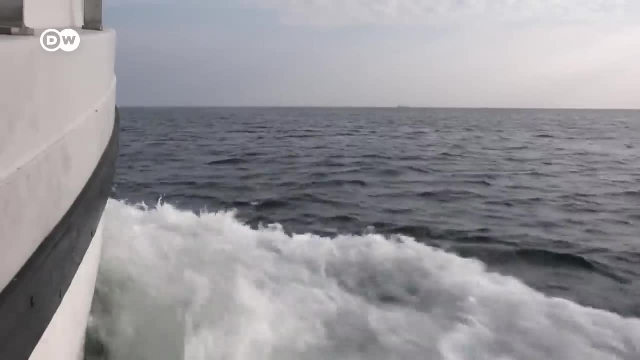 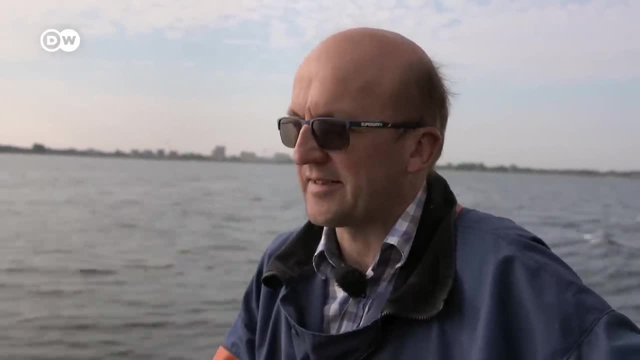 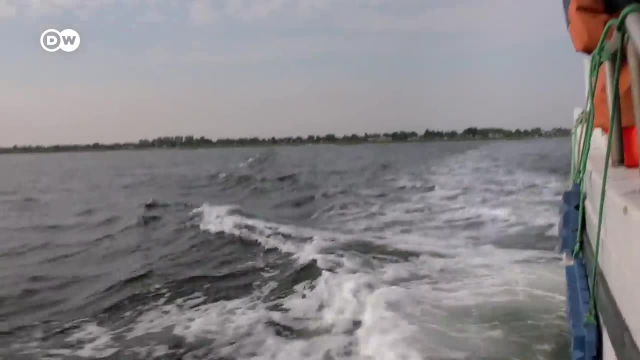 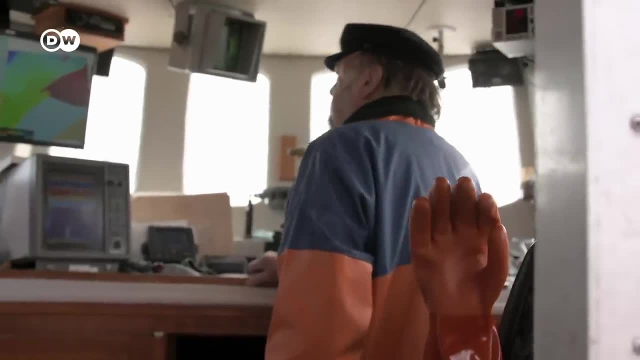 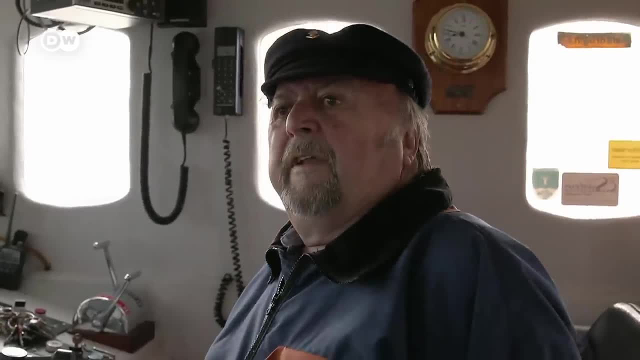 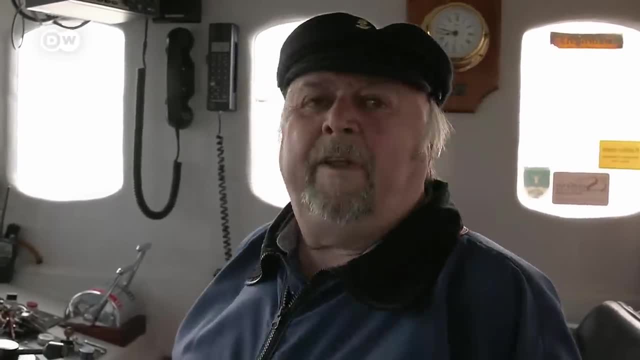 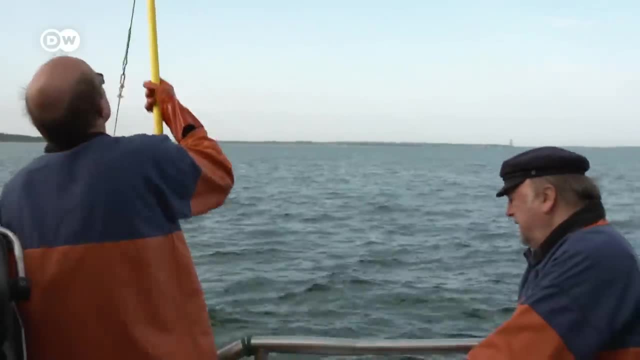 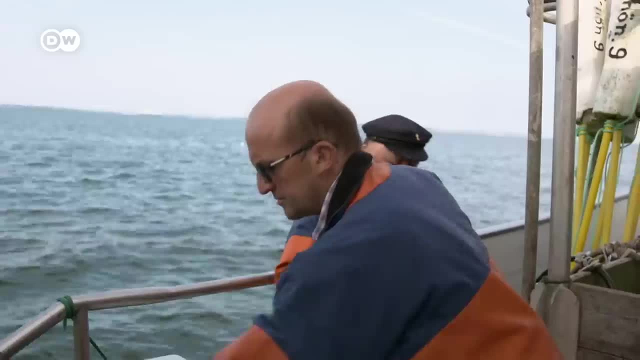 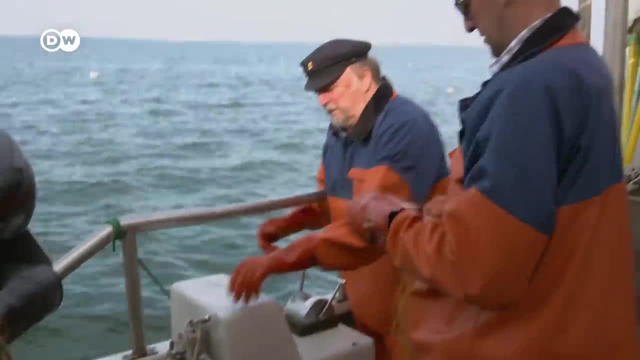 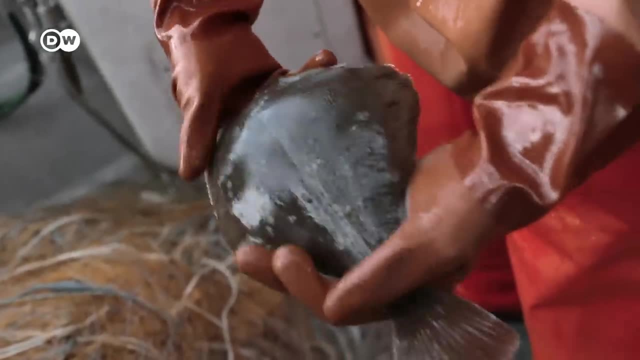 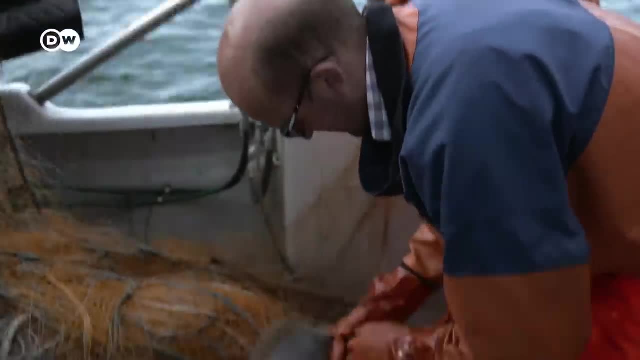 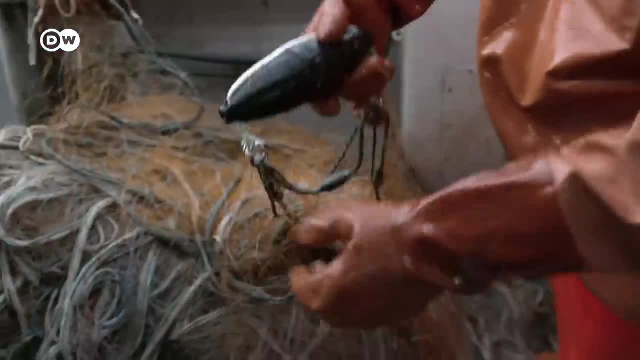 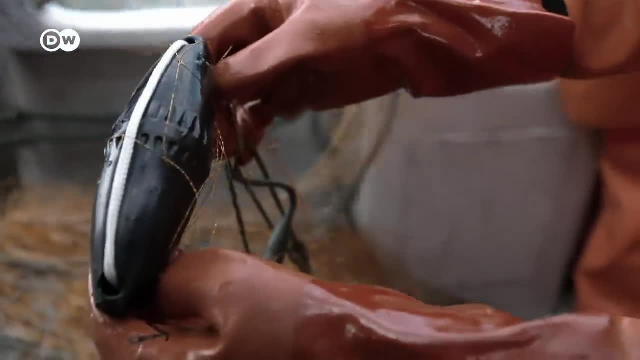 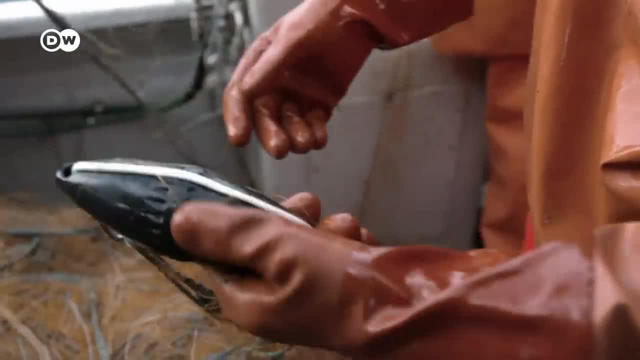 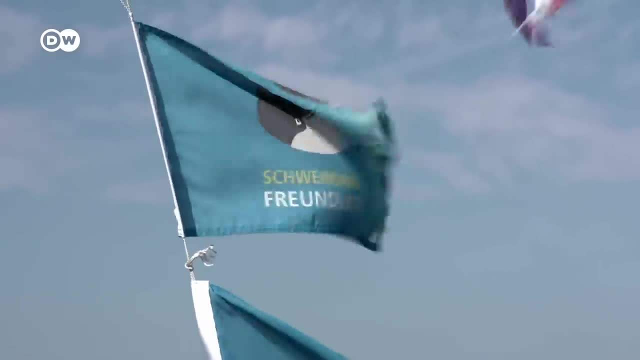 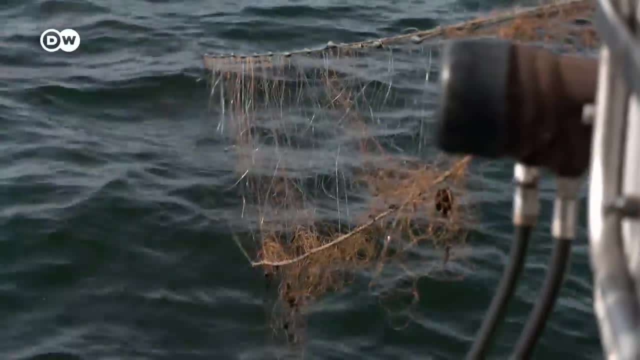 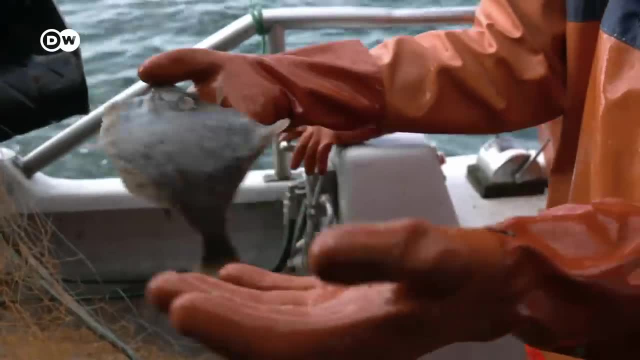 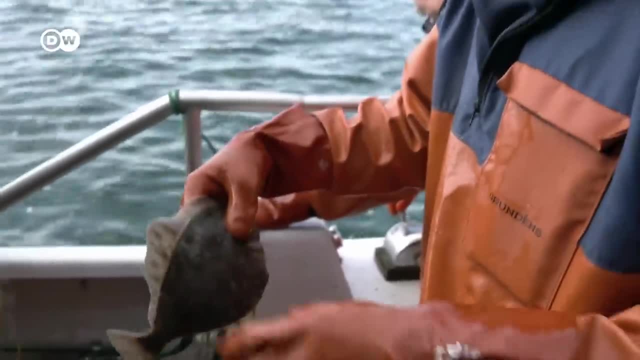 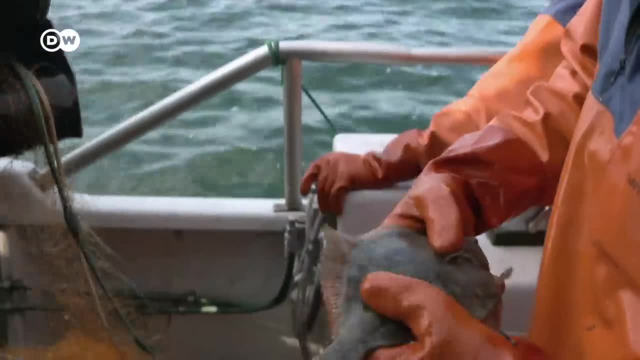 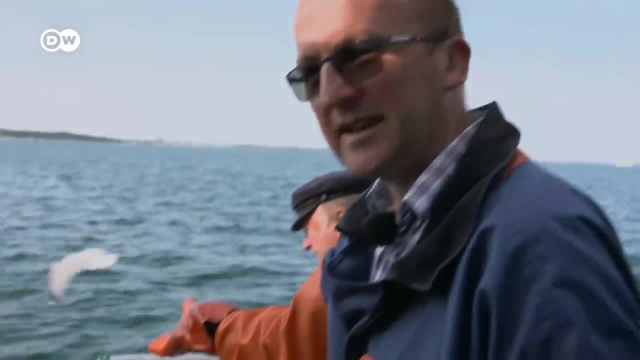 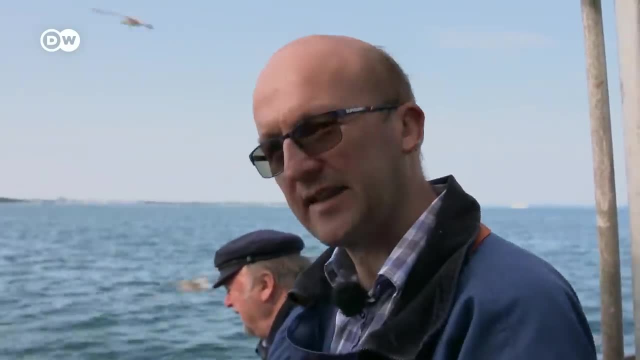 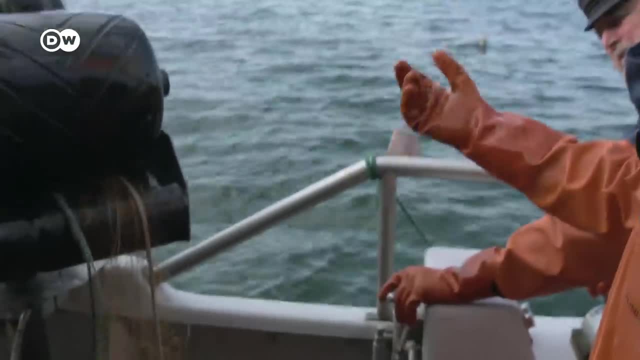 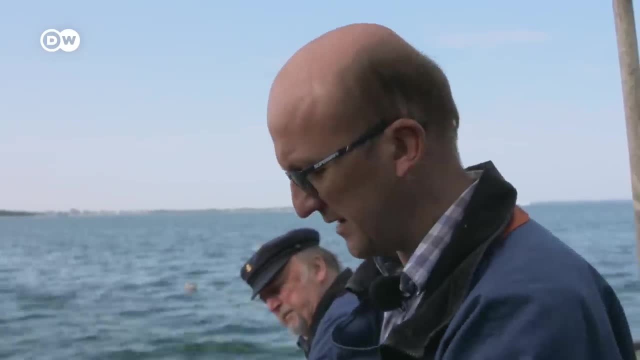 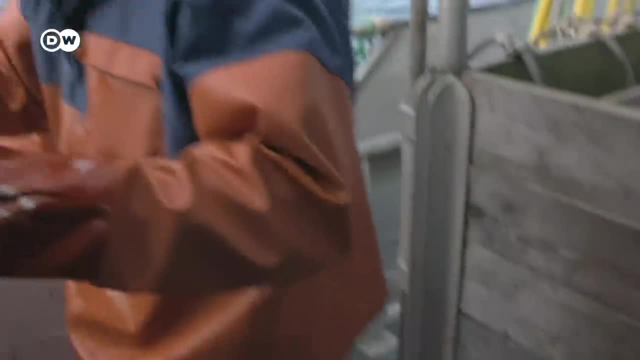 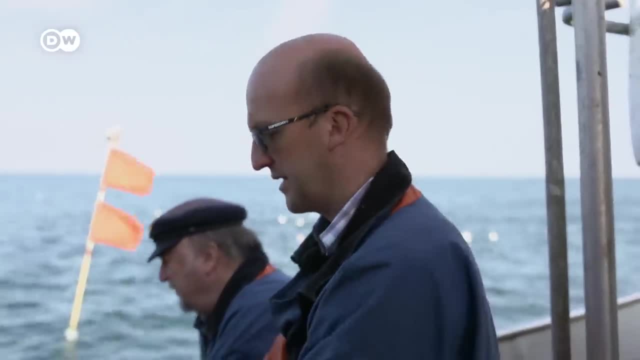 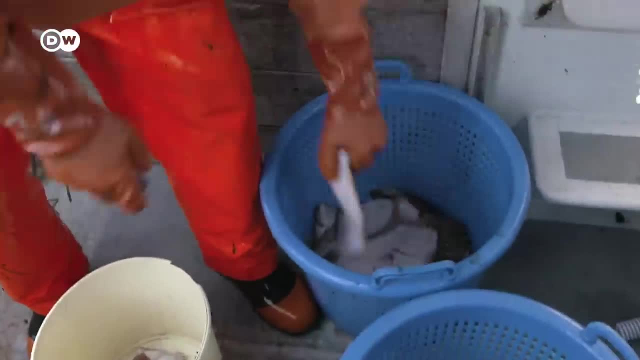 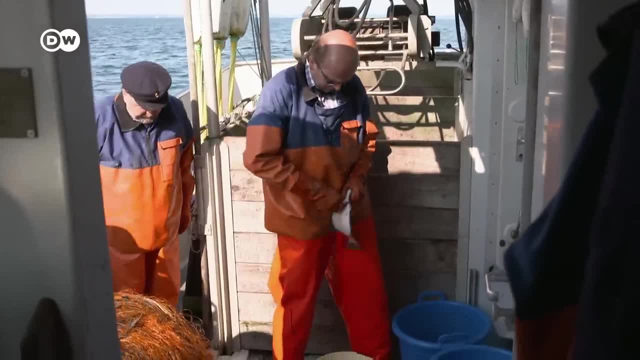 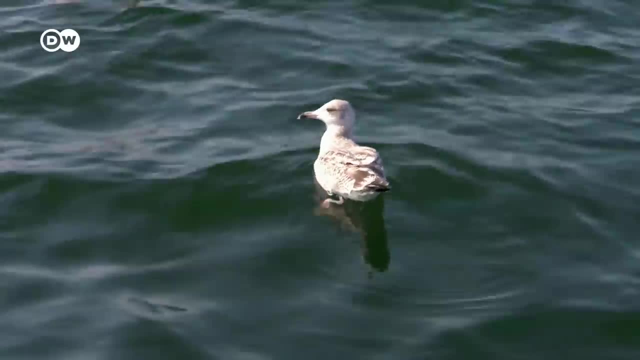 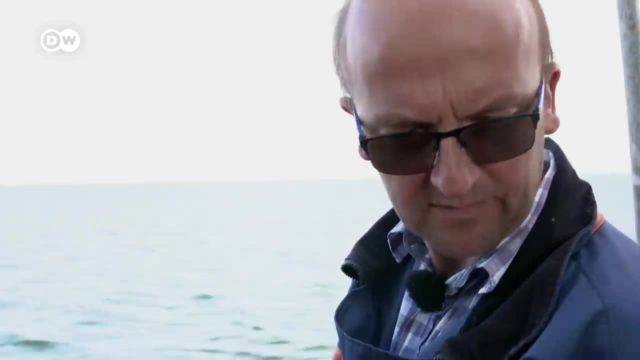 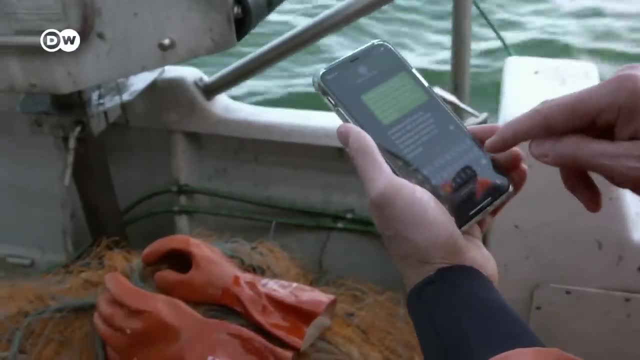 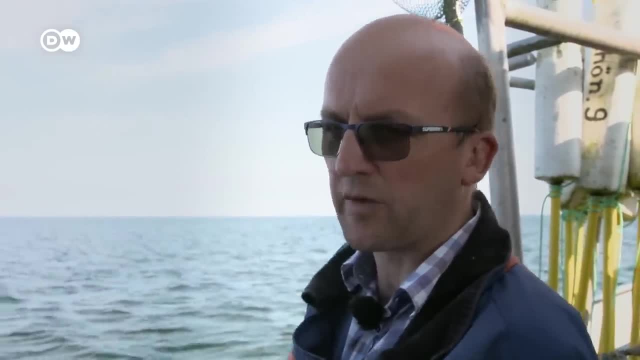 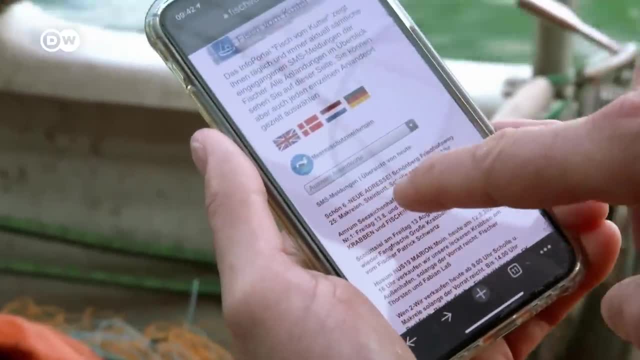 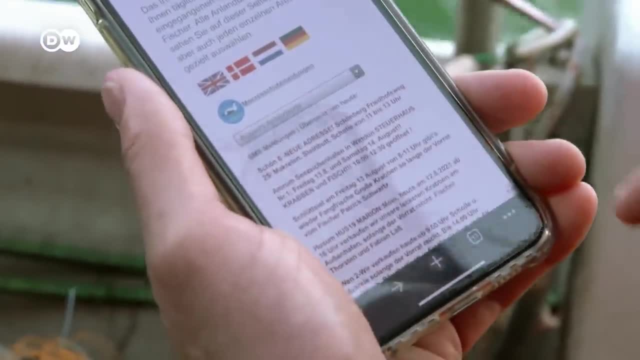 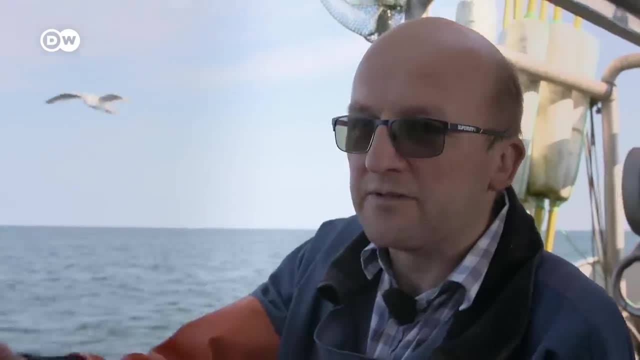 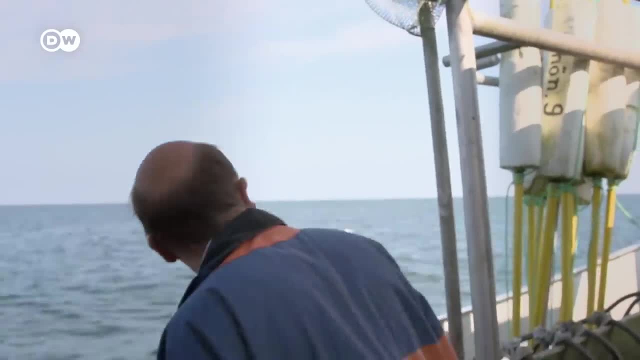 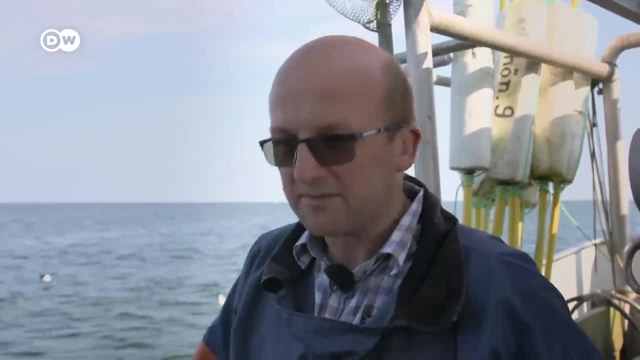 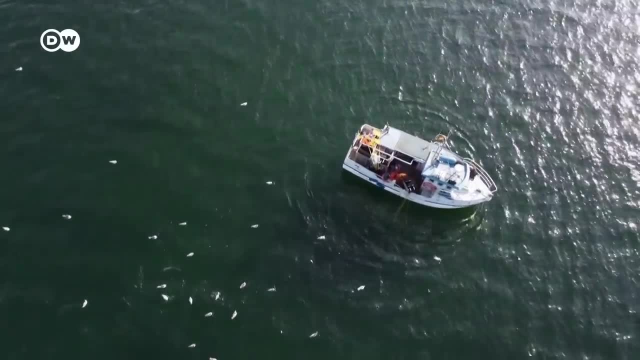 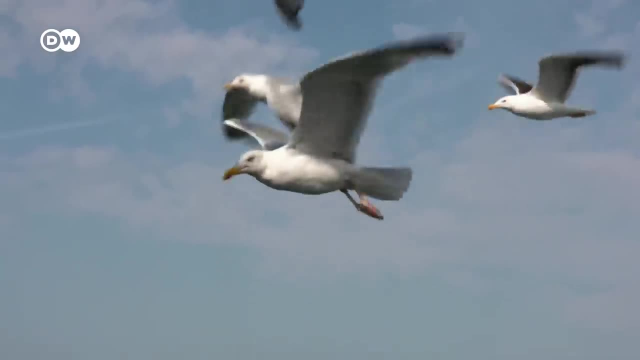 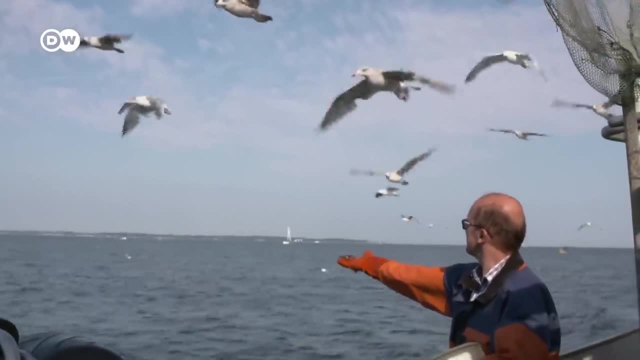 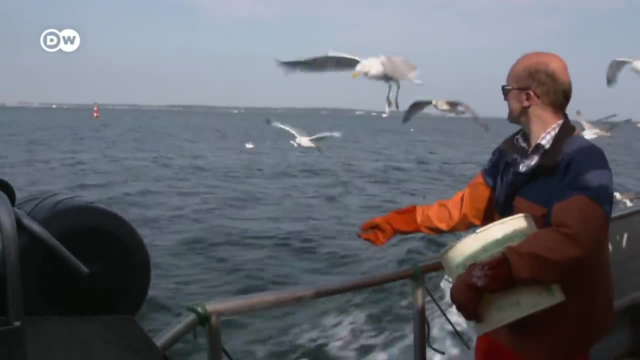 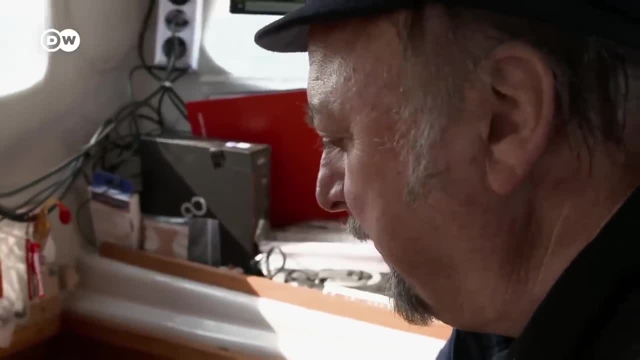 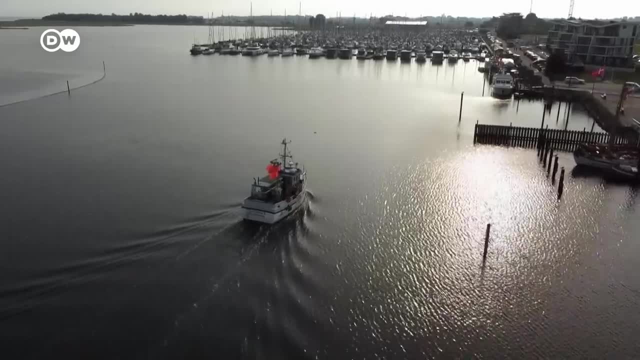 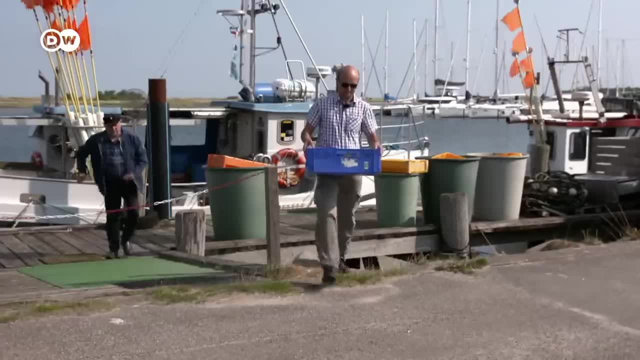 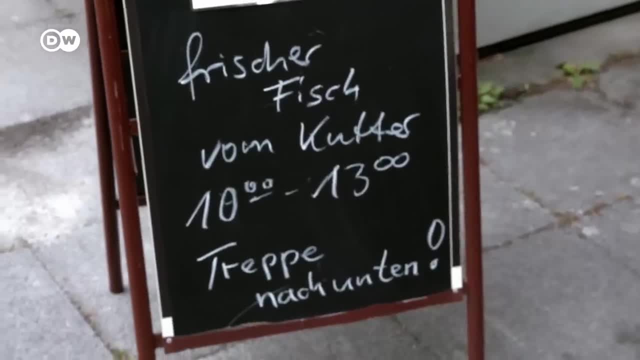 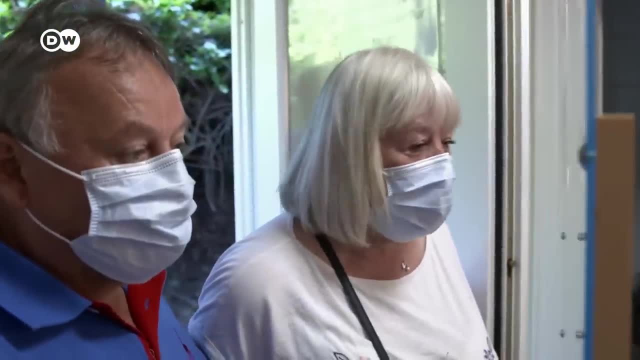 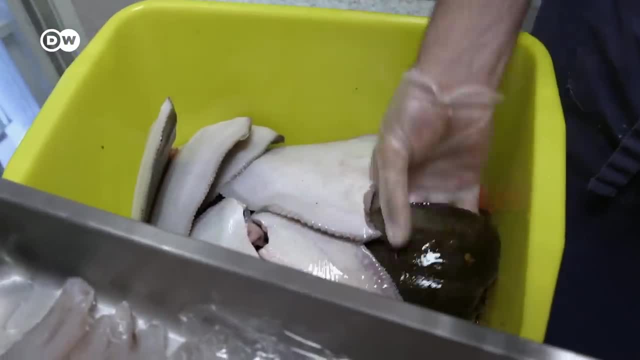 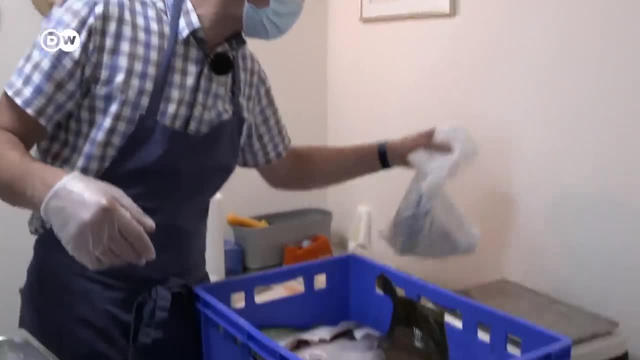 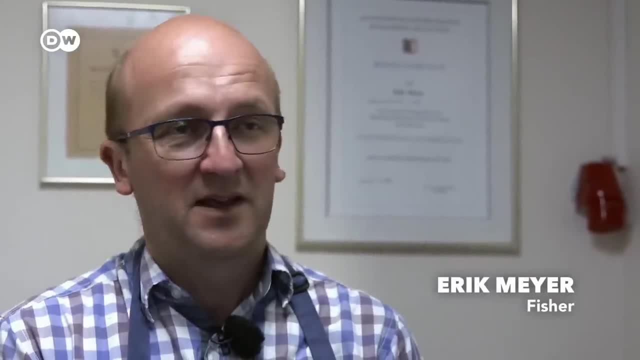 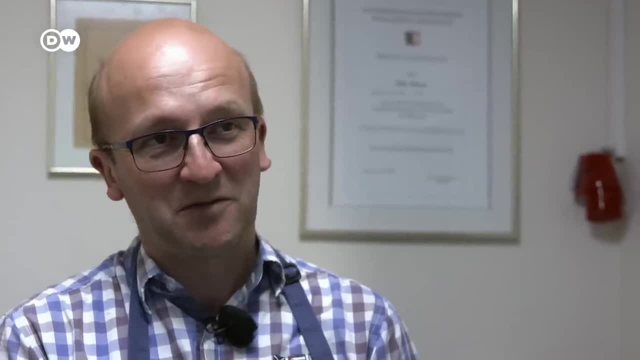 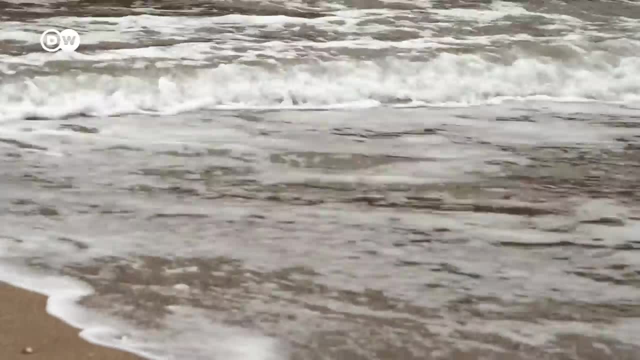 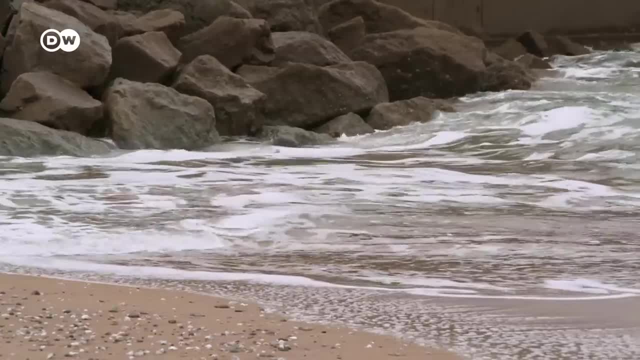 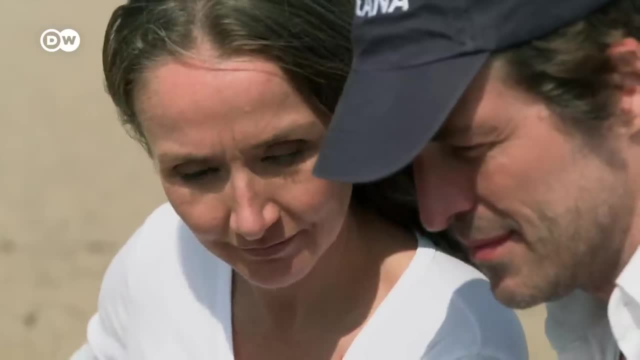 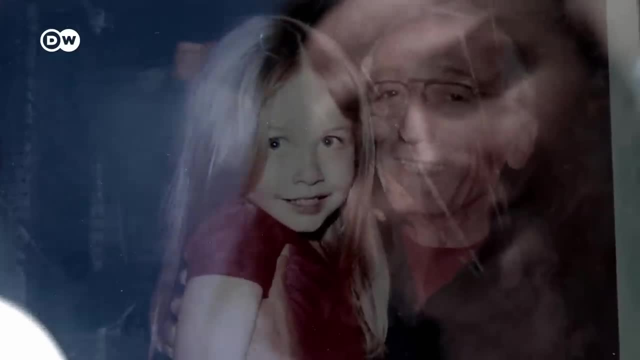 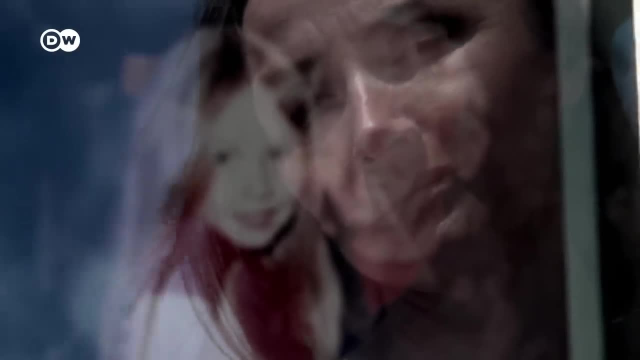 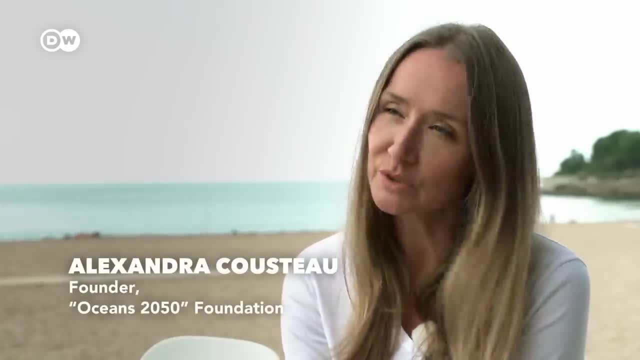 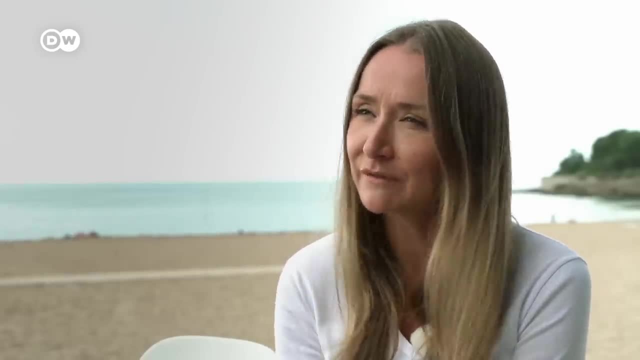 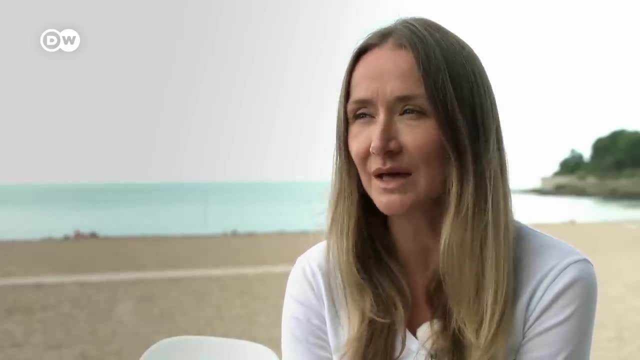 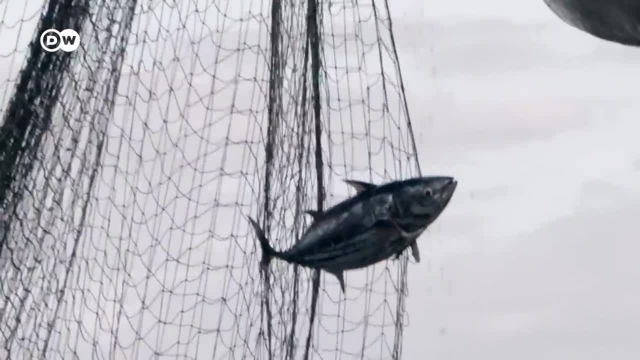 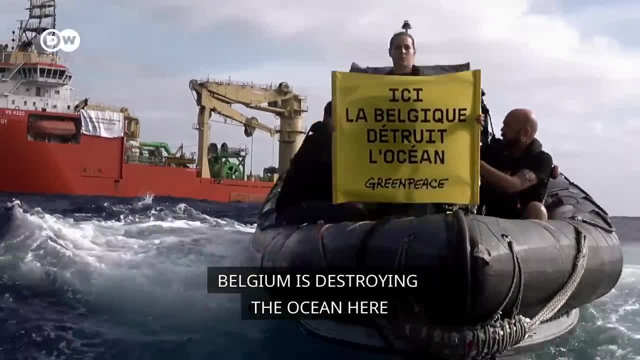 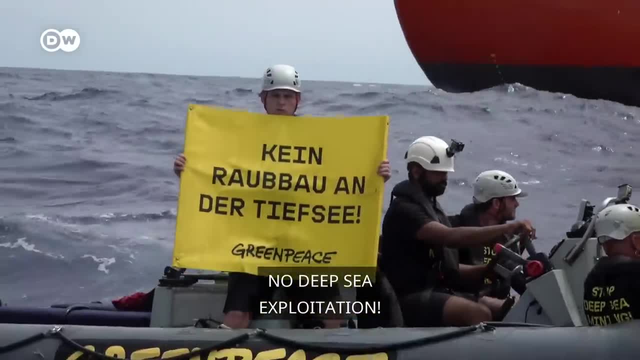 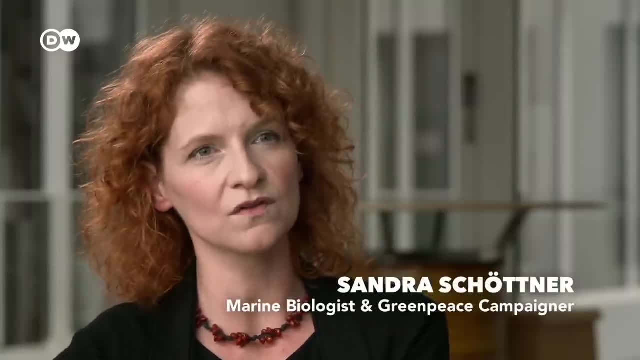 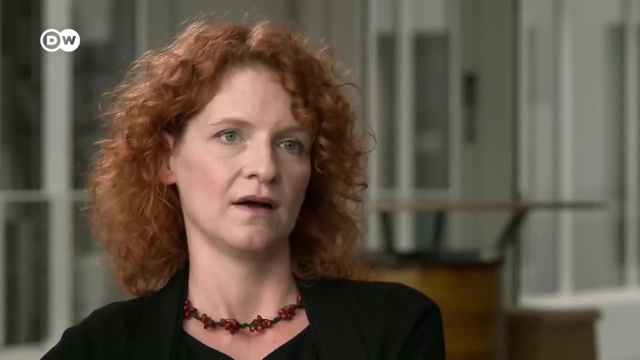 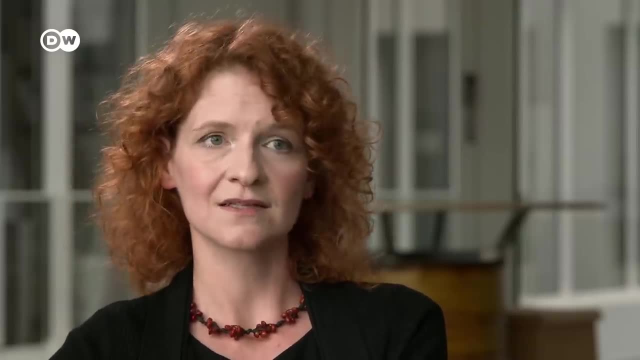 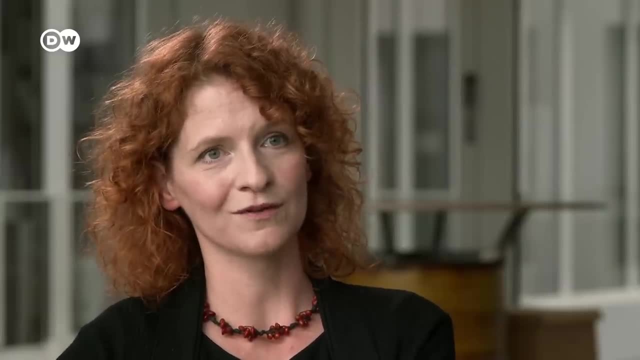 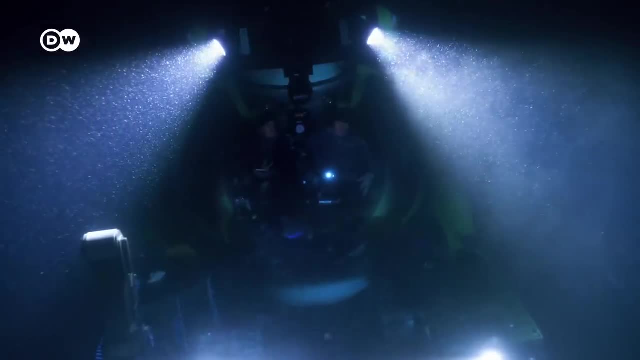 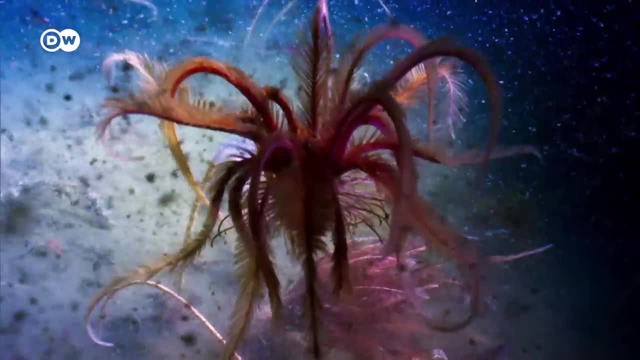 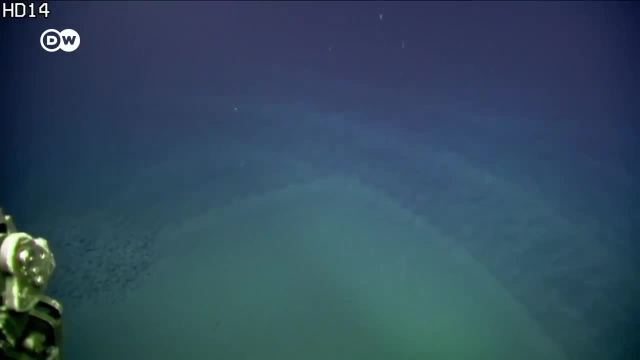 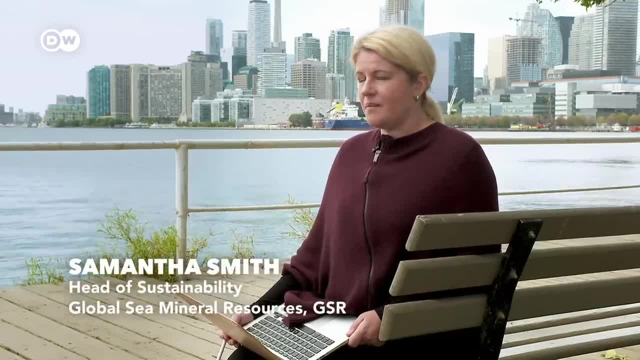 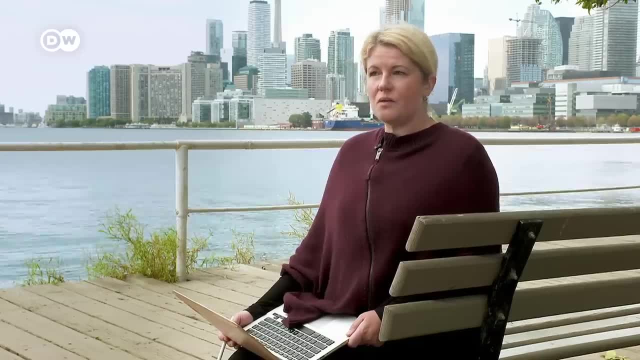 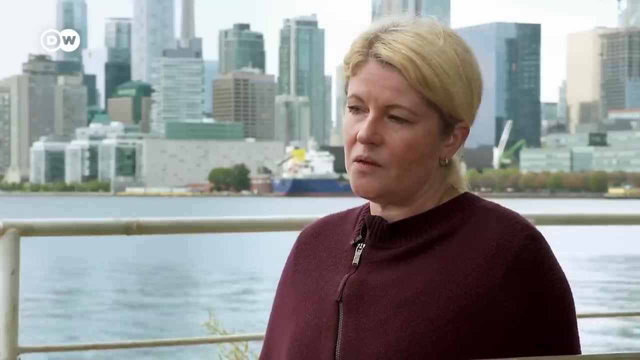 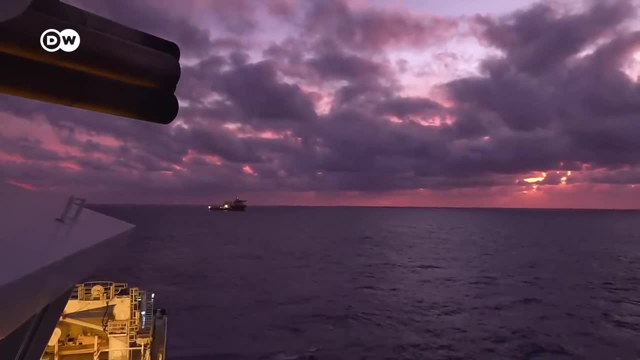 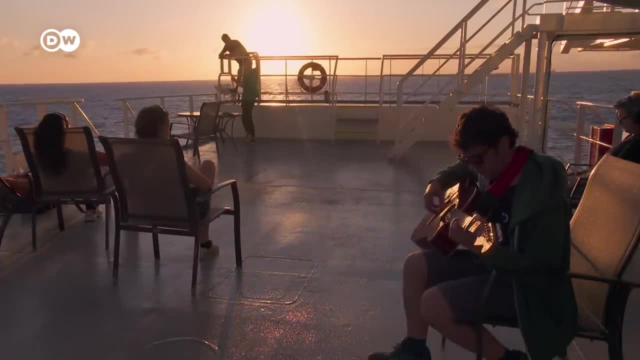 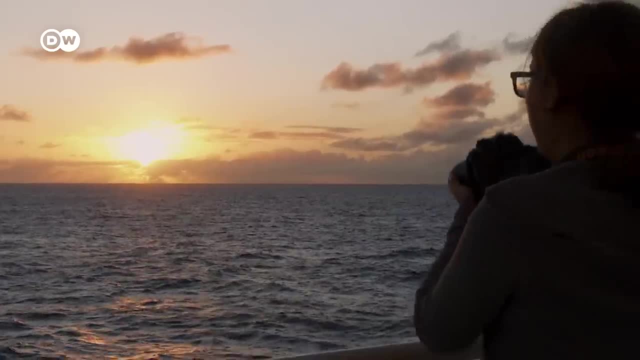 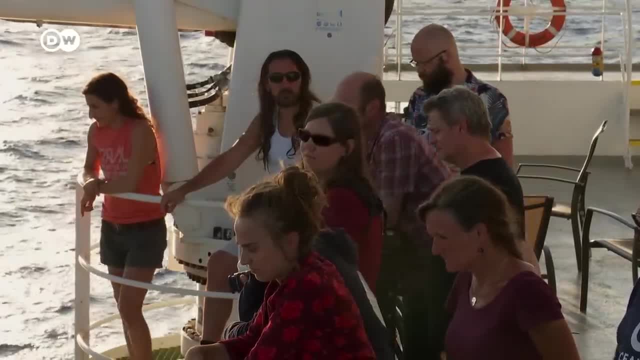 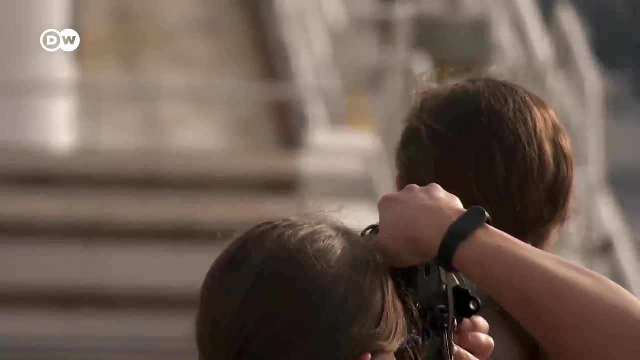 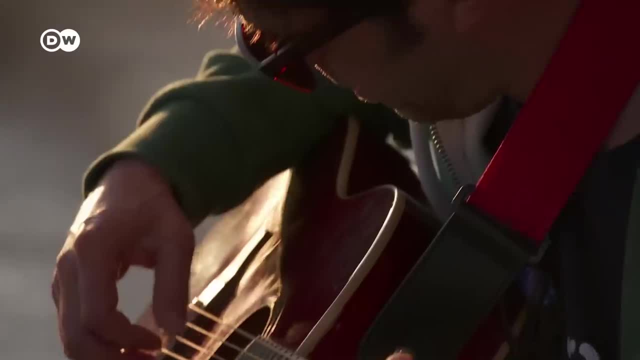 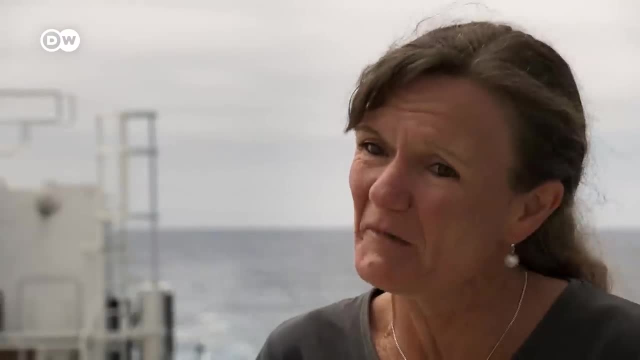 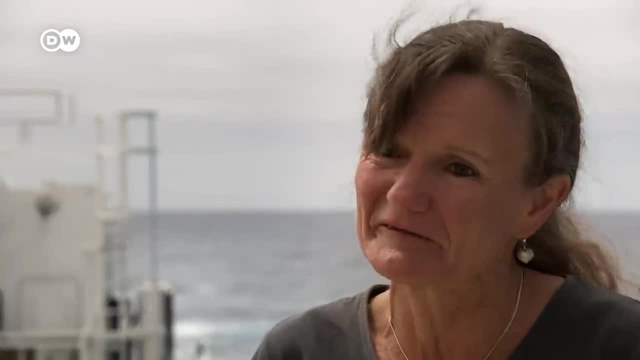 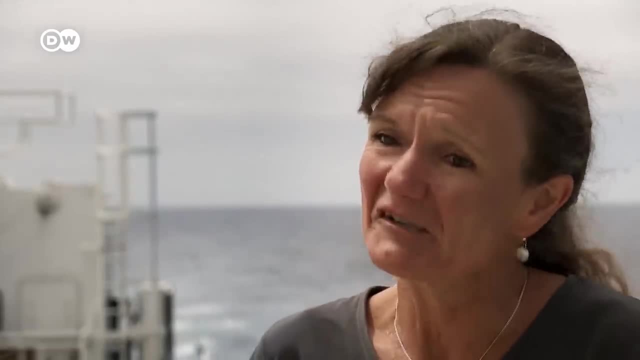 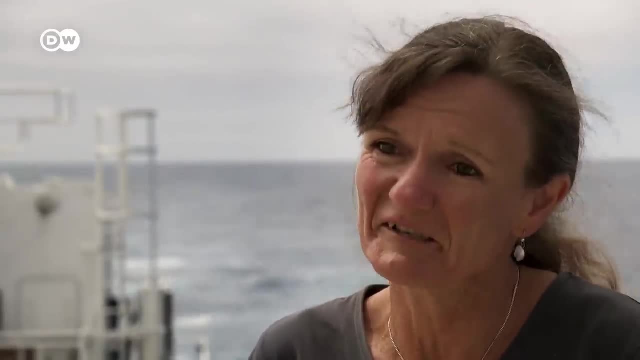 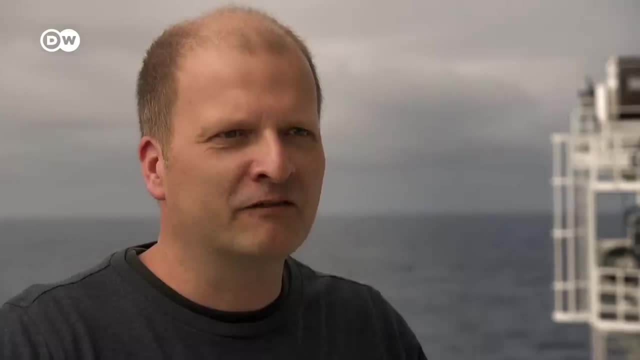 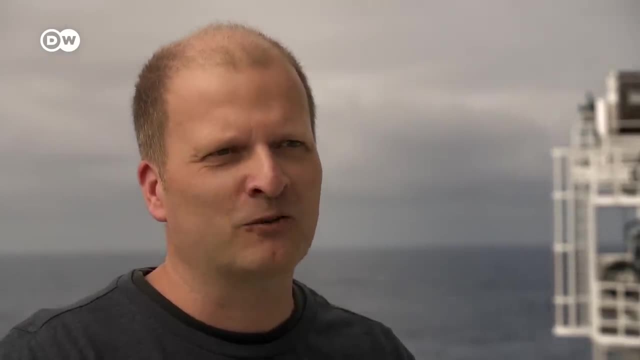 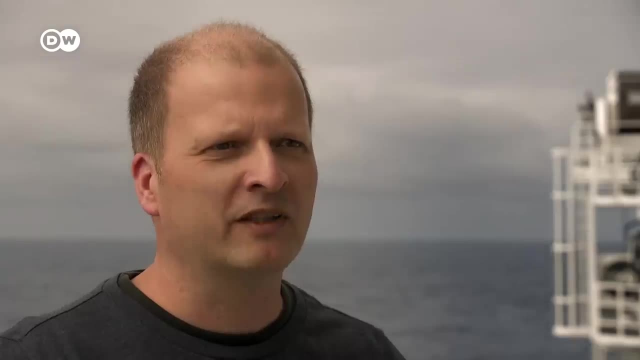 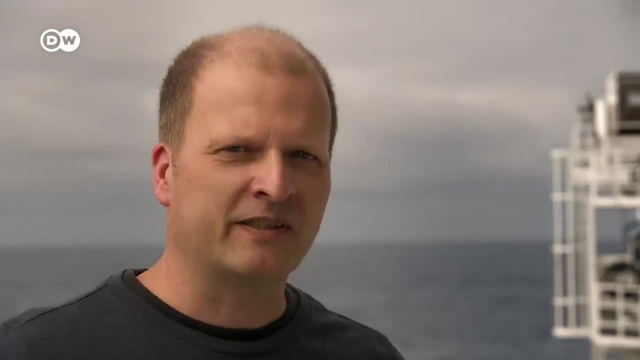 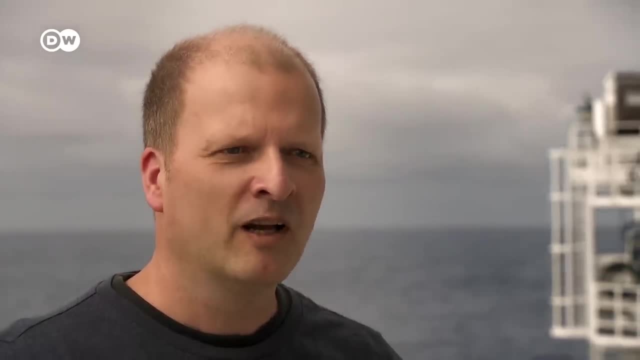 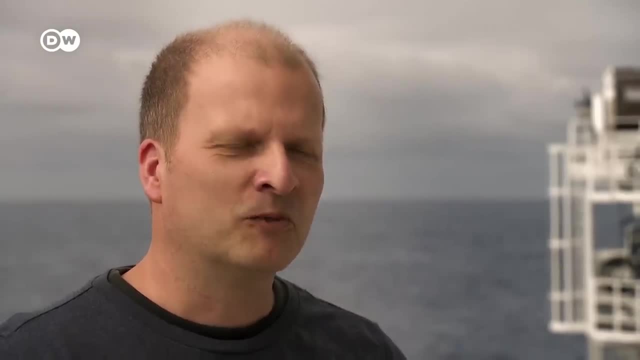 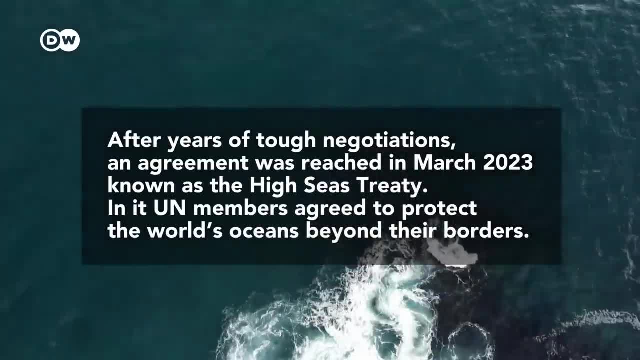